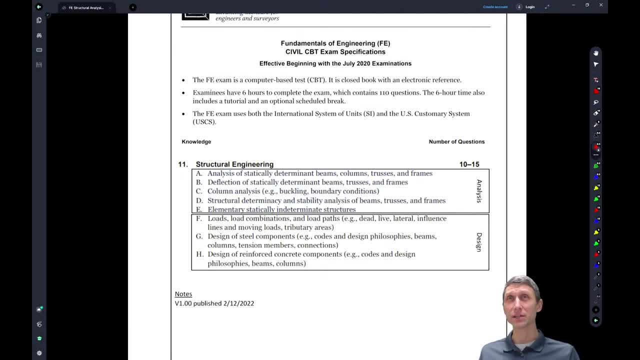 engineering, And the way that I see this is I kind of break it into two sections. Normally in a civil engineering program you're going to be taking like a structural analysis type of course, and then you're going to take some design level courses on top of that as well. So, like concrete, 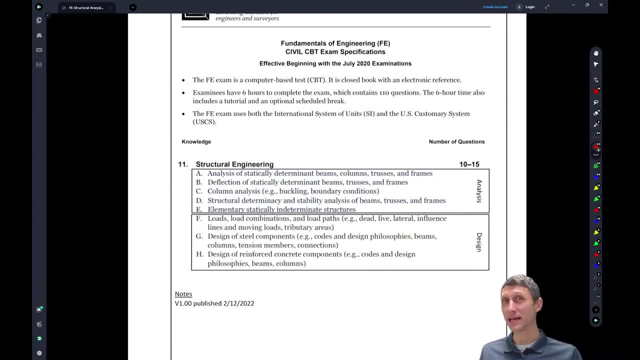 or steel design, And some of you won't take concrete or steel design, so we'll get to that next week, But this week what we're going to do is we're going to jump in on some structural analysis problems. So if you don't have the problems yet, take a look at the link below and 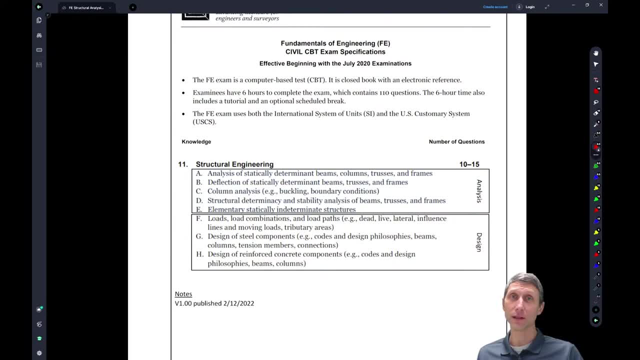 there's access to those problems with a PDF that you can follow along with, And you can print those out or do them on the screen or in a notebook, Whatever you like. But we will just get started here and hopefully this makes a little bit of sense, Because what we're going to be looking at 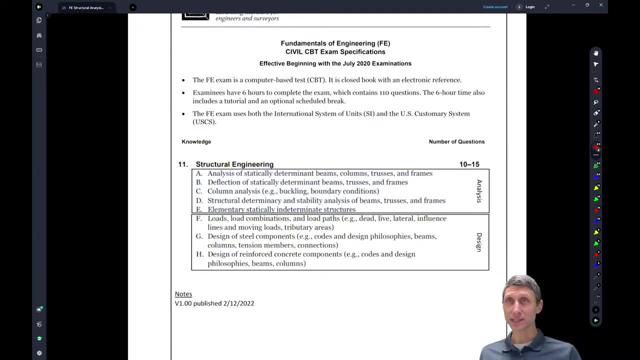 is the statically determinate beams, columns, trusses and frames, And a lot of this is kind of a carryover from a statics class, So similar things that you'd be looking at in statics, but it takes it a little. 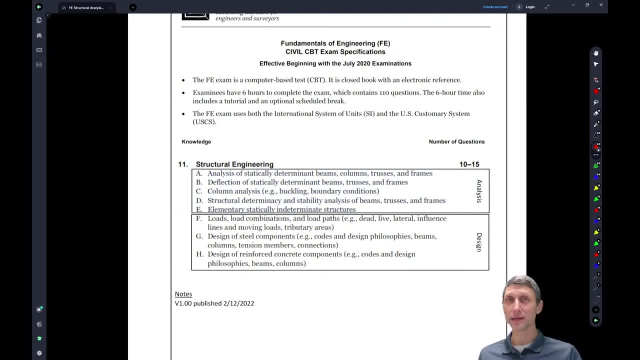 bit further. maybe the next step Maybe helps you to see it a little bit more advanced And we'll go into deflections and we'll do a couple different methods here. We'll look at the principle of virtual work, kind of briefly for trusses. We'll look at some basic beams and those sorts of 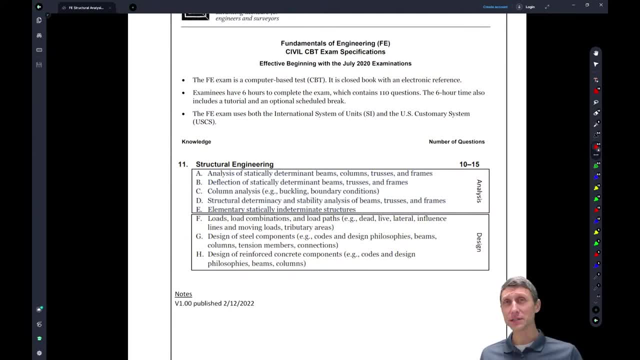 things We'll get into. columns, Columns is interesting because actually there's some column formulas in the mechanics and materials section of the review handbook But it shows up here in the structural engineering piece And even some indeterminate structures we'll take a look at. We're not going to get into like super crazy, like really long and complicated. 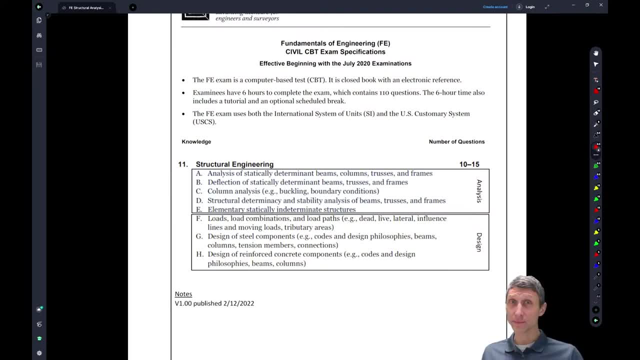 processes, But we will take a look at some of the ones that are in the manual and go from there. So, with that being said, if you have comments, drop them in the box and we will just get started here. So we went to a little too far here, But all right. The first question. This looks an awful. 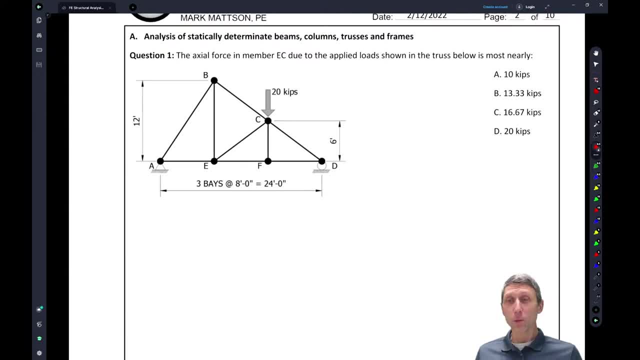 lot like a statics question that maybe we saw last time, But what this reads is the axial force in member EC. So what are we looking for? We're looking for member EC. So right here, this member, here the axial force in that member, due to 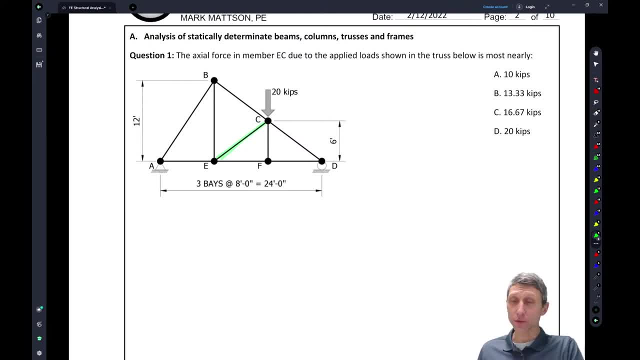 the applied loads shown in the truss below is most nearly So. to remember, with trusses we're not dealing with self-weight. We're going to ignore the self-weight And what we're going to do is we're just going to take a look at that one member. So this truss is 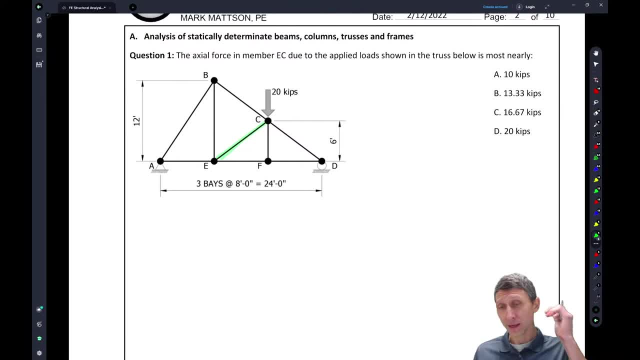 a little bit more complicated than some of the ones we've looked at. Some of the trusses are parallel cords And what you can see here is these. you know top cord and bottom cord. They're not parallel, So it makes it a little bit more complicated. You can't just do sum. 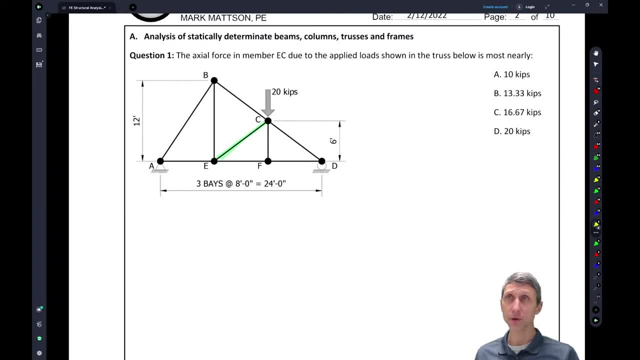 of forces in a y direction or x direction. to get a component here You really kind of have to use the sum of moments formula. And I like this question for a number of reasons. One, because it really focuses you in on that sum moments question. But two, if you think about it right, you start to understand trusses. 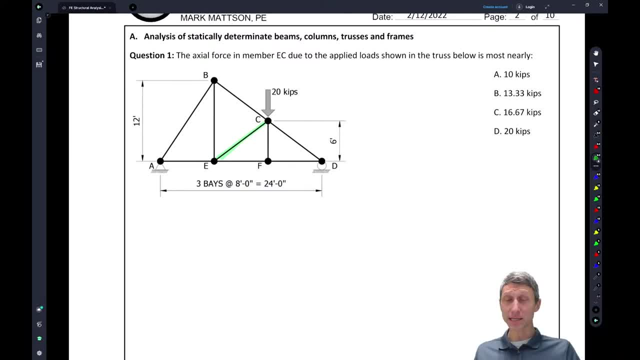 a little bit better. It's going to help you with this process of solving them. So this is going to use the method of sections And to do the method of sections. what I like to do is I like to kind of draw a section around, a part of it, And the reason I'm drawing. 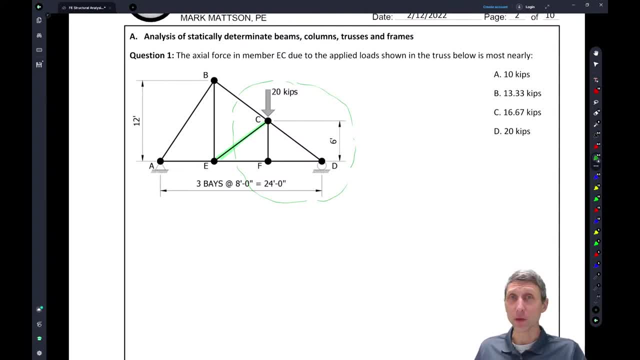 the right side is just because it looks simpler to me. OK, so the right side looks a little bit simpler, simpler. I kind of like this little, this little truss in here Right, And you know, it just looks a little bit, a little bit simpler. So what I'm going to do is I'm 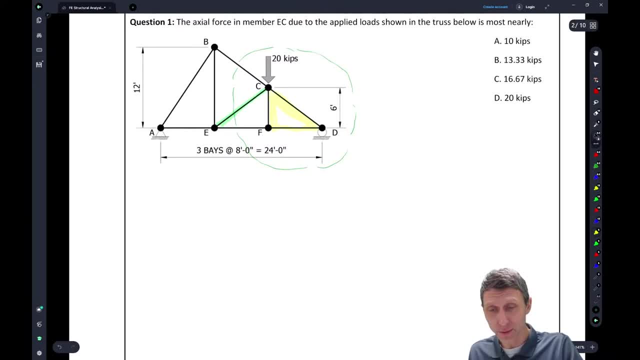 just draw a free body diagram of that and then we're going to take a look at it again. So I'm just going to copy this down here to draw my free body diagram. All I'm doing is kind of redrawing this thing, and I'm not probably drawing it perfectly here, but just read around. 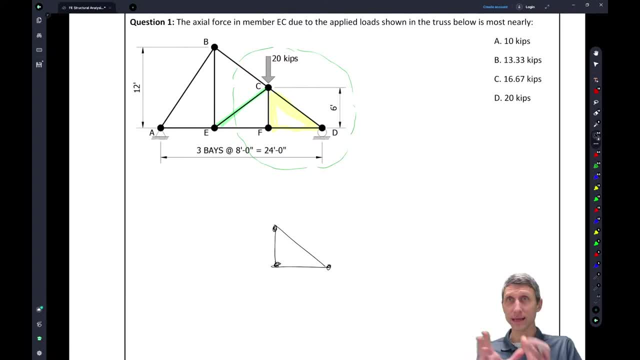 that section And what I like to do is just take that, the yellow triangle first, Right. So we have what C, D and F had back the forces that are known. So we have maybe 20 kips here And we know that we have some reaction D, Y at a roller. So there's going to be some. 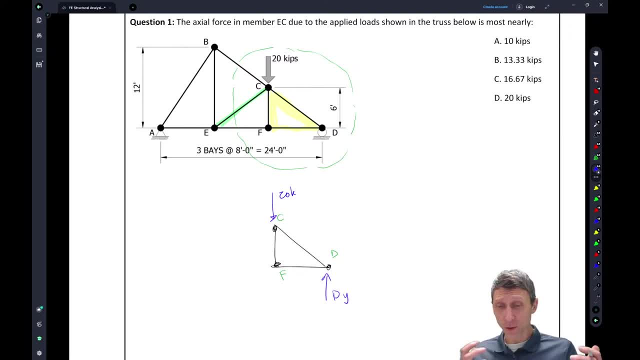 vertical reaction at a roller, And then what I like to do is I like to just always assume tension in trusses, So that way if I get a negative value, I know it's compression. But what I like to do here is I'm just going to start in and I'm just going to draw my 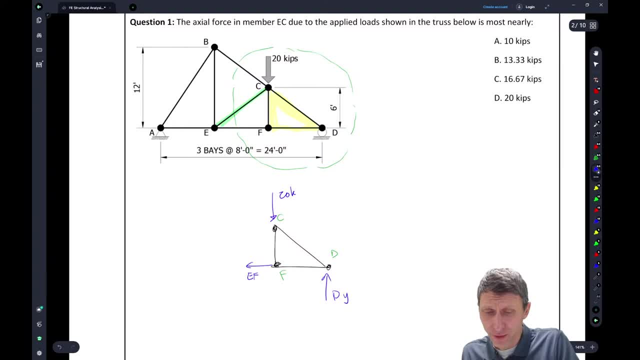 forces that I don't know. So I'm going to draw- Yes, I'll draw CE And I will draw BC. So this is kind of a basic free body diagram. This is kind of the basic free body diagram, kind of step one when you're getting into trusses. So that's where we're going to get. 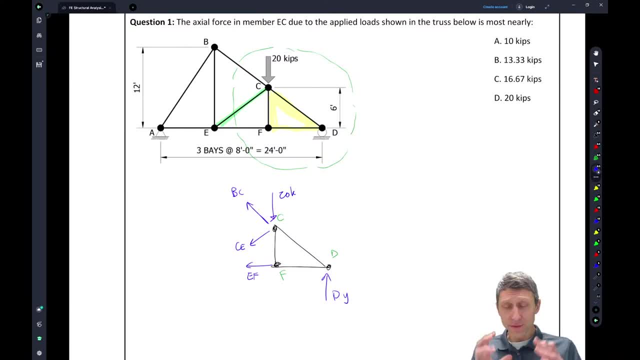 started with this, And then what we have to take a step back is okay. so we're still trying to find this force, this CE force. So what I like to do whenever I get a question like this is to look for one of two things. One: is there a parallel top and bottom cord? 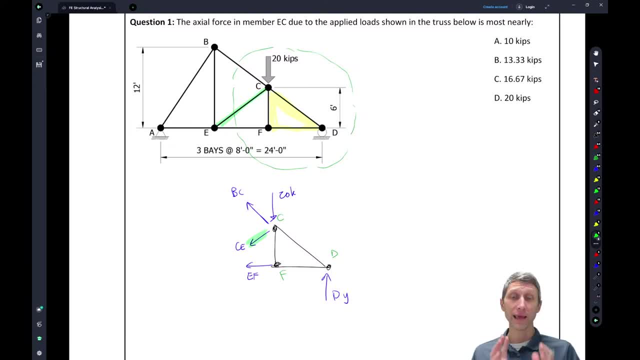 Because if so, then I can just use some of the forces and find components. If not, what I like to do next is I'm just going to come back here and get a couple of colors. So what I like to do next is kind of look and see. are there any points of intersection of the? 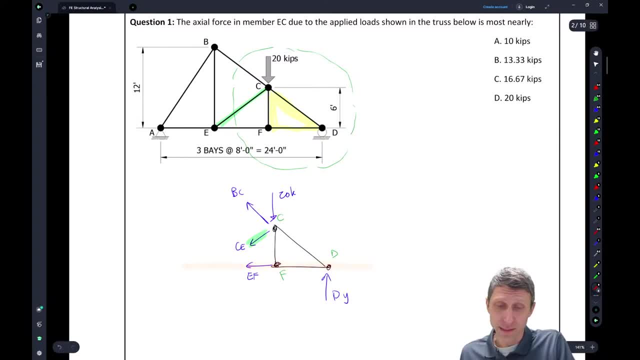 unknown forces that are going to be a convenient place to take a moment. So, in other words, I'm going to draw a line right through EF. that red line I just drew on the screen, That's a line through EF. That's kind of the line of action of EF. That's the line that EF is. 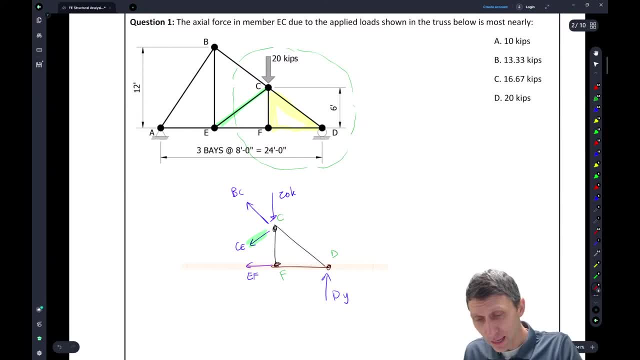 passing through, and that's where it's acting. And, similarly, I like to do the same thing. So I'm going to draw a line through this point. So I'm going to draw a line through this point. So I'm going to draw a line through this point. 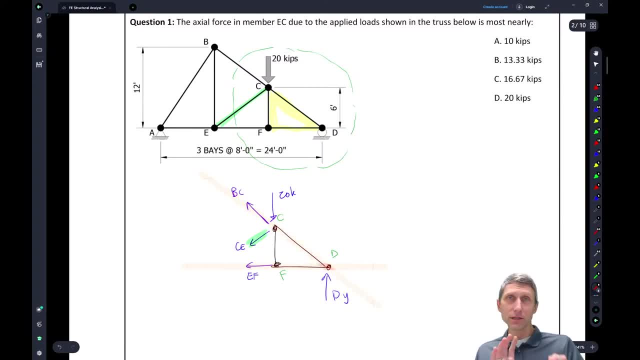 to draw one through BC. And when you do that, when you're doing method of sections, this is actually a really cool thing, because what you see all of a sudden is there's a point of intersection there, And that point of intersection is an important point, because that point is 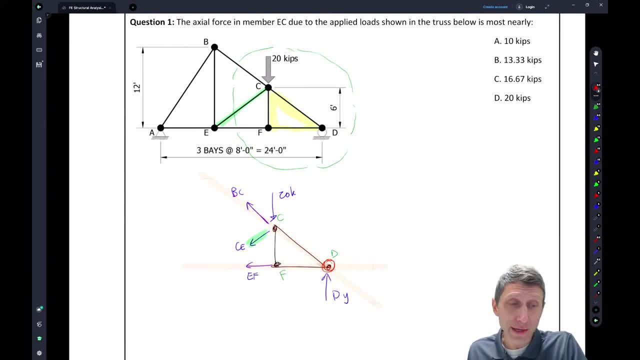 going to tell us where we can sum moments effectively. So for this question, what I'm going to do is I'm just going to sum my moments about point D. Okay, so if I sum moments- and this is just a sigma moment- about point D equals zero, And it's funny, I was showing some of this. 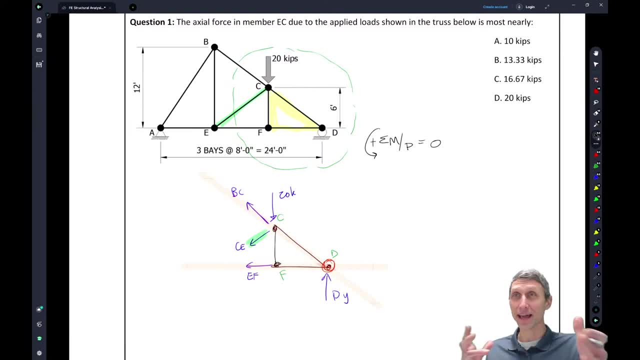 stuff to my sister-in-law, who's a algebra teacher. She teaches algebra like all day, every day. She's like Mark, that looks like Greek And it is Greek. There's a sigma, But she 100% has the algebra. And you guys, I know you have the algebra too. The algebra is not the. 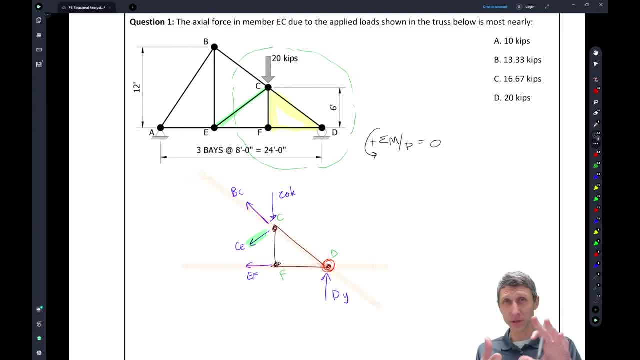 hard part. The hard part is writing these equations and using these weird letters and putting them into practice. But all that we're doing here is a moment equation. We're looking for force, times, the distance and trying to figure out what forces cause moments. So, right away, 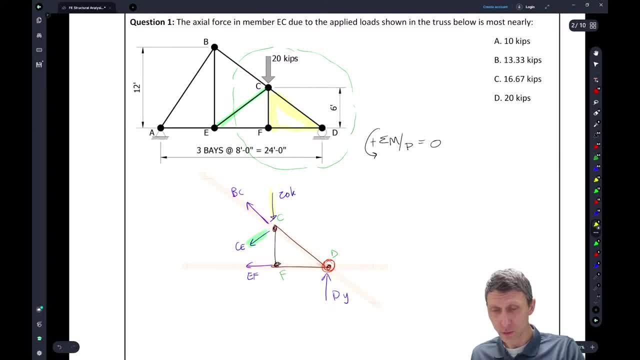 what we can see is there's a couple forces that don't pass through point D, This 20 kips and our force CE. So those two forces have to balance each other rotationally in this free body diagram when we sum moments about point D- Anytime I'm summing moments- I can apply that force, that unknown. 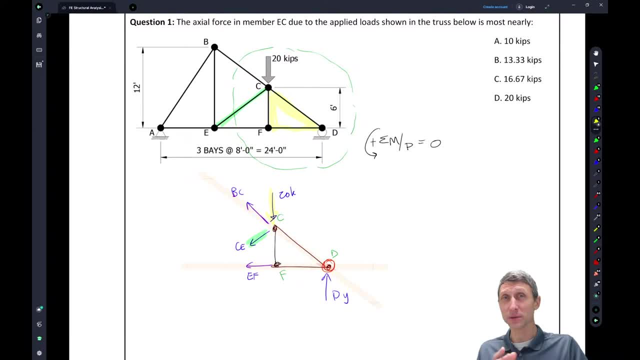 force like CE, for example, anywhere along its line of action. In other words, if I put a rope and pulled it somewhere, I could put that anywhere along its line of action and it will cause the same moment. So if I take that force, for example, right, and I say, well, what's its line of action? 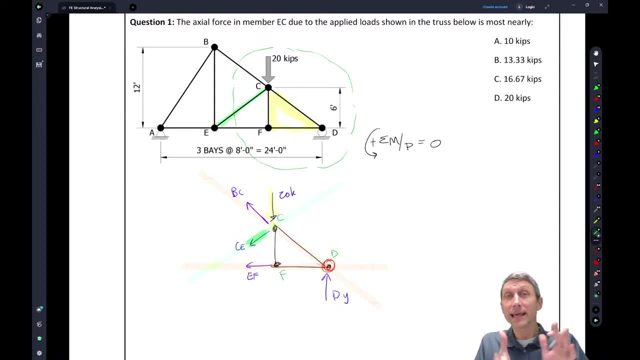 look like It, looks like maybe this green line. You'll see that green line doesn't pass through point D And that's important because if I put that force, CE, anywhere along that line, it's going to create the same moment: about, about point D. 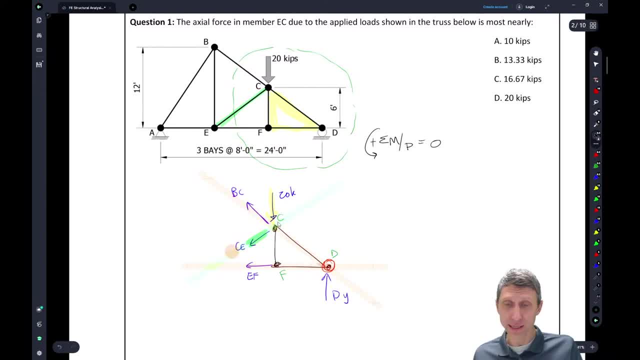 So I can go anywhere along this line here and that force CE is going to create the same moment. So what I like to do, I mean if I knew what this perpendicular distance was, that would be great. If I knew that perpendicular distance I could solve for it directly. I don't know that. 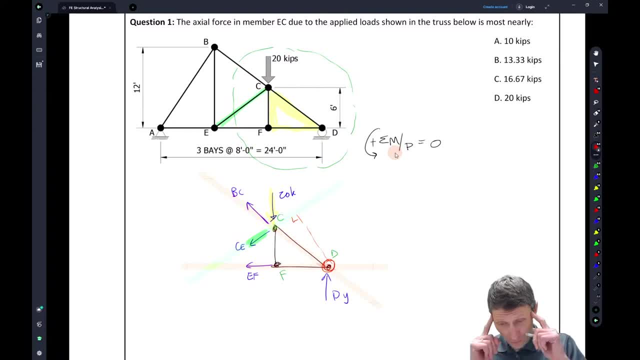 perpendicular distance. I could probably do some geometry and figure it out. But what I see here- what I see is a little bit easier- is I can just take that force and kind of bring it down to this point And now I can apply some components. so I can apply like maybe CE1, CE2, CE3,, CE4,, CE5,, CE6,. CE7,, CE8,, CE9,, CE10,, CE11,, CE12,, CE12,, CE12,, CE13,, CE14,, CE14,, CE14,, CE15,, CE15,, CE14,, CE15,, CE15, CE15,. 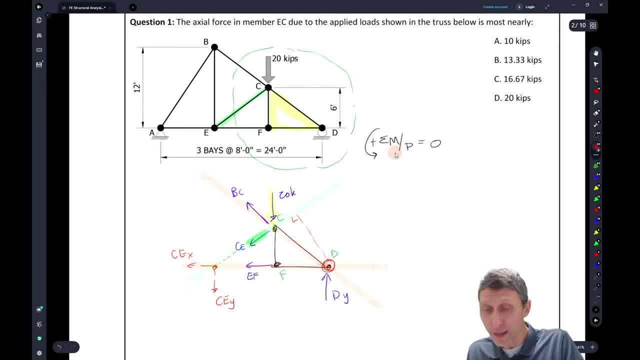 like maybe CEY and CEX. Why is that important? Because what you see is CEX passes through point D, So we're left with kind of one component here that we can solve directly. So when I saw my moments, I'm going to say: well, CEY times its moment arm, So its moment arm is going to go from. 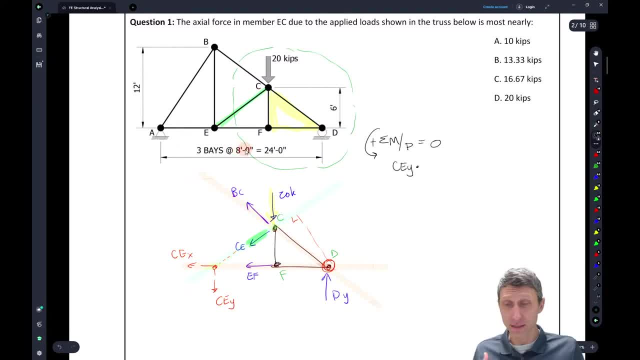 this point E to point D, And if these are eight feet on center, that's going to be a total of eight times two or 16 feet Right. In which way is that causing rotation? That's causing rotation kind of in this direction. 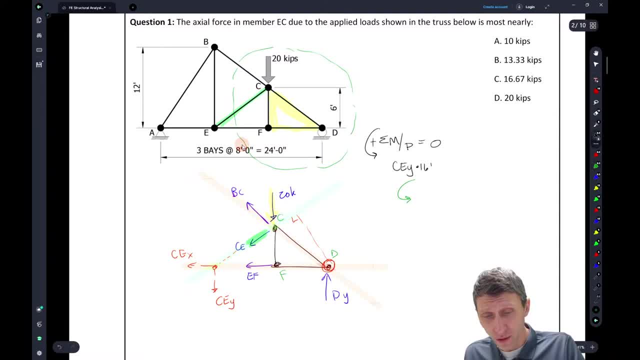 that matches our positive sign convention. This is going to be a positive value. Okay, And what else do we have? We have plus 20 kips. All right, So here's our 20 kips. That's in a positive sign direction as well, or a positive rotation as well. That's causing rotation this. 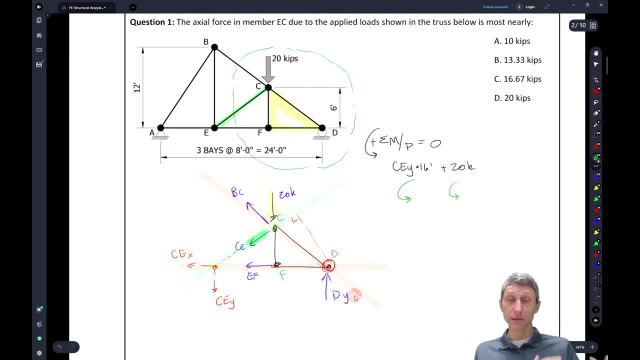 direction. And what's its moment arm? Well, it's the force times the perpendicular distance. The perpendicular distance from its line of action to point D is this horizontal distance of eight feet. So I can put that in here: This is times eight feet, And all that has to equal zero. 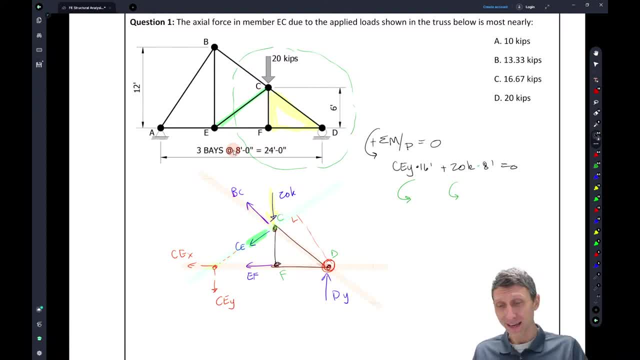 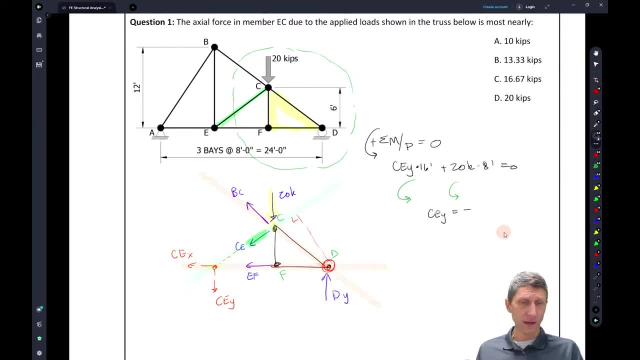 But if I put that in here it's going to be a negative value. But if I put that in the calculator, what do I get? I get 20 times eight divided by 16. And that gives me a value of negative 10 kips. 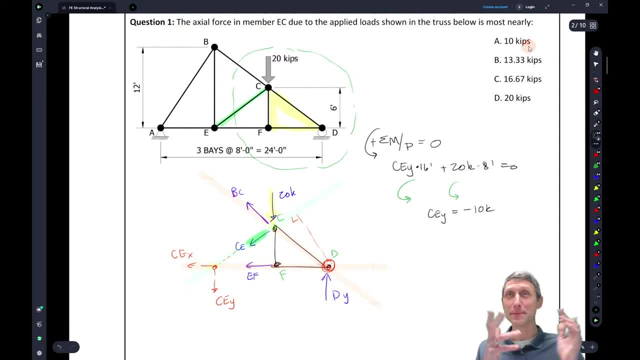 So you might be tempted to say, OK, we got 10 kips, I'm happy, I'm just going to move on. But don't do that, because that's just one component, That's the vertical component, And what we want are, or what we want really is, is this total force here. So we want this total. 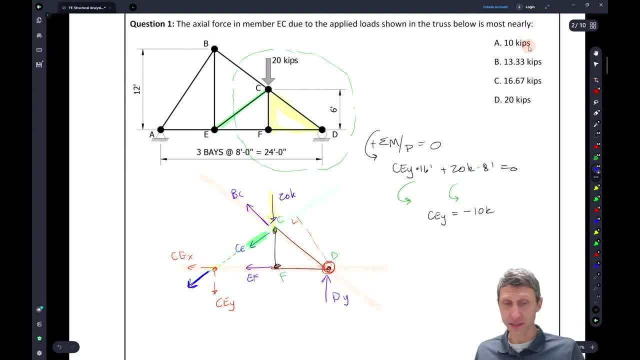 kind of resultant force here, which is CE or EC, however you want to do it. So to look at that, what we have to do next is kind of take a look at at this, this whole triangle up here. So if we take a look at this whole triangle, 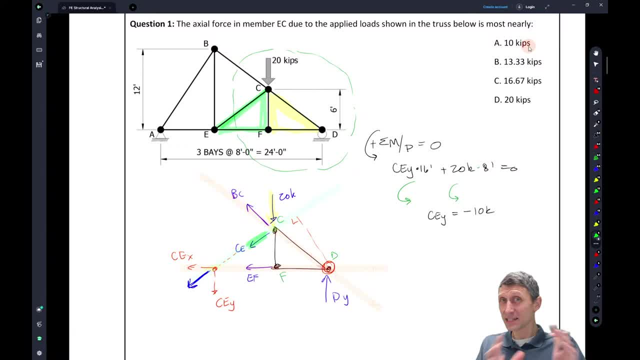 right. this whole triangle here is going to is going to help us to relate the component to the main force. So the way I like to show that is by saying: OK, we know, we have this triangle here. Right in this triangle between E, F and C, we have some dimensions, The dimensions we have. 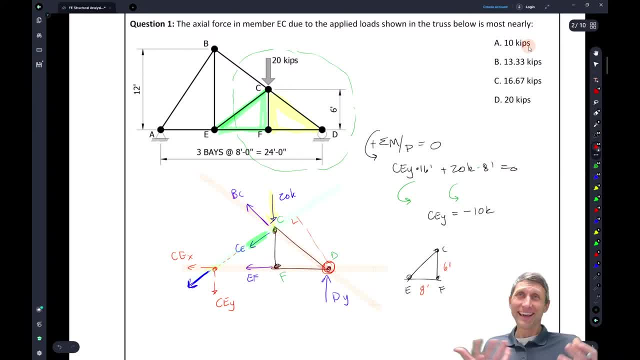 you know this is eight feet, We know this is six feet And I'm a sucker for six, eight and ten triangles, so you'll have to forgive me for that. But this is a six, eight, ten triangle, OK, And what that means is that's going to mimic or match our force triangle. So if we have this, 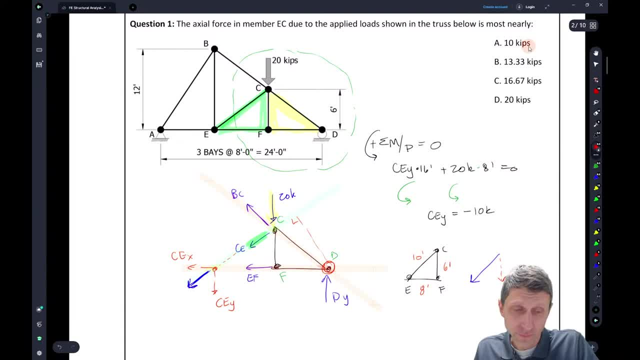 force here and we have some components, Right, And maybe I'll go back to saying this is easy, just to just to be more consistent with what the problem says up here. Easy, So easy. Why easy X and force altogether, Easy, Right? That's what we're trying to find here, Right? So we're trying. 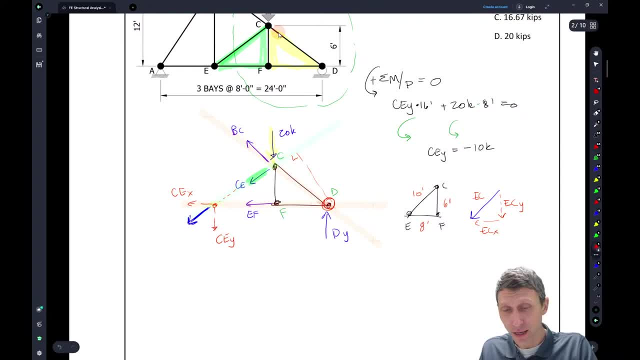 to find that easy. And now this is just a similar triangle thing, because I know that this angle and this angle are exactly the same. So if we have similar triangles, what we could do is we could write: well, I know what do I know, I know easy Right, And I know easy Why. So if I know those, 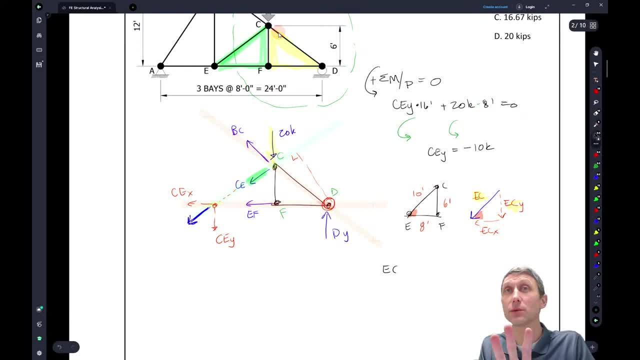 I can say: well, easy, I don't know. Easy, I'm sorry, Easy is the one I'm trying to find. easy over easy. Why Has to equal what it has to equal essentially ten over over six, Right? So when we 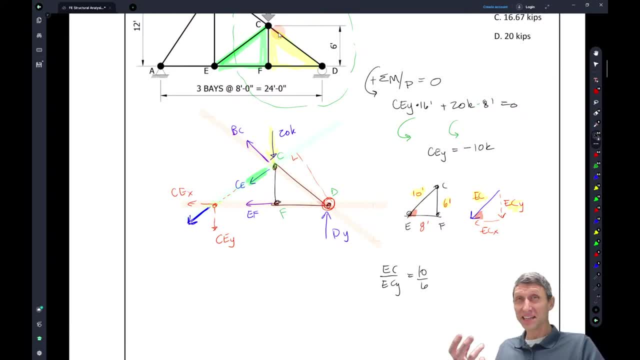 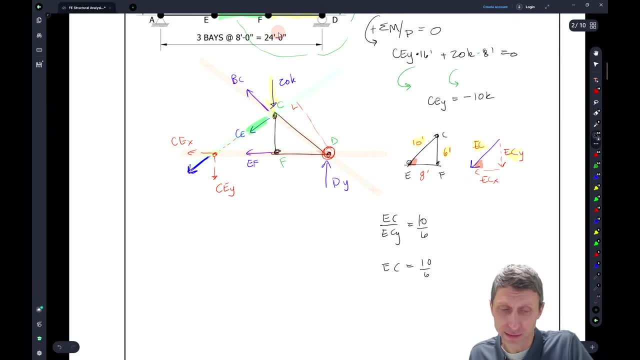 have this here. what we can see is all to get easy. all we really have to do is cross, multiply and we get easy equal to ten, over six times easy. Why? And when I did this out earlier, I think I got like sixteen point six, seven, Right, So sixteen point six, seven. 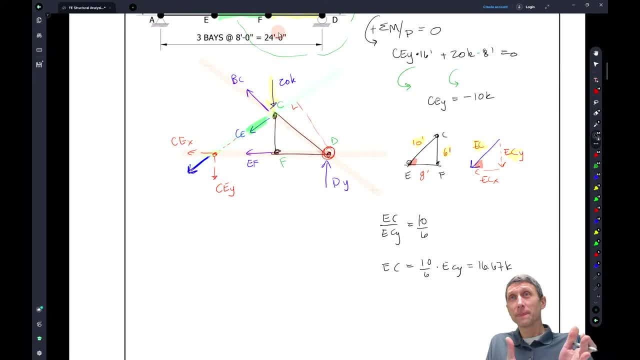 OK. So the cool thing with this problem is we didn't even have to do that reaction, I mean got level. First thing I do a lot of times when I see trusses like this is: I'm going to, well, I'm going to go solve for D, Y, But on the, every minute that you can save is going to help you. 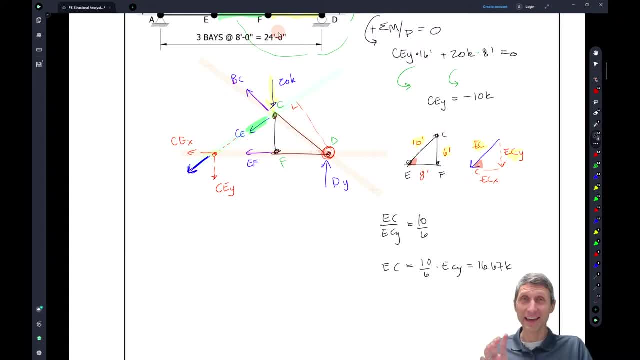 get to another problem where maybe you can't save it. OK, It's a little bit more difficult. So if you can save not doing those reactions, you know it saves you. It saves you a few seconds there and that's going to help you. But this should be. 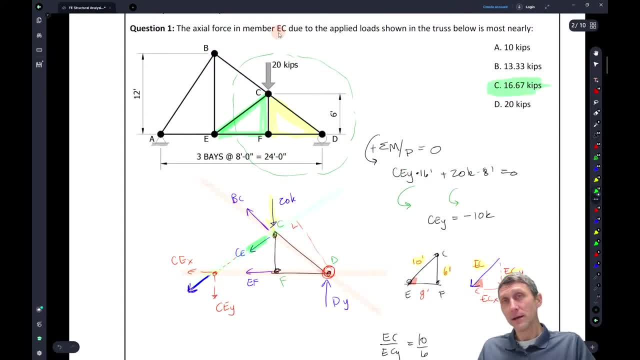 Our answer, which fortunately is up here in our answers as well. So hope that one makes sense. I mean, it's just taking another look at trusses, trying to introduce method of sections a number of times here, method of joints, But hopefully this makes a little bit of sense. It also hopefully it. 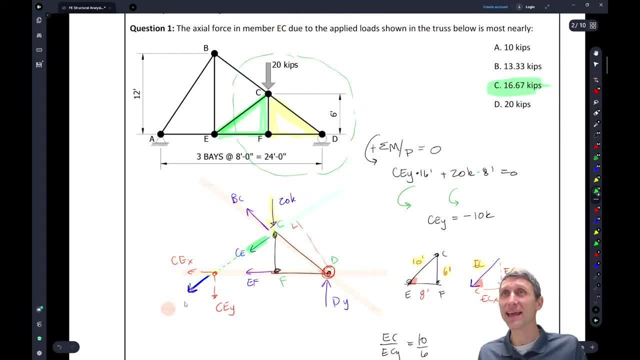 makes sense that we can apply, or we can apply this moment anywhere. I'm sorry, we can apply this force anywhere along its line of action and it's going to equal the same moment. And just again, I don't want to. I'm trying not to get too. I'm trying not to get too. I'm trying not to get too. I'm trying. to get too. I'm trying not to get too. I'm trying not to get too. I'm trying not to get too. I'm trying to get too. I'm trying not to get too. I'm trying to get too. I'm trying to get too. 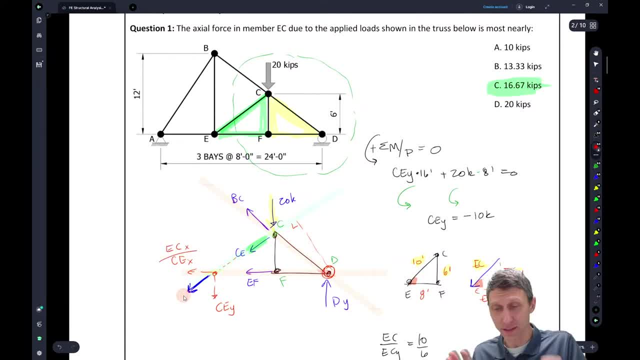 People. this can be easy X or CX. the same same thing, right, It's not divided by. these are the same things. I'm not trying to mess with people with different notations here. I probably should have kept this at easy X and easy y, So hopefully that's not confusing, But I don't know. 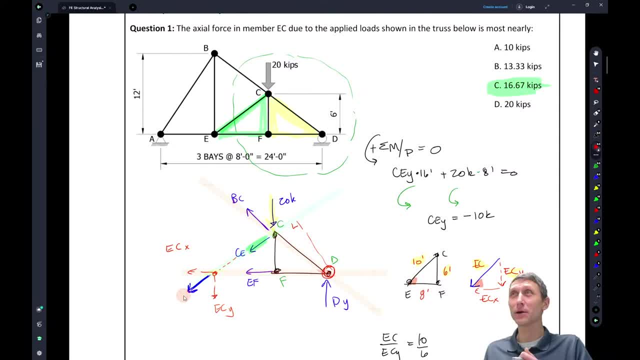 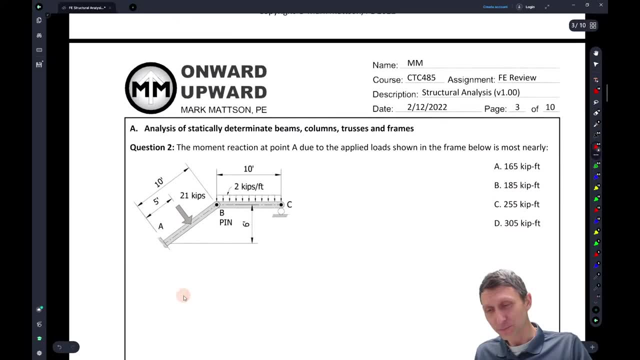 if you have questions, definitely put them in the chat or we can keep going here. but we'll just keep moving. So this is good. So let's go to question number two, Speaker 2. Again, we're in this analysis of statically determinate beams, columns, trusses and frames. 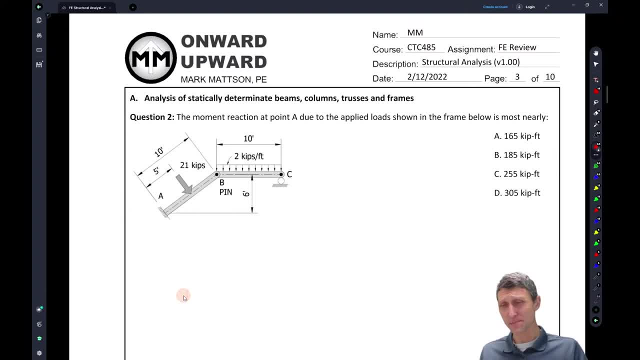 So this is. you know, we just did a truss. Now we're into this kind of beam frame type thing where we get the impact of two members connected by a pin and we have to look at what's one member going to do to the other. 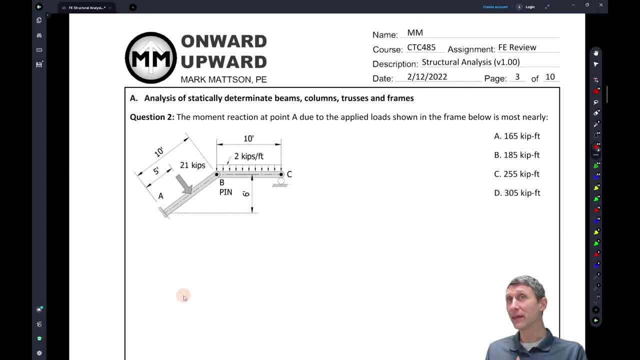 member. So one member is going to have an impact on the other member right. So this, this- you know this top member here is going to have an impact on, you know this member here. So these are connected by a pin in the middle. 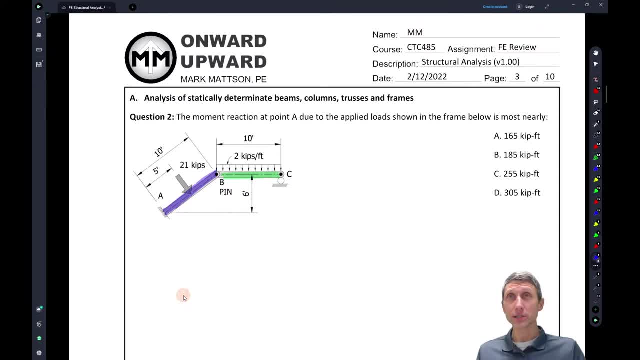 And what that means is, in order to solve this question. this question asks for a moment reaction at point A, right. So down here, down here, point A: the moment reaction at point A due to the applied loads is most nearly So. what is it? 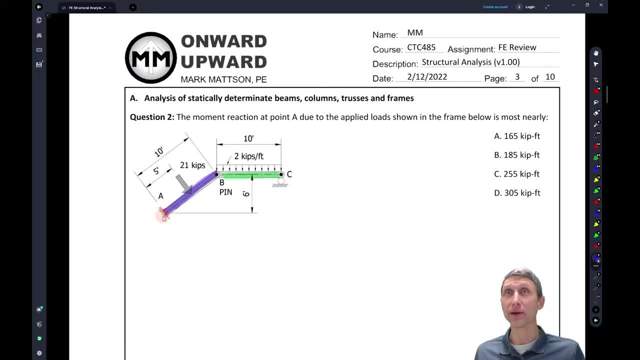 How do we get it? Well, what we're going to do here is: first, we're going to separate this thing out And we realize: well, maybe we can take a look at this first, but there's too many unknowns, There's too many things that we don't know. 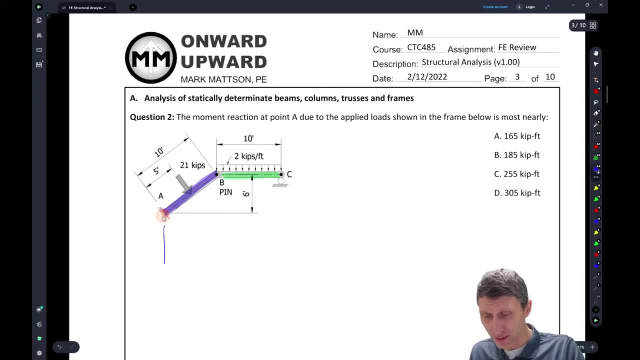 Like if we, if we were just to just draw a free body diagram of this thing, you know we'd have a y and a, x and c, y, and you can't forget this one, right, This is at a fixed support. You have the moment of day. 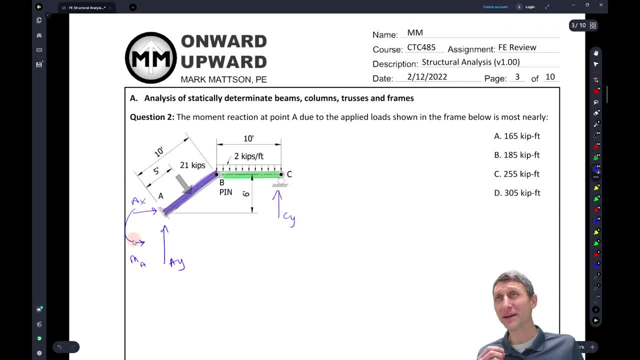 If we were just to some moments at this point, we'd have too many unknowns. We'd have the moment of day and we'd have to see why. So we can't just do that directly. And whenever you get problems like this, that are 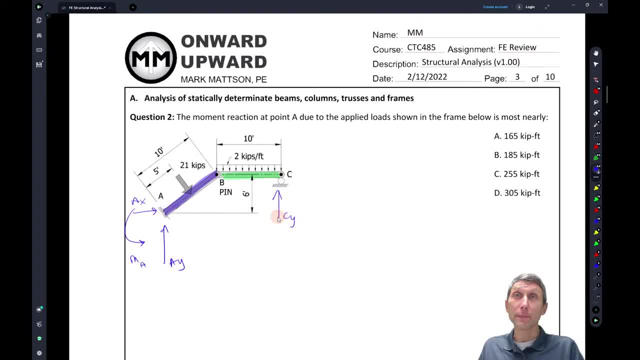 You know separate or that have multiple members joined by a pin. that's where we have to separate them out. So we're going to do here is we're just going to start with member BC, So I'm going to just draw in member BC here. 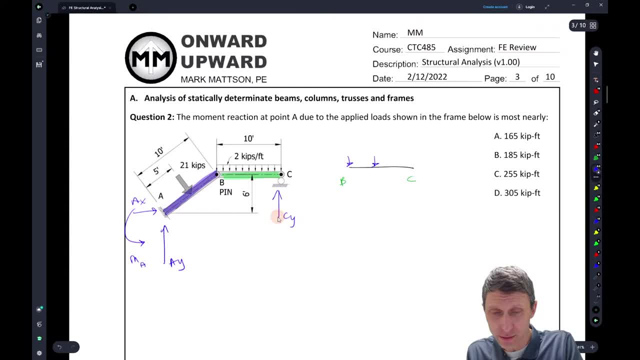 And when I draw member BC right, I've got this load That's two kips per foot and hopefully a uniformly loaded, simply supported beam is something you've seen before, Right? So this is one of those. One of those ones. 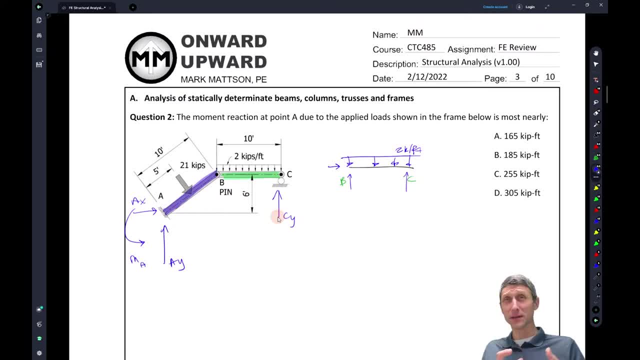 That, honestly, when I was in consulting and we'd interview people, I would ask somebody, some, some people, this question: What's the maximum moment, What's the maximum shear in this type of a beam, of the uniformly loaded, simply supported beam? It's one of those things you know, it's just W all over two. 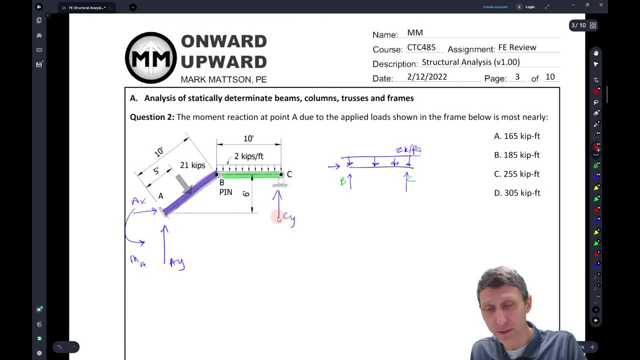 It's really easy if you, if, even if you don't know that, if you know the symmetry here, Right, And this is ten feet Two times ten is 20 kips, Right, So we get the total kind of resultant force here of 20 kips. 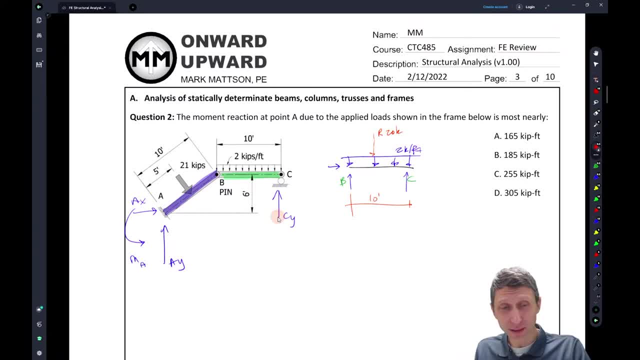 If you know that- Hopefully you don't have to do a lot of work here to get that- CY and BY are both going to equal 10 kips. Right, That's the. you know. BY equals, CY equals what WL over two. 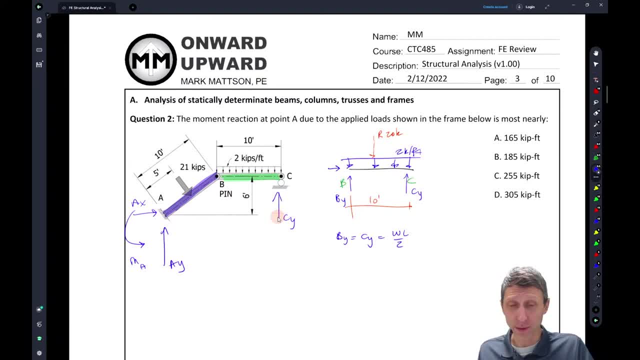 We'll take a look at that a little bit later. to the beam diagram. if you don't remember what it is, I mean again, if you don't remember what it is, that's OK. You could also find it by just summing moments about point B, equal to zero. 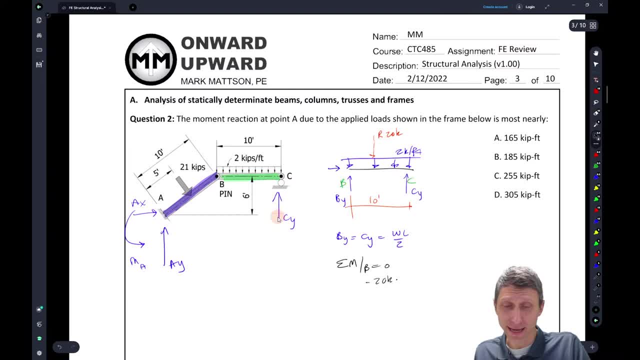 Right. If we did that, we'd get you know minus 20 kips times Right, The five feet. So what's where's the five feet come from? That's this five feet Right. So that's the moment arm. 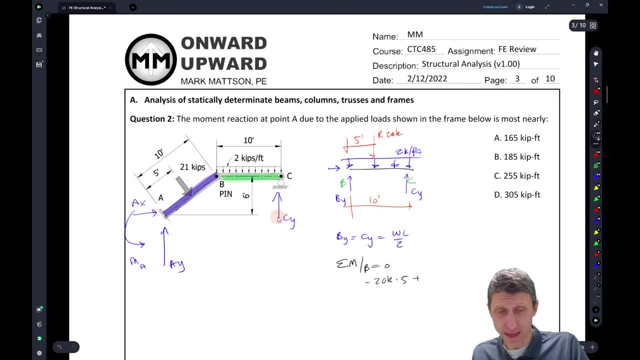 And then we're going to what we're going to add CY times 10 feet. So either way, when we, when we're all said and done, we should get a value of CY equals or 20.. Divided by two is going to equal 10 kips. 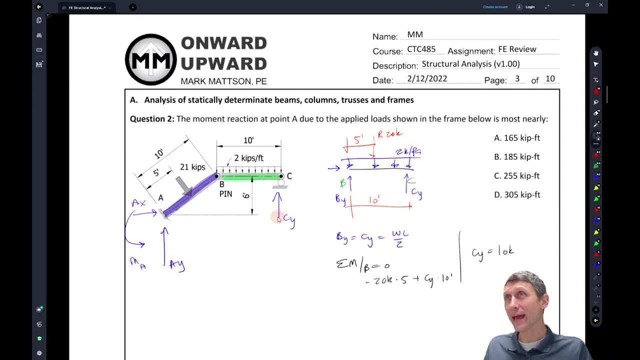 So that's kind of the starting point, And once we have that, What we have to do is we have to take a look at these pin reactions right, This BX and BY, So I sort of left those over here for a second. 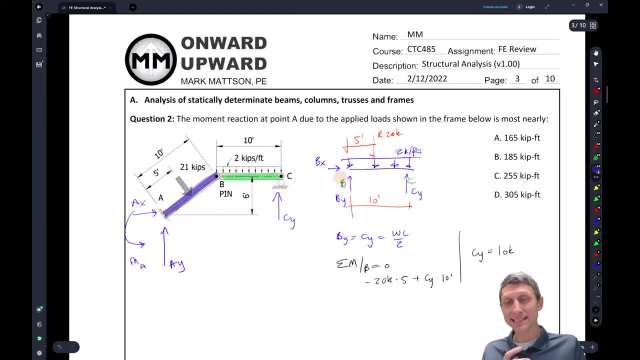 So we have BY and we have BX. So when I separate this, this piece at the pin, what I'm doing is I'm kind of exposing these forces. You'll notice I didn't show the forces here to start because I didn't separate that piece. 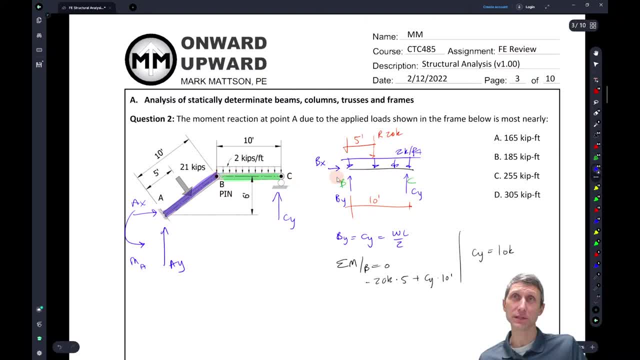 apart. But as soon as I separate it out, that's when I have to show these forces, That's when they kind of show up. right, The forces balance if the pin is connected. Once the pins not connected, they no longer balance. 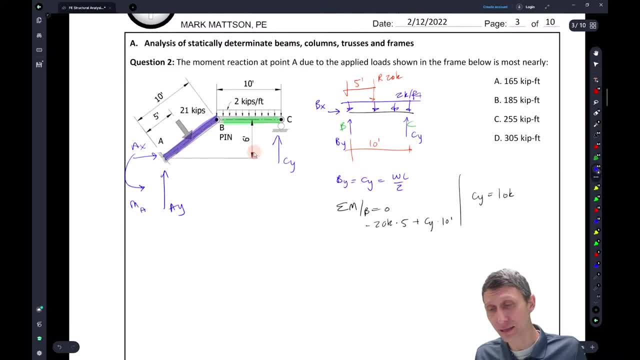 And that's where we have to add them in. So what I'm going to do next is I'm going to take a free body diagram of this other member here, of a member, AB. So if I take a look at AB, this is where I still have, you know, I still have my 21 kips. 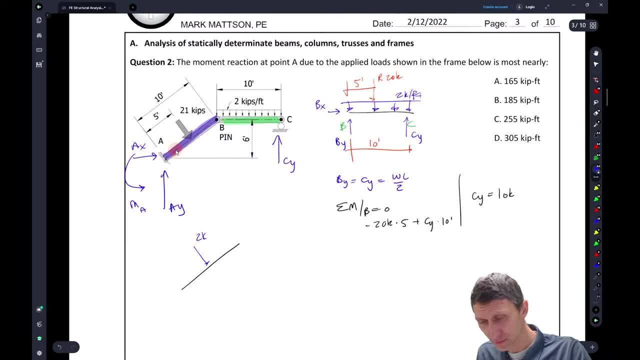 right, My 21 kips acting here, I'll get a one in there, And this is at five feet from the support. Okay, so I got my 21 kips, but the question is: what other? what else do we have going? 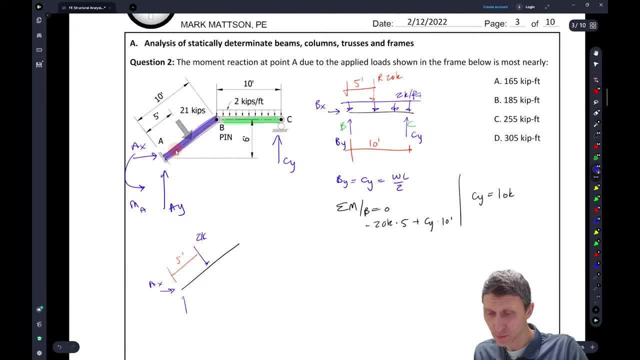 on here. We still know we have AX, We still know we have AY, We still know we have the moment at A, And this is where equal and opposite sides of the pin will have equal and opposite reactions, right. So we have to deal with those forces, the BX and BY forces that are in that pin, right? 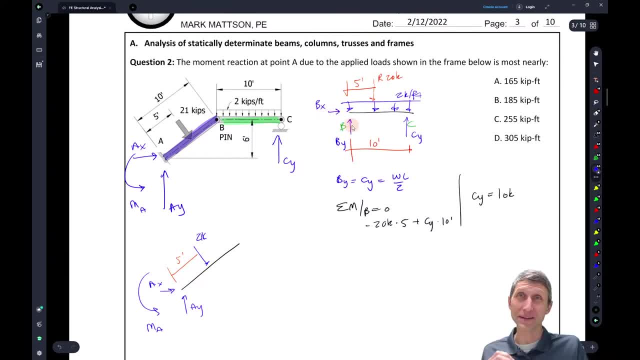 But when we show them, You know, up into the left or, I'm sorry, up, and that's the right- up into the right here, right up into the right here, on the other side of the pin, we have to show them down. 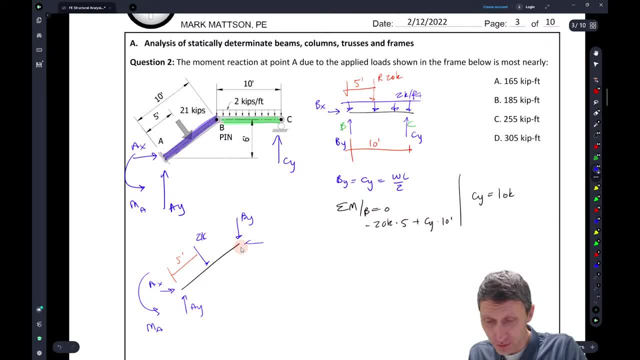 So what's this? BY, and you know, to the left, BX. So on opposite sides of pins, the forces are equal and opposite. So don't forget that We never solved this. but we could come back up here and we could say: well, if we sum, 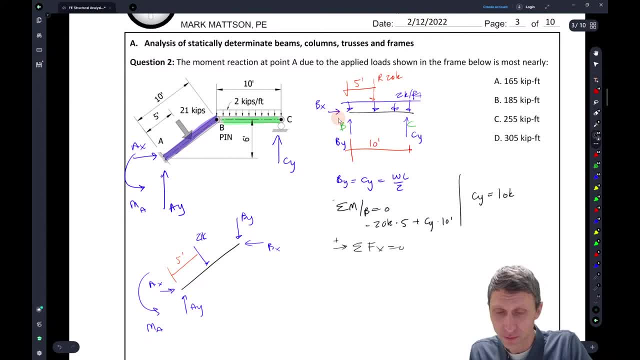 forces in the X direction equal to zero Right. My sign convention in there just for for completeness. But what we have here is we're just going to get BX equals zero right. So if, if, if C is a roller, BX has to be zero. 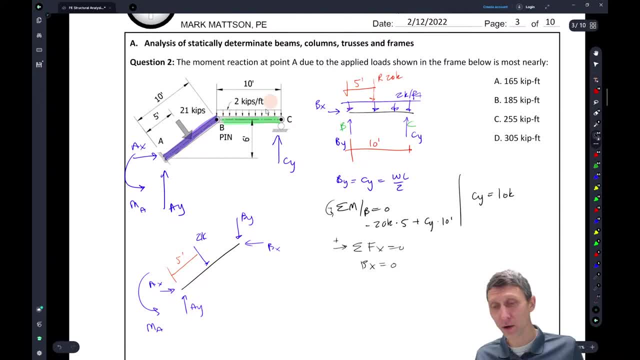 So that's just going to be zero as well. So what we know here is: I'm just going to take this and I'll leave it in there for now. I'll just call it. I'll call it zero, Right? So this equals zero, and BY equals, what do we get? 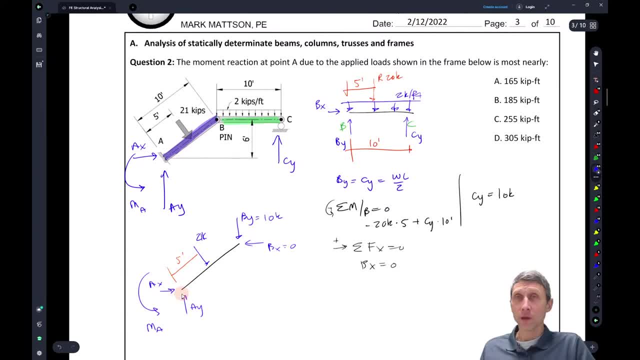 We got BY to equal to 10 kips. So now this is just a sum of moments, equation Right, And that's what we're trying to do. We're trying to find the moment reaction at point A. So now what I can do here is I can. 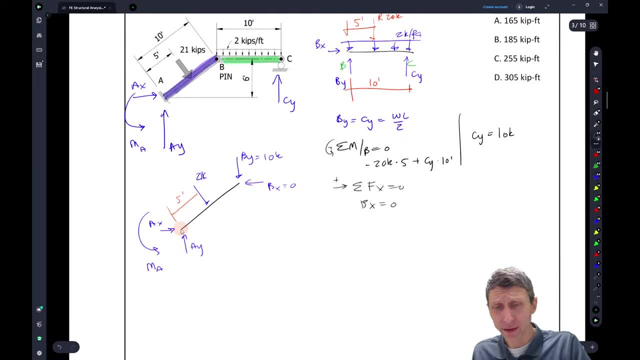 some moments at point A, And if I do that, I'm just going to sum my moments at point A. make that equal to zero. And what do I get? I get: you have to remember your mother, You have to remember Ma right. 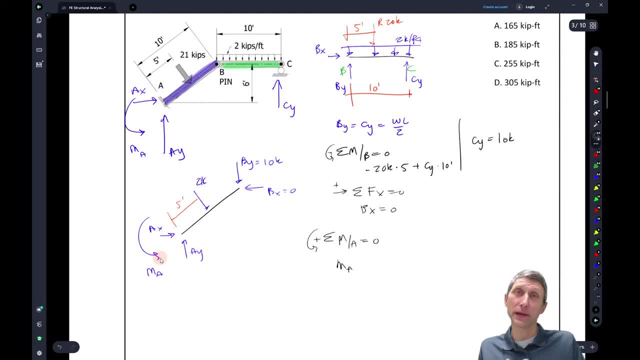 Your mother, your mother, your mother. The moment of day is a moment of day. You got to remember that one. It's there, Don't forget about it And, honestly, when you're done with this, go give your mom a ring and just say: hey. 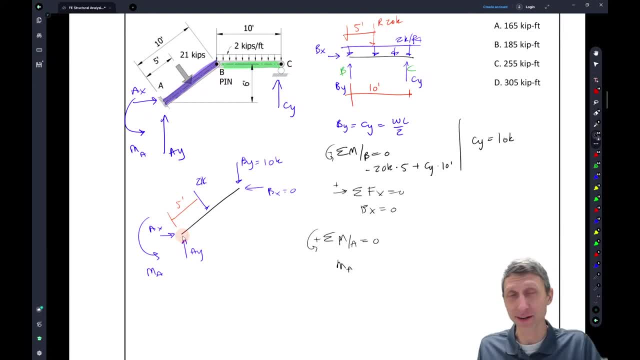 Mom. thanks, I love you. I'm so glad you believe the best in me. Sorry, that was just an aside That has nothing to do with the FE, but it's just a piece of advice, you know. So, as we go through there, what we're going to do is we're going to sum moments at point. 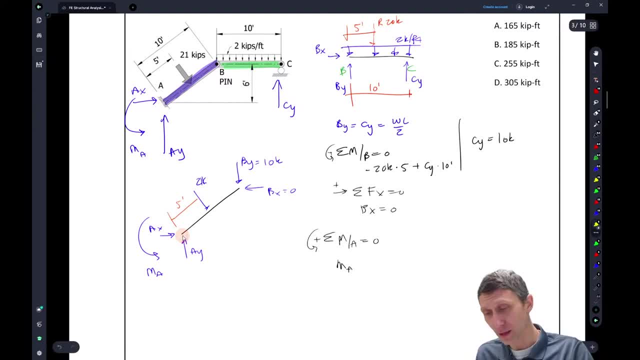 A. Well, forces don't pass through point A. Again, we have some couple of forces here, We have the 21 kips and we have BY. And a moment is what? A moment is equal to a force Right? A moment is equal to a force times a perpendicular distance. 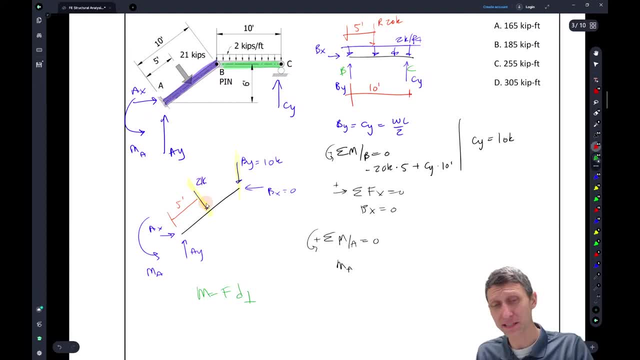 So the cool thing here is the 21 kips. I probably could have put this in the problem statement. I probably should have said that this is perpendicular, But I'll tell you now that force is perpendicular to member AB. And if that's perpendicular, the cool thing is we already have this moment arm. 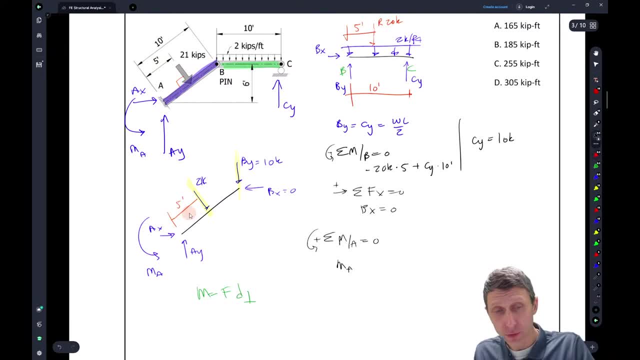 We already have the perpendicular distance, So the moment of day is going to be 21 kips times. I'm sorry, the moment of day is going to be: we're going to subtract off 21 kips times that Right, 21 kips times this 5 feet. 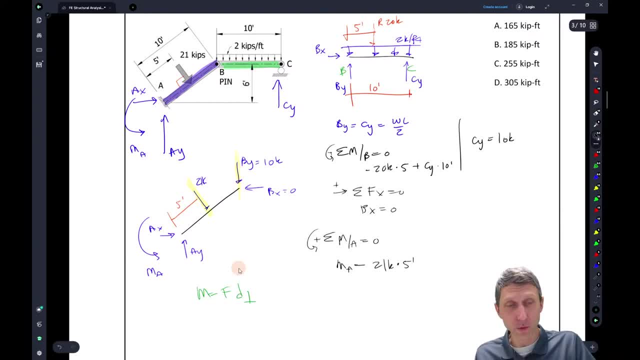 And then the only other force here is this BY, and we have to figure out its moment arm. So what I'm going to do is, if I kind of extend the line here, its line of action is going to have a moment arm, a perpendicular moment arm, from point A to its line of action of. 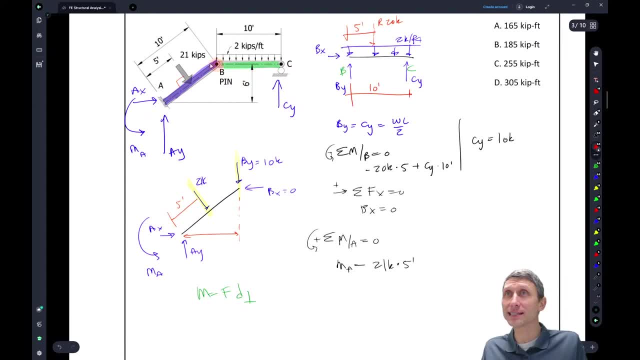 well, shoot, we don't even have this, Right. We know 6 and 10.. And there's my favorite one again Right, That favorite triangle of mine, where we have a 6,, 8,, 10,, 11,, 12,, 13,, 14,, 15,, 16,, 17,, 18,, 19,. 20,, 20,, 21,, 22,, 23,, 25,, 26,, 27,, 28,, 28,, 29,, 30,, 31,, 32,, 35,, 34,, 35,, 36,, 34,, 37,, 38,, 39,, 40,, 42,. 49,, 42,, 41,, 41,, 42,, 42,, 43,, 45,, 46,, 47,, 48,, 49,, 45,, 45,, 46,, 49,, 49,, 50,, 51,, 52,, 1,, 2,, 0,. 6,, 8,, 9,, 1,, 2,, 8.. Three: 4,, 5,, 6,, 8,, 10.. So three, four: 5,, 6,, 8,, 10.. 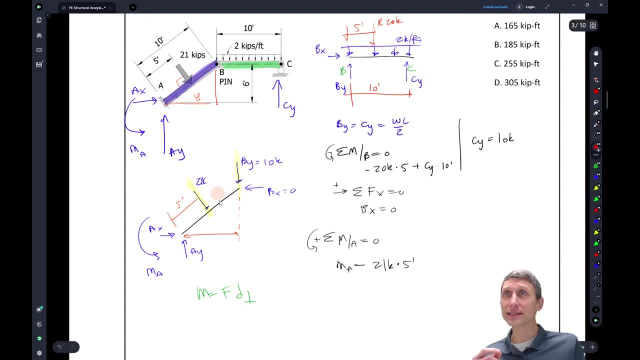 I'd have to think to go even higher, but it's. it's some of these Pythagorean theorem type triangles If you have. you know the hypotenuse in one side, you should be able to find the other. Okay, 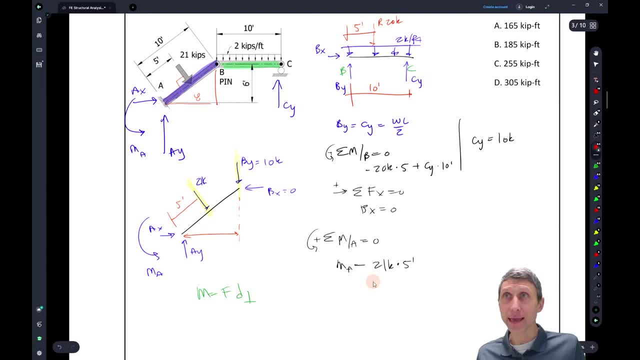 So a squared plus b squared equals c squared, type of things. Okay, and then we also know that this distance here is that eight feet. so what that? what does that mean? we're gonna subtract off as well by times eight feet, that's gonna equal zero. so the good news is we, we basically have one equation, one. 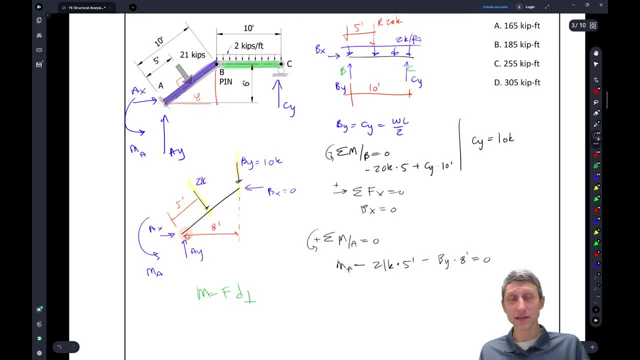 unknown and if we're summing moments about point a, that those the only two things that cause a moment about point a. so we get the moment a day equal to what 21 times 5, you know, plus B Y, which is 10 times 8. so if I do that on my 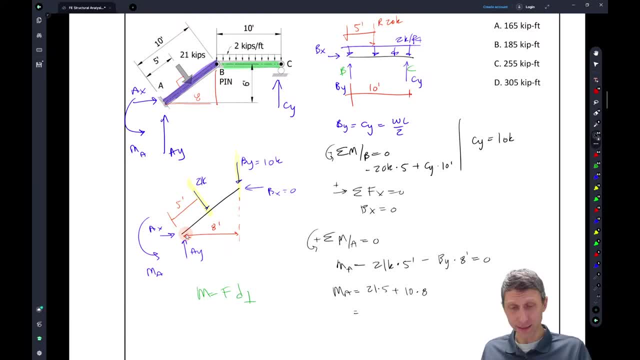 calculator. hopefully we get an answer, but I think we do. so we get 21 times 5, I think that's 105. yeah, so 105 kip feet plus 80, not kip feet, so that's gonna equal a 185 a kip Beat. okay, and that's our answer. right, so that's the answer. 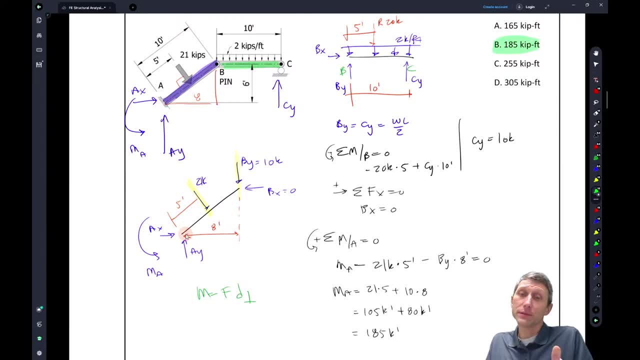 that's our answer, right, so that's the answer that we're looking for here. But with frames, what you're gonna have to do is you're gonna need to separate them, probably at that internal pin. So that internal pin is something you have to deal with. 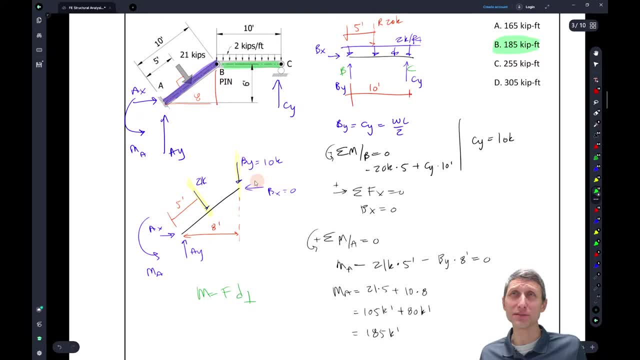 And then what you're gonna have to deal with is you're gonna have to deal with the reactions on each side of it. So on each side of a pin they're gonna be equal and opposite. So when you put that pin back together, 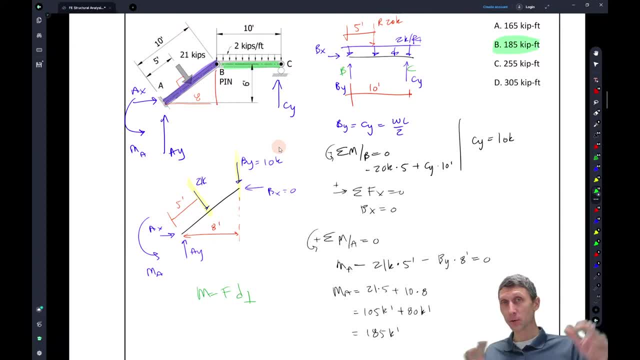 those forces cancel out. When you pull them apart, you see them, okay. So take a look at that. You know that's one of the things that you're gonna have to deal with, all right, Okay, well, let's keep going. 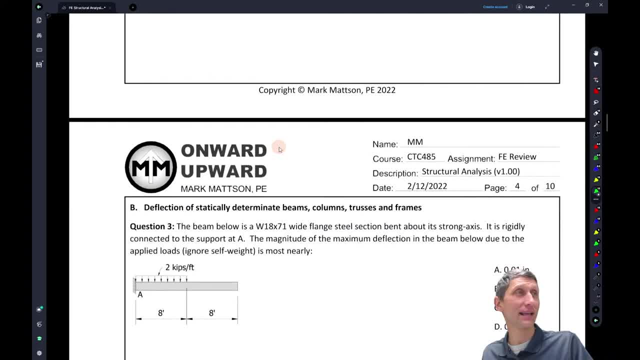 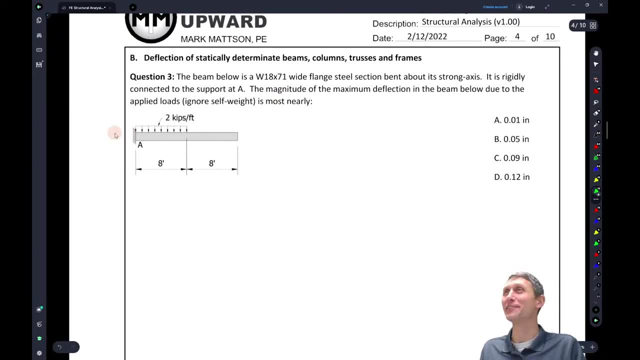 So we've got two questions down. I mean, honestly, today's session probably won't be as long as some of the last couple, So hopefully we'll get to that a little earlier, who knows. But let's look at this. Deflection of statically determinate beams. 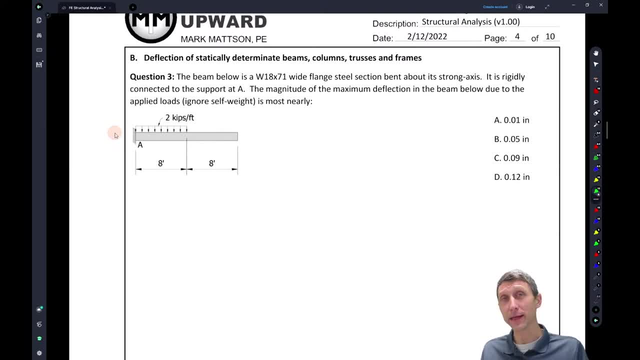 columns, trusses and frames. So now we're to deflection. In the deflection there's a couple different methods. I mean, some of you probably learned how to integrate and integrate, and integrate and integrate until you finally get a deflection formula. 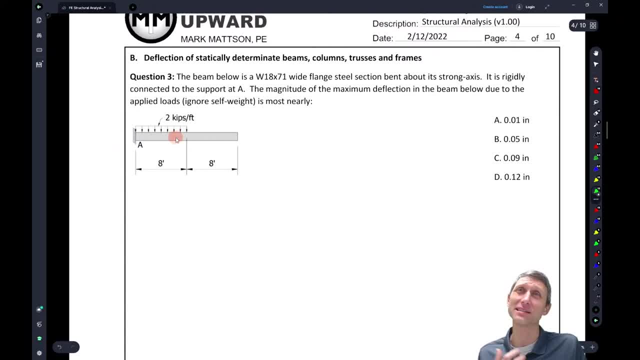 and you can do that. And when you get questions like this that are piecewise, they get annoying honestly. They just get long and annoying And there's an easier way, okay, So the easier way is to come in to your reference handbook here. 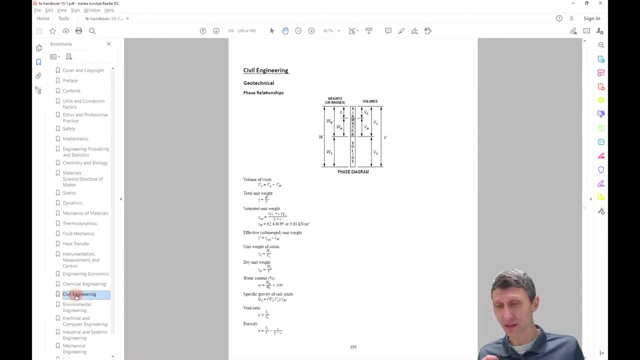 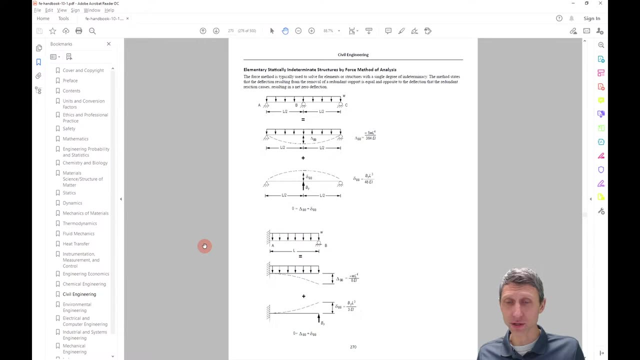 And in the reference handbook if we go down to civil engineering there should be a structural section right. So we go past geotechnical and eventually we get to the structure section. So this is kind of helpful, except that I think. 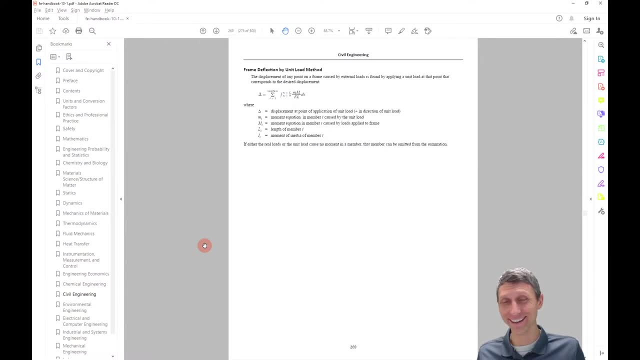 it's a little bit more complicated. So we're gonna go down to the structural section, right? So we go past geotechnical and eventually we get to the structure section. So this is kinda helpful, except that I think I'm looking in the wrong section. 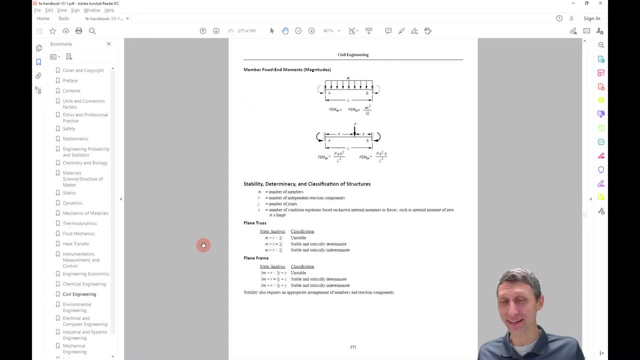 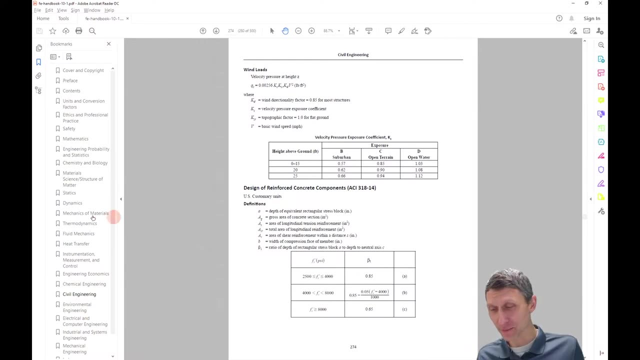 and it's less helpful there. So we have a couple things. We have a static indeterminate. you know, we've fixed end moments. we have structural design and we think, uh-oh, we missed it, Where are those beam tables? 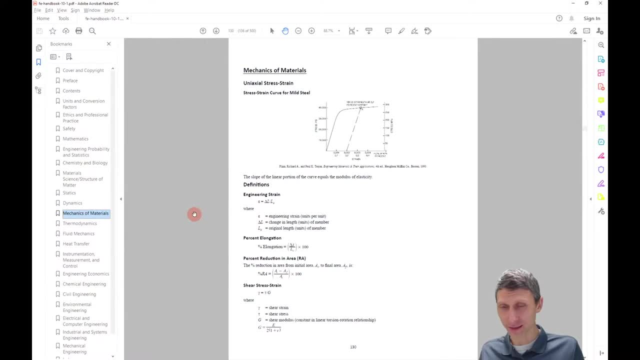 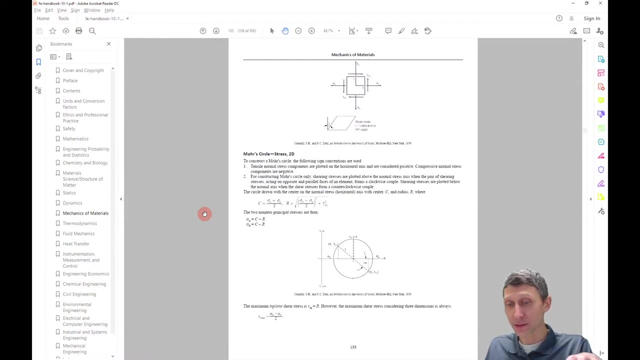 Those beam tables are actually in mechanics and materials, I think. So I think I got that wrong. but let's go back here and look And, honestly, there are gonna be some pieces in structural analysis that go back in mechanics and materials. So, like I talked about earlier, 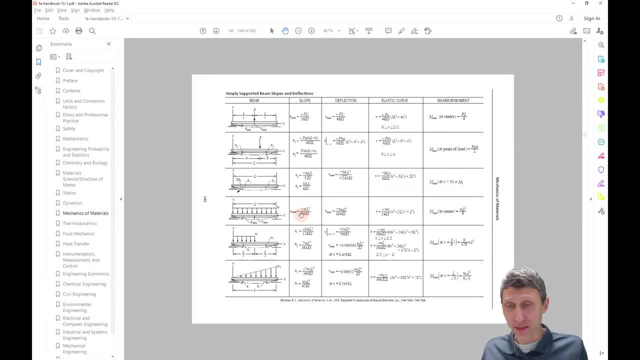 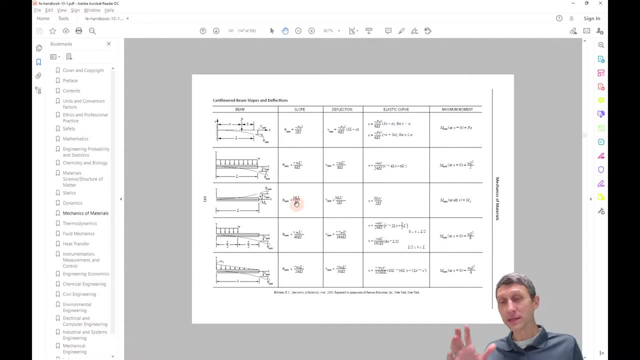 like the column formulas. the columns show up in: oh, that's what we're looking for. We'll come back to that. but well, we'll come back to it, Let's just do it now. So what we see here is: we have some beam diagrams, right? 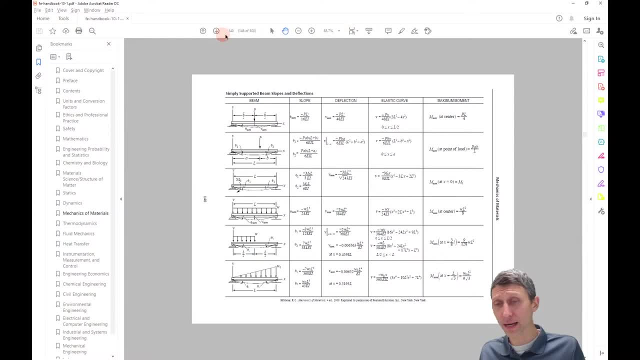 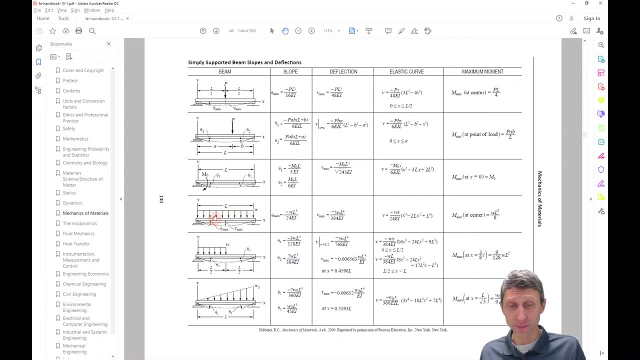 And these beam diagrams are gonna be what we're gonna use, And I just picked one of them. I mean, it could show up like any of them. This is one of those super common ones. It simply supported uniformly-loaded beam. I have WL to the fourth over 3D, 4EI. 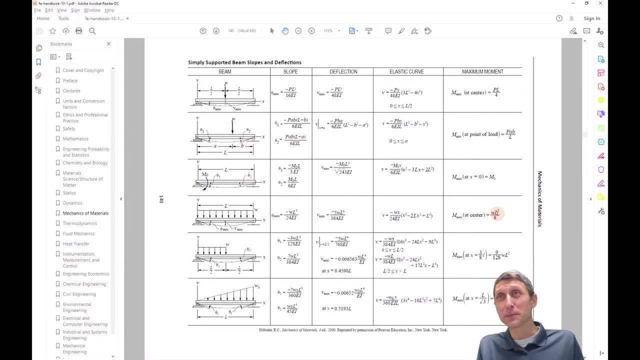 the maximum moments WL squared over eight. That's not the one we're using, but I pointed it out just because it's a super. it's a super, super, common one, And you might be tempted to look at this and say: 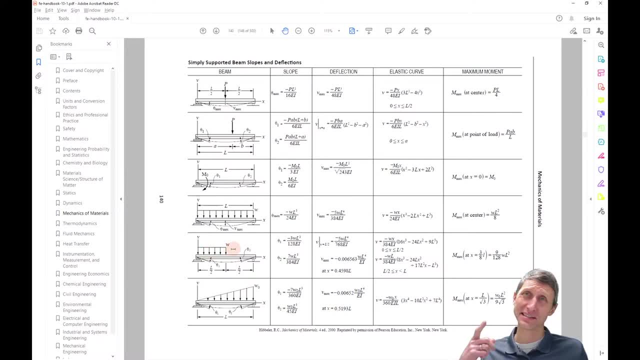 oh, that's the same loading we have and it's half the span, but don't use it because it has a pin on one side and a roller on the other, right. So what we're doing is we're gonna come down here. 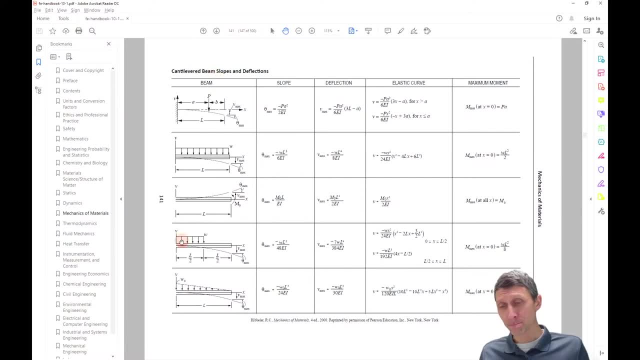 and we're gonna look at where we have a cantilever beam and we have this maximum deflection at its end. So that's what the question asked for, right? So if we come back to the question, we see we have steel flange section. 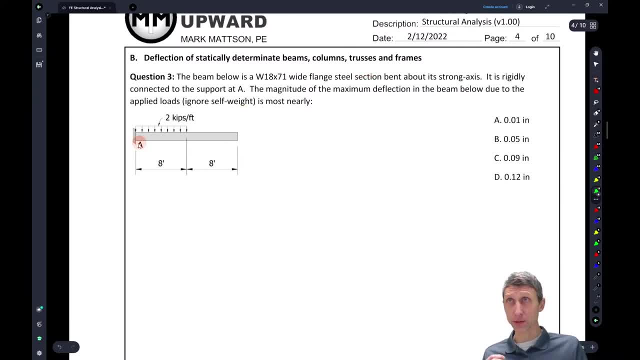 metamount. at strong axis It's rigidly connected at support A. So rigid connection means it's resisting rotation. This is a cantilever And the magnitude of the maximum deflection. So if this thing is going to deflect, it's gonna deflect, kind of like this. 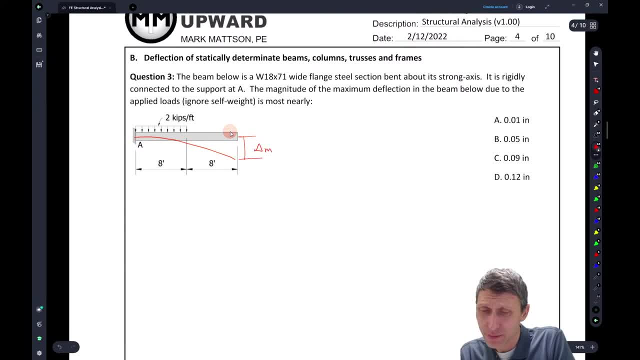 And we're looking for this kind of. I like to use delta and this is gonna be like our maximum deflection. The reference handbook uses that V or nu, but I just like to use this. So what does that mean? So let's come back here and see what we have. 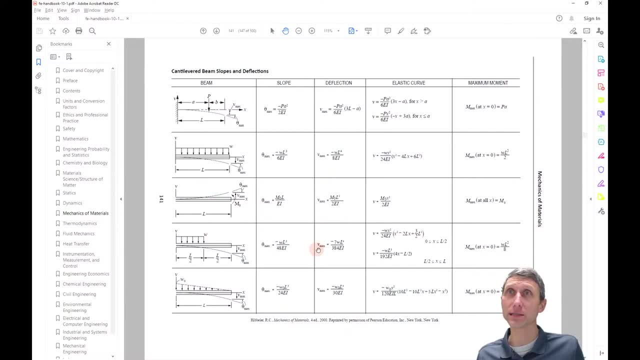 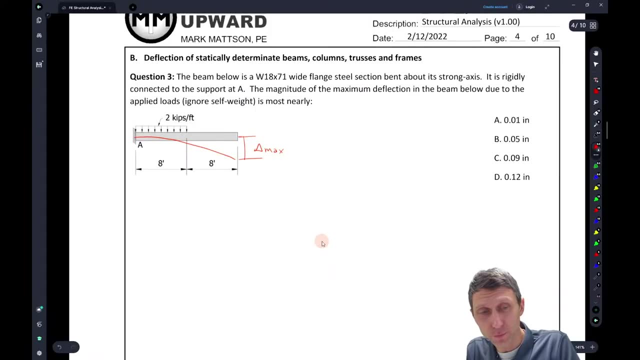 So we got this formula here. We got a maximum deflection and we're gonna get seven WL to the fourth over 384 EI. So let's just write that out. And so the formula that we're solving here is seven. So our delta max or our nu max, 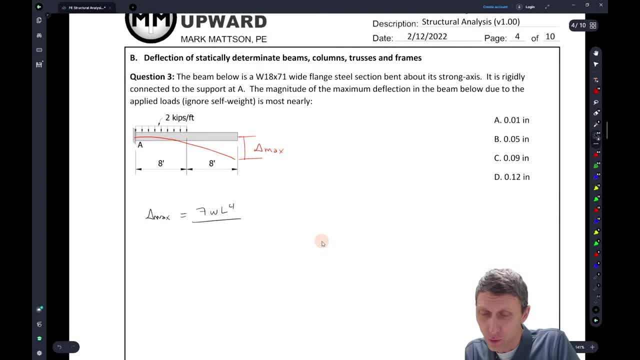 is gonna equal seven WL to the fourth over 384 EI. And I dropped the negative sign cause I don't really care so much that this is going down. I mean, I know the load's pushing it down, but yeah, You could keep the negative if you want. 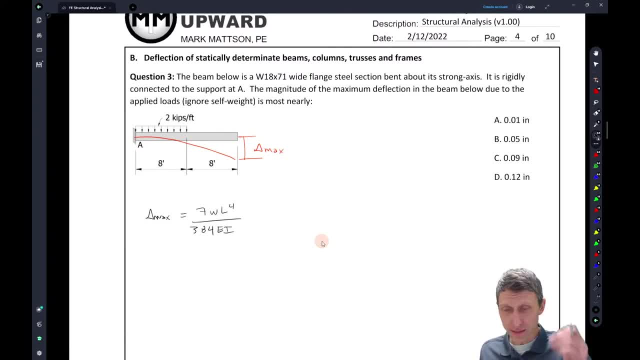 So let's go with it. So let's go here, Okay. so I just saw a comment, So I'm gonna hit that comment real quick. How come the first two questions aren't just considered statics? They kind of are. They kind of are statics, okay. 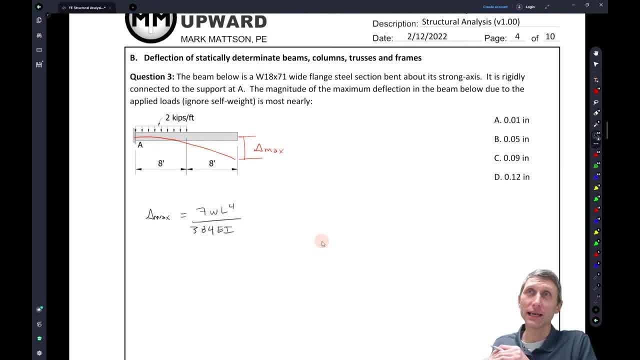 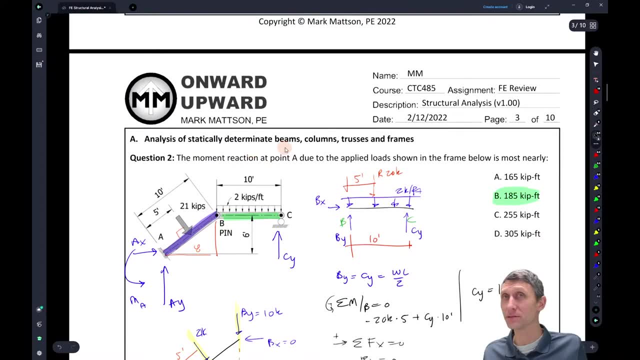 And just not to burst your bubble, but they kind of are statics. But when we're looking at- okay, I'm just gonna come back here for one second- When we're looking at analysis of statically determinant structures, typically we're just looking at statics. 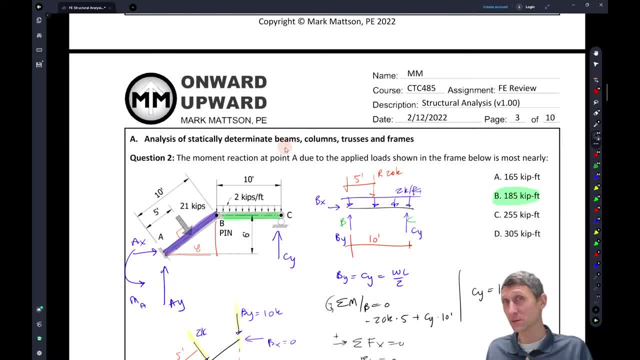 It's just maybe a little bit more complicated than it was in your 200 level statics And now this is 300 level and it's a little bit more complicated. It's sort of like pre-algebra and algebra: You're doing the same things. 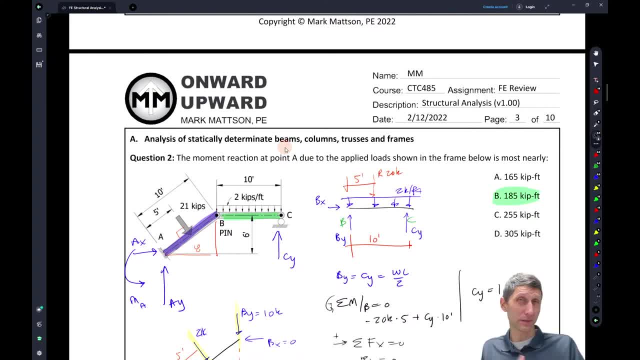 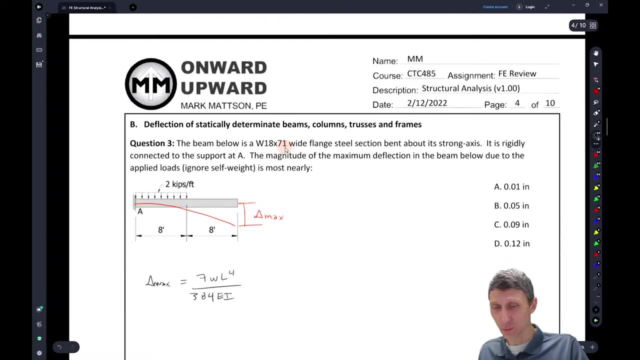 or pre-calculus and calculus. You're kind of doing a lot of the same things, but sometimes it's a little bit harder in calculus versus pre-calculus, Statics versus structural analysis. Okay, that's kind of the way I'll throw it there. 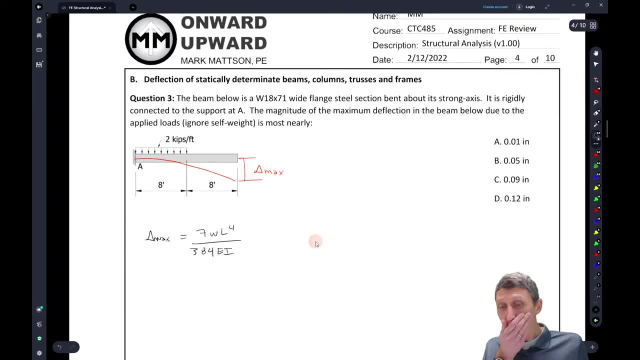 So sorry for seeing that comment late, but let's keep going here. So let's see, Let's define our variables right. So our variables here: we have our W and that's gonna be our uniform load. That's just gonna be two kips per foot. 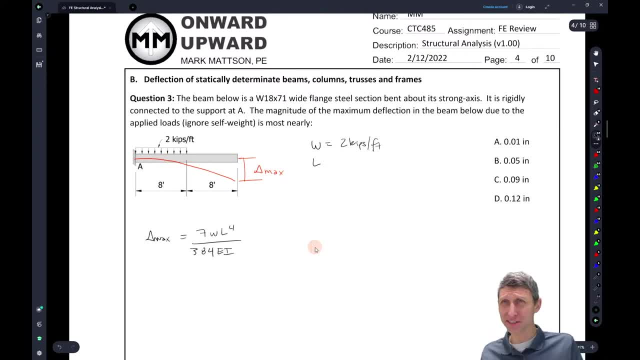 Okay, good, L. well, is L at eight feet or is it 16 feet? Let's go back and take a look and see what that is. So if we come back and we look at our reference handbook here, what do we get? 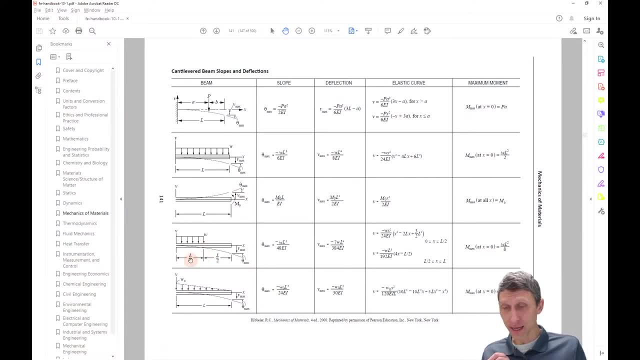 We get L. If we look at L, we see L over two is gonna be half the span and L is gonna be the whole span. So let's come back here and look at L is gonna equal the whole span: 16 feet. 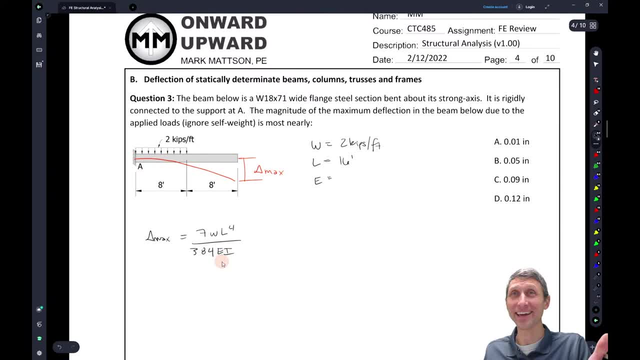 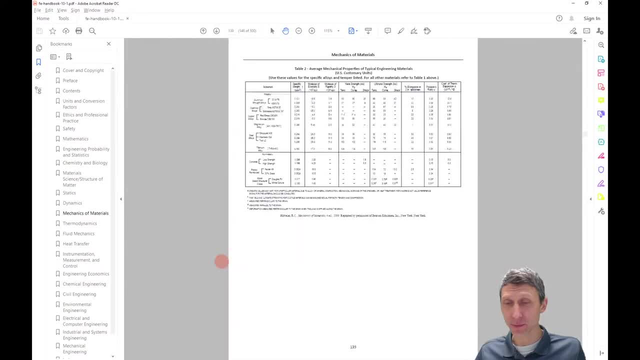 E. do you know what E is off the top of your head For a steel beam? hopefully you've memorized E. If not, there is that table. I think we just passed over it. right. We looked at this, maybe in the mechanics and materials section. 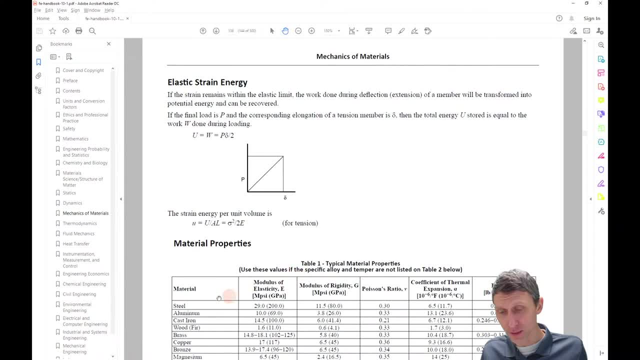 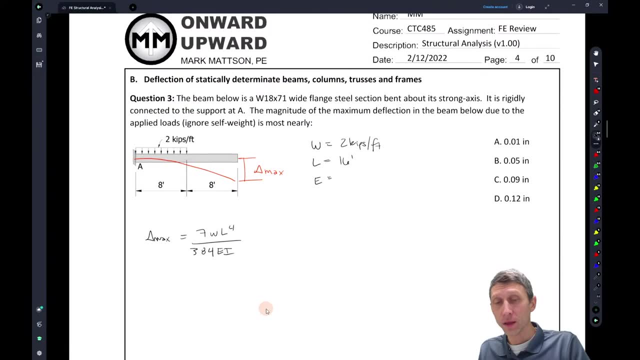 but what do we get right? So for E, if we come down for E steel, we get 29 million PSI. So 29 MPSI. So what do we have? We have 29 MPSI, which is the equivalent to 29,000 KSI. 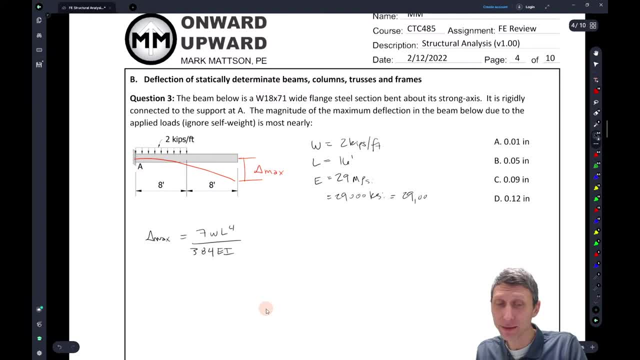 Or I mean we could say: well, this is also equal to 29 million PSI, right? So you have to know your unit conversions. there We got some unit conversions And then we're gonna look at I and some of you are gonna be stumped and say: 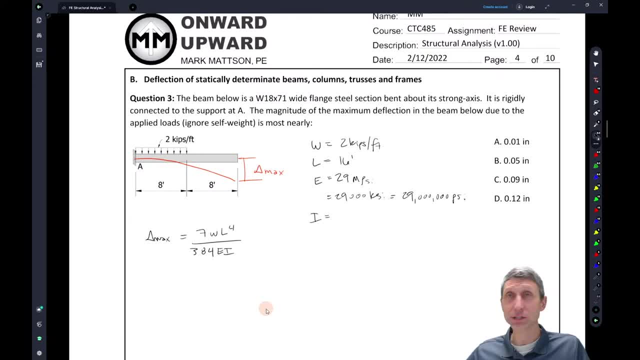 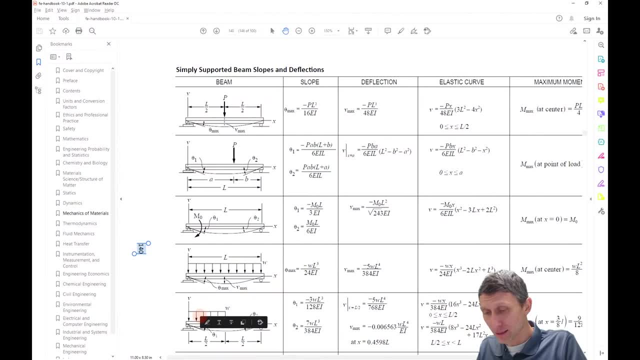 I'm like, hey, isn't there a steel manual for that? And the answer is yes, there is. And the other answer is some of these members are actually shown in the civil engineering section. So if we come back and look at the civil engineering section here, right, 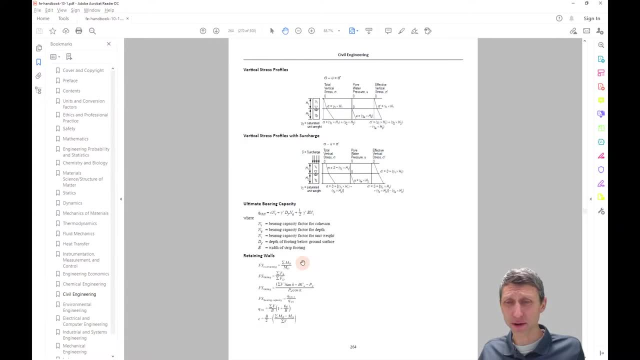 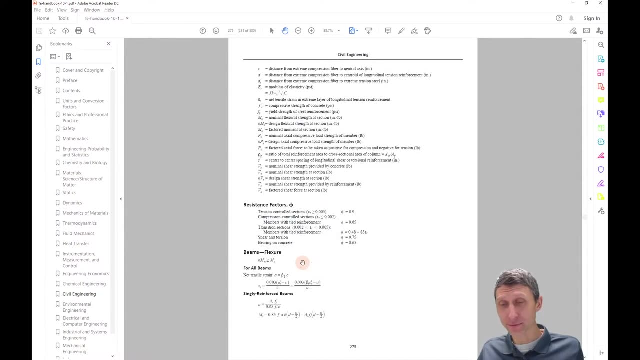 And I come in and I look and I scroll down far enough I should be able to find we'll come back to geotech in a couple of weeks. that'll be fun. I should be able to find some sections So you could just do a quick control. F. 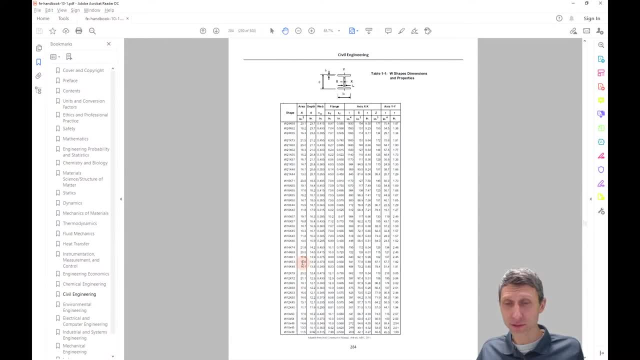 that's probably gonna get me there sooner. Oh man, I probably should have done it, So control F would have gotten me there sooner. right, An 18 by 71, though, is I get some values here. So if I look at that, 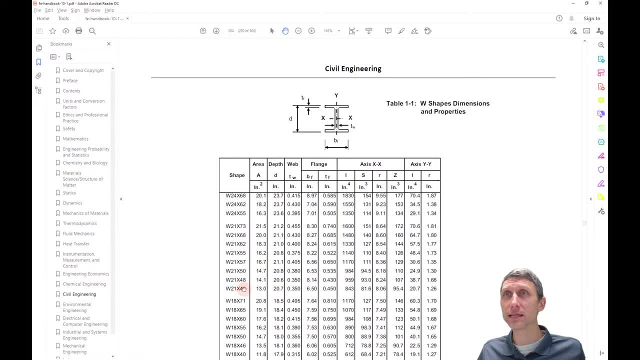 I'm gonna zoom in just a little bit here. So what I'm looking for is an 18 by 71.. I got that And I'm looking for I. so I see an I here and an I here. Which one do I use? 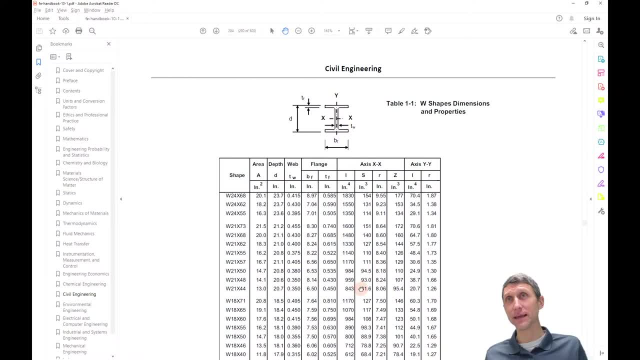 If it's the strong axis, use the big one. So the strong axis is gonna be the X value. So we're gonna take the W 18 by 71.. I value here, of what's that, 1170.. 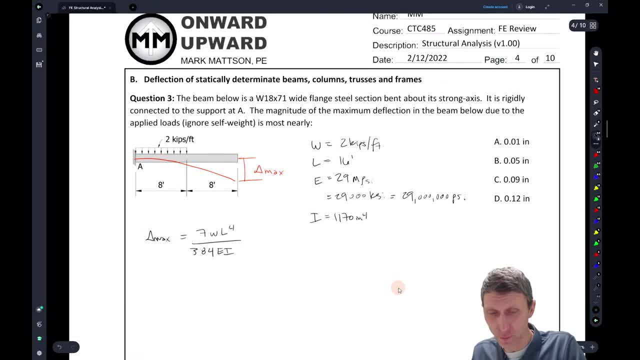 Okay, so 1170.. And that's in inches to the fourth. Did I say units are important? Maybe not this one this session so far, but units are super important. So let's look at our units here as we plug this in. 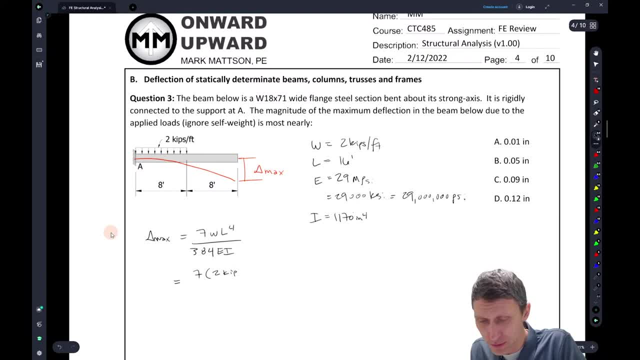 So seven times W, which is two kips per foot, times our length, which is 16 feet, That's to the fourth. Okay, And then I'm gonna divide that by 384 E, which is in, since I have kips up on the top. 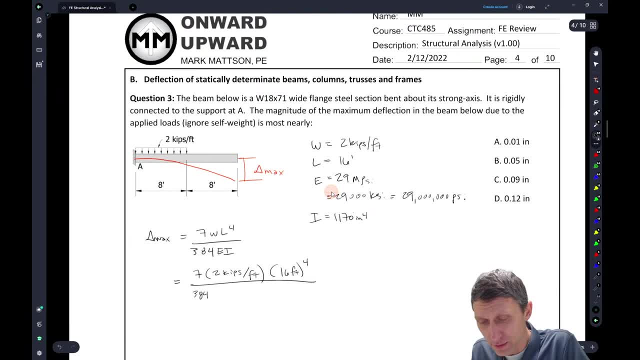 I'm gonna use kips on the bottom. I'm gonna come back in here and I'm gonna say this is gonna be times 29,000 kips per square inch. Sometimes I like it like: rather than write KSI, I like to write kips per square inch, like that. 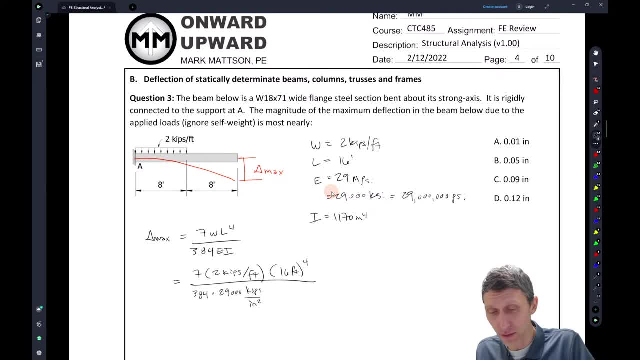 because it's easier to cancel out units, right? So we have the kips per square inch, And what else do we have? We have our I. our I was 1170 inches to the fourth. Okay, so we have all the numbers. 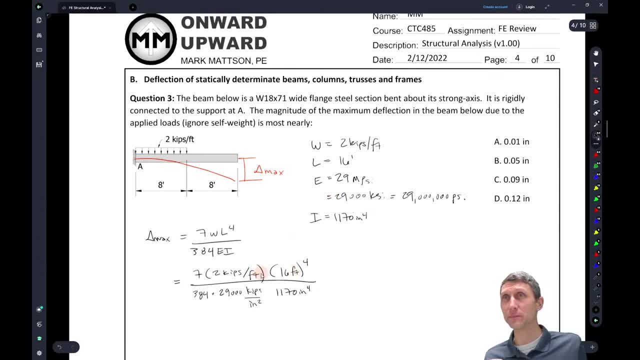 but you'll notice that we have units that are inconsistent. We have feet on the top, we have inches on the bottom. The kips are nice because the kips cancel out. Okay, so the kips cancel out, those are good. 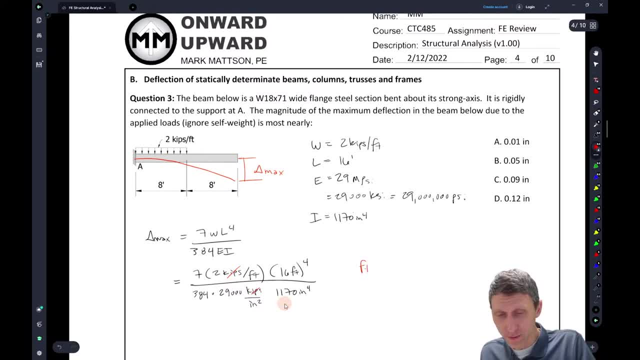 But if we just look at units, we've got feet to the fourth divided by feet. right, That's our feet to the fourth divided by feet, And then on the bottom we have inches squared under. well, here let me, actually let me write it this way: 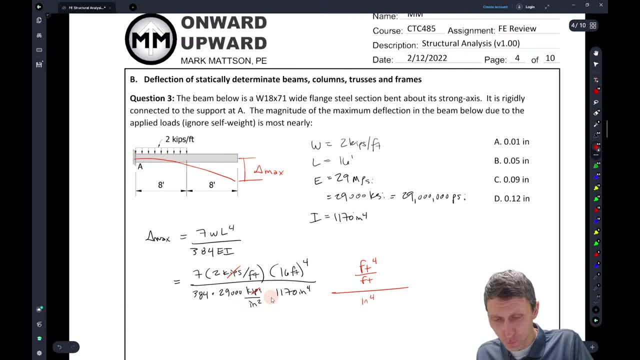 We've got inches to the fourth divided by inches squared. So if we keep going we're gonna get feet cubed divided by inches squared And we see we have to do a conversion. So the conversion that I'm gonna do is I'm gonna multiply this. 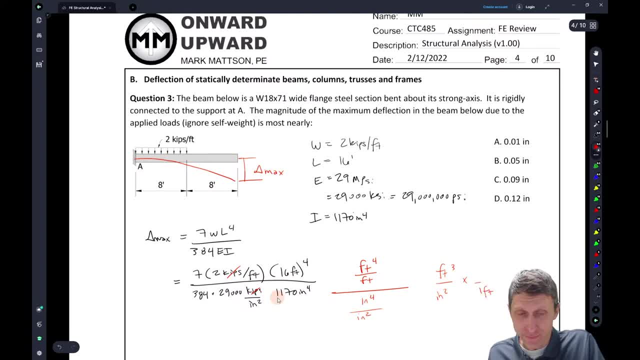 by what I know, for every one foot I have. my units are in inches, So I'm gonna try to get this to inches. for every one foot I have, I have 12 inches and I'm gonna cube that. When I cube that, what happens is the feet go away. 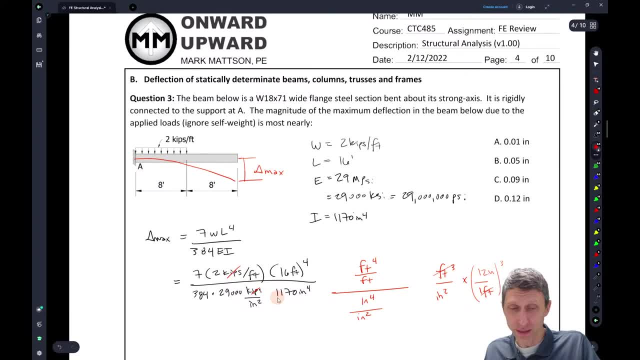 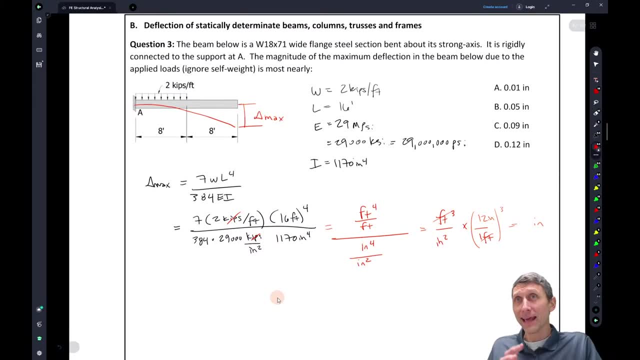 All the inches except for one. this kind of gets me to units of inches, right? So the red here is just the units. The red is just the units. but basically the long and the short of this is this is: these are kind of like that's not equal. 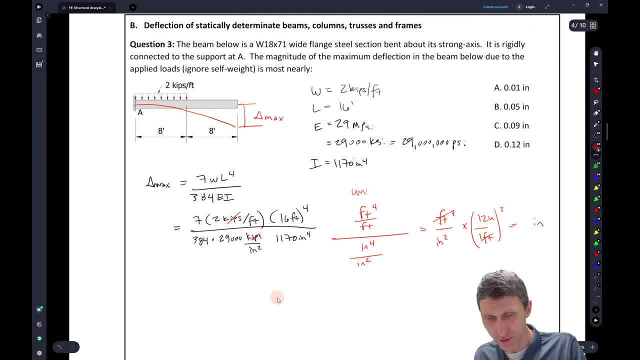 These are just units, right? So this is just units over here, And if I could spell it, that would even be more helpful. So units, okay. So what we have here is these are all our units, but we need to multiply this by 12 cubed. 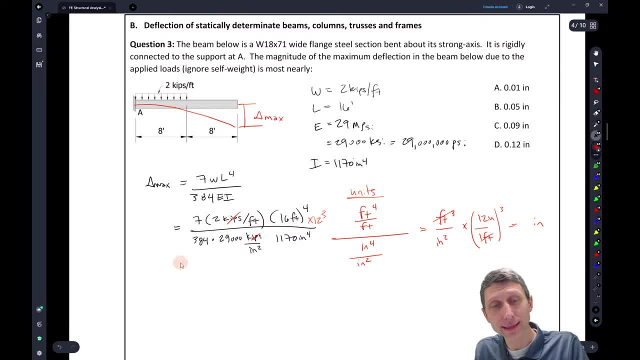 in order to get our answer. So once you know the units, this gets a little easier. This is a little bit of a maze to go look up the different pieces, whether it's E or it's I or it's the fourth. 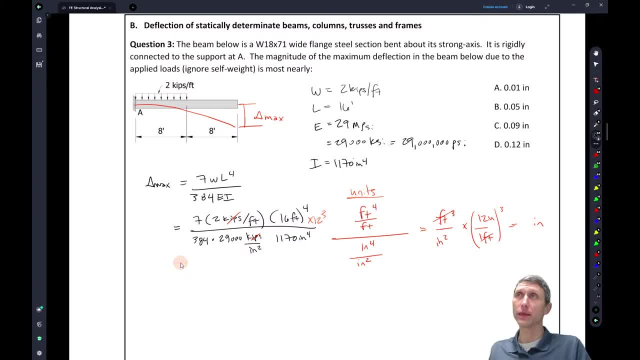 or it's the formula in the first place. So you have to be really familiar with that reference handbook to go do this. But if we type this in now, hopefully we get the right answer. So seven times two times 16 to the fourth right. 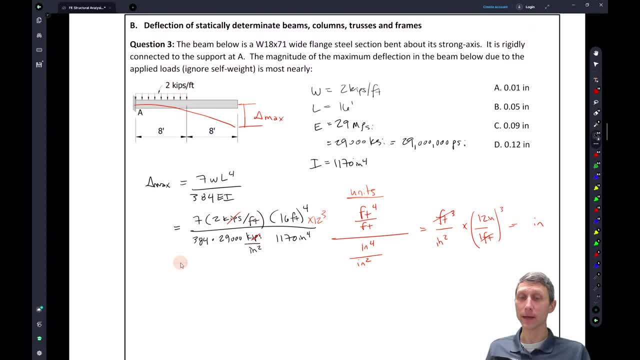 Times 12 to the third, okay, And then divide all that by 384 and divide that by 29,000.. I can plug it in right here And divide that by 1170, which is our moment of inertia- And I get like 0.12.. 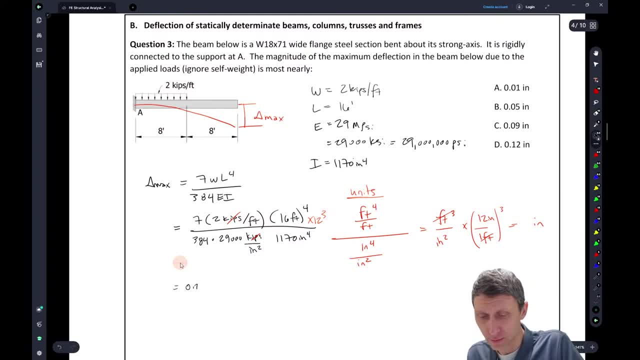 So 0.12,, 1, 2, it's like 121 or 122 inches, So that's close enough. It's most nearly the 0.12,. okay, But this brings up that approach to the FE where you have to understand. 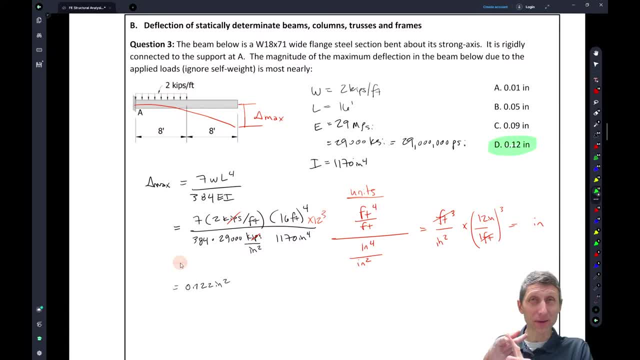 you have to totally understand where these formulas are when to go look them up. You have to understand what the units are. You have to understand kind of where to find your E, your moduli of elasticity, if you don't just remember it. 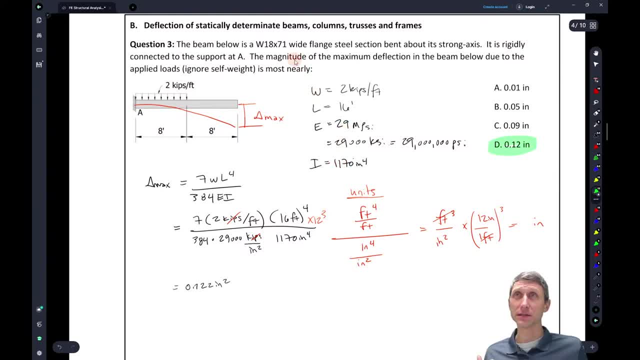 And you have to know how to find this I value, because it's not just gonna be given. I mean, maybe it'll be given to you. If they do give it to you, that's even better. Then you don't have to go find it. but there it is. 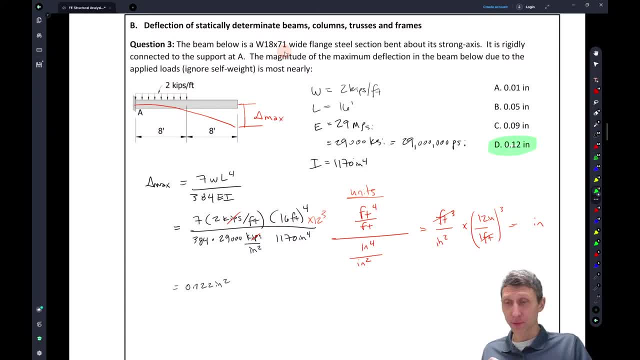 All right, question three is done. Okay, let's keep going, because we got another deflection one, And, for those of you that are still watching, you can do that here as well. If you don't do it now, I think that's gonna be a challenge. 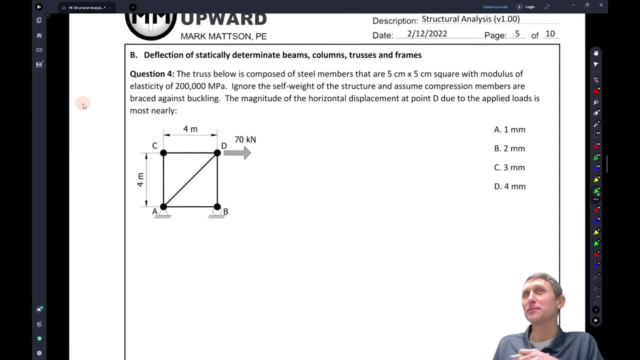 You could do that in the next one, you that took structural analysis with me. you guys are going to grow and you're like principle of virtual work. oh man, that's terrible. okay, it can be terrible, it can be, it can be complicated, but i've, you know, i've been surprised sometimes talking to people where, where you know, 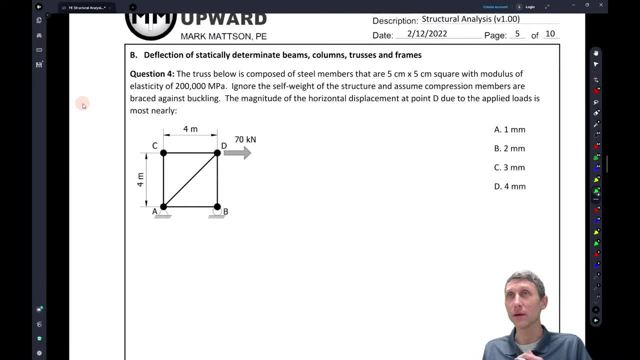 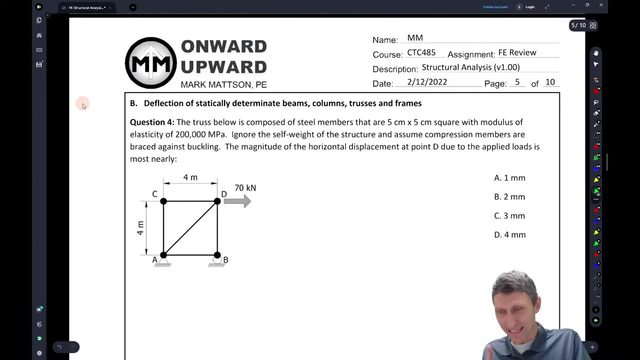 they'll take fe concepts that i think are too complicated to throw on the exam, but they'll take them and throw them on the exam and try to make them less complicated, okay, so, uh, so we'll go from there. so, so let's take a look at this one, right? so, ah, man, i keep seeing comments a little. 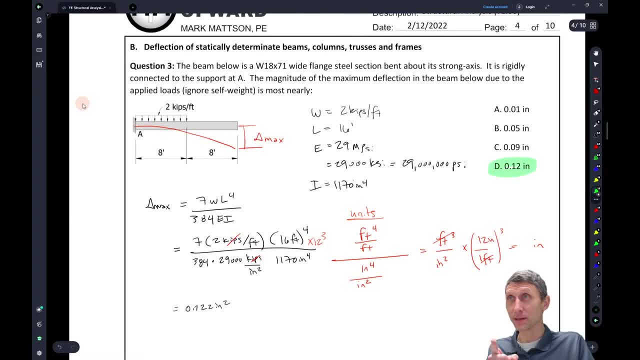 bit late here. i'll try to keep a better eye on it. uh, but thanks, mike for jumping in there. the x axis, right? um, if we're, if we're bent about its strong axis, that's ix. a strong axis is ix. there you go. strong axis is ix always. 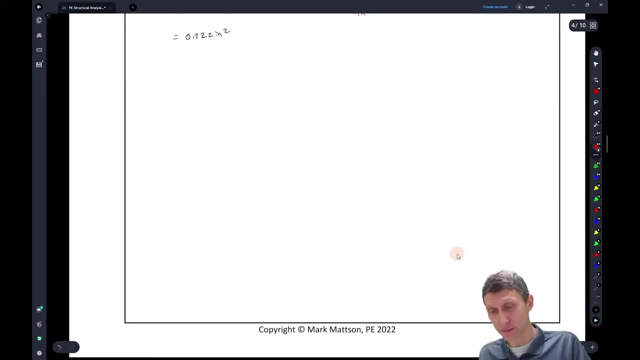 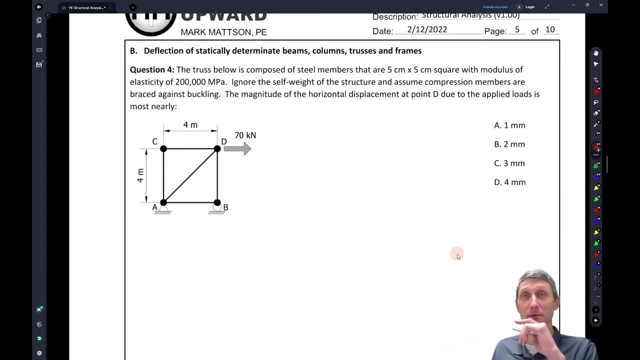 you for, for what we're doing in this, this, uh, for this test. let's come back here though. principle of virtual work for trusses, deflection and trusses, they say. one of the one of the requirements here is that deflection is statically determinant. trusses, okay, uh, we kind of did columns last. 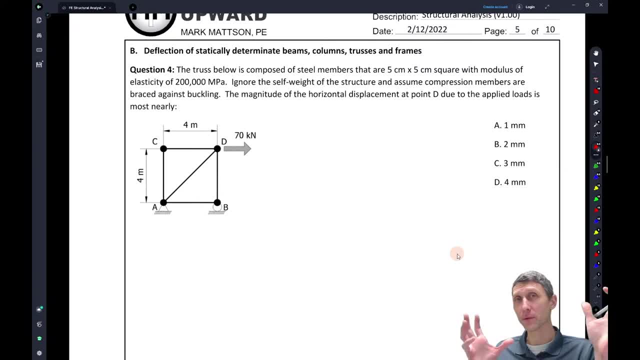 time with that pl over ae formula. if you remember the pl over ae formula with a couple members, that in mechanics and materials section and we said: well, what force will cause this thing to deflect a certain amount? so that's kind of like a column with pl over ae and the trusses is honestly 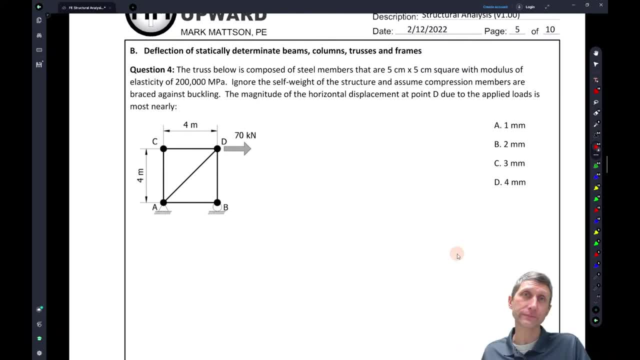 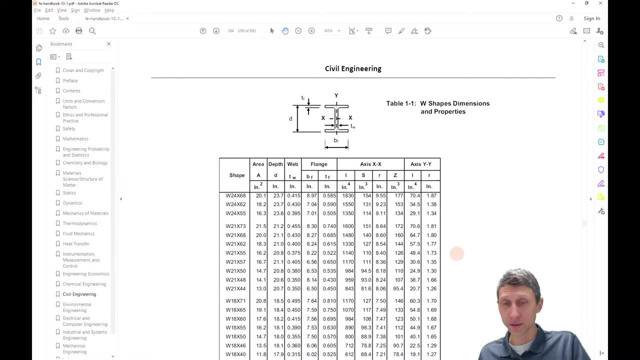 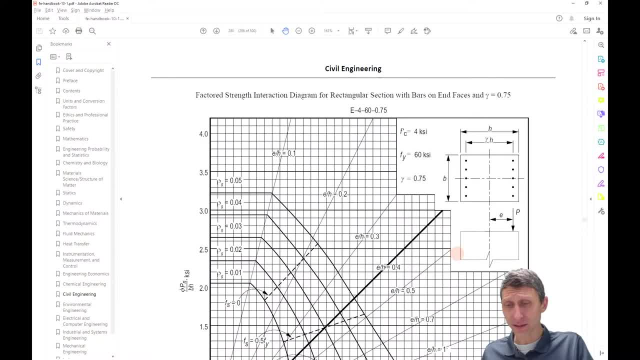 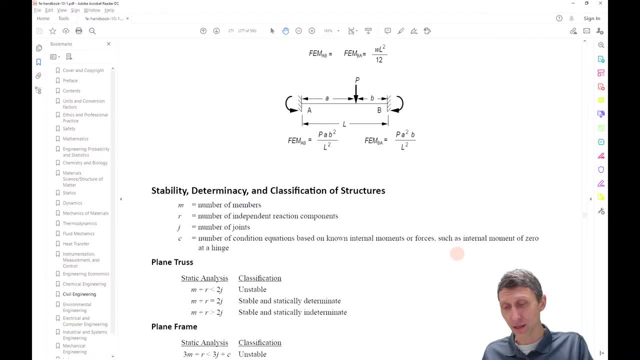 what we'll see here is actually: i'm going to keep coming back past steel components, back into our structural analysis section. so if i come back all the way to structural analysis section, uh, there's determinacy. we'll come back to determinacy in a little bit here, but i want to just keep coming. 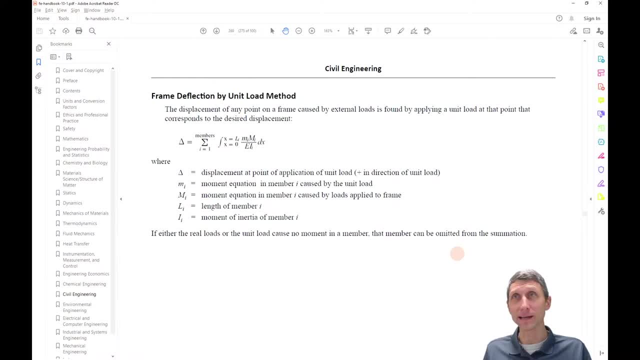 here, and this is framed a little bit differently than what we've seen in the past. so let's go back here. and this is framed a little bit differently than what we've seen in the past, so let's go back. deflection using a unit load method: again, this is more kind of uh, this is more calculus, and 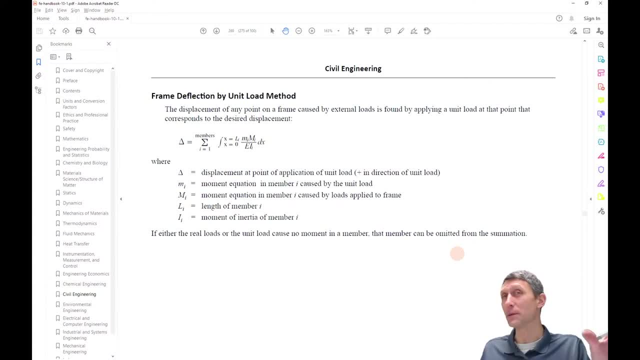 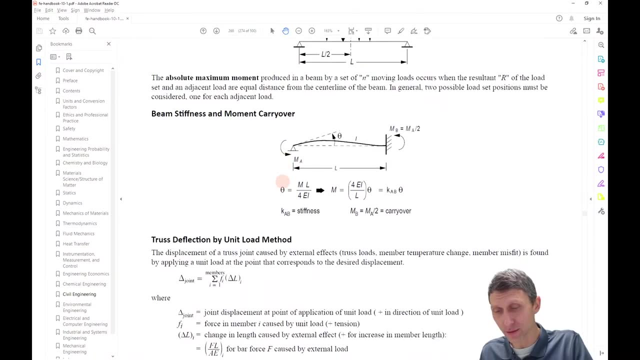 integrations. this is kind of a a follow-up to the question we're doing, so this is a little bit more complicated than the question we're doing here. but the question we're doing here is going to take a look at the truss deflection by the unit load method. so this is a similar type of thing. 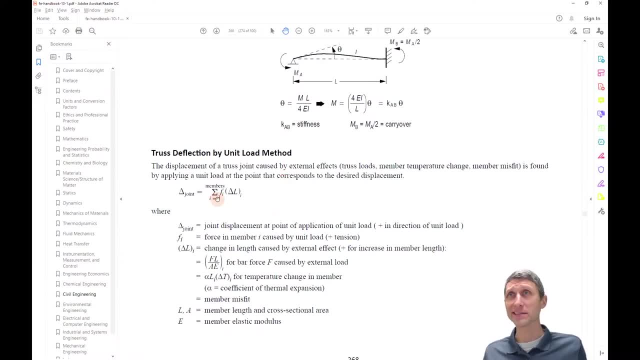 but instead of using integrate integrals, we're using a summation. it makes it a little bit easier, makes it a little bit more doable, but what we see here is a big formula and you might want to look at, you might see this formula and just say: flag, i'm moving on and uh, not even uh, not even try to solve. 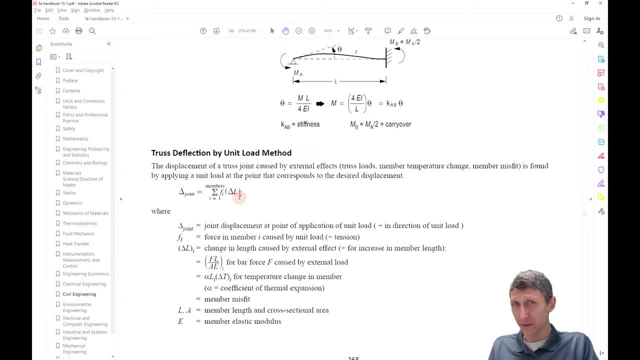 it. but honestly, if you see a principle of virtual work, uh problem uh for a truss or deflection into truss or something like this, it's probably going to be actually a fairly simple truss or a fairly easy problem in the sense that there's going to be a lot of zero force members to make the analysis. 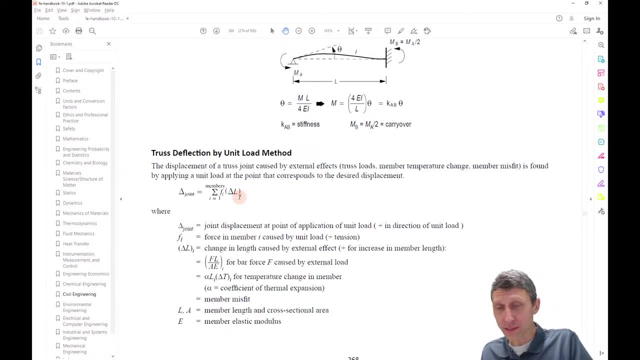 doable in a short amount of time. so what we see here is this, is this, uh, is this formula of: we have a delta of a joint, so displacement of a joint is equal to the summation of fi, which is the force in the member caused by a unit load. 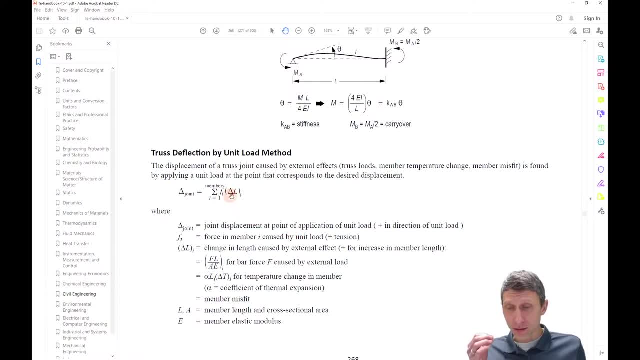 like a one kilonewton load here the times delta, li, so delta. i remember that pl over a formula from this is fl over ae. it's the same thing, but f is the force instead of p, right, so we have this. f times fl over ae. okay, so the um. 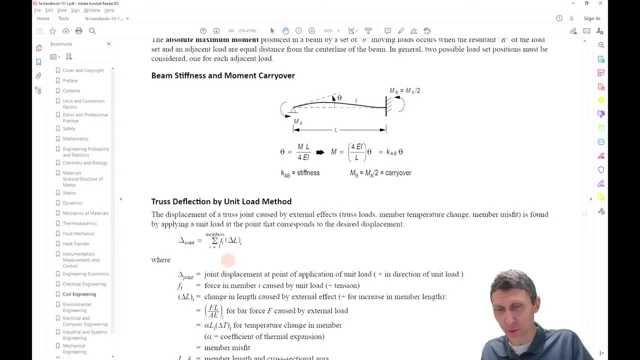 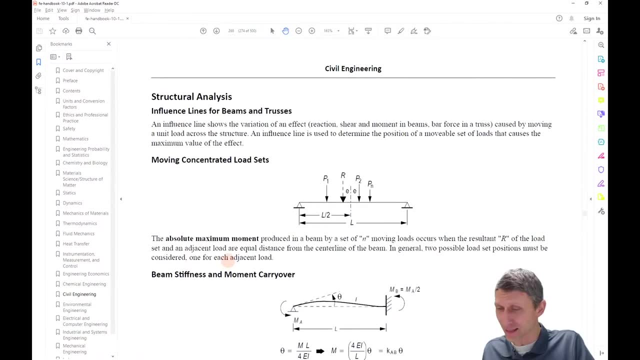 so so yeah, i mean this kind of gets in there principle of virtual works a little it's, it's, it works kind of the same way. um, but yeah, we're not going to get into all that there is. i do, does this have a principle of virtual work section? i'm trying to think, uh, if i, if i remember in here, 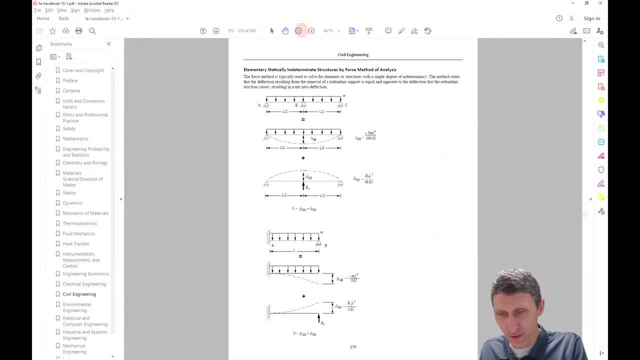 correctly we? i don't remember i'd have to search um, but why don't i? why don't i for shul uh work. sorry, i can't spell today. actually my keyboard is off to the side, so there is no principle of virtual. this is essentially a principle of virtual work. okay, so 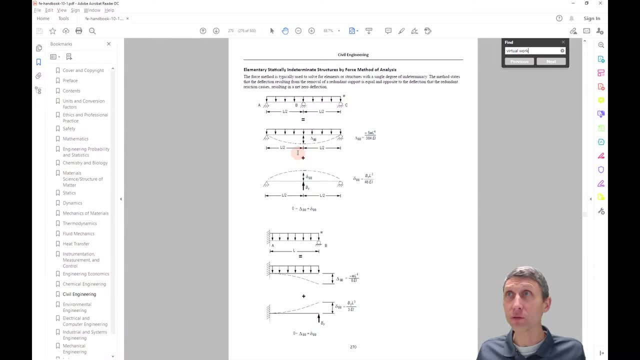 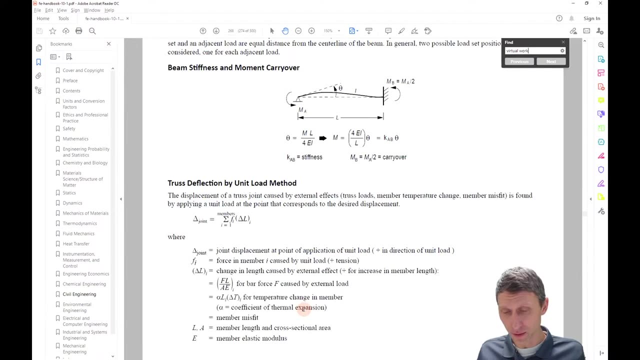 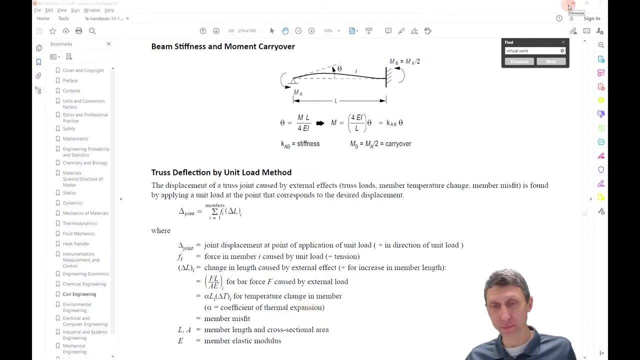 it's just that that's where we're going with it, okay, so, um, so, let's just jump in here and we'll we'll take a look at what this looks like, okay, so, so, so, let me come back over. let me come back over here. um, what we have is uh. 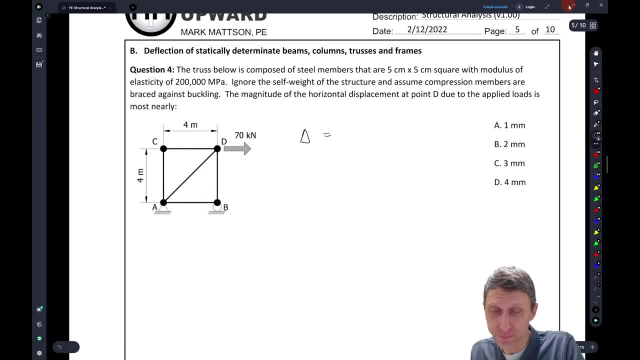 formula that essentially says the delta equals the sum of little f. you know, big f- l over ae. okay, so we need this on that. so we need to find a couple things, and this is where, um, the little f is the force. uh, based on a unit load, um, big f is the force. 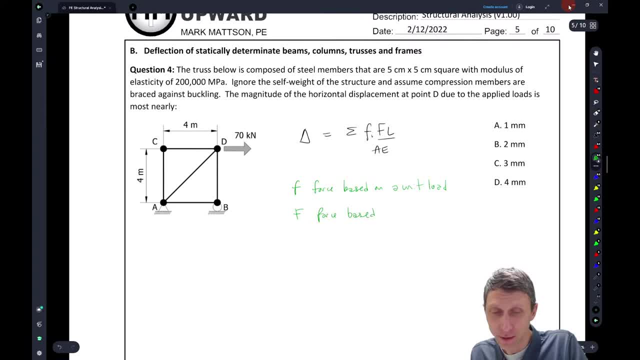 uh, based on, uh, the actual loads. okay, uh, the l is the length of the member, a is the area and e is, uh, the modulus of elasticity. all right, so with this we have to find a couple things, but what we can see here is is right off. 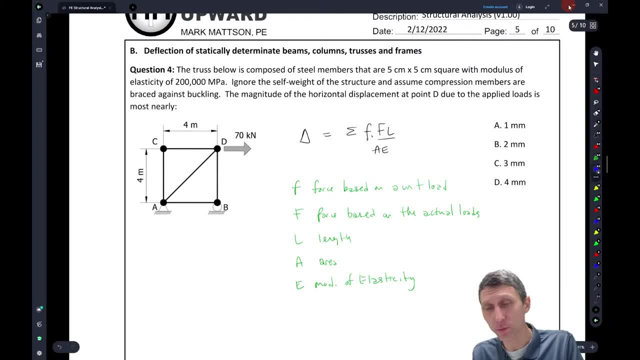 the right off the bat. we see, well, if we put, what are we trying to find here? we see that we're trying to find. we have, well, we have a truss. we're given five centimeter by five centimeter squared members with a modulus elasticity of 200 000.. so this question, the modulus elasticity, is. 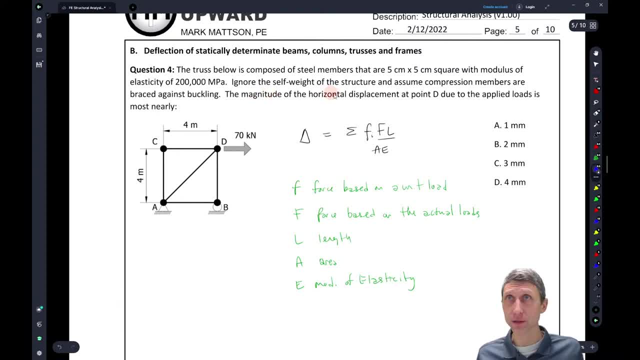 just given. okay, ignore the self-weight truss, ignore self-weight, assume compression. members are braced against buckling, so we're not getting weird things going on and you don't have to evaluate for buckling. um, the magnitude of the horizontal displacement at point d due to the applied loads is most nearly so. anytime we're doing this, what we're. 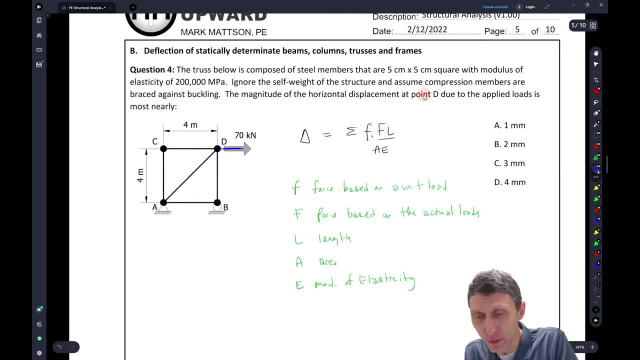 going to do is we're going to put like a unit load at that point. so we're going to put this like one kilonewton load at that point, and and first we're going to analyze it like that. and if we do that, um, i'm just going to throw, throw a couple things out there real quick. so do you remember? zero force. 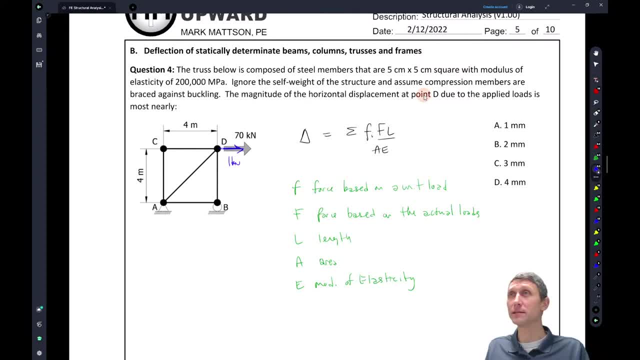 members. zero force members could totally show up on the exam as well, uh, but but zero force members here if, if you remember, like let's just, let's just take a walk down zero force member lane for a minute. so if we look at like joint c for example, okay, joint c um, we have a couple forces. 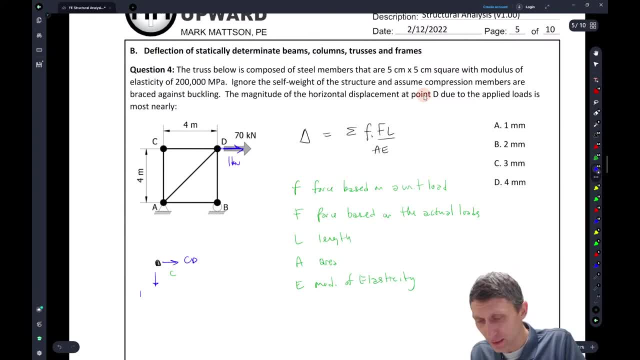 coming out of joint c, where this would be like cd and like uh, ac. if you just look at joint c? um, basically what we have going on here is we've got joint c and and if you take a look at this um, we're looking to see that the sum of the forces in the y direction equals zero: the sum of the forces. 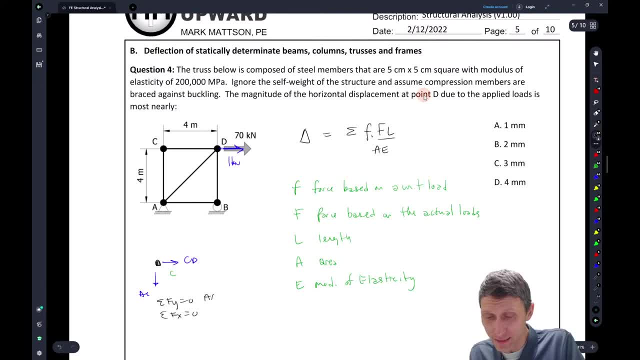 direction equals zero. we can see from the y that ac equals zero. we can see from the x that cd, um also equals zero. okay, so we can see both of those right. so so hopefully that makes sense and isn't too crazy. but what that tells us here is that this is zero force. this is a zero force. 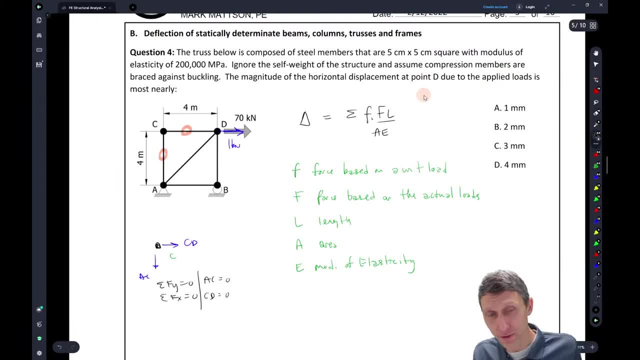 similarly, if we look at, you know, joint b at the bottom here, if we look at joint b right, if we look at joint b, and this is what joint uh b, um, we're going to have some reaction at b right, this is going to be like by. i will probably have like a bd. 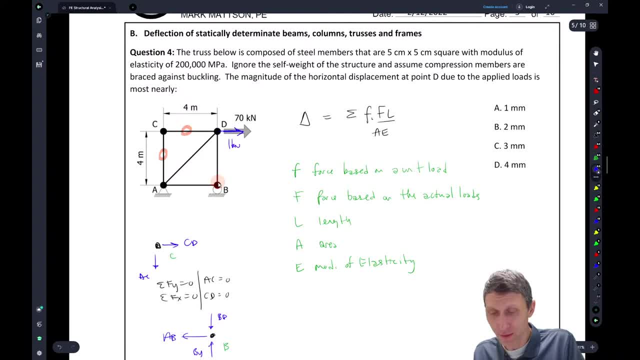 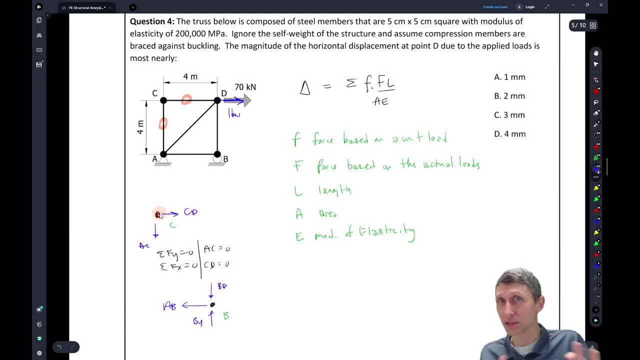 and then here we're going to have like a, b, but if you remember, i mean, hopefully you don't have to go through these free body diagrams on the fe- i'm doing this here just to kind of refresh your memory about zero force members. right, did you remember zero force members? zero force, uh, members. 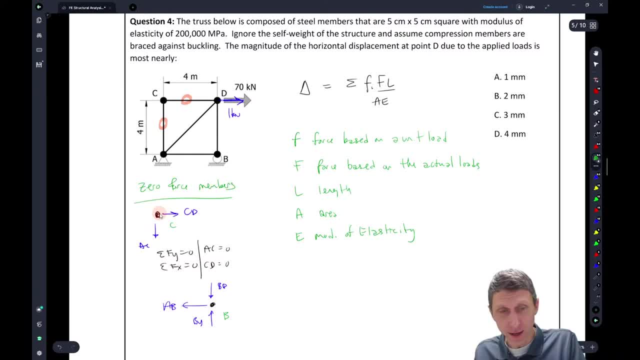 right. so this is where, hopefully, you can remember some of these things. but, um, what you can see here is, if we sum forces in the x direction equals zero. um, a, b equals zero. okay, so so basically same thing going on here. and what does that mean? so that means we have a force here that's zero. so 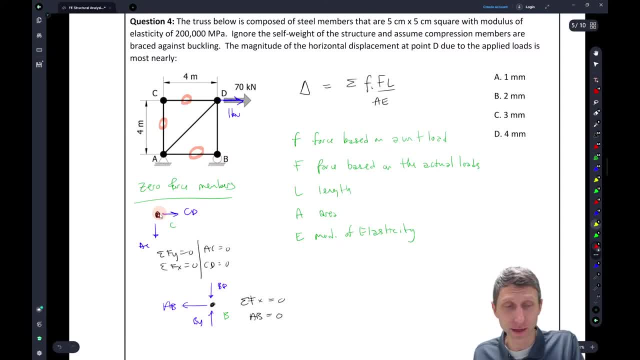 there's only two forces in this truss that are going to have to, you know, have to hold, or, i'm sorry, there are only two members in this truss that are gonna have to hold four, so we have, uh, ad and db. okay, so, hopefully, just from remembering a few things about zero force members. 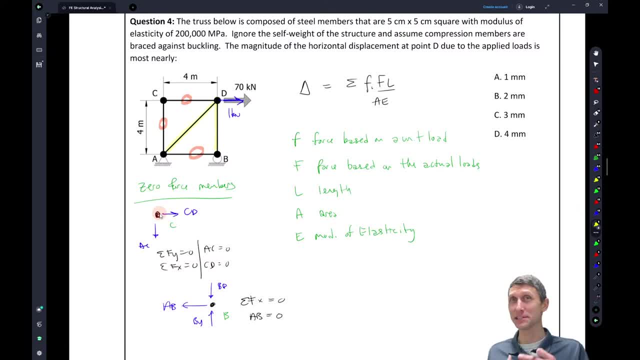 can go ahead and you can take a look at these members and just say, oh, you know, not having to do this whole kind of like analysis here, you can go ahead and solve and say, okay, I know, this is your horse members, I really only need to solve for. 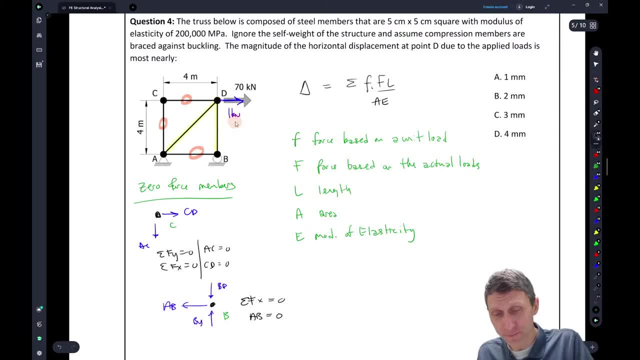 these two forces. so if we do that, what we're gonna do here is we're gonna take that joint. what joint do we have left? we have joint. let's look at joint D and I'm gonna put my one kilonewton force here and I'm gonna have my force. what's this? 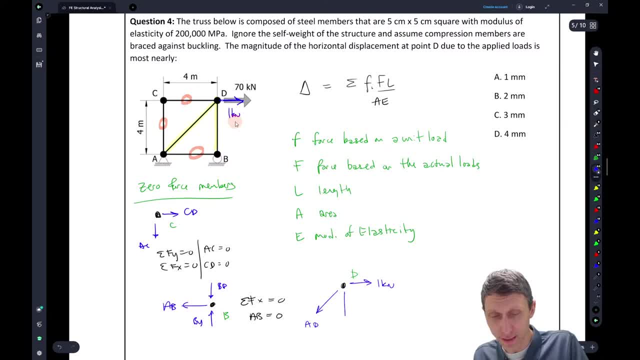 this is maybe called a D and force a B. I'm gonna put a B up because I kind of know it's in compression, but let's take a look at the geometry here and see if you guys can do this, maybe in your head a little bit even. but 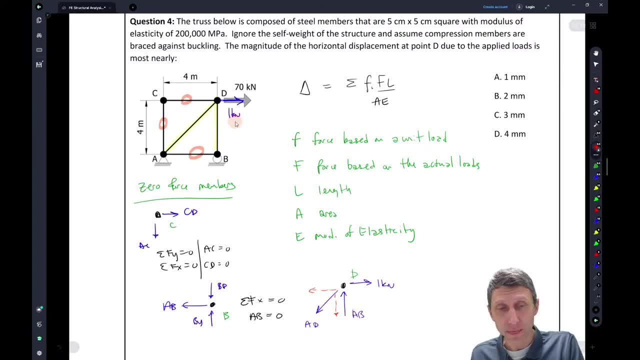 if we take a look at this thing going on, what do we have? we have the sum of the forces in the X direction equals zero, right? so what do we get? we get this component. ADX has to equal, essentially, ADX has to equal one kilonewton. do you see it? these two forces have to be equal. 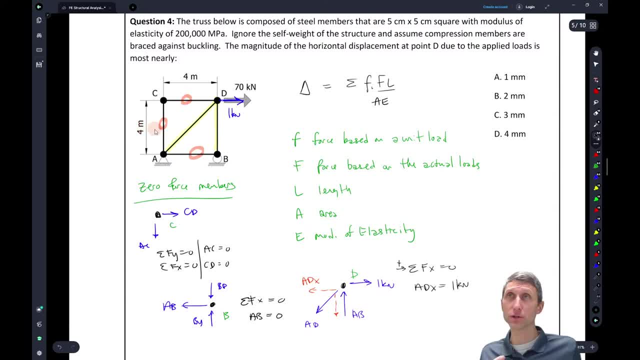 horizontally. and then this truss got even easier because we have a 4-4 triangle. so I tried to make this kind of easy. so the math wasn't too crazy. you didn't have to go do geometry to relate components here. hopefully you can see, since it's a, you know, a 45 degree, you know. 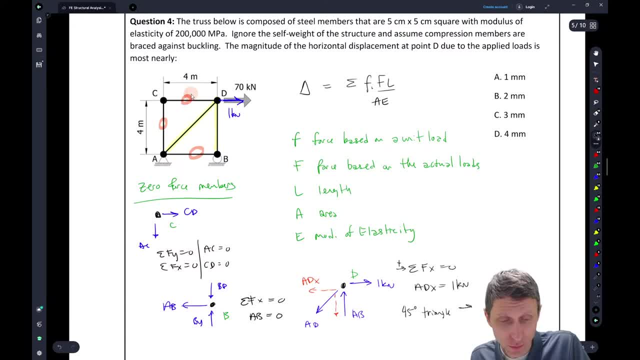 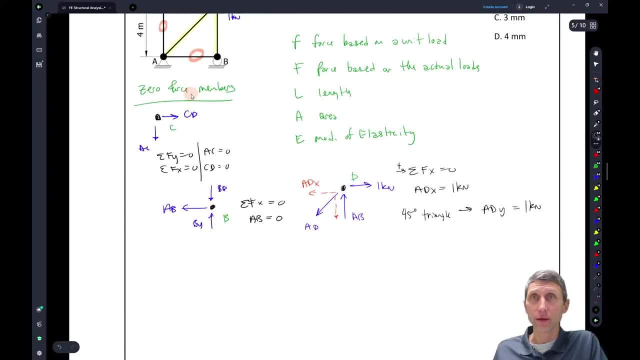 triangle. you can see that it's a 45 degree triangle. so you can see that it's a 45 degree triangle. that means that means what it means. ADY also equals one kilonewton. okay, I'll get my head out of the way, right, and can you just? can you? can you do that without having to write it down? 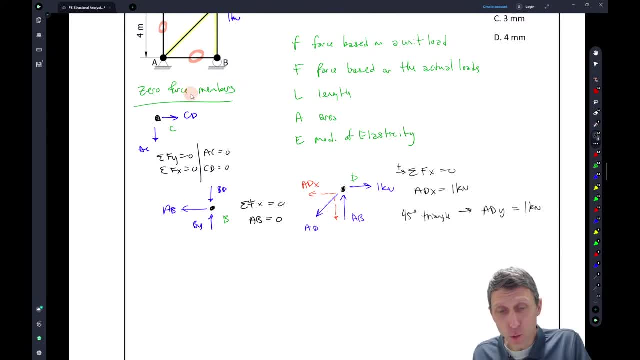 I hope so and hopefully that means now, once we have that, we can say: sum of the forces in the Y direction equals 0 and we can say: well, AB, you know, AB equals ADY, y equals one kilonewton, right. So this trust, the analysis of this trust, everything just equals. 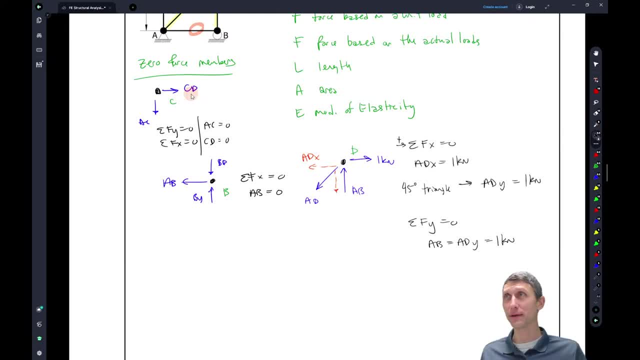 one. I mean it's kind of a simplified version here, but hopefully it makes a little bit of sense right? I mean basically the horizontal forces have to balance, So the one kilonewton balances the ADX. The vertical and horizontal components of AD have to be the same. I should. 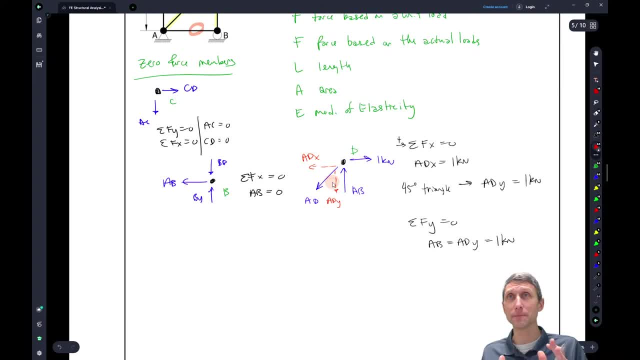 probably label this one here AD, why they have to be the same. So since they have to be the same, that means you know they both have to be one. Then AB and ADY, they're the only two vertical forces that each have to be one. So again, trust analysis, but we're taking it a little bit further. 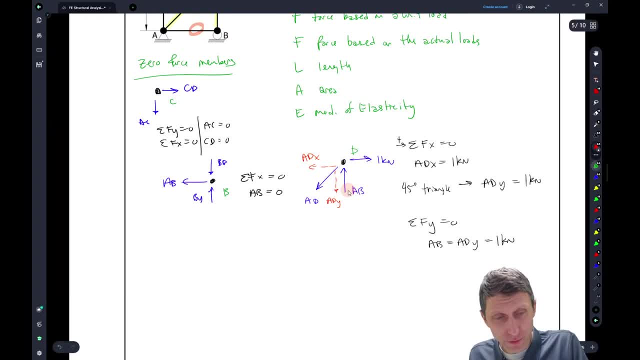 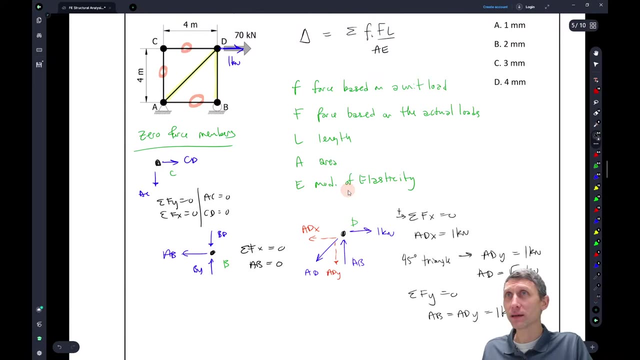 here. Okay, The last thing that I want to do is with that 40 feet five degree triangle, we also can solve for AD, and that's just going to equal the square root of two kilonewtons, So one times the square root of two. Okay, Once we have that, okay, once we have that, we can take a look up. 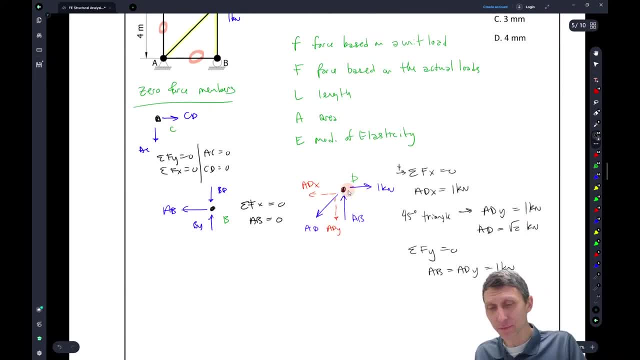 here And what we see? Okay, So once you solve it once for one of these, as long as all of those only one load, it makes it really easy if that's two. So what we see is: what's the difference between the free body diagram we just drew and this? 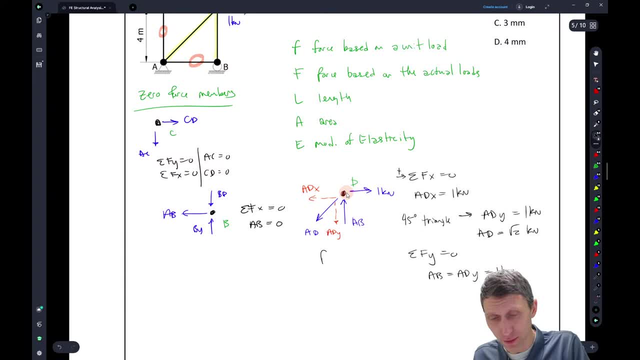 this. so this is for, like little forces, Fi Right, So that's for low forces left. I what's the difference between that one And you know, if we have a D, 70 kilonewtons and AB, you see, 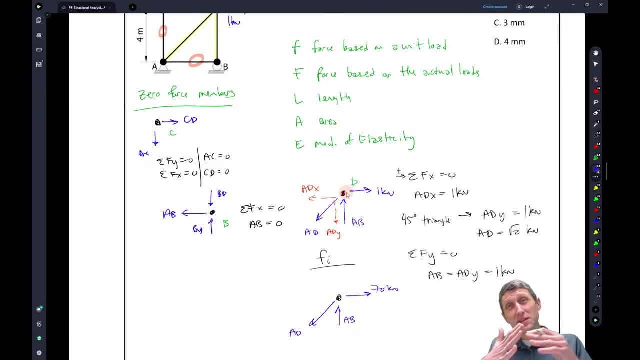 the only difference is multiplied by 70, right, So once you solve it once for one of these, as long as all there's only one load, it makes it really easy. If that's the only one load, it makes it easy. 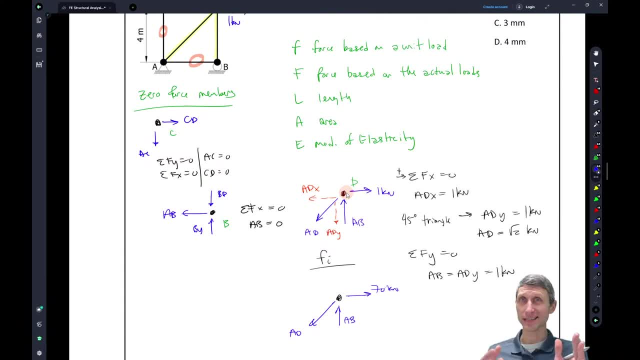 it makes it really easy. If there's only one load, it's super easy. And I say super easy, you don't have to go reanalyze it. So this, you know, this is essentially, if we have F, I capital, F, I right. So this is the, this is the big oops, this is the big load here, right? 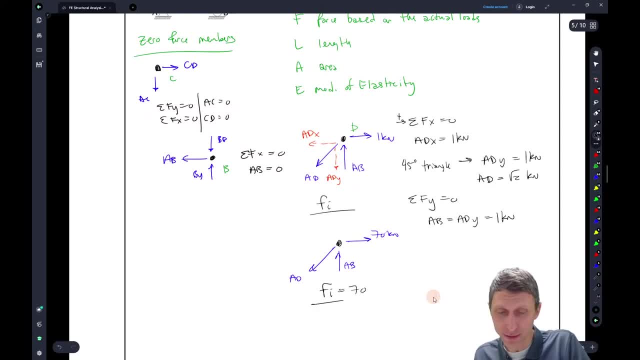 Fi is just going to equal 70 times little fi. That okay In, because it's all the same geometry and it's all the same, except for the magnitude of the load. Okay, so if we're, if we're doing the unit load, the principle of virtual work here for trusses- what are we going to do? we're going to 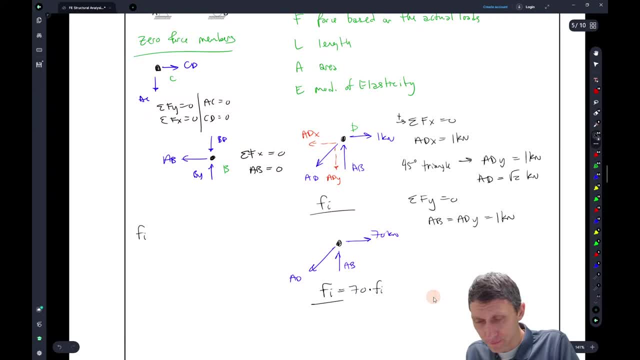 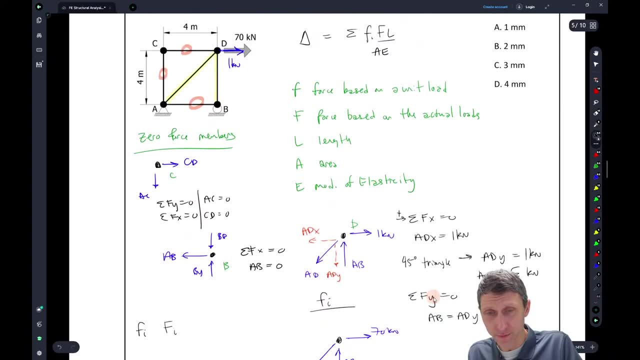 say that we, I'm just going to make a table, I'm going to say fi, F, I, and then what else do we have? we have what's our formula? it's FFL over a. so I'm just gonna do FFL and then F, F. 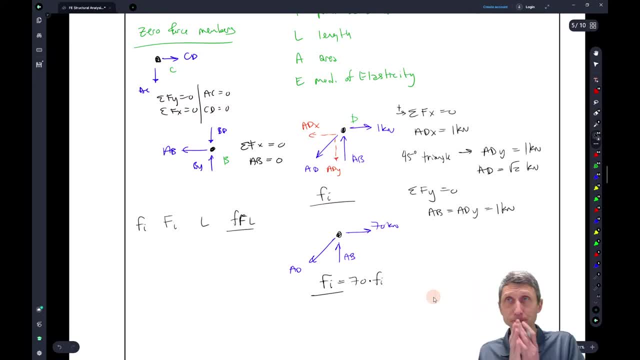 L. So I'm just gonna- I'm gonna leave a out for a second, And what I'm going to do here is I'm going to do one for each member and I'm at. it didn't look good, So I'm just gonna rewrite it here for a second: F capital, F L. So what members do we? 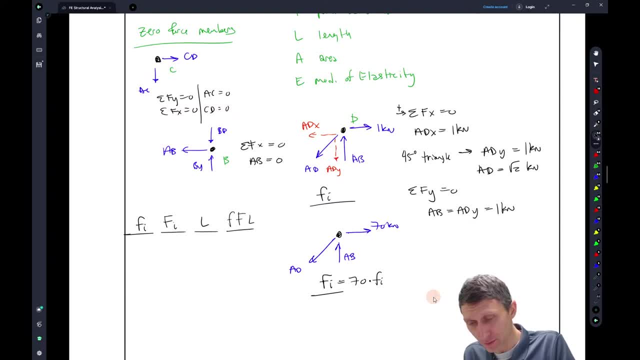 have? we have two members. basically we have member members. I'll just write it here: ad and ad, Right, so we have two members. ad we said little fi, right. so little fi ad was going to be the square root of two And big fi is going to be 70.. So we're going to write it here And. 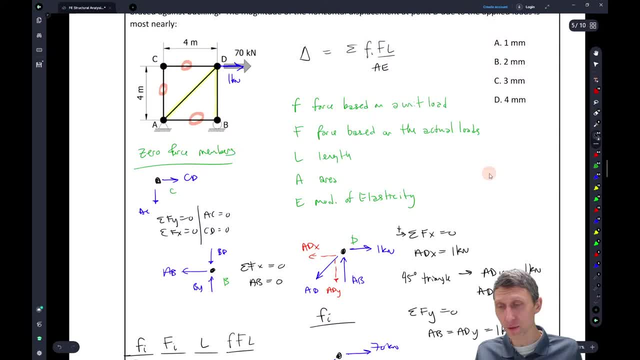 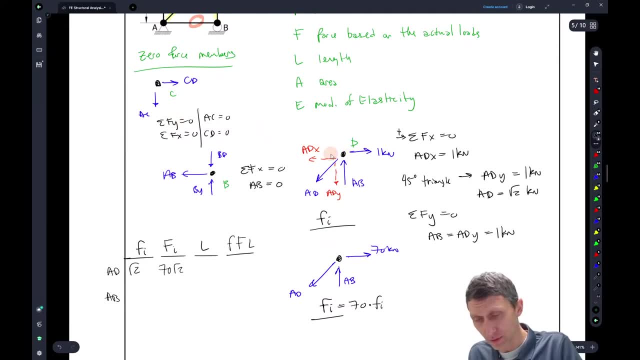 then the length, right the length. if we have a four, four triangle, this length is going to be four square root of two. Okay, so, let's come down here. So four square root of two, And if we multiply all that out, what do we get? we get 70 times four times, two times the square root of two. 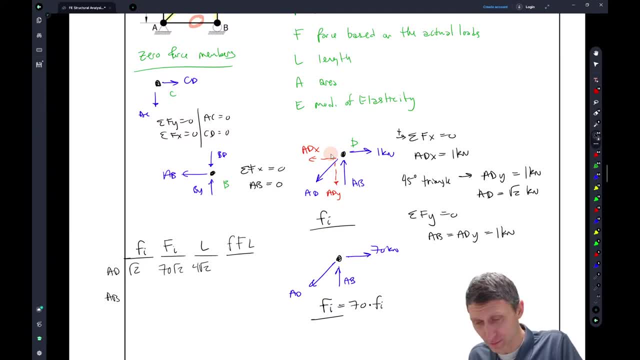 did I do that Right? I got like 791 or 792.. Roughly okay, I multiply all that out ad ad. what's ad? Well, ad, we said was one. we said was 70.. We said the height here. 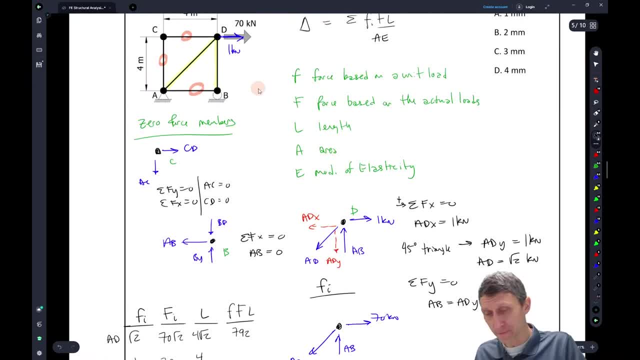 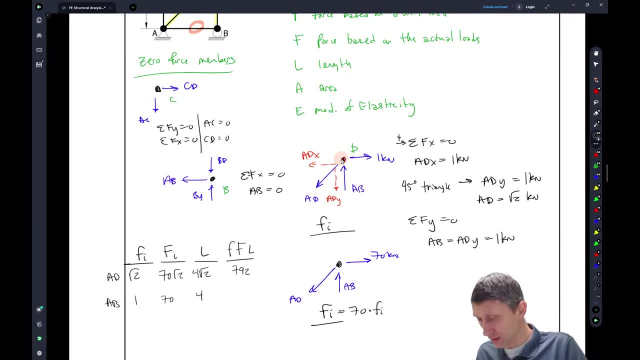 that height is going to be just the four meters, right? So what's the height? it's going to be four, So four times 70. What's that? 280?? I believe so, if I can still do math that. so if I add those two together- 792 plus 480, or 280,, I'm sorry, I get about 1072.. 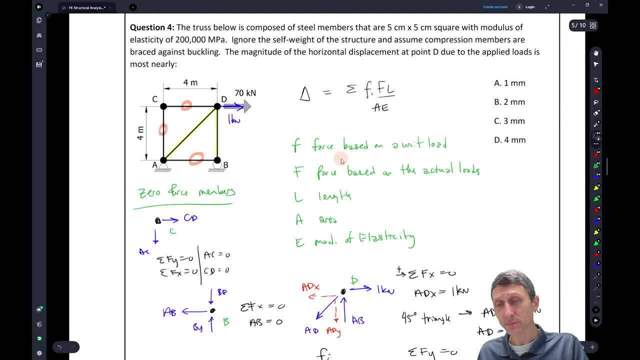 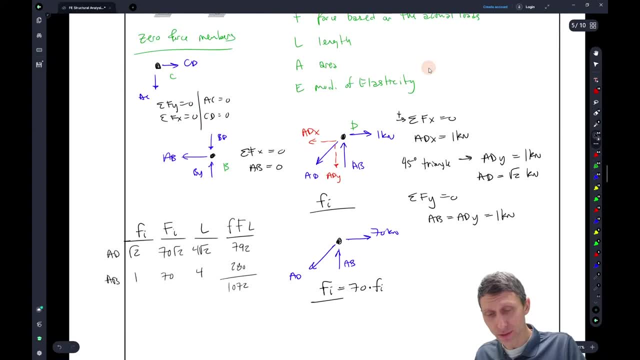 And somebody's out there is wondering: well, what about A and E? Well, A and E are constant, So I'm not going to put those into my my sum here. I'm gonna, I'm going to do those afterwards. So let's do this out And we'll, we'll plug in the equation. So here's kind of where that principle. 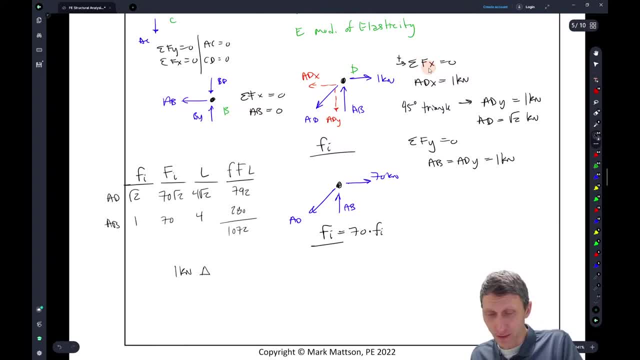 of virtual work comes in we're doing: one times delta is going to equal one kilo. Newton times delta equals what? it equals the sum of F FL over a E, and since he is constant, we can pull this out. So now I'm just gonna write this in. So what's that sum? this sum is right here, So it's gonna be. 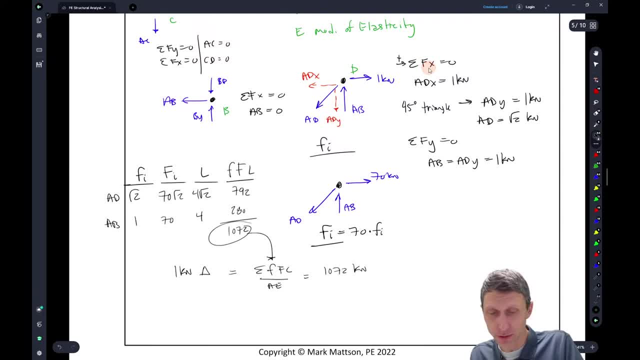 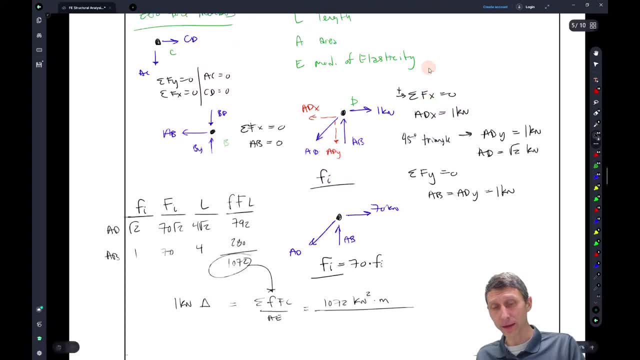 1072.. And if you look at the units, I'm gonna have kilonewtons squared times meters. and now I'm going to divide. And what am I dividing by? Well, I'm given centimeters and mega pascals. So what? 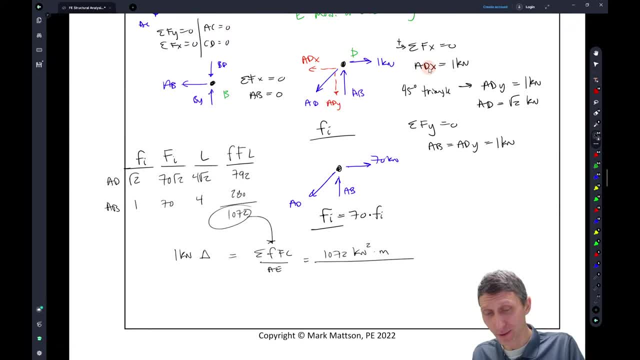 units. you want to use the units that I'm going to use here. or I'm going to say: well, I'm going to say, I'm just going to translate this to millimeters And I'm going to say: 50 millimeters times 50 millimeters times 200,000, mega pascals. mega pascals is a Newton per. 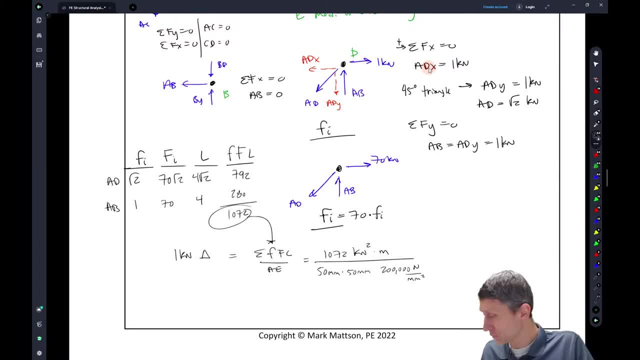 millimeter squared. Okay, so let's see if I can do my units right. And so what do I need to do here? I need to. I need to figure a couple units out, So let me just make sure I'm doing my units. 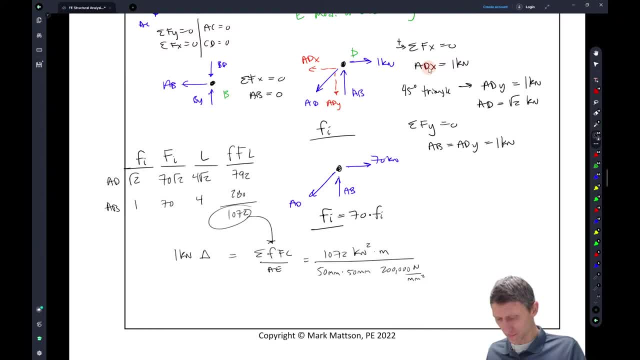 right, Because I think I screwed something up. Did I screw something up? Maybe I might have screwed up units here. So let's just take a look, Let's see what we got: The kilonewtons go away, Right. so if I'm just going to cross things out, the kilonewtons go away. 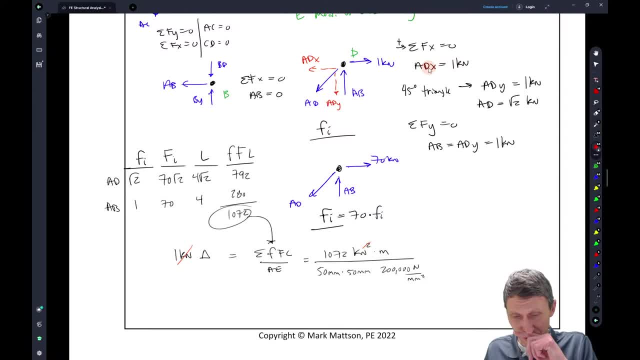 I get one kilonewton to go away. What else do I need to do? Well, now I have the millimeters squared go away And I've got some inconsistencies with the main units, I've got a kilonewton on top. 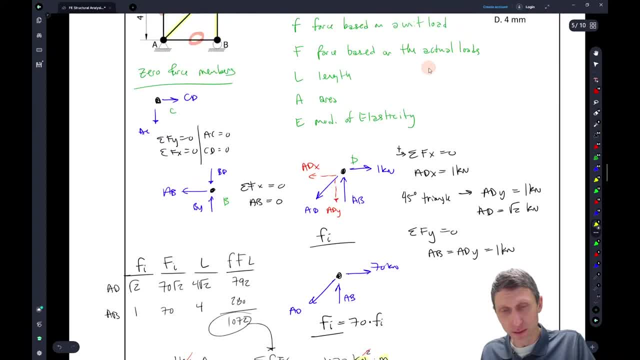 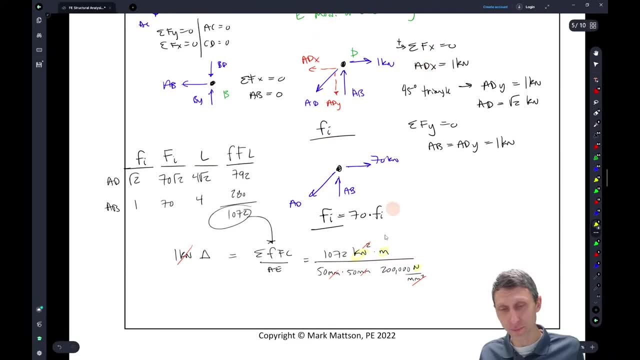 a new on the bottom. I've got a meter on the top And if we're looking here, we want our deflection or displacement in millimeters. So I want to convert everything to millimeters. So I'm going to come back down here And what I want to do here is I want to get rid of that killing and so 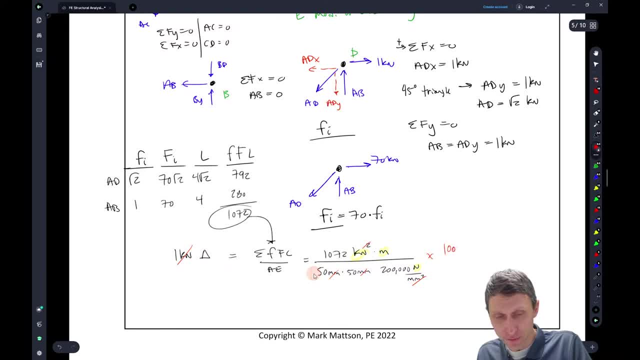 I'm going to multiply times per 1000 newtons, I'm gonna have one kilonewton. So my new kilonewtons are going to cancel out. My newtons are going to cancel out. And then what else do I have? I have. 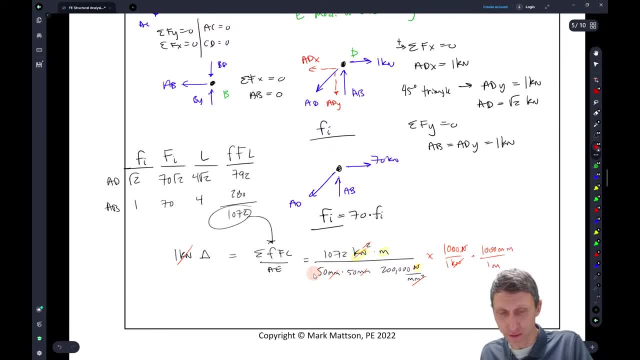 1000 millimeters per kilonewtons, And then what else do I have? I have 1000 millimeters per one meter. okay, so is this a long problem? yeah, it is. it's a long problem, but it hits on some fundamental principles, right? the fundamental principles are like units. do you know units? 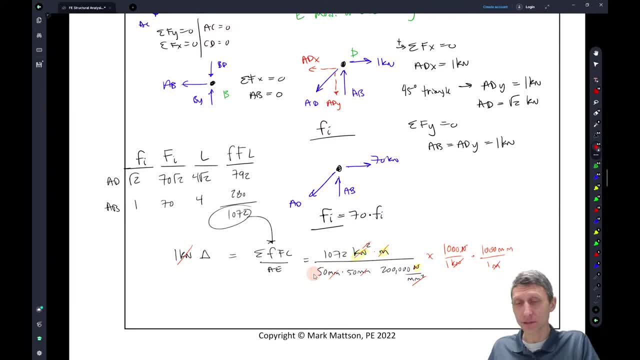 do you know how to apply some of these more complicated methods- instructional analysis- and can you put them into your calculator and take the basic trust analysis and apply something that's a little bit more complicated here? so if we type 1072 times a thousand squared, you know, divided by 50, divided by 50, divided by 200 000, i get 2.144 millimeters. so i get my delta. 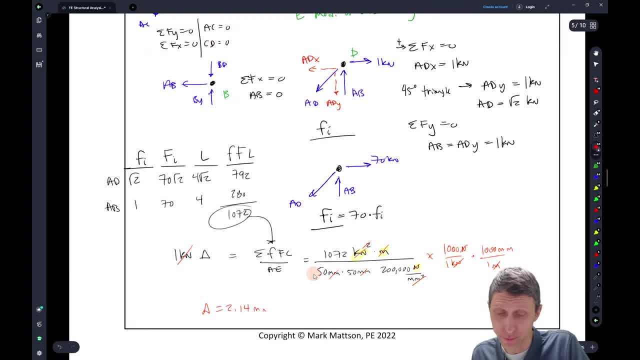 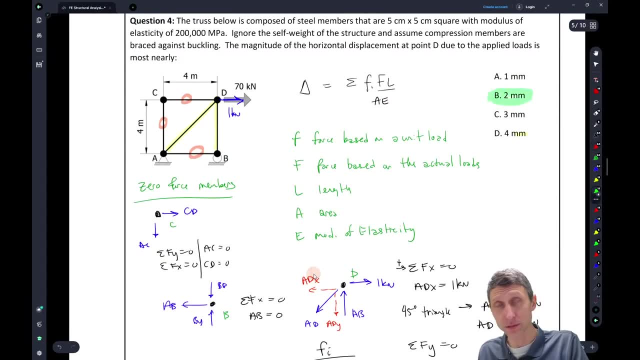 equal to 2.14 millimeters, which should match one of these up here. so, in theory, this matches our two millimeters. it's most closely related to that. okay, so is this problem going to be on there? i don't know, maybe, maybe not. you could i see a problem like this where, instead of having the load be, you know, horizontal? 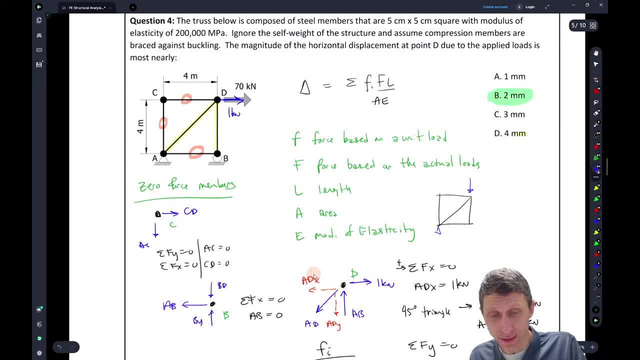 the load is maybe vertical. i could see that. why. why is that that? that question's even easier because when you look at this question, this goes to zero, this is zero, this is zero. they're all zero force members except for one member here. and then this just simplifies to what it simplifies to like. 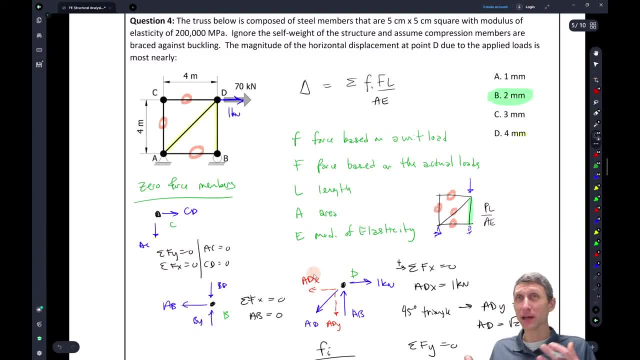 a pl over ae problem. so like column right, and then this just simplifies to like a p l over ae. i mean it's that's where it's like it could get. it could get simpler right, and this isn't the problem we have. you know, this isn't the problem that that um we were given. you know that in this problem, 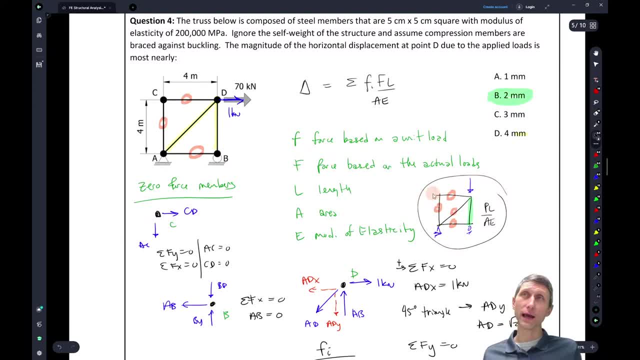 statement. but is it something that if he could give you, sure, why not? it's that same idea of like: i'm going to give you something that looks really complicated, but once everything goes to zero it makes it a little bit less complicated, a little bit more doable in that five minutes. but if you 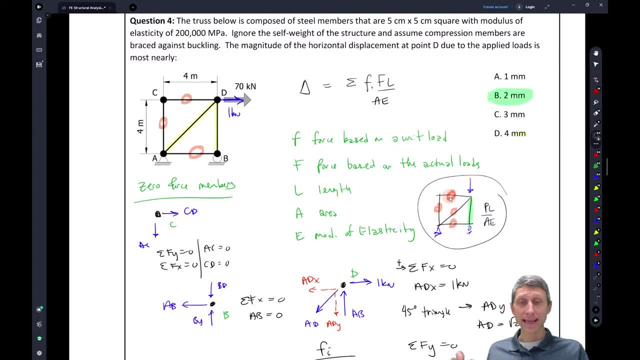 understand the fundamentals of that trust analysis of zero force members. this that's going to help you a ton. oh man, that was. that was, um, quite the problem, you know. but let's just, let's keep going. if you have questions, let me know, but hopefully this is helpful as well, just remembering zero. 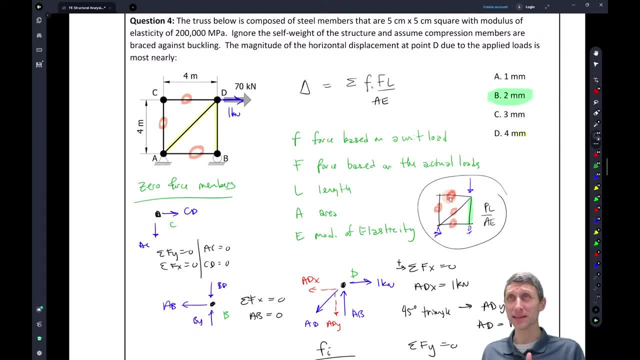 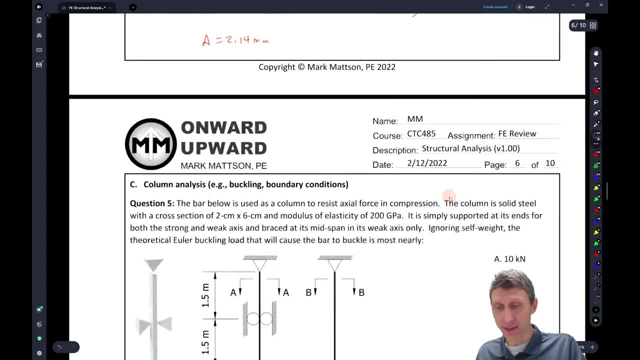 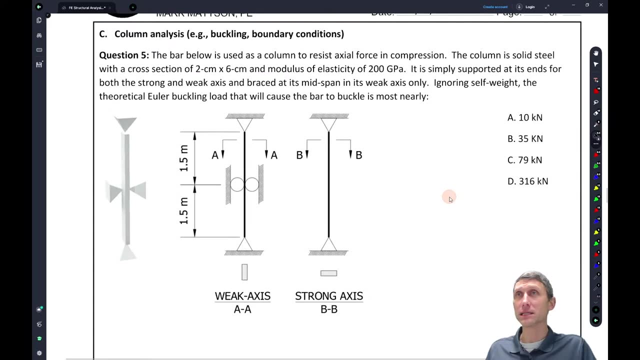 force members remember that, like you know, principle of virtual work kind of thing, the, the unit load, uh, type of thing. so let's keep moving. so we are on to question five, and this goes into column analysis: buckling boundary conditions, um, probably when we get into steel. 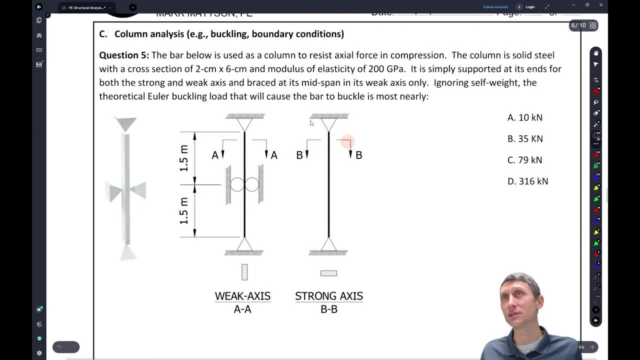 analysis. we'll get more into columns as well, but this one kind of just shows, shows up and says we have a bar. it's used as a column to resist axial forces and compression. uh, the column is solid steel, so we get that um, you know. e thinking in the back of our head what's e? um for centimeters. 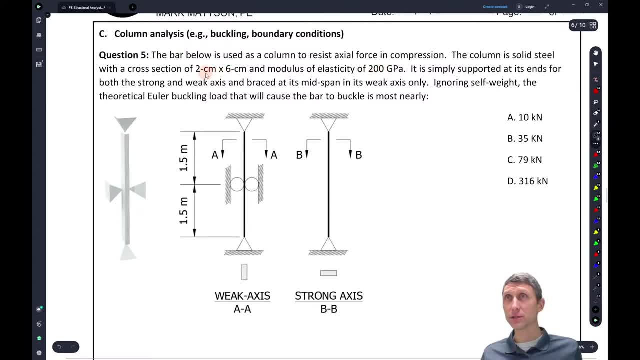 it's going to be that 200. okay, they give it to us. this is a cross section of two centimeters by six centimeters and modulus elasticity 200. it's simply supported at its end for both the strong and weak axis. so we have simple support at its end for both the strong and weak axis. so we have simple support. 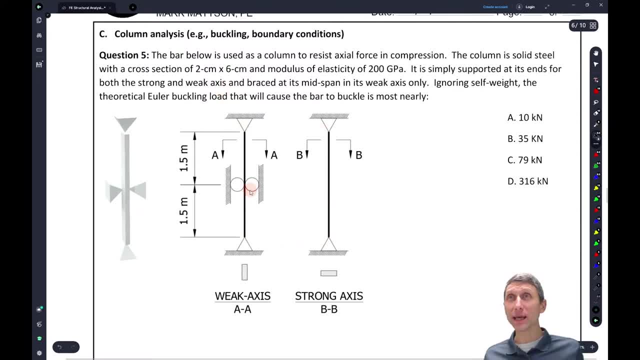 at both ends, okay, and then in the weak axis it's braced at the midpoint as well, okay, only in the weak axis and not in the strong axis, okay, so what's the theoretical euler buckling load that will cause the bar to buckle, okay? so this is where you kind of need to know what those 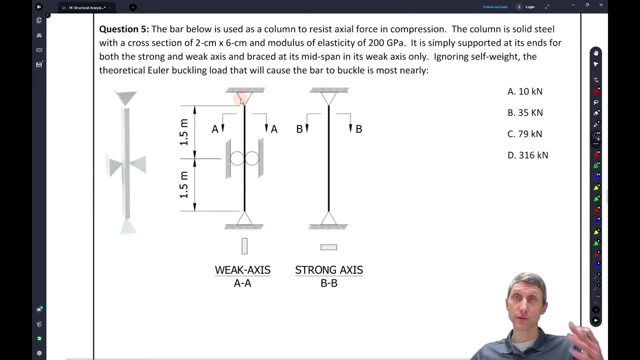 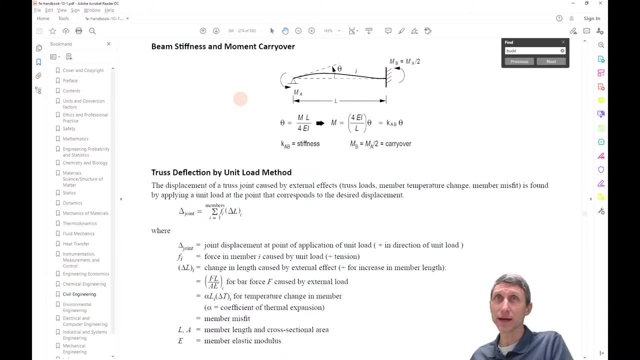 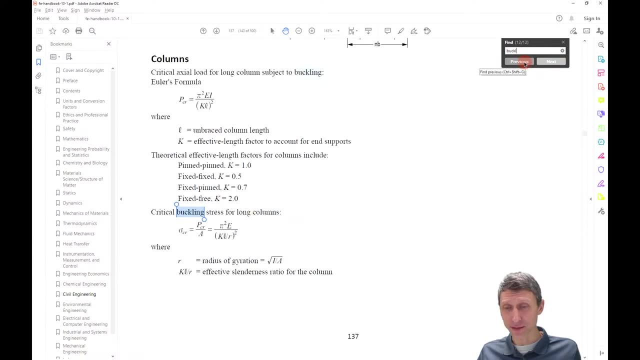 uh, those, those, those formulas are right. so if we come back- and this is where this is a great one for the- for uh control f, so if i just start to type in buckle, there's lateral torsional buckling. uh, and honestly i'm going to go to previous and look here. so, so if we have columns, uh, if you kind of know how this 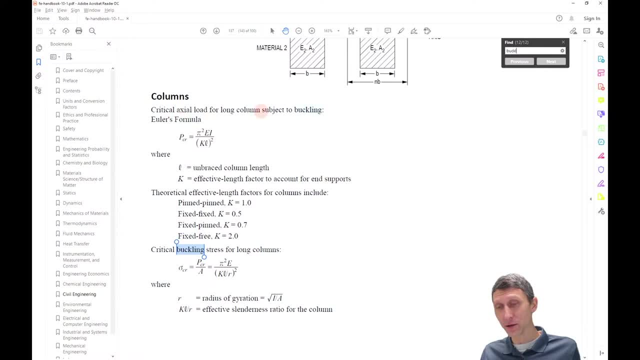 this works. we have columns. we get a critical axial load for long column subject to buckling. euler's formula: is p critical. pi squared ei over kl squared. the other thing i'll throw out here is: if you get pi squared ei or, i'm sorry, pi squared, e over kl over r, squared sometimes that kl over r. 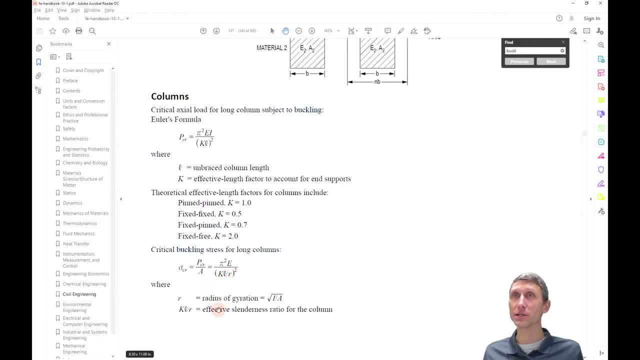 is also known as a square, and if you get a square e over r squared, you get a square e over r squared slenderness ratio. you have to know r is. r is the radius of gyration. it's just the square root of i over a. so that might be asked as well. like it's radius of gyration, you might be given a critical. 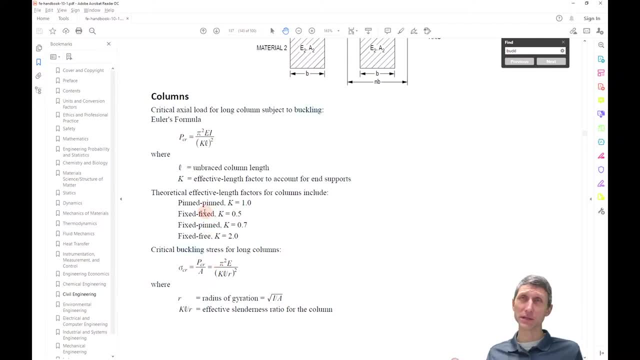 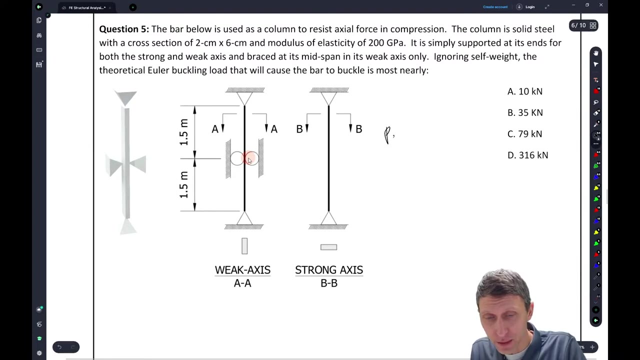 buckling stress instead of a critical buckling load. you kind of have to use one equation or the other. but let's go here and we will take a look at that. so we got pcr: is pi squared, ei over kl squared? okay, so we'll come back here and we get- i'm just gonna write that down- pcr equals. 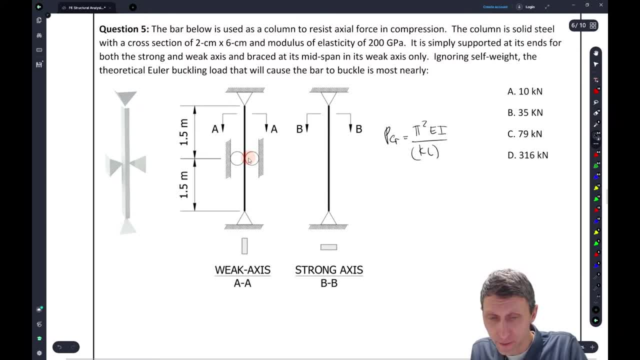 e i over kl squared and the nice thing for you is when you're taking the fe you're gonna have the handbook on one side. you're gonna have your work kind of in front of you on your little you know tablet thing that you get to write on, and then you'll have your problems on the other side. that 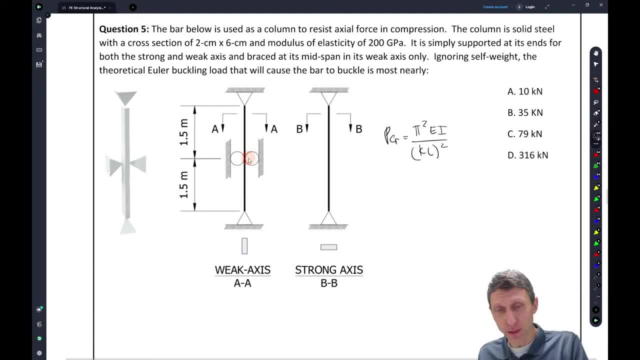 you get to work through as well. so this is our pcr. so so we we already we're given e, right, so we're given, uh, we're given e. so e we know is 200 gpa. uh, we don't know k we have to go look up k we. 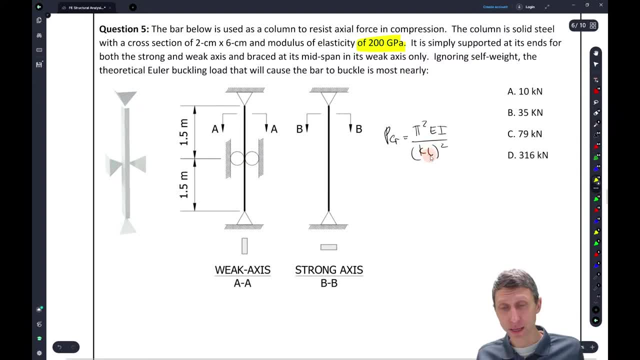 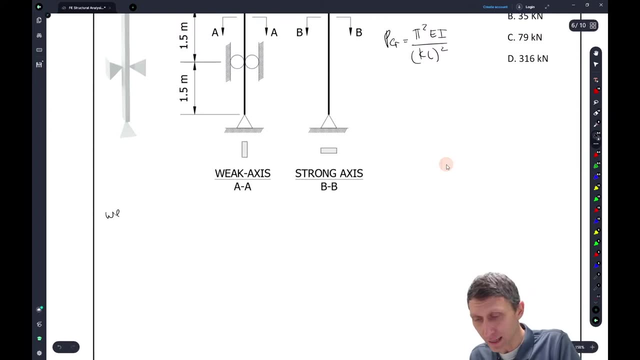 have these l values here, uh, that we can use, and specifically, l is going to change depending on which axis you're at. so if we're looking at, like the weak axis, uh, let me, uh, let's, let's, let's just draw it down here, why not? so if we're looking at the weak axis, right, we know that the, the unbraced, 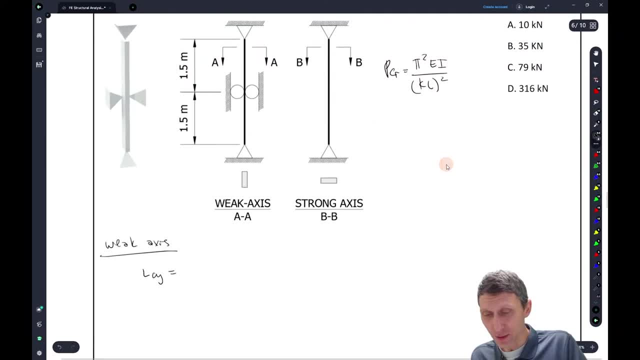 length is lcy, the unbraced length. you can call it lcy. you can call it ly- it's probably ly is a better term for it- but ly, the unbraced length, is lcy. the unbraced length is lcy, the unbraced length. 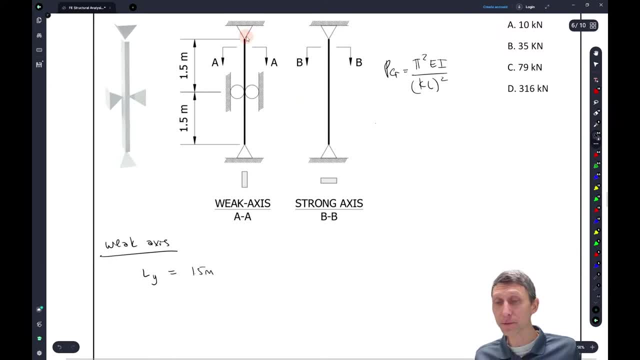 is going to be 1.5 meters, right. the length between bracing points is just that, 1.5 meters. similarly, uh, lx. right, so we have lx. i'm sorry, actually, let me come over to, let me, let me come back here for a second and i'm just going to do this. strong axis on this side. 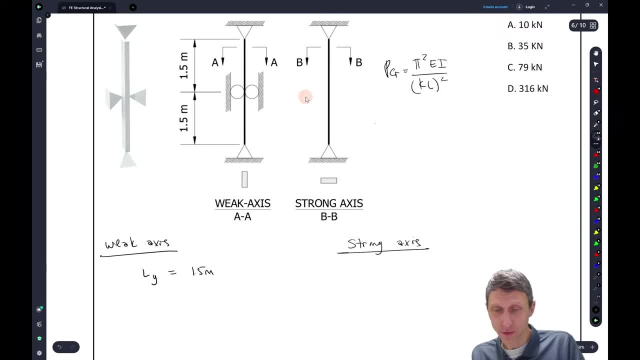 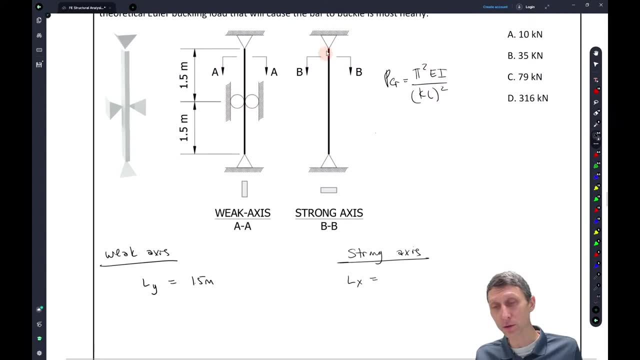 okay, so, similarly, over here, the strong axis, we have lx, and this is where we get that total length. we get the total length, which is three meters, because it's it's it's braced at three meters. okay, we need to think about ky and kx, right, and this is where, hopefully, you kind of remember what that is. but 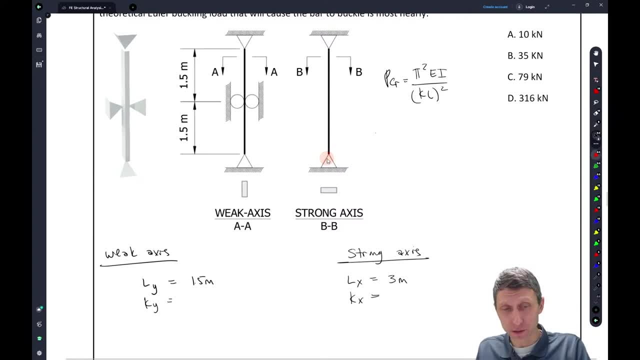 this is kind of that uh, effective length factor. so if we're looking at how these things are going to buckle, we're going to have this buckling and kind of a bow shape, right. so we're going to have a bow shape here. but but for the weak axis, we're going to bow, but it's going to, it's going to come. 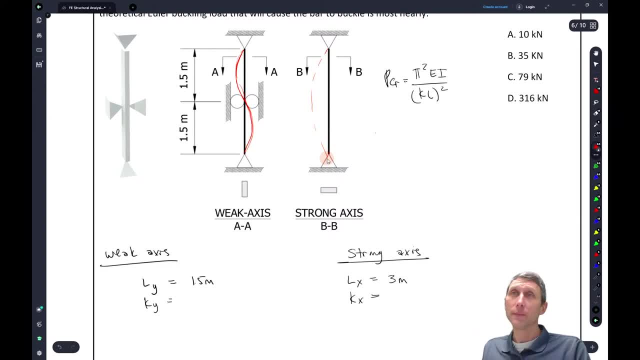 back on itself here. so it's going to go through, uh, that bracing point. so for the the strong axis, there is no extra bracing point. it's just going to be braced right at both of the pins, right. so? but for the weak axis, it's going to be braced at these, these three points here. so we have to look. 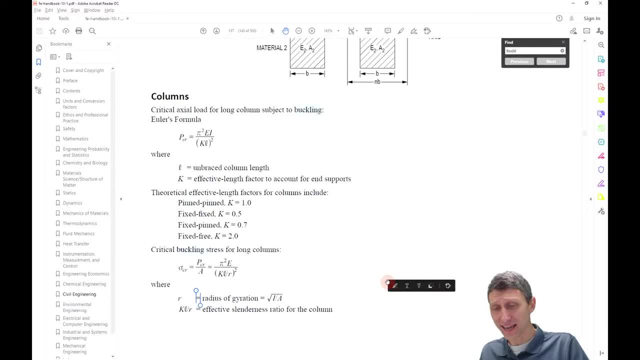 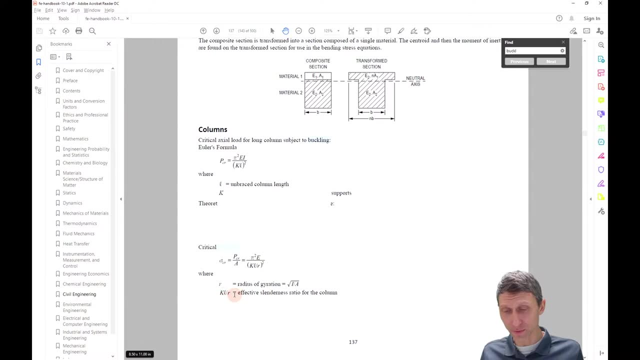 up the effective length factors and if we come back to our reference handbook, let's see if we have them, let's see if we, if we can find them here. so, um, you know, if we look at this, we have k, which, uh, you, my computer is not liking me today, so let's, let's uh see if i can fix that. uh, or maybe it's. 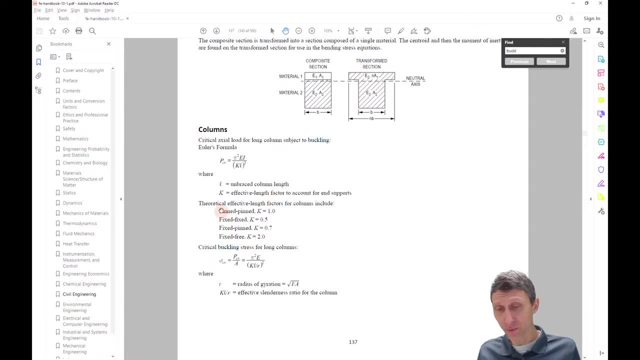 just okay, i don't know the k. what we have here is the theoretical effective length factors. pin pin is going to be k equal to one, fixed pin, 0.5, or fixed, fixed, fixed, 6.5, fixed pin, you know 0.7, two. but effectively what we have here is we have pinned, pinned. 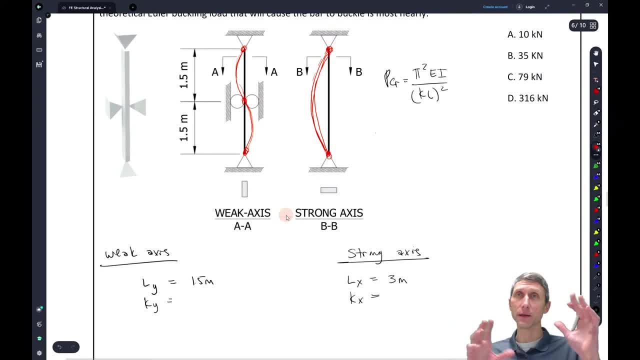 for both of them, right. so if, if, if we think of a pin, what's a pin? pin allows free rotation. it allows free rotation. so if it at this point- and at this point we have free rotation. so we're going to say k equal to uh, 1.0, uh. similarly, over here we have free rotation at both ends. 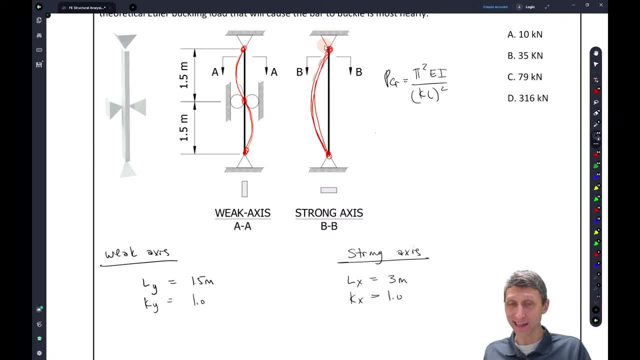 and kx is going to be 1.0. so we got the k, we got the l. we know that e already. we said e was well, e was 200, uh gpa, which is equal to two hundred thousand mega pascals. okay, however, whatever units you like. and and then, what else do we need? we need i, so let's come to. 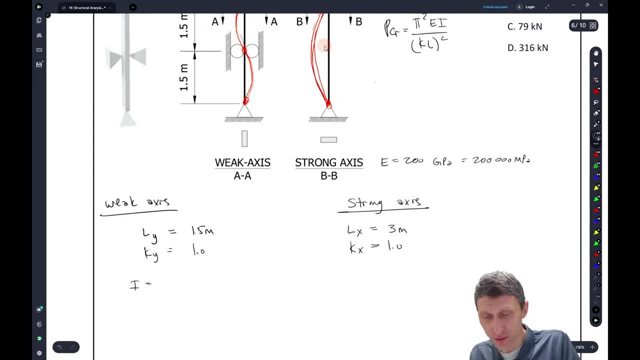 the strong axis and weak axis, i equals. you know i y. this goes back to that question that came up kind of earlier: what's strong axis, what's weak axis? well, as strong as the one where essentially get the bigger h value right. so it's like it depends on how you're going to buckle this thing. 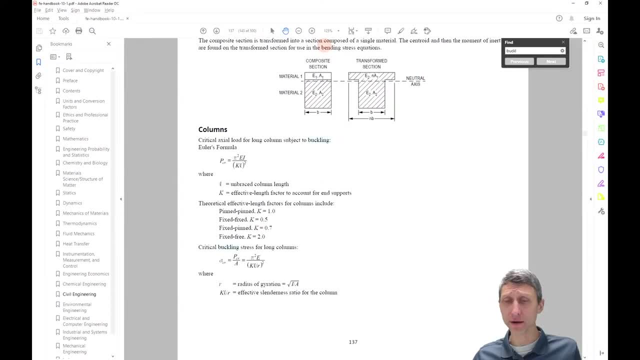 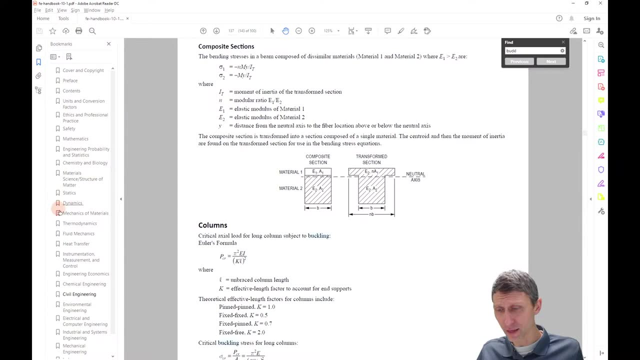 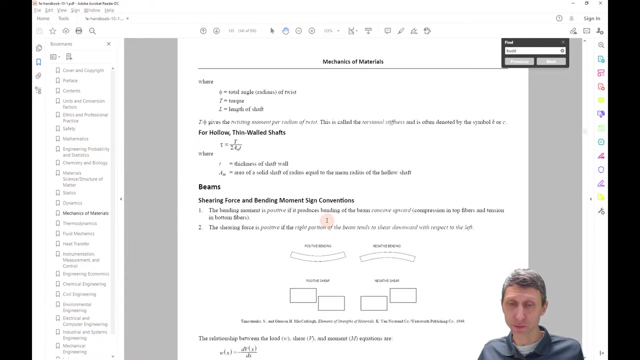 but the bigger h value. so if we come back to our our mechanics and materials section in here- or well, actually this is civil engineering now- but if we come back to our mechanics and materials section, we have some values here for- uh, for moment of inertia and we kind of went over. 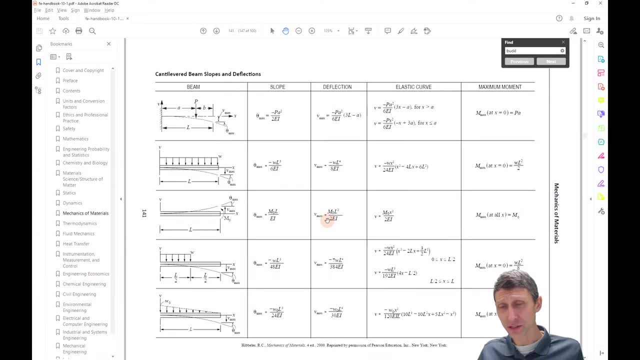 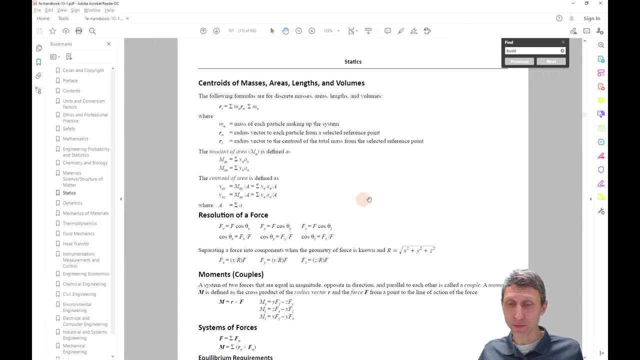 this in the mechanics material section, but it's worth doing again because it shows up, uh, when we get to. actually it's in the static section. oh man, i missed that one. this, this is in static section. moment inertia is in the static centroid's, uh, centroids: masses, areas, lengths and volumes. 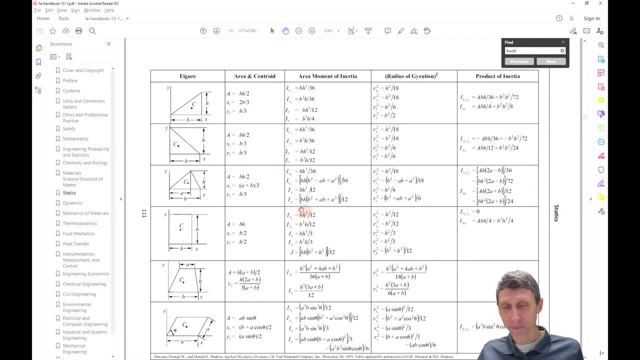 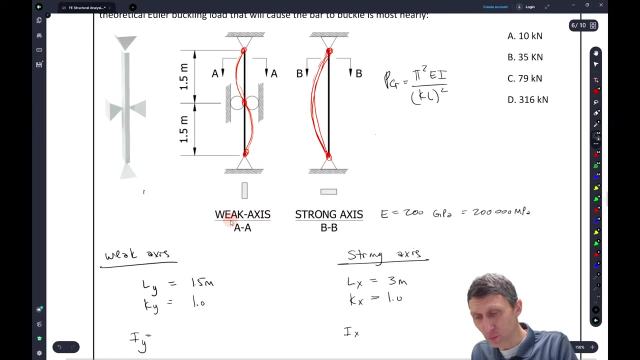 right, this is where we have a standard value here and we have: i x is base times height cubed, so the big height here versus i y is the base cubed times the height. okay, so in other words, when we come back here, we're going to see the general rectangle formula. 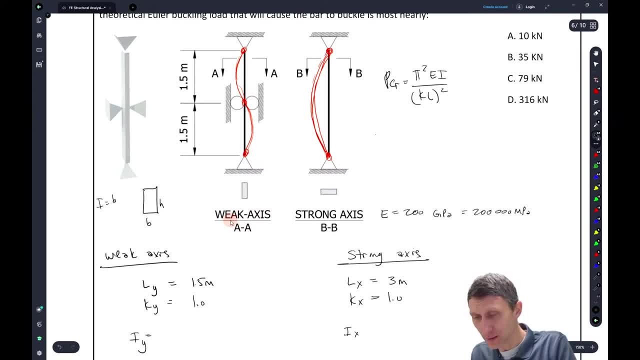 here is base height. i equals base height cubed over 12.. so when we go to the weak axis, we want the smaller moment of inertia. so what's this going to be? it's going to be 6 times 2 cubed over 12.. and honestly, i'm gonna, i'm just gonna make the commitment now. i'm just gonna make the commitment. 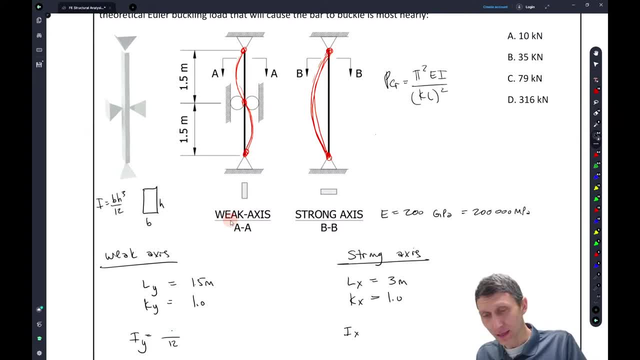 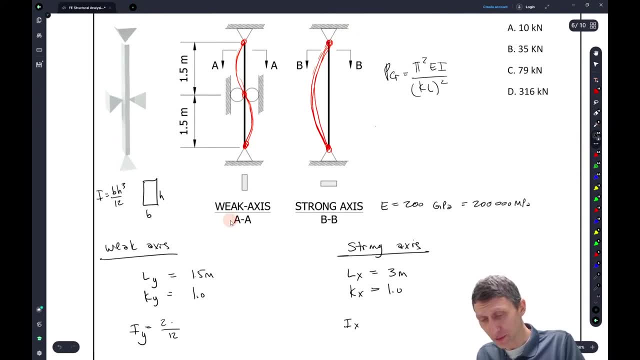 and i'm gonna say, rather than do that, i'm gonna say: if this is, what do i have? i have two centimeters by six centimeters. i'm gonna say: um, i'm sorry. i'm gonna say, i'm gonna just convert everything to millimeters. i i just i'm gonna say 60 millimeters times 20 millimeters cubed and that's. 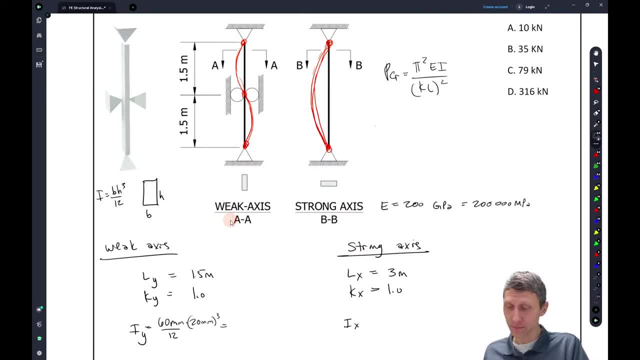 gonna give me this value here, right? so 60 times 20 to the three, uh, over 12, uh, what do i get? i get about 40 000, and so 40 000 millimeters to the fourth. okay, and then we can do the same thing. 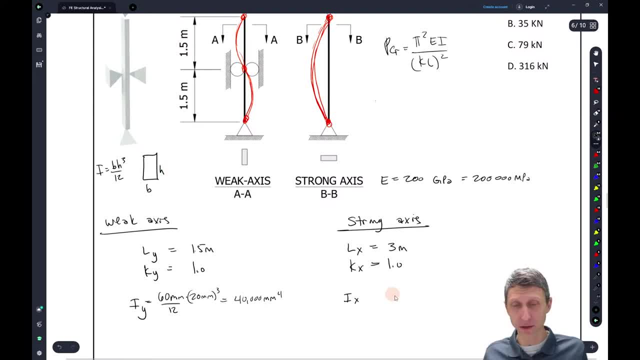 for the strong axis, but for the strong axis, the h is going to be the one that makes it bigger. so what i'm going to do here, i'm going to say this: equals to 20 millimeters times 60 millimeters, cubed all over 12, and that's going to be a bigger number because the 60 gets cubed, not the 20, right? 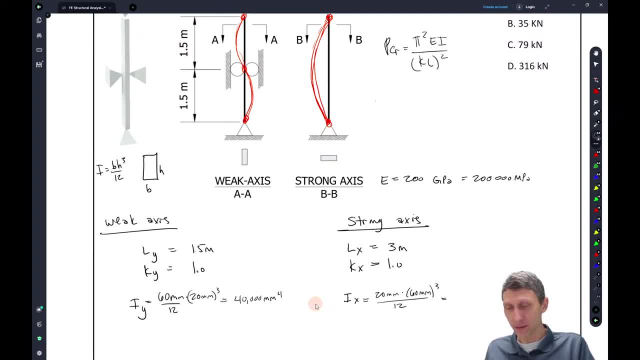 so, uh, so what i'm going to find here? i'm going to go to 60 and i'm going to get 360 000 millimeters to the fourth. okay, so that gives us. that gives us some things, and then all we have to do really is: 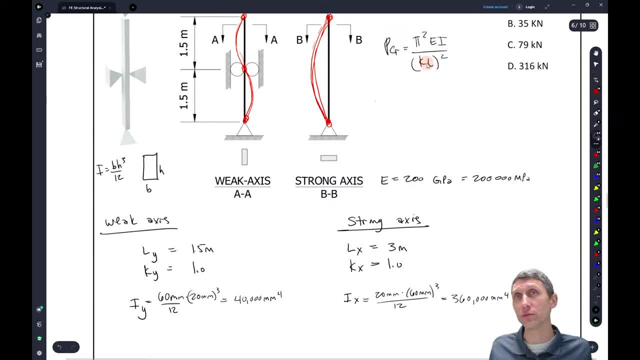 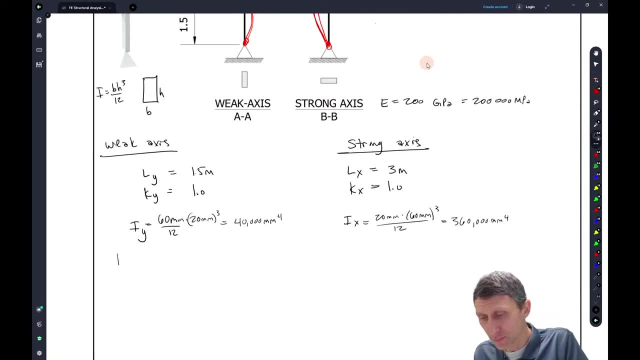 is, we have all our values. we just need to get the right units and and use or apply our equation right. so we're going to get pcr y and pcr x. i'm just going to make a little bit of room here and i'm going to say: well, pcr y, the critical. 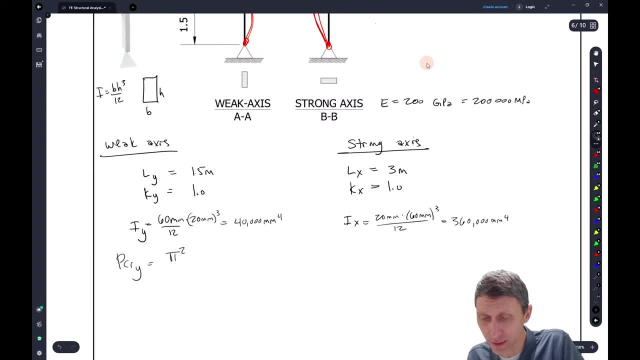 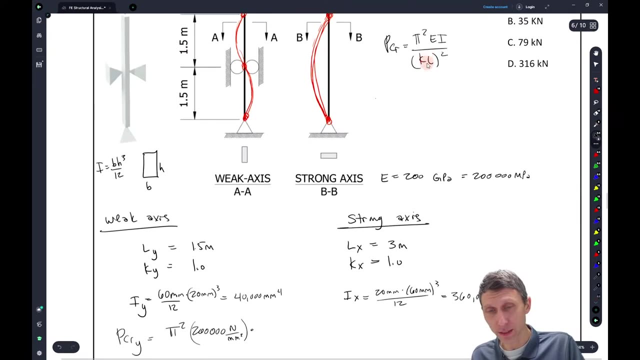 buckling load for y is going to be pi squared e, which is going to be 200 000- i'm just going to do the mega pascals or newtons per uh millimeter meters squared times. what was it? there's pi squared e i over kl squared so times um i, which is forty uh thousand. 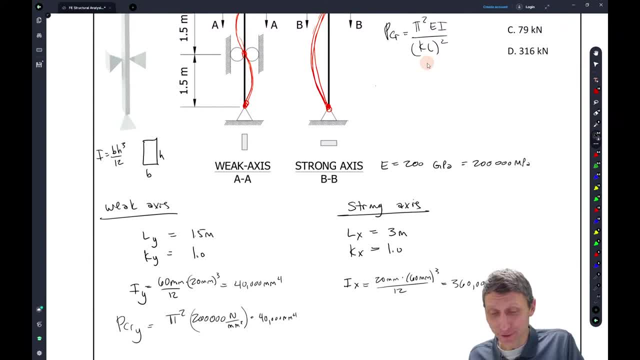 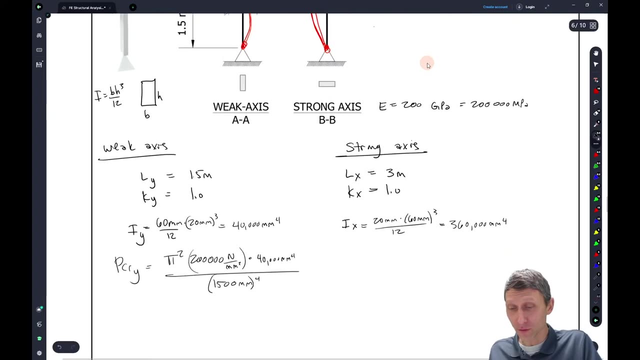 millimeters to the fourth, okay, and then we're going to divide that by kl squared, so we're gonna have 1.5 or 1500 millimeters to the fourth. i'm doing a conversion on the fly there, but uh, 1500 millimeters to the fourth, okay. so what do we get? well, let's plug it in, because i don't remember. 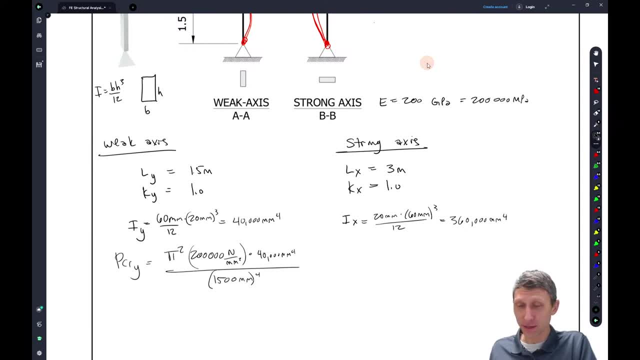 it's a pi squared uh times 20. no, not 20 200 000. i squared times 200, 000 times 40 thousand, so big numbers. but it's either really big numbers or really small numbers of the meters. i like the big numbers but some people like them smaller, i don't know. so what do i get? i get like um. 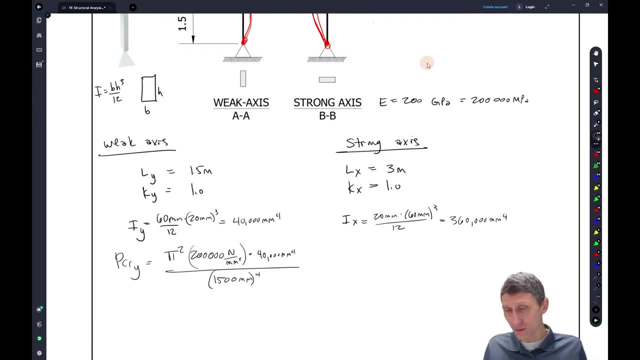 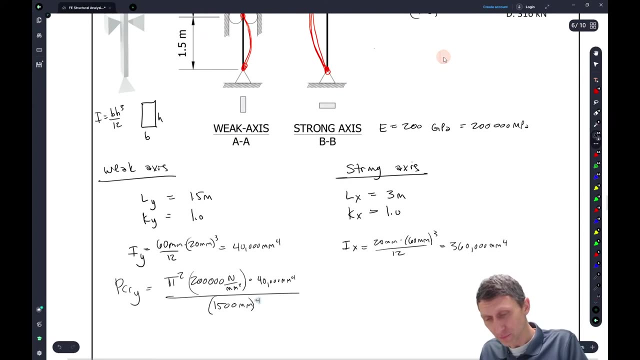 something that doesn't make sense. so what did i do wrong? uh oh, um, i don't know. i probably did something wrong. oh, i'm sorry, it's not. 1500 to the fourth. it's over kl squared. there it is, it's a kl squared. i was getting too many fourths going on in here, that's. 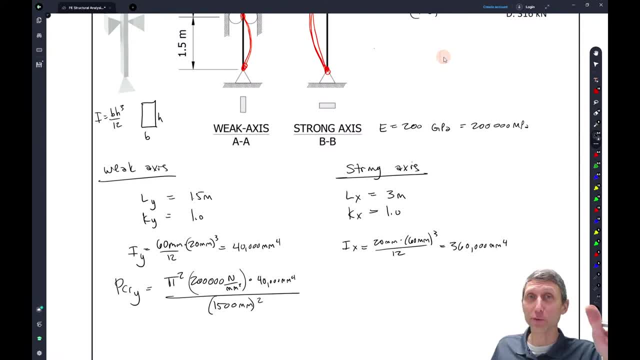 um, it also helps on the fe, when you write down a formula, to actually use that formula. just saying it's gonna help. so the nice thing with your calculator is, if you get a weird number you can just go back to second enter and and sort of change it around here, and you know, and then i get. 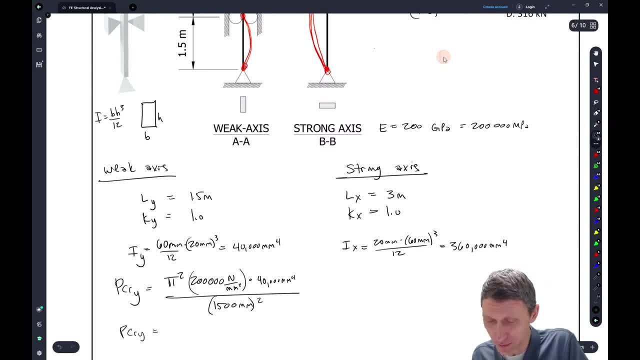 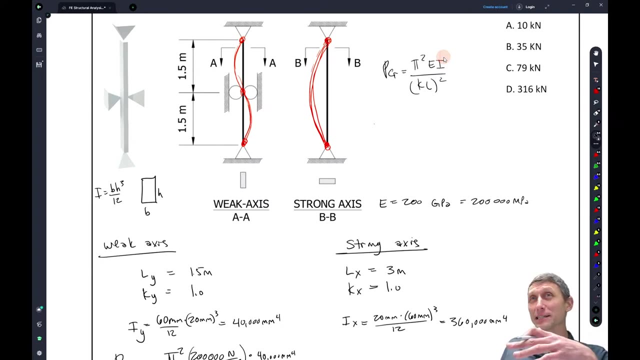 the 35 000. that makes more sense. so pcr y equals about 35. you know, 100 newtons, 35, 100 newton. okay, so we could just stop and say, great, we got 35. but what if? what if the strong axis? because it's got that longer. 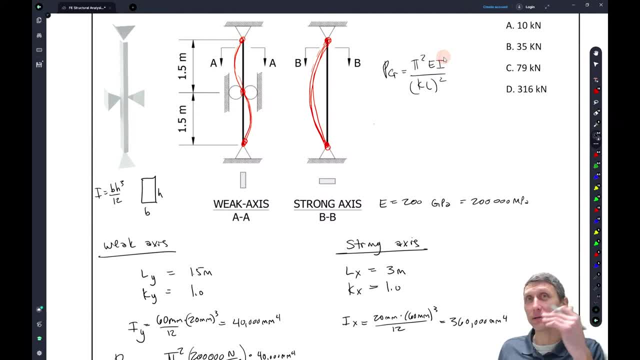 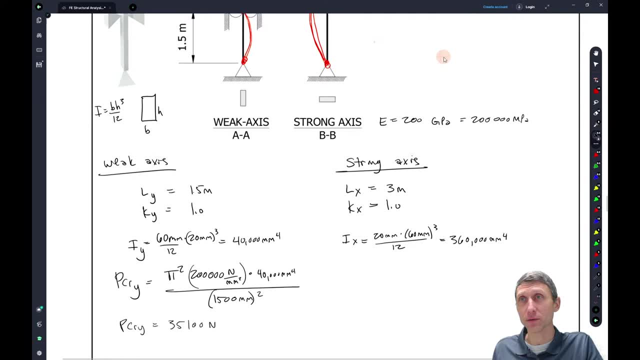 three meter length. what if the strong axis actually buckles in 10 kilonewtons? then we'd feel really sad because we'd get the problem wrong. so let's go and get that, let's just- i mean, it doesn't take that much longer to do this- right- let's do pcrx and just confirm that that's. 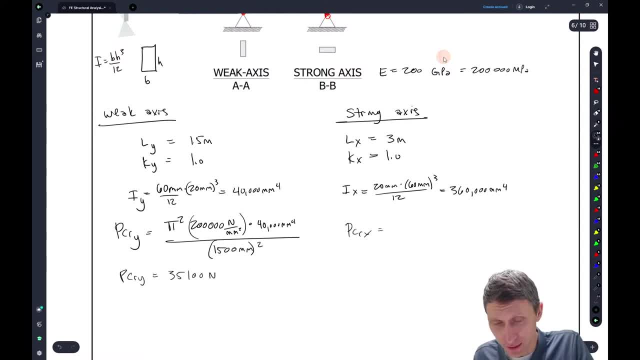 not the 10, you know, 10 kilonewtons, and uh, be on our way. so pi squared times 200 thousand newtons per millimeter squared times 360, a thousand millimeters to the fourth, divided by that kl squared- and we'll get it right this time- so 3000 millimeters squared. so pcrx, is this going to be? 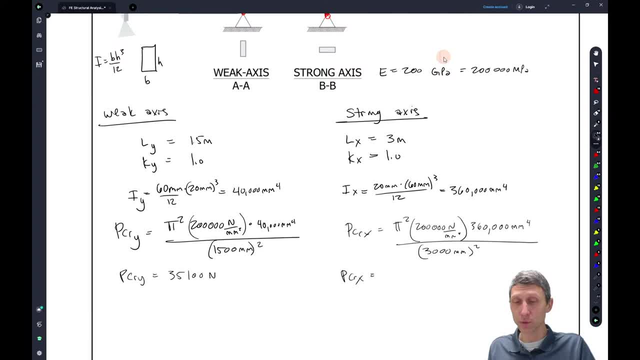 smaller than pcr y? if it is, it'll buckle that way. which which one is it so? um, the nice thing is with your calculator you can do is you can just go back to the previous one that you just did in and modify them, or you can just plug it in all again. i mean, it's it's up to you how you like to. 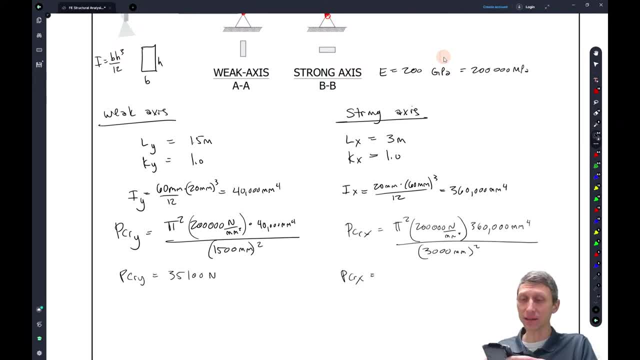 use your, your calculator. but this is where it's like it's helpful to get a calculator that you like and do what i call calculator practice. just plug these things in and see if you can get the same, the same values, because what i get here is is roughly 79 000 newtons. okay, inconceivably. you. 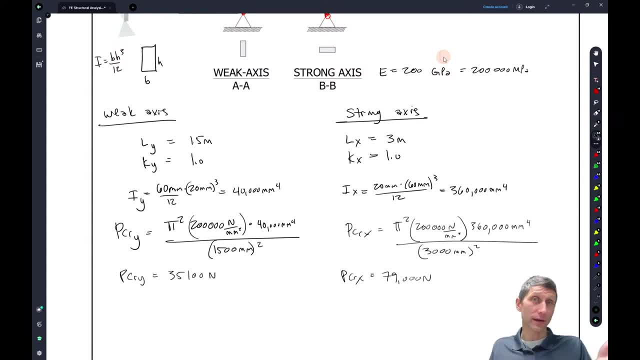 could have a problem where you have, you know, more weak axis bracing and the strong axis actually controls, or you can have something where maybe the x and the y are close and the strong axis controls as well. so it's not going to be a given that the the weak axis 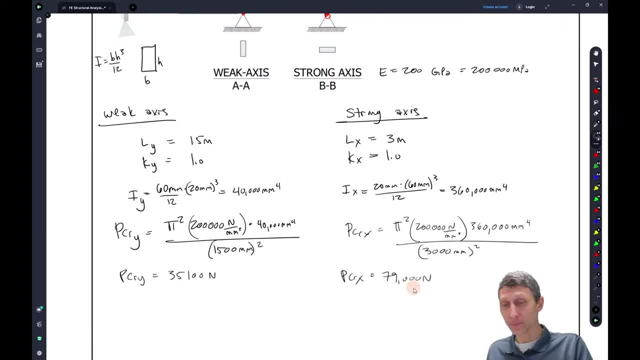 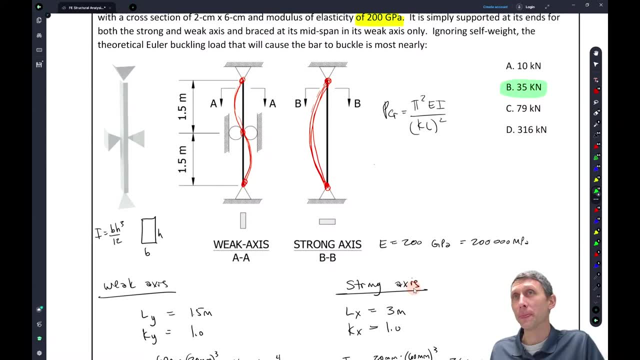 controls most of the time. that's what it's going to be, i but, but for here you know the, the value of 35 000 newtons or 35 kilonewtons is what's going to happen, okay, so i mean, if you have a smaller h. 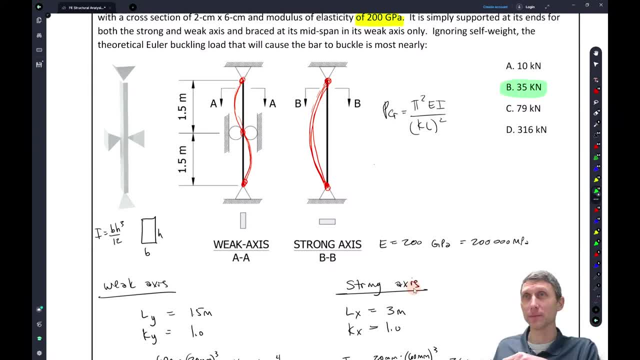 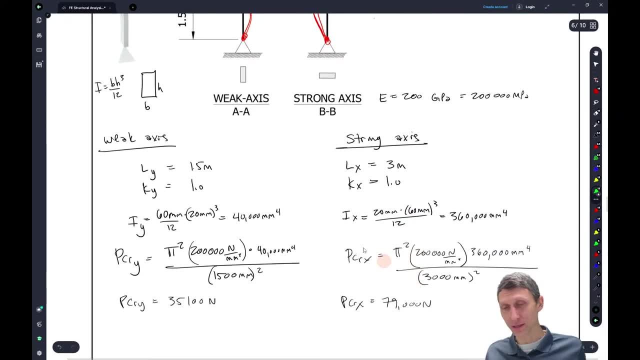 maybe the strong axis would control. it's just it depends, you know, on the, on the values that you're given. but this is where understanding kind of this value, understanding some of these values, is going to be helpful. so you got all you got to get rid of these values, like you know, you gotta. 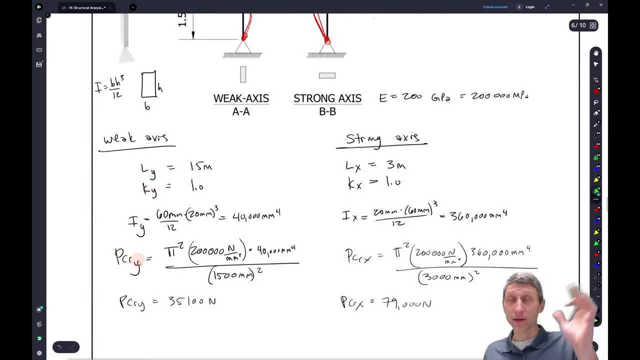 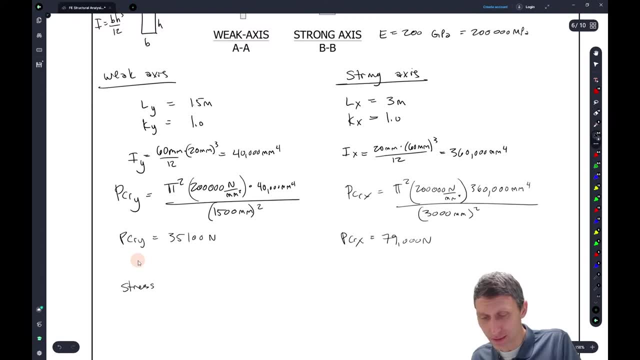 k, you got the i, you got pcr, and then again, just just to throw this one out there, because this, this can show up too if you get the buckling stress. so stress, um, stress, is dependent on kl over r, which is your slenderness ratio, and you just have to remember what's our r equals the. 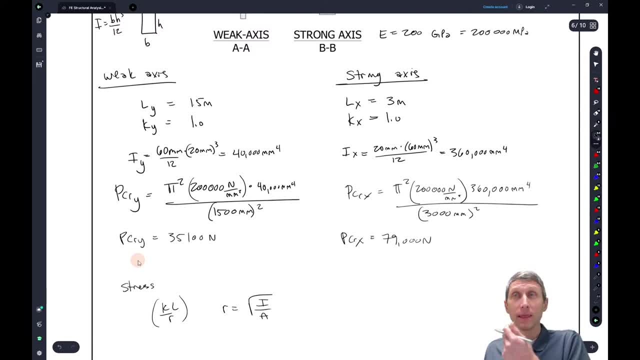 square root of i over a. that's the radius of gyration, and it i mean for for, like the weak axis, for example, what would this be? it just be, oh, we'd have. we'd have 40 000 millimeters to the fourth, divided by its area. of what? 60 millimeters times 20 millimeters? and take the square root of 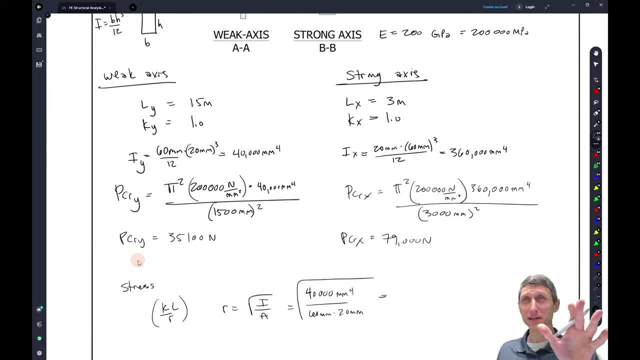 all that. and you might be saying, mattson, why are you doing that? because, um, didn't we just already solve this problem? yeah, this is just extra. this is just like extra, this is like a bonus and the reason. you know the extra, and i'm just gonna say, you know, needed, uh, for 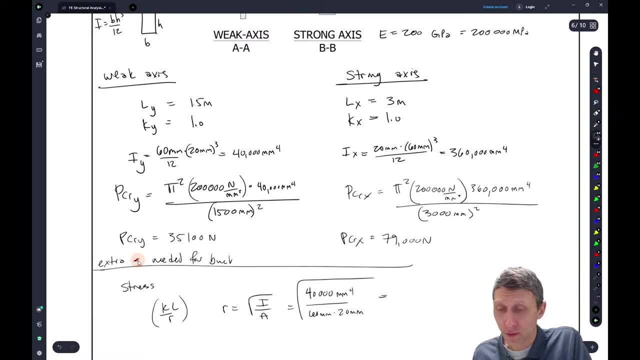 you buckling stress, right. and the other reason it might be needed is because i was talking to somebody. they're like, yeah, they asked for radius of gyration, man, they so. so what's radius of gyration? it's the square to i over a, okay. so the question is, why did i pick the? uh, um, why did i pick the, the, the weak? 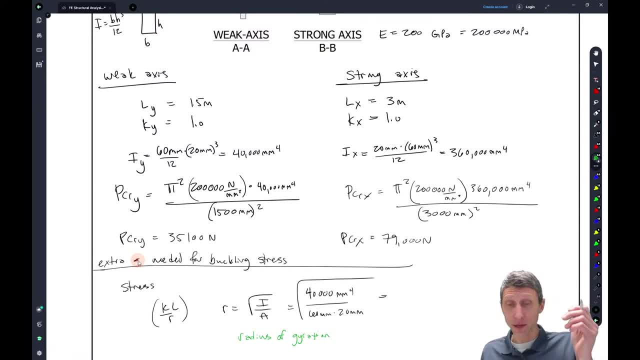 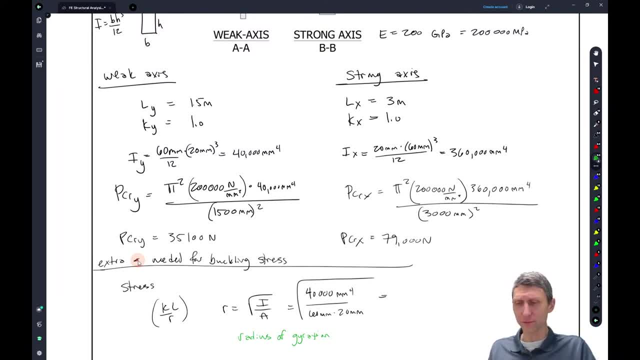 the original value of a radius in: thank Block東西. so that's LEED is theck. get there. i'm just going to do this math out real quick. so if i do the square root of 40, 000 divided by 60 divided by 20, i'm gonna value of like a radius duration of like 5.77 inches. okay, so, 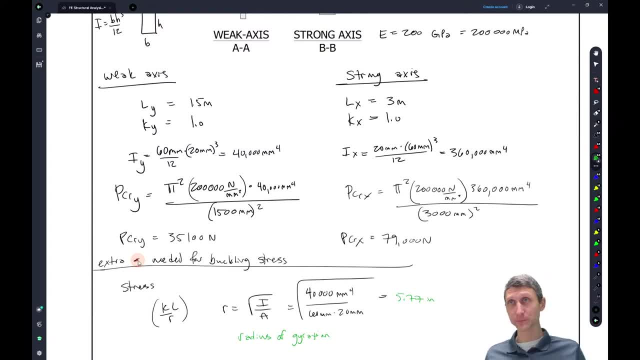 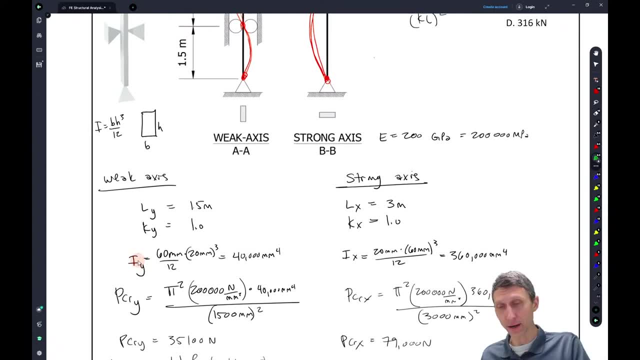 that's just a little tidbit. you you need that value if you're doing the buckling stress, so i just wanted to throw that one out there. so you have it. nothing you needed for this one. so why did i pick pcr y or pcr x? so let's just come back up here for a second and think about this. 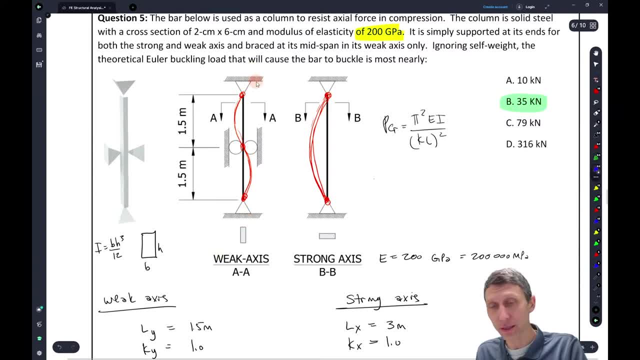 as you're loading this thing, this column gets one axial load. it gets one axial load, p. so the question is, when is it going to buckle? it's going to buckle when, i mean, if we're taking a look at papers, right, it's going to buckle like, do you see this? this is going to buckle. 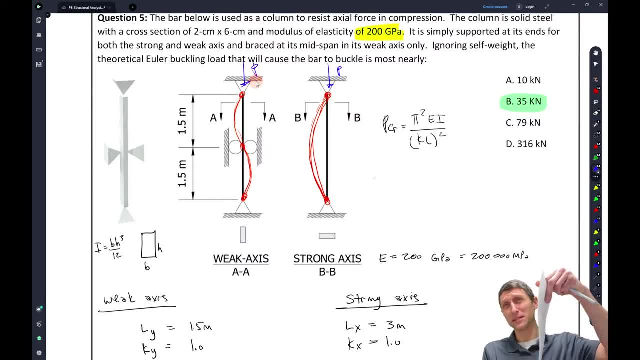 eventually. and it's never going to buckle in a strong axis with a piece of paper. it's just going to buckle in the weak axis, right. but if we brace in the middle, it's not a piece of paper so thin- it's still going to buckle in that weak axis. it's conceivable if you brace this one in. 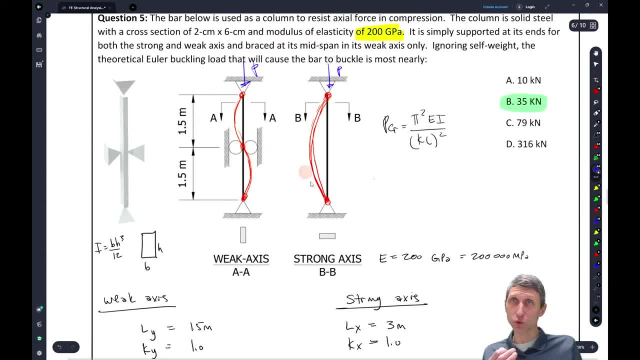 the weak axis. it's conceivable that this strong axis could buckle first. but if we think about it like this, we have one common load, p, that's being pushed down here. if the buckling load for you know, this side is 35 kilonewtons, the buckling load here is 79 kilonewtons. we're never going. 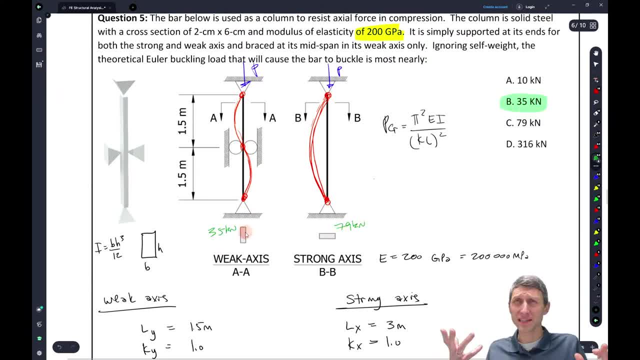 to make 70 kilonewtons because at 35 it's going to buckle. does that make sense to it? oh, it's already going to be buckled before you can even make it to the 79. so the 35 is going to control. but i hope that answers the question. uh, but you know, if not, definitely put some more things out. 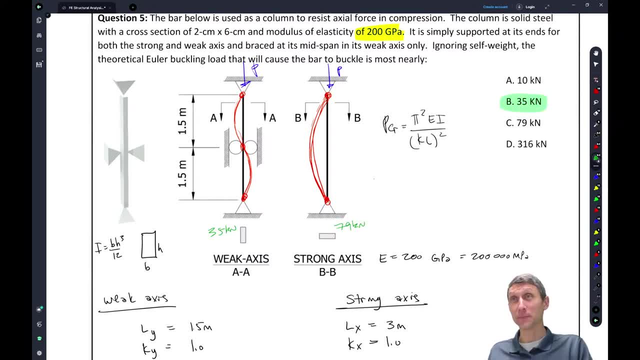 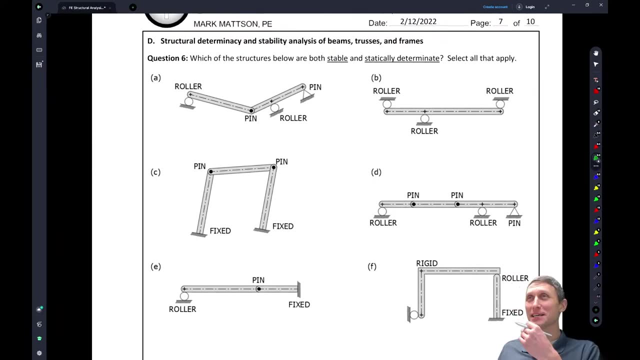 there. i'd love to try to answer, if i can. okay, the smallest load, perfect. yeah, i love that answer. smallest load, that will cause buckling, okay, awesome. oh man, let's go back to structural determinacy and we will just keep moving on here. structural determinacy, stability, analysis of beams, trusses, frames- i mean, we're on question six. we thought 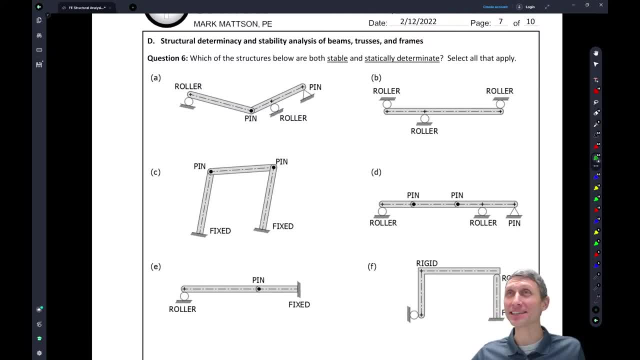 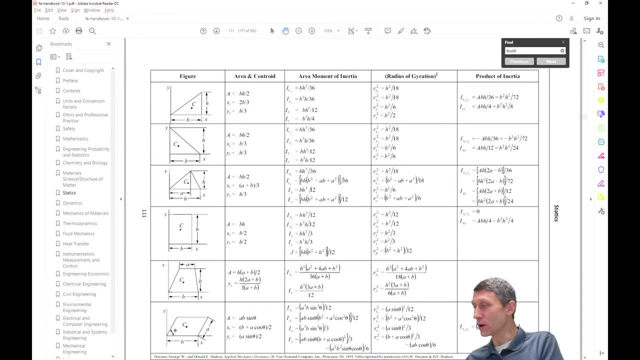 we were going to get done early. um, hopefully we can still get done early here. but let's look at this. maybe i'm just talking too much, doing too many extra things like radius of gyration, structural determinacy. so if i just search determinacy right, can i did i do the right word? 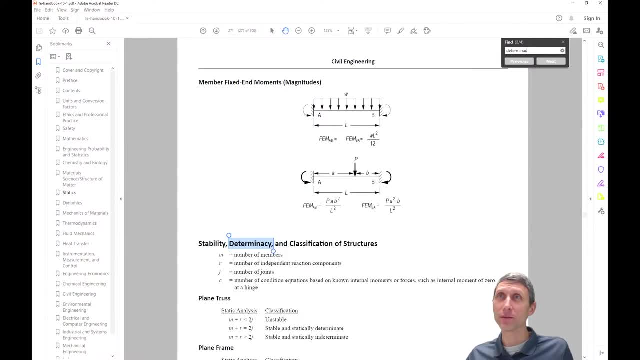 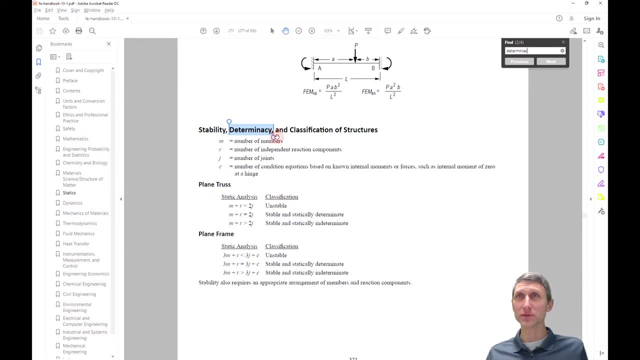 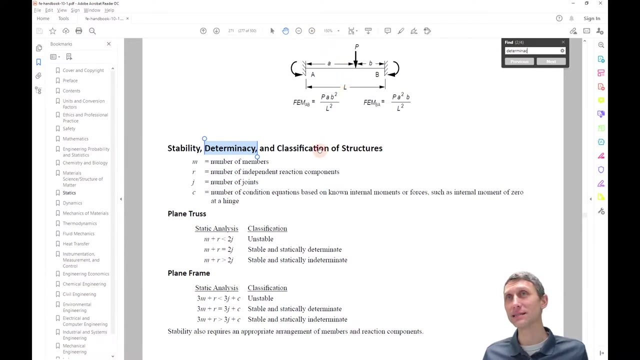 um, indeterminate, indeterminacy, uh, what else do i get- determinate classifications of structures. so this is interesting because i give you- you know, this is one of those things i sort of throw into my structural analysis class- just to kind of get the idea of what determinacy is it's. it's not something you necessarily always do when you're. 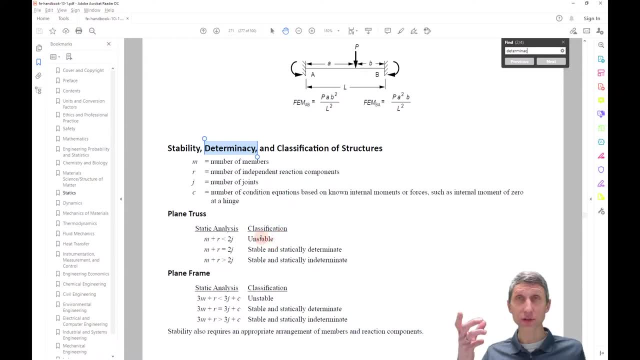 working in the real world. but it's one of those things that you have to understand: whether structure is stable, it's- i'm saying it's- unstable, it's stable and determinate. in other words, you can determine everything just by using the equations of equilibrium- or it's indeterminate. 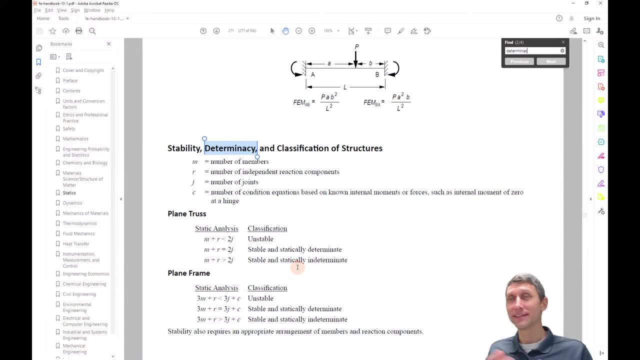 and you can see you throw up your hands. i can't determine it. get it um so? so i can't determine it in the sense that the equations of equilibrium aren't enough to determine everything. so we can do this with trusses, we can do it with frames, and what, normally, that i like to do here is is i- i sort of take this a. 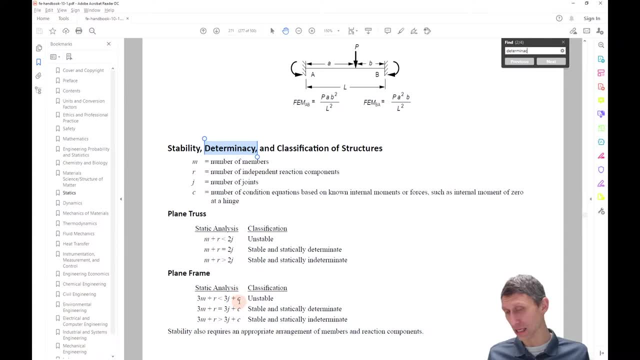 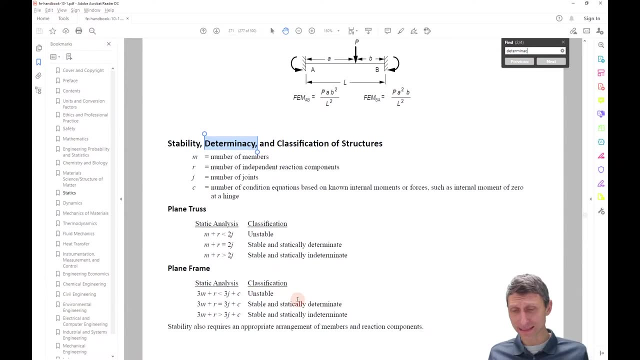 step back. i mean three times the number of joints plus c. all right, so 3m plus r? um, normally i think a little bit differently than that, uh. so, oh man, let's just take a look back over here. normally when i'm looking at structural determinacy, 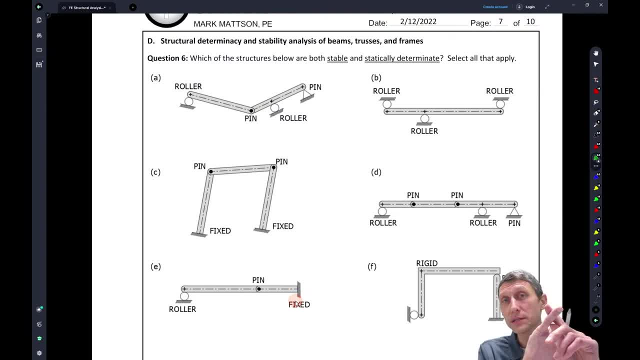 what i know is i have three equations of equilibrium: some forces x, some forces y and some moments for every beam. if i have three unknowns, i can solve that beam just using those three equations. if i don't have those beams, it's an indeterminate structure and it's gonna be. 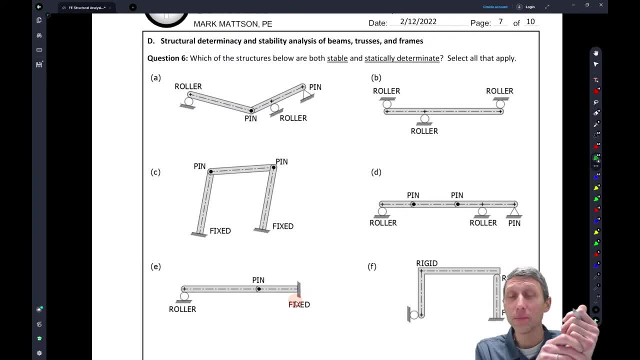 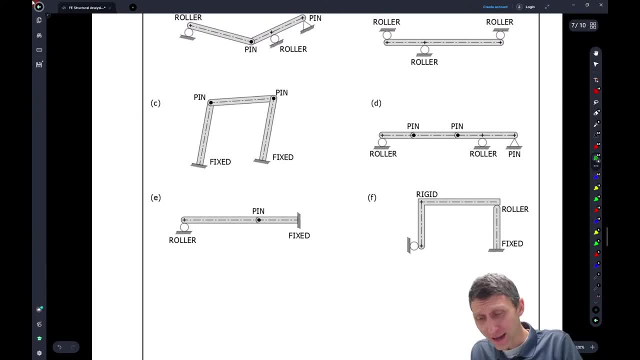 harder, you're gonna have to use some other method. okay, but what i like to think of is is, specifically here i'll just write out the notes again here for a second. but if if i have, basically what i'm going to do is i'm going to count the number of beams. so i'm going to say 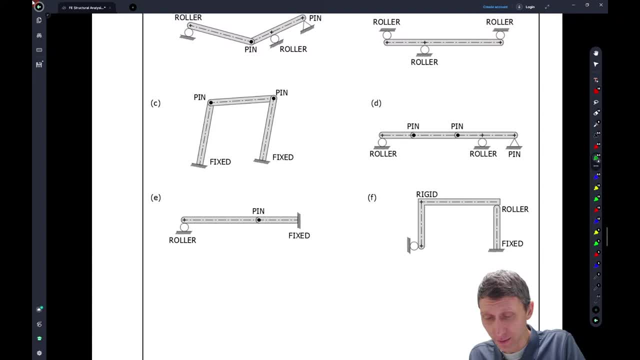 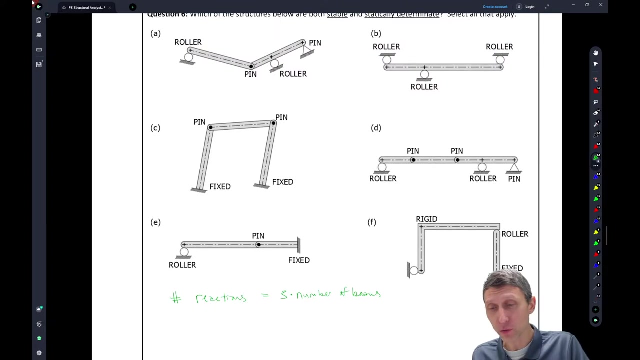 uh, you know i'm going to look at the reactions. so if i, if i, if i look at the number of reactions and if that is equal to three times the number of beams, it's going to be statically determinate as long as it's stable. so this question says which of the 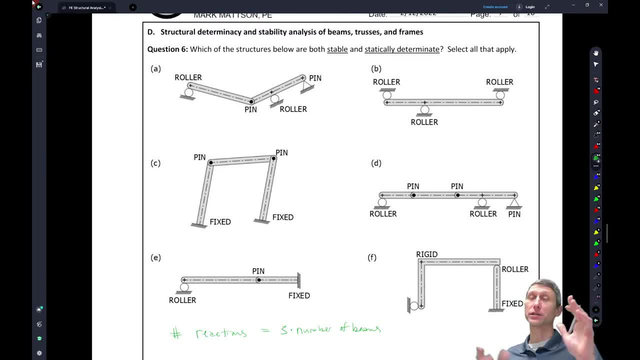 are both static, stable and statically determined. this might be one of those alternative types of questions where you just have to click. and you have to click which ones do i click? there's six of them, i can't just pick a and this is. this is one of those annoying ones where it's like you. 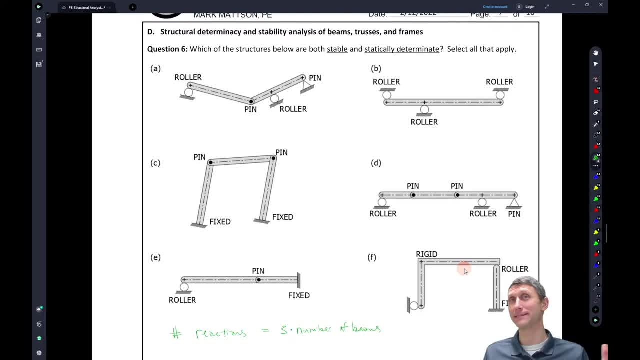 don't know, and you can't just pick b, because b is the answer that i like to use the most. i don't know. you know it's like you can't pick c. c's the, the, the, uh, the, the, the common answer. i don't know. 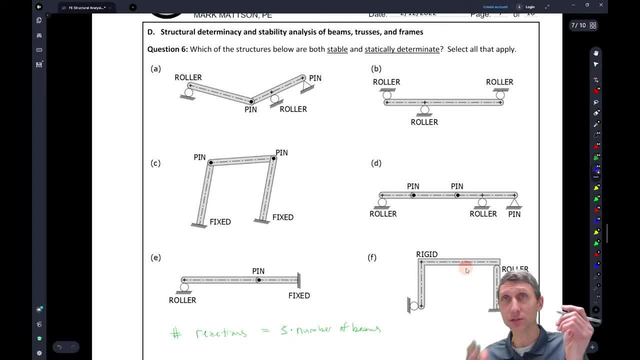 so what you have to do is you have to kind of understand. so when i see these structures, what i do is i like to just sort of draw in reaction forces instead of support symbols. so i'm going to draw in one reaction force here for that roller. i'm going to draw in two forces at the pin because remember those forces on either side of 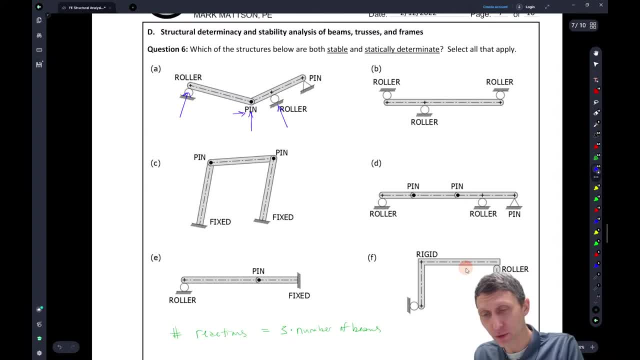 the pin are equal and opposite. i'm going to draw in another reaction force at a roller and two more at a pin. i like to draw the ones at the pin as vertical and horizontal normally, but then what i like to do is just go back and count them up: one, two, three. 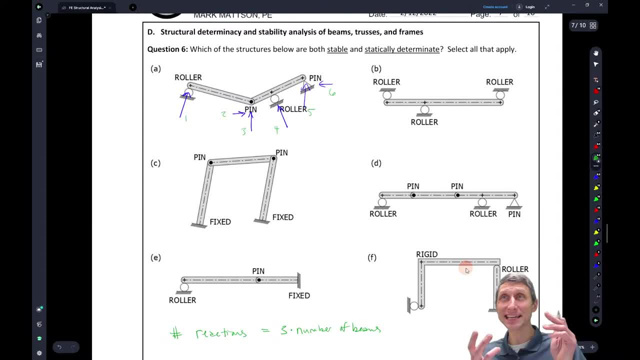 four and five and six and seven and eight and nine and ten and eleven and eleven and eleven and four, five, six, so i've got six um six reactions. so this is kind of like, if we think of it like this: six reactions, six r, and that is, is that equal to or greater than or less than? 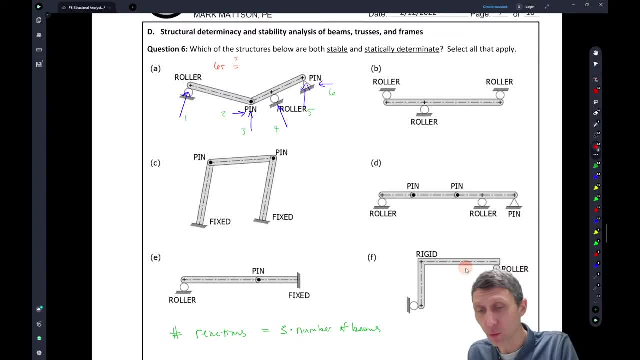 three times the number of beams, so i've got one beam here and two second beam here, so i've got three times two beams equals six. so this structure is technically statically determinate. you can determine every support reaction, pin reaction just by using the equations of equilibrium. so that checks this structure is statically determinate and you would circle this. 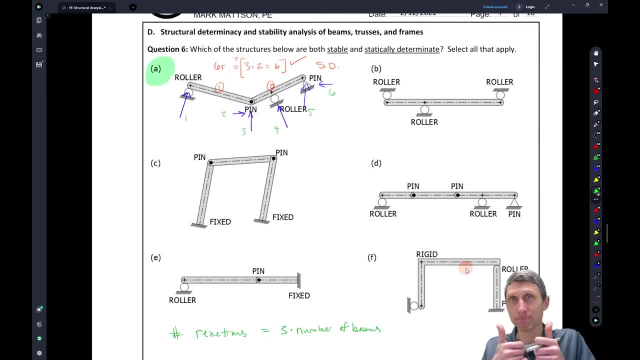 or put this down as statically determinate, okay, good. so now that we've done that, let's, let's apply our algorithm to the same thing. we got a roller, we got a roller, we got a roller. great, so we can count these up. we got one, two, three, so we got a roller, we got a roller, we got a roller, we got a. 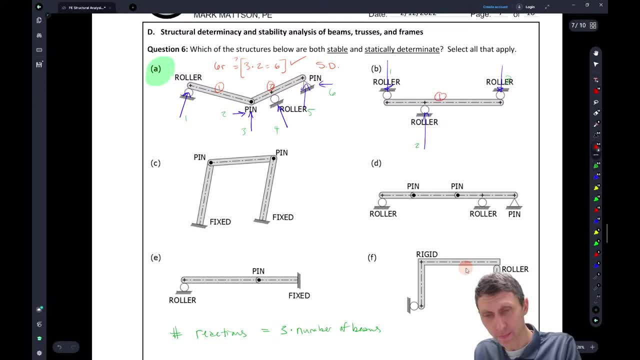 you know, we got one beam, okay, so this is great, we got. we got what we got: three reactions. is that equal to three times our one beam? yes, so three times three equals three. you know, whatever, three equals three. what's the problem? the problem is: any force. what do rollers do? the problem is: 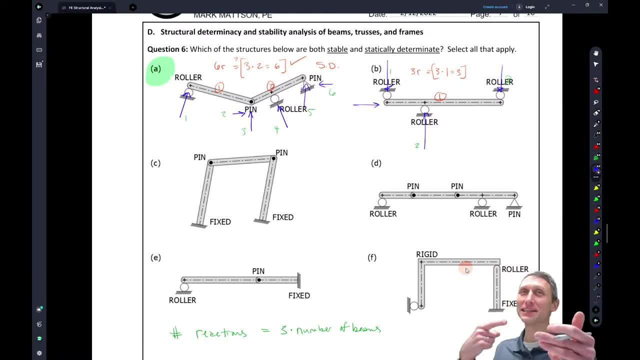 rollers roll things right. the problem is any force on this thing. the horizontal direction is going to be the resistance to x and z, and this is going to be x and z and this is going to be x and make this beam just roll away. And even though we got three equals three, this is just means this. 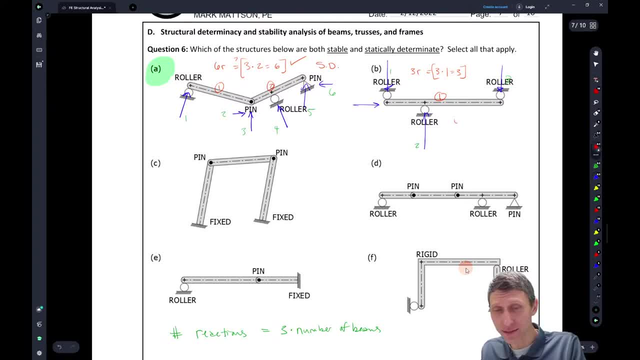 one is going to be what? this is bad because this is unstable. right, There's nothing resisting the horizontal forces. This is unstable and it's a big fat. No, Okay, It's not stable and steadily determined. Okay, Let's go to the next one, And again, I just like to sort of apply this. So I 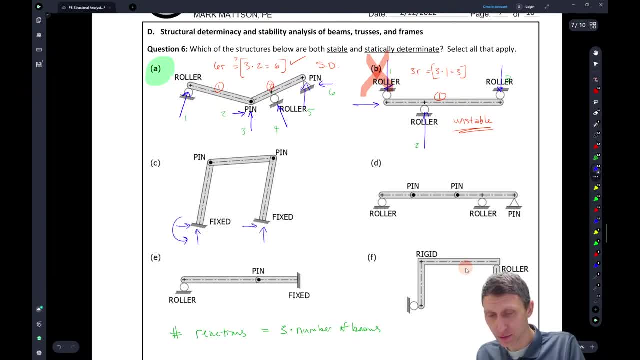 got one, two, three, one, two, three. So every fixed reaction is going to have three. How do you prove it, You don't? you just have to look at it. I mean, it's like this: yeah, this isn't like. 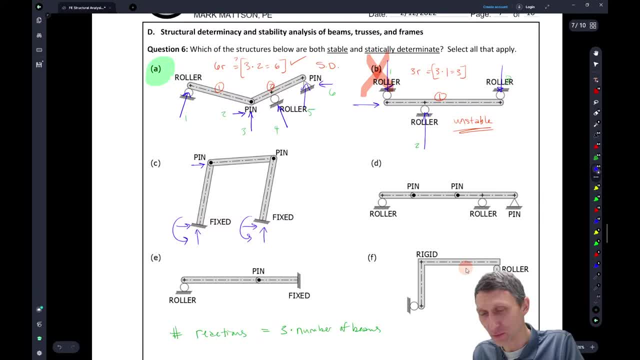 a prove or unprove thing, It's just a thing thing. Um, so we got one, two, you know one two, and uh, what do we got? The one, two, three. actually there is a way to prove it, Uh, maybe. 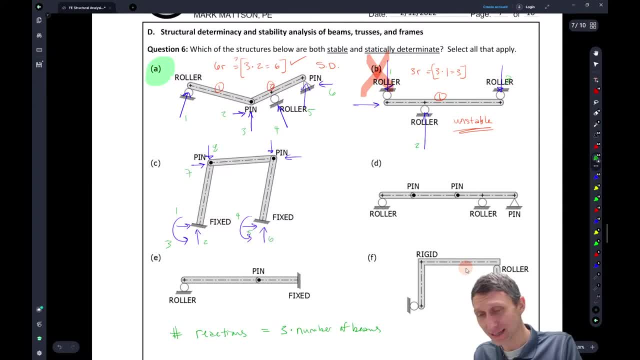 I'll show that to you in a second. Hold on Four, five, six, seven, eight, nine, 10,, anytime we don't get a multiple of three, or we should just stop and think for a second. but here, how many beams do we have? We have one, two, three beams. So what do we get? We get how. 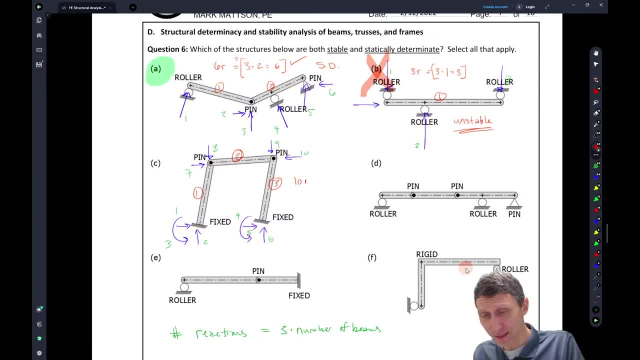 many reactions. You have 10 reactions. We got, we got three times. Well, actually we got um 10 reactions and three times three is nine. you know um nine equations and 10 is bigger than nine. So that means this is statically indeterminate to the first time. 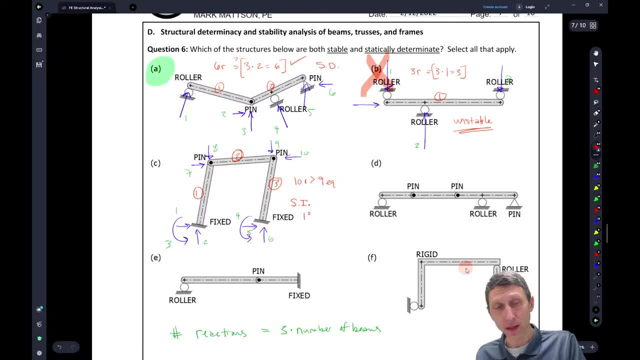 Okay, So the I just raised SI to the first degree, but also that means this is not statically determinate. Okay, How do we prove this one here? Uh, one of the things is, if you sum forces, I mean honestly if, if you sum forces in the X direction and let's say we put this force P here. 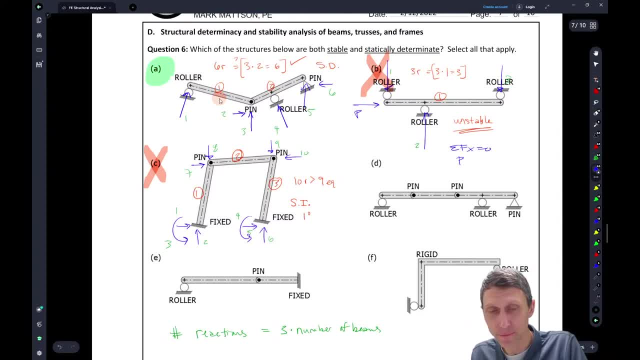 we sum forces in the X direction equals zero. P does not equal zero. We know that P is some value and P doesn't equal zero. P is the only value. So we know that P is the only value. So we know that P is the only force in the X direction. It's not being resisted by anything. 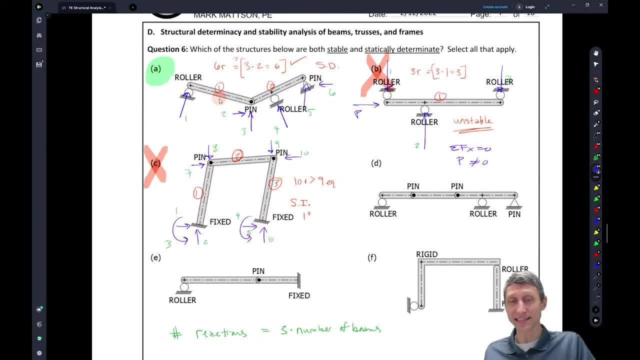 So that means it's going to move. There's going to be some mass times acceleration. It's not static anymore. Does that make sense? So that's one way I'd say you could prove that one. Okay, Let's keep going here. So we've got a roller, a pin, So we're rocking and rolling here. One you know we got. 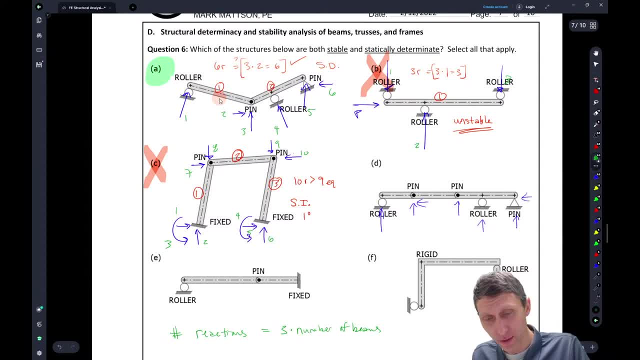 rocking and rolling and we're good, So, um, let's just count these up. So 1,, 2, 3, 4,, 5, 6, 7.. Okay, 7.. Did I count all those right? No, I missed one. I missed one in here, I got. I got an eighth one in. 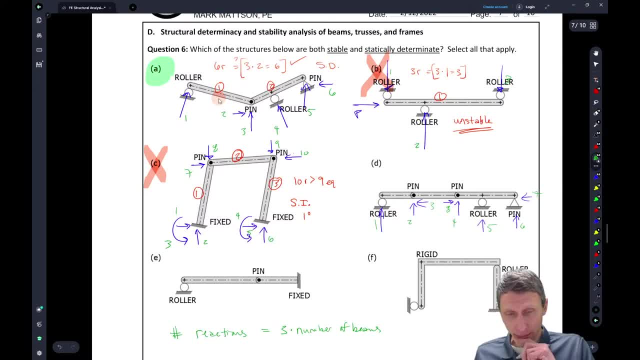 here that I missed. I got two at the pin. Okay, So I got eight reactions, eight, Uh, actually, let me just switch colors here. So I've got eight reactions, maybe, um, eight reactions, which is less than. uh, how many beams do we have? We have one, two, three beams. 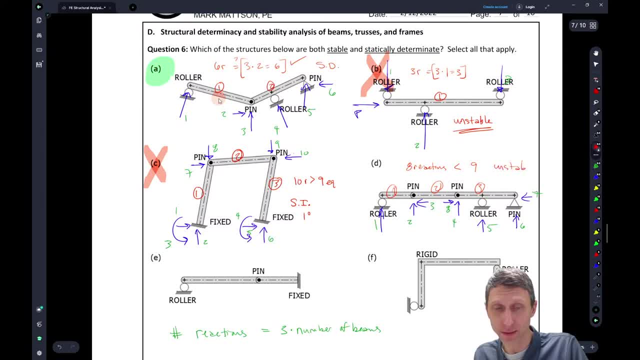 less than nine. That means this is just unstable. You don't have to do anything else. We don't have enough reactions. I mean honestly, you can just look at this one and hopefully see that this thing is unstable, right Cause this pin, this, this thing is just going to want to collapse. It's a. 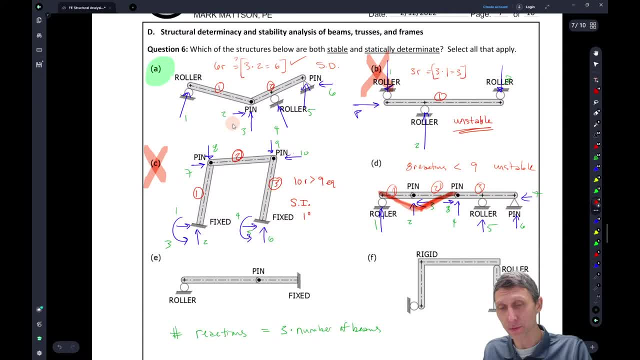 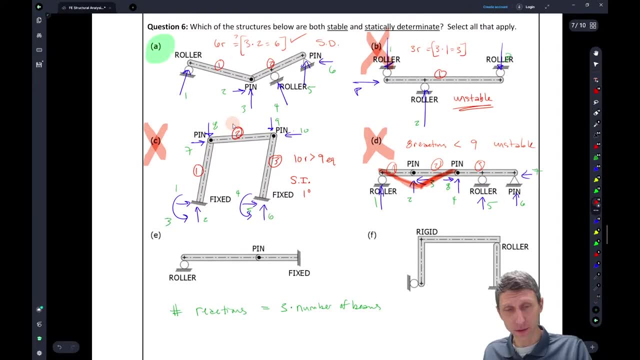 collapsible mechanism. Okay, So if you have got a collapsible mechanism, you don't even have to keep going, cause it's just going to collapse and that's unstable. So let's keep going, though, and figure out what we're doing next. We've got a roller. we've got a pin. a roller has one, a pin. 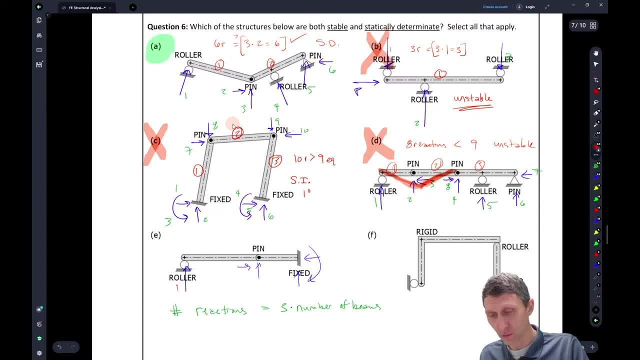 has three, a pin has three, a pin has three reactions. So, uh, we can do the same thing, kind of going here. We got one, two, three, four, five, six. This is looking good. We got a multiple of 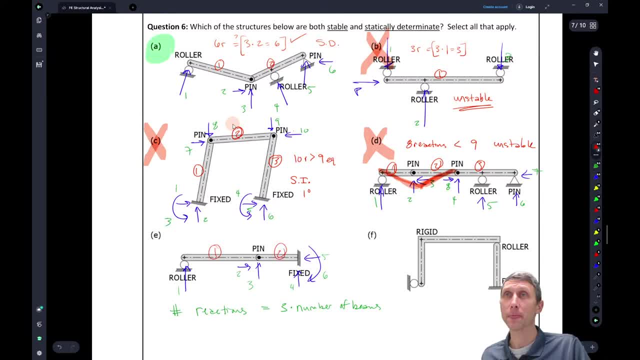 three. How many beams do we have? We have one, two beams, So that means we got six reactions. This is equal to three times two. three times two, that equals six, And this one is statically determinant. So we've got another one. 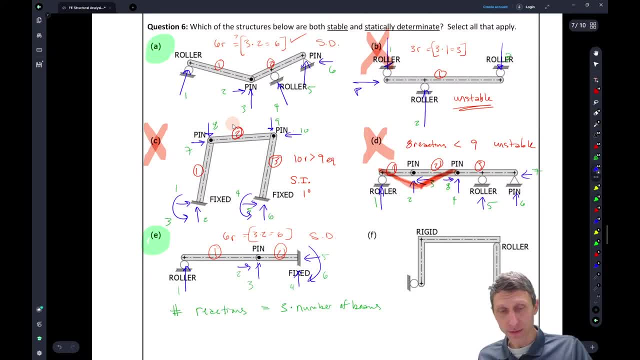 Okay, So we've got a three-beam. Okay, So this one's got a three-beam. Okay, So we've got another one. that's good, and then, lastly, we're just gonna go here, so we got, you know, one. 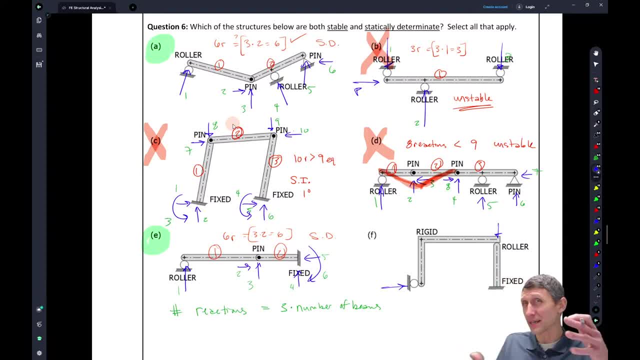 reaction there, one reaction at this roller. so sometimes you have rollers that connect things rather than pins. but this is a, you know, this is, this is another one, and then two, three, four, five. so this again we can see. hopefully you can see one, two, three or five reactions, five reactions. 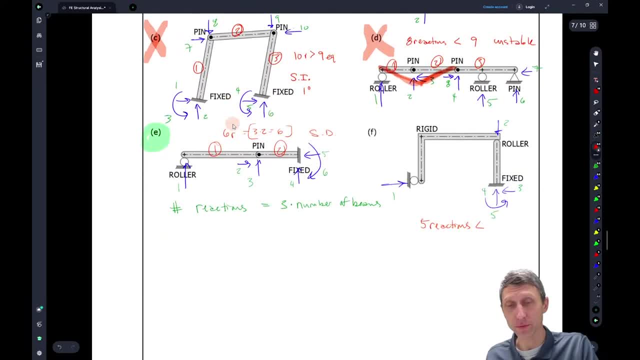 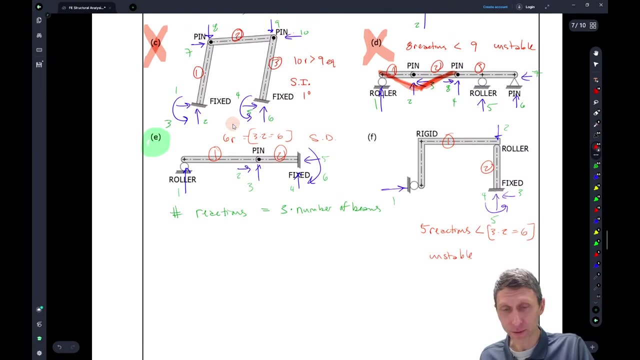 which is less than how many beams do we have? we have one beam and a second beam, so we got three times two. it's less than six. so that's gonna be also unstable. so we got a couple that are. we got a number of them that here that are. 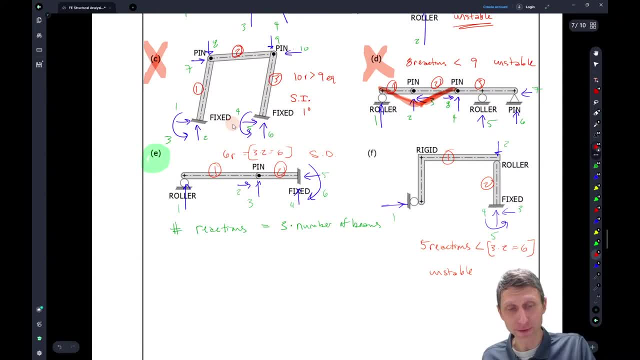 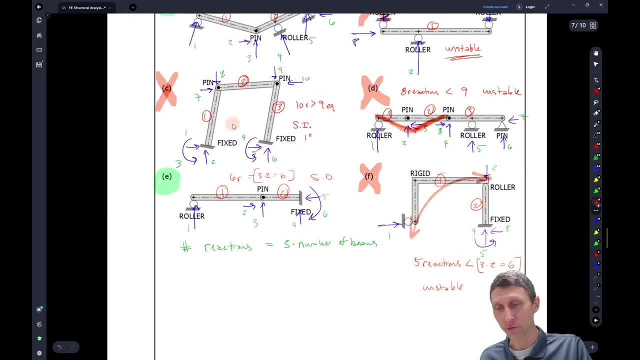 unstable. I mean with this one even um, what you could see is you have kind of a, you have a rotational instability here. if you think of it like that, there's a rotational instability as well. so when we're also sudden done, we get two that are statically determinant. we got two that 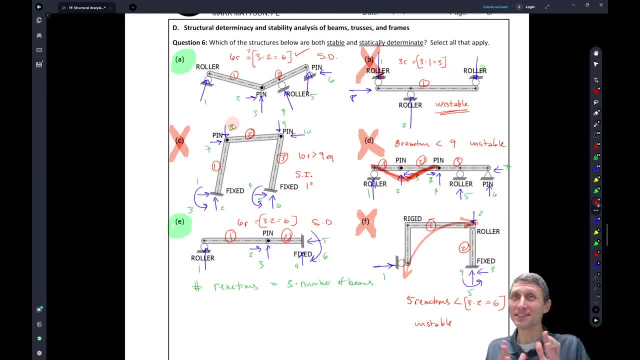 we can, we can deal with okay, so. so sometimes I mean it's just, it's it's getting those numbers down. but hopefully you can get a little bit of this where, like, you start thinking like, okay, so they determine it, and you don't have to write these things down. you're saying okay, one, two, three, four, five, six, and you 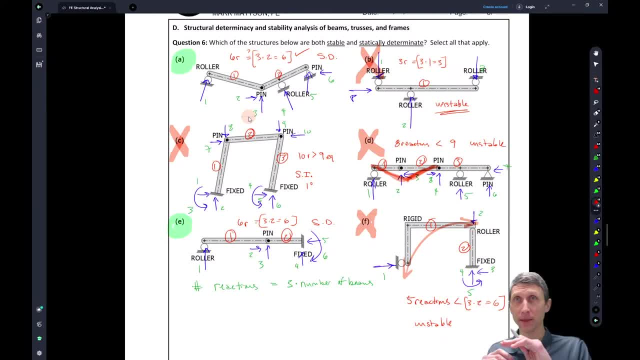 can just say six, and there's two beams. six equals six. we're good, okay. are they gonna ask all this? maybe not. could you sit a similar thing with trusses? yes, you could. this is kind of the big picture, how to look at it, though. okay, gotta three questions left. let's, let's keep going here. 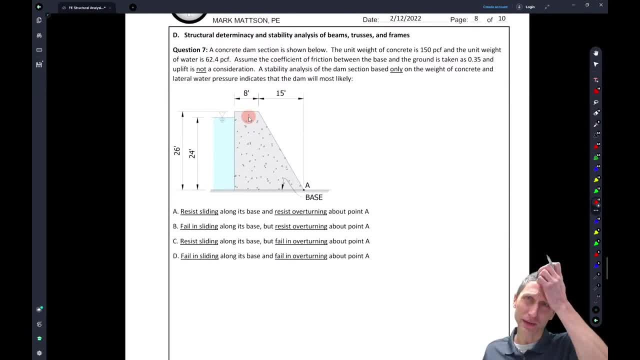 and this might be the hardest one of the three questions. I don't know, maybe it's not, but oh man, actually when I first saw it, when I first was reading through that fees back and I saw it: determinacy and stability analysis. this just brought me back to consulting, where we did concealed civility analyses. so the damn. 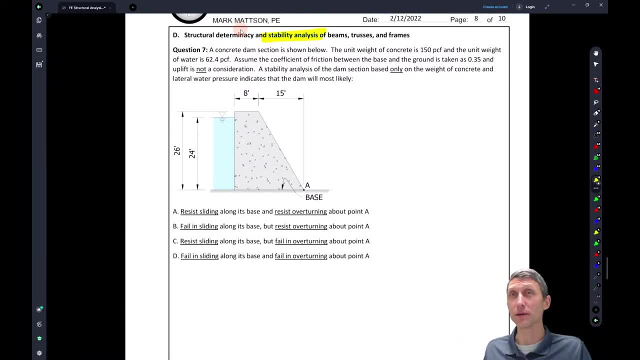 sections for a living. I mean, like we get paid money you to do this stuff. but I'm I'm not joking, I'm not making it up. You get paid money to check to see if a dam is stable. Okay, I way oversimplified this stability analysis. 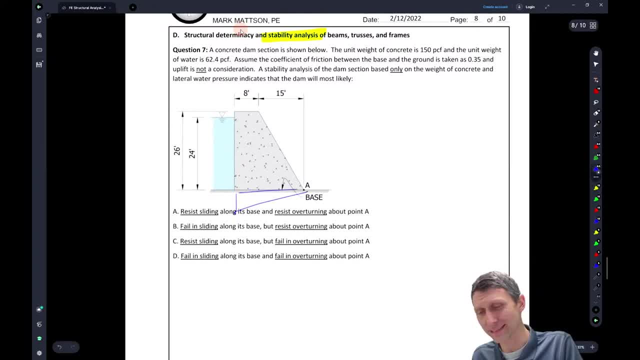 because I just said, don't assume any uplift, okay, But is that a real? is that real? Probably not, but let's just go with it for this question. Okay, the question says we have a concrete dam section below. 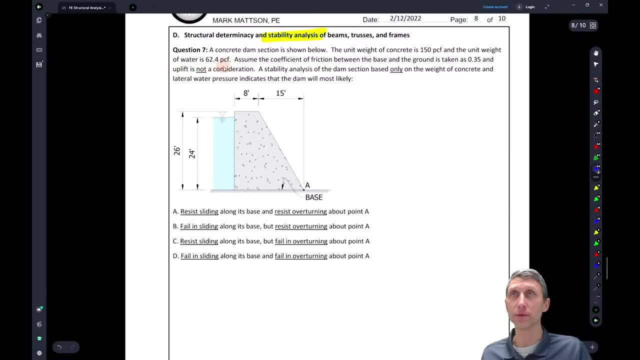 unit weight is 150 pounds per cubic foot. unit weight of water is 62.4 pounds per cubic foot. Assume the coefficient of friction between the base. so down here the base and the ground is 0.35, and uplift is not a consideration. 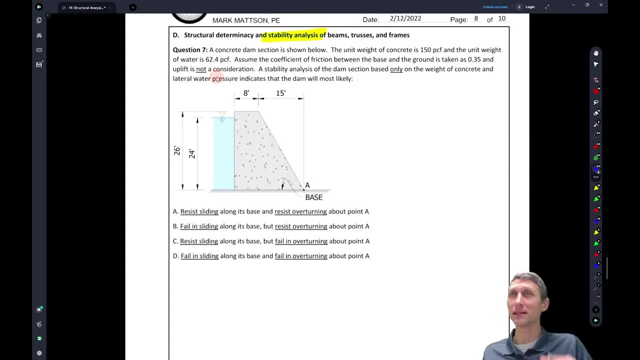 So we're not. I mean, maybe when we get to geotech we'll deal with some of those flow nets, uplift, all that fun stuff, but we're not gonna deal with uplift right now. Okay, stability analysis of the dam section. 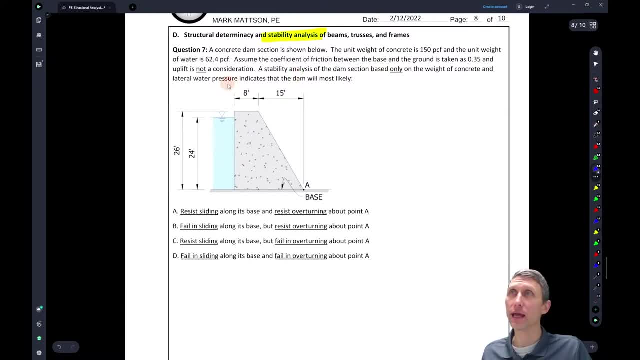 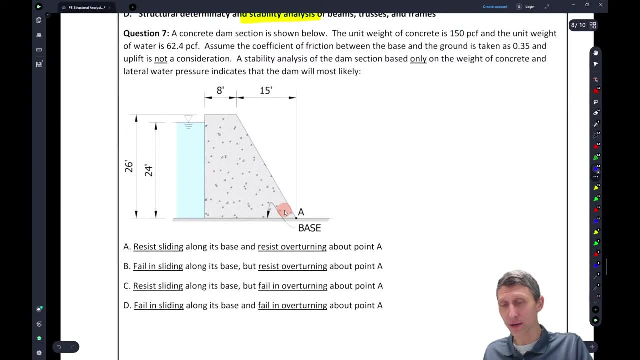 based only on the weight of concrete and lateral water pressure indicates the dam will most likely do what It'll: resist sliding and resist overturning. It'll do none of the above and it'll fail and fail. I don't know. so basically, we have to check two things. 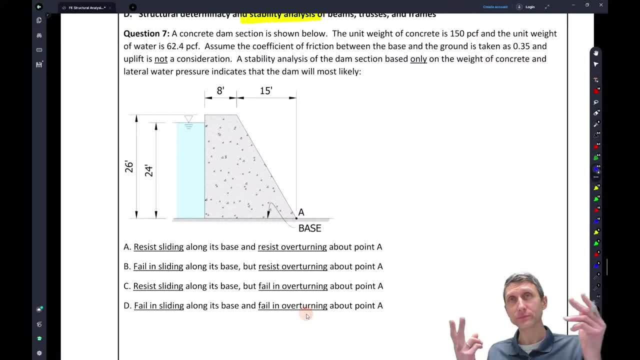 We have to check sliding and we have to check overturning. Okay, is this doable? I think it is. Let's take a look, though, and see. So if I just redraw my dam section here for a second, So ah, I probably could have drawn that better. 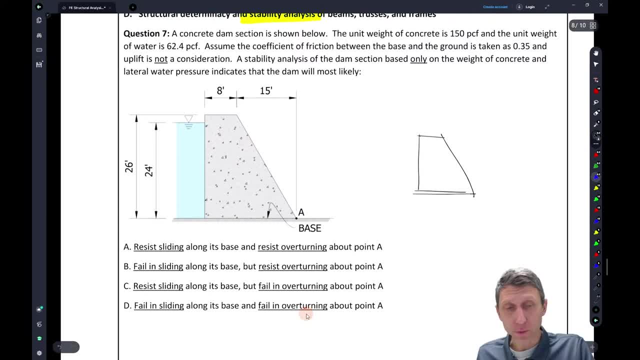 What forces I mean? well, let's think of the free body diagram for a second. What forces do we have acting on this? We have some water force. we've got some concrete weight right, And the concrete weight I'm gonna break up into kind of two sections here. 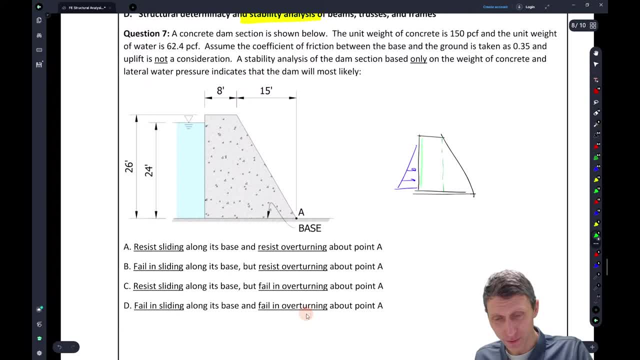 I'm gonna break up into, you know this, maybe this rectangular section and then the other section I'm gonna do here is gonna be kind of this triangular section, Because the weight's gonna vary. So if we think about this, we have to think about: well, how much does this thing weigh? 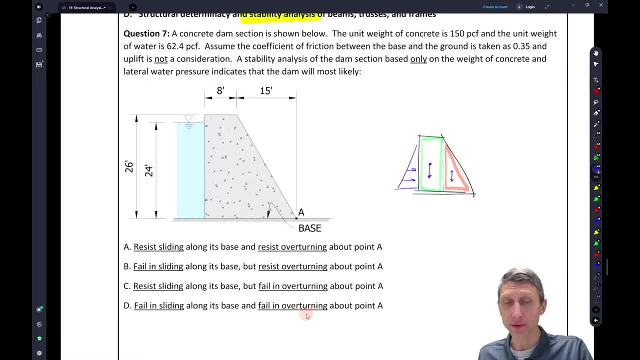 How much does this thing weigh? And the way that I think about it is, it's sorta kinda, kinda sorta. actually, it's just like if we have a uniform load up here and a- you know, horizontal load or, I'm sorry, a linearly sloping load here. 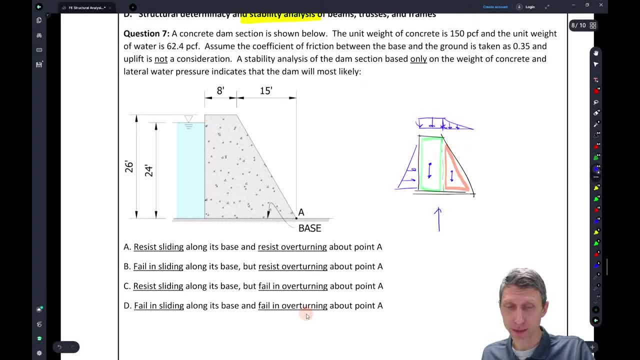 Those are kinda the forces that are holding this thing down. Now, what's pushing back? Obviously there's gonna be some normal force, there's gonna be some friction force, Okay, So let's just see what's going on. So let's take a look at this and see how this works, right? 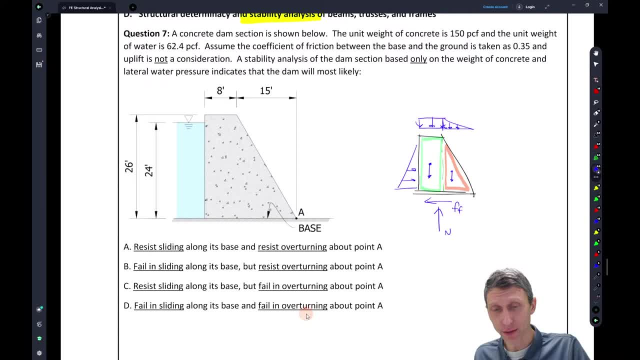 So, as we get started here, we have to find a couple things. We have to find this pressure down here. What's that pressure? Do you remember? do you remember it's gamma water times H? Remember that. What's the pressure, so to speak, of this concrete weight? 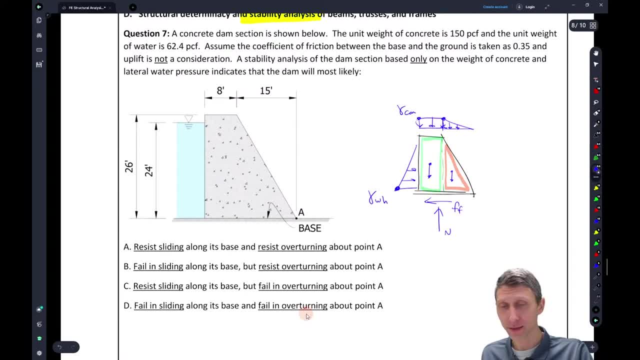 The concrete weight is just gonna be the gamma concrete times its height, right? So that's gonna give us these pressure values. So, if we think of this, you know this one, what's that? Well, we have 62.4 pounds per cubic foot. 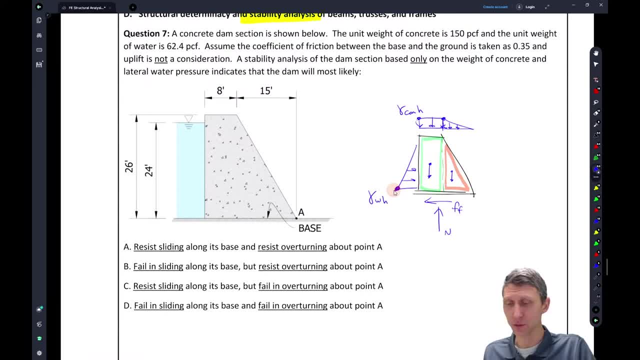 So let's go to a one foot section. What do we get? We get 62.4 times what's the height of the water. The height of the water is 24.. So 62.4.. Let me just write this in: 62.4 times 24 feet. 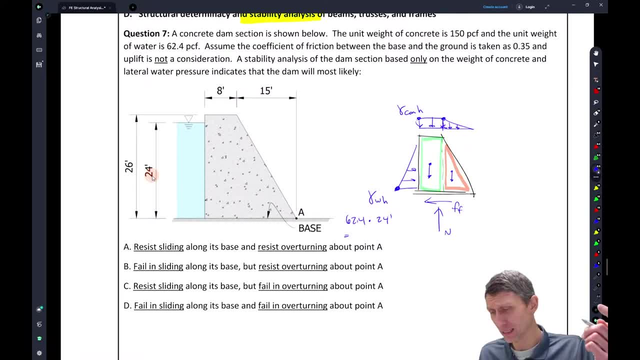 What's that gonna equal? It's gonna be about 1,500, 1,498, 1,498.. What's that? pounds per square foot? Okay, and then if we do the same thing for the concrete, what's the concrete? 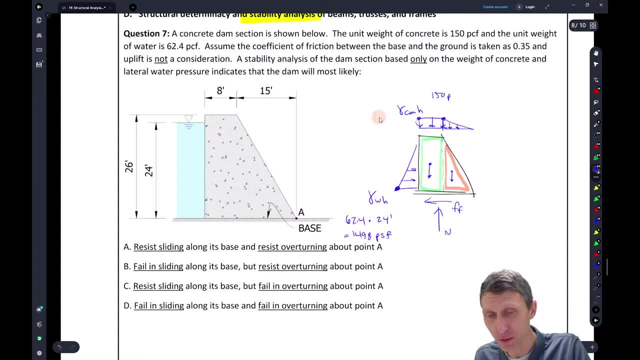 The concrete's gonna be 150 pounds per cubic foot times its height. its height is actually a little bit different: It's gonna be 26.. So maybe there's some gates in this dam and the water's not going over it. Okay, so let's look at it. 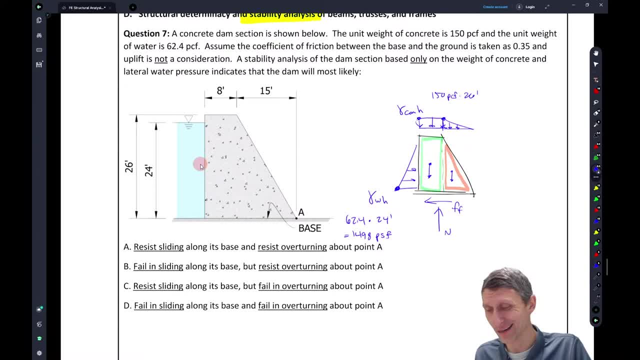 150 times 62.4 is gonna be 93,. I'm sorry I did that wrong 150 times. I wrote down 26,. I said the wrong thing. This is gonna equal 3,900 pounds per square foot. 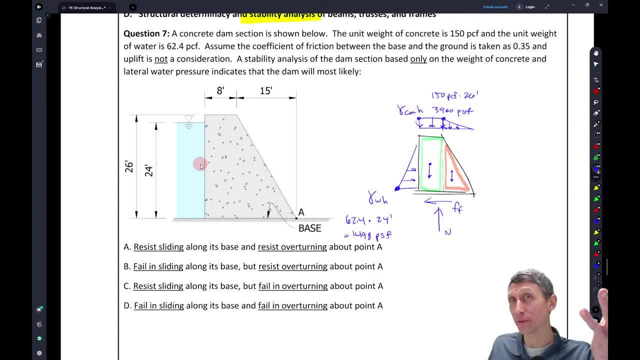 And if you think of a one foot section, this becomes pounds per foot. okay, There's nothing super crazy there, And now all we're trying to do is we're trying to figure out what these forces are, So we know that we're gonna have some resultant. 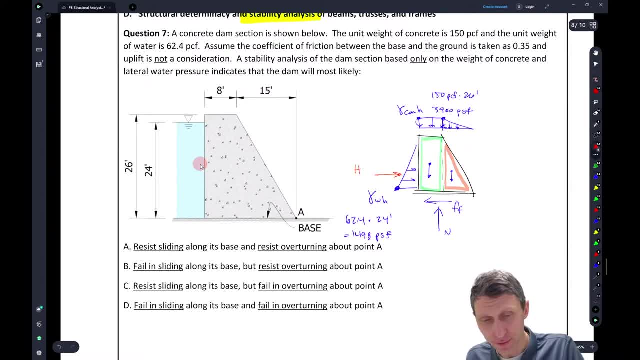 kind of forces here. We're gonna have this horizontal force, We're gonna have this: the weight of the concrete one, you know kind of like weight of concrete two. I'll just do it like that. But let's figure out what those forces are. 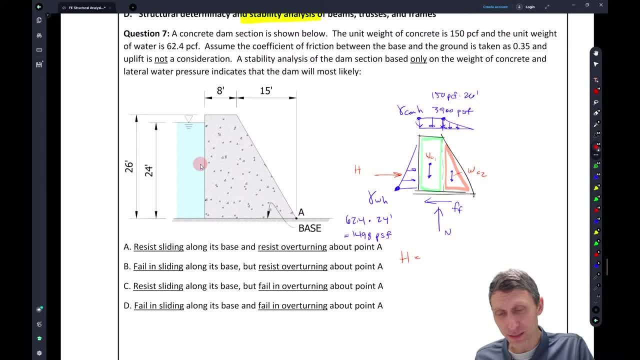 So H is gonna be what It's just gonna be. this pressure of the water right Times its height again times one half. So this is gonna be one half of what 1,498.. I'm gonna change this to pounds per square foot. 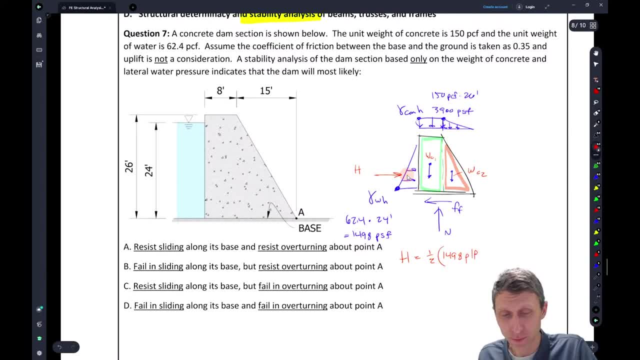 I'm gonna multiply it by one foot to do a one foot section, just a one foot section. I'm gonna multiply it by one foot to just do a one foot section of the dam, And then I'm gonna multiply this by 24 feet. 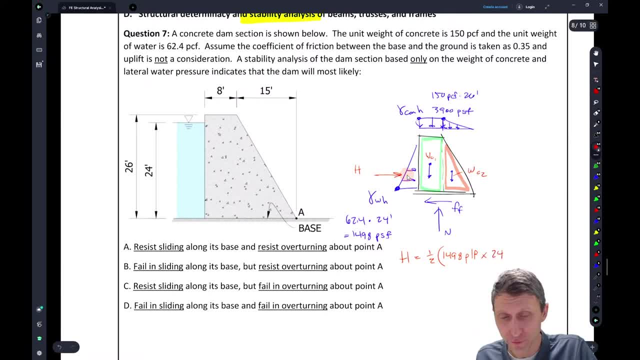 its height again to get that H force. So if I do that, 0.5 times 1,498, times 24 is gonna be like 1,7976. So almost 18,000.. I'm just gonna call that. 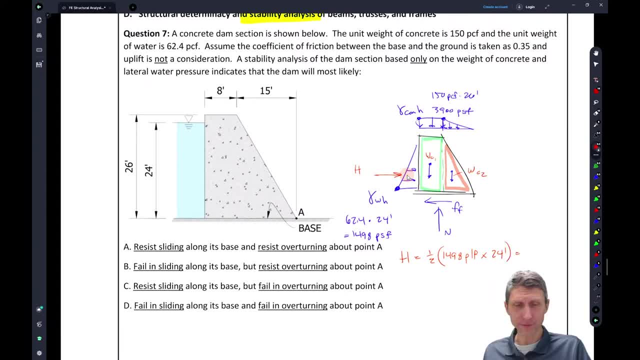 I'm just gonna call that 18,000 and just round it off 18,000 pounds. Okay, let's look at the weight of the concrete one. What's that? It's gonna be like. it's gonna be like. 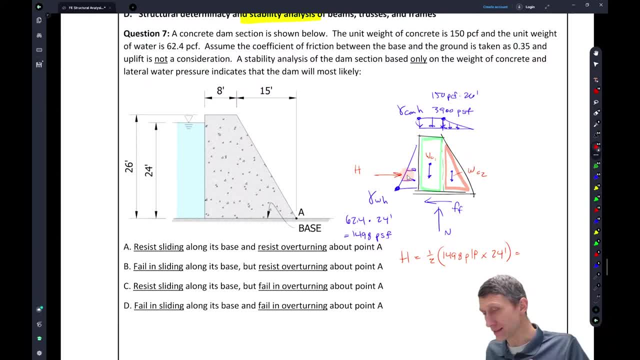 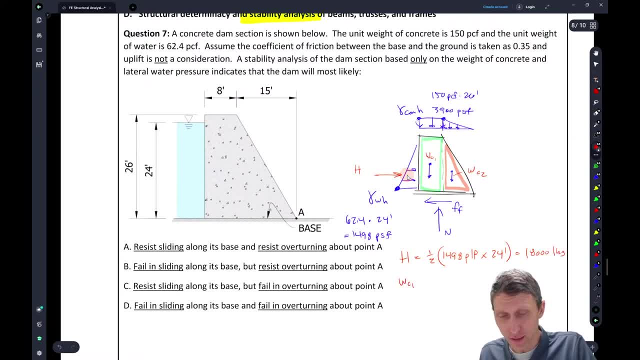 How far does that act over? It acts over 8 feet. So times 8 feet Equals what? So 3.9? so 3.9 times 8. times 8 is 31.2. times 8 is 31.2. 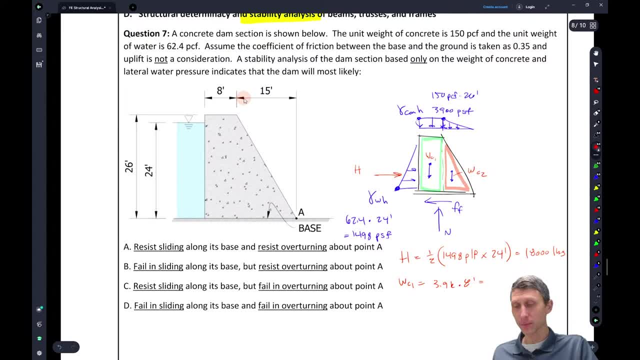 times 8 is 31.2 kips. Okay, So I'm just check the conversion on the fly here a little bit. If you go 4 feet a little bit more to the side, a little bit more to the side. 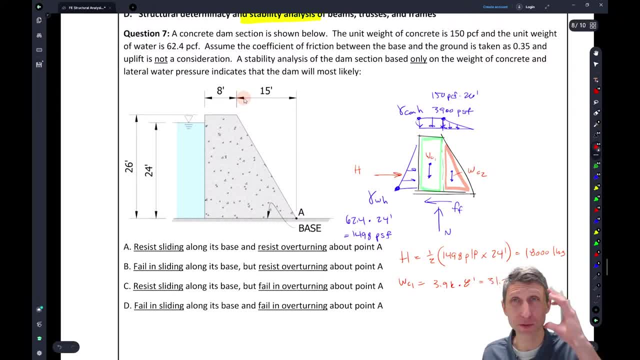 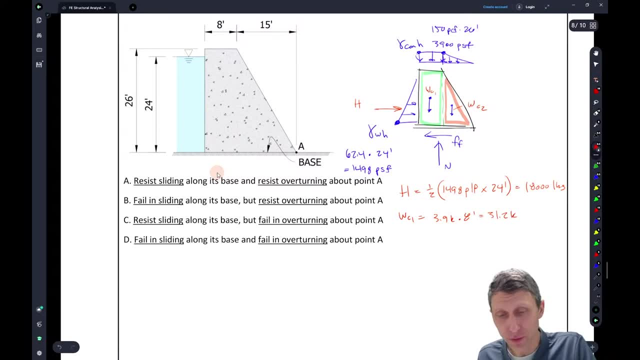 You rip that edge out. So this third comp square, you get 100住mca, that 11th comp square. So if I go 4 feet from 5 feet here, pounds to kips, right, 1,000 pounds per kip, And then this WC2, what's the weight of the kind of? 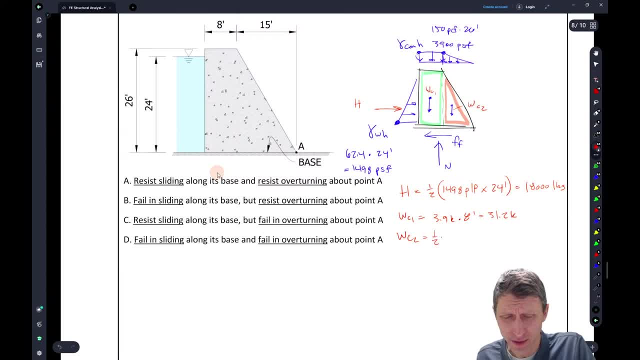 the triangular section. So this is going to be similar. It's going to be one half of 3.9 times. it's not eight feet anymore Now. the length of that triangular section is 15 feet and kips per foot- I should probably put in here kips per foot. So what do we get? So one half, so 0.5 times the. 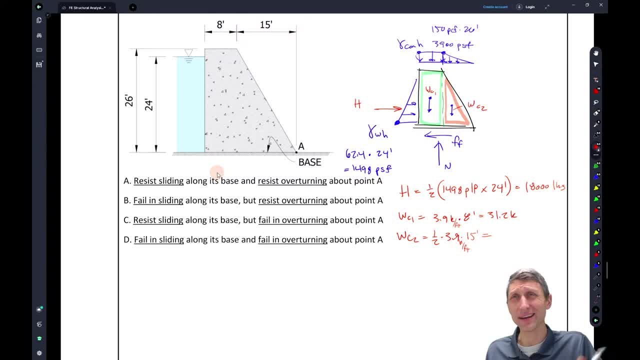 3.9 times 15, and I get like 29.3, roughly so 29.3 kips. So these are kind of the components of forces in that free body diagram. So now let's, now that we have those, let's tackle this a little. 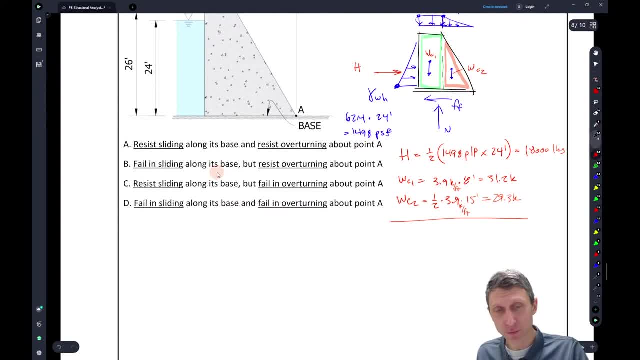 bit right. So let's just start with sliding right. So for sliding, this is kind of a statics problem. I mean it's this is honestly a statics problem. The stability analyses are kind of just like let's. 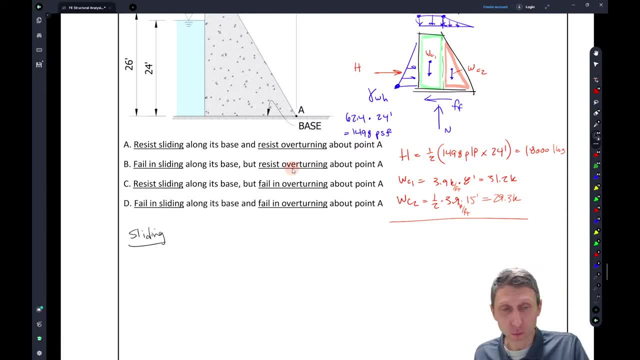 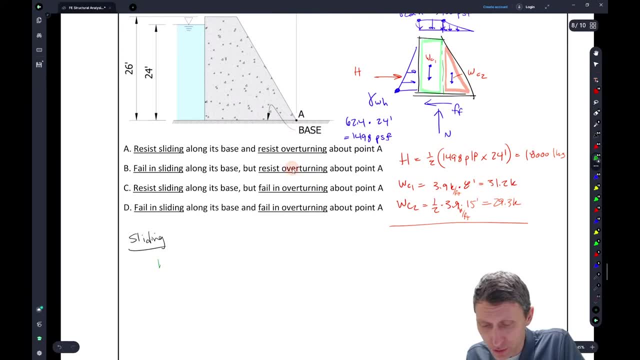 let's do statics. but for sliding, what do we? what do we want? We want, or what we want, is this thing to be stable. So for it to be stable, what we want is the horizontal driving forces. So the horizontal forces, you know the driving, maybe we could just put driving forces. 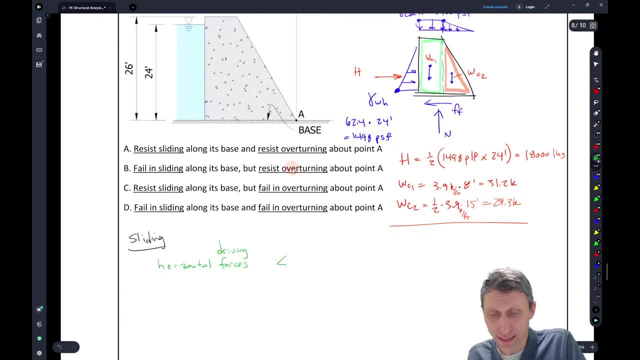 has to be less than what the friction force is at the base to resist sliding right. So this has to be true. to resist sliding, Does that make sense? So the water that's trying to push this has to be less than the friction that's available. 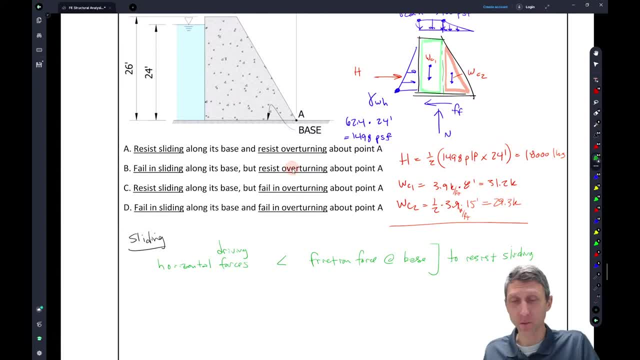 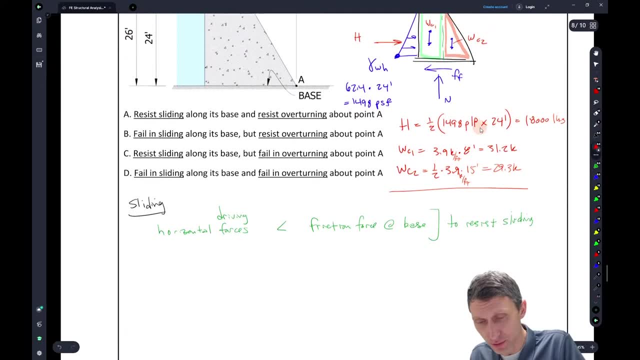 so that this thing resists sliding. Okay, so what's the horizontal force? The horizontal force is just this 18,000 pounds, right? So the horizontal force is easy. This is just the driving force. is h equals 18.. I'm just going to convert here 18 kips. 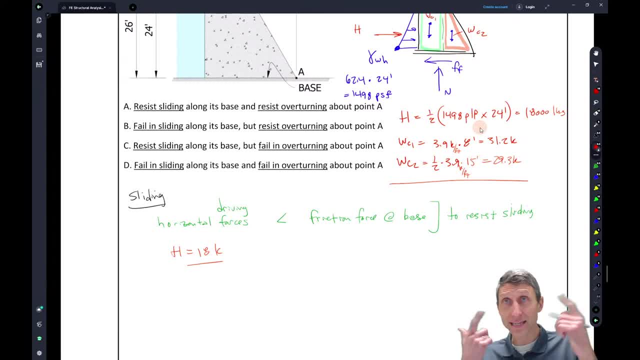 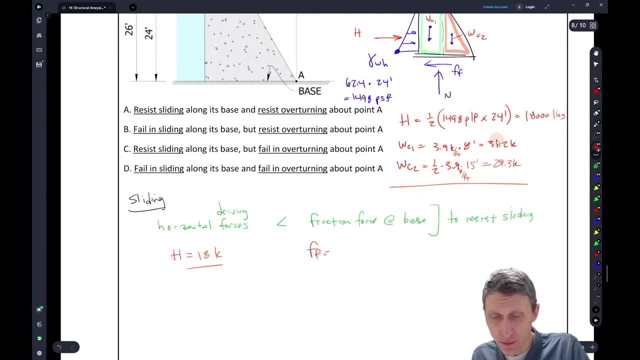 We already know that. so it's the water force trying to push this thing. Is that less than the friction of the base? Well, what's the friction of the base? The friction of the base is developed how. The friction of the base is equal to mu times the normal force, right? 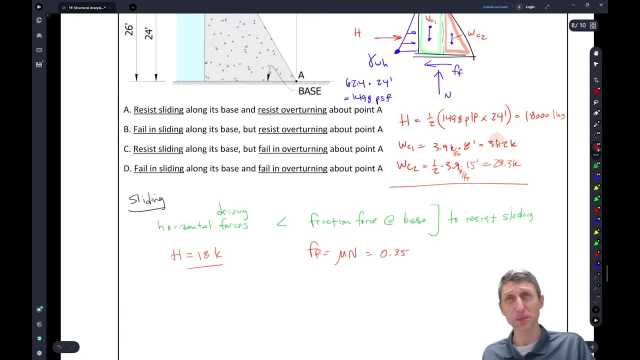 So what's this? We were told that the frictional coefficient was 0.35 in the problem. above times what? The sum of the vertical forces? essentially The sum of the forces in the y direction. You catch that. So, just like friction and statics, it's the same type of thing. 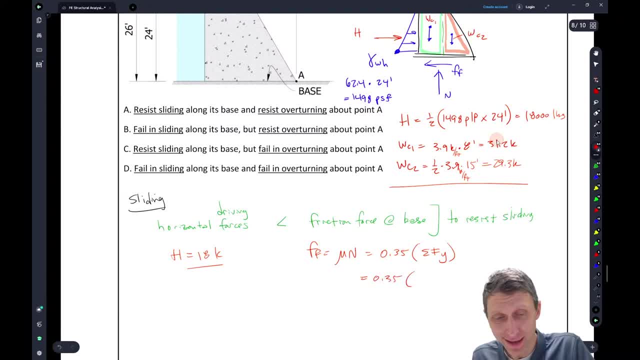 What do we get? We get equal to 0.35 times. oh, what's 31?? What do we get when we add this up, 31.2 plus 29.3 is going to be 60.5.. And when we do that out, we get 0.35 times 60.5, and I get like 21.2 kips. 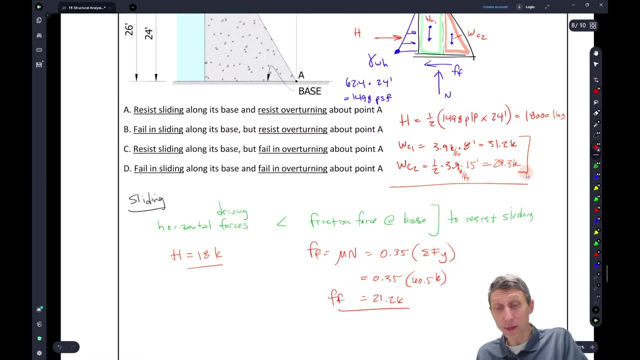 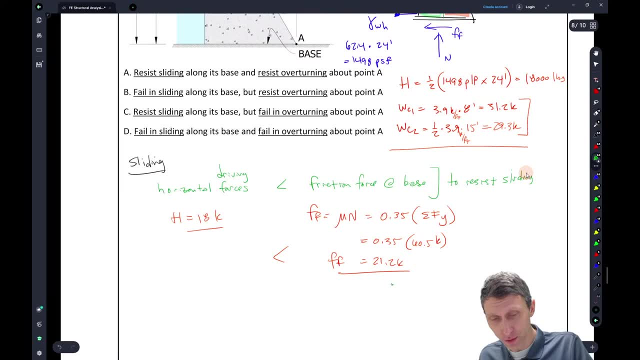 So the force of friction is 21.2.. Which is indeed greater than our horizontal force. So this structure therefore, stable in sliding. Okay, So it's stable in sliding, It's not going to go anywhere. The friction, and you might be saying, well, is the friction going to push it back? 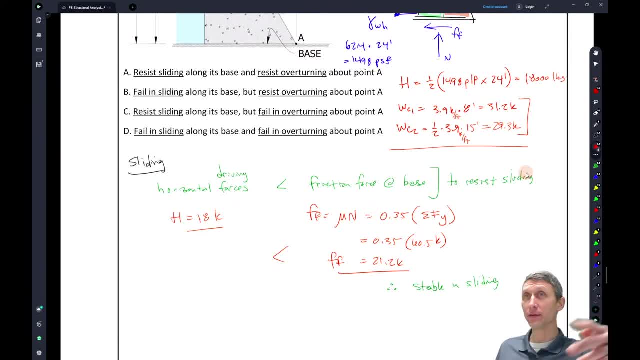 And no, you only get as much friction as you need. If the horizontal force is bigger than 21, then there would be a problem. But I've never seen a dam. I've never seen a dam go travel back upstream into the river because friction pushed it up there, right? 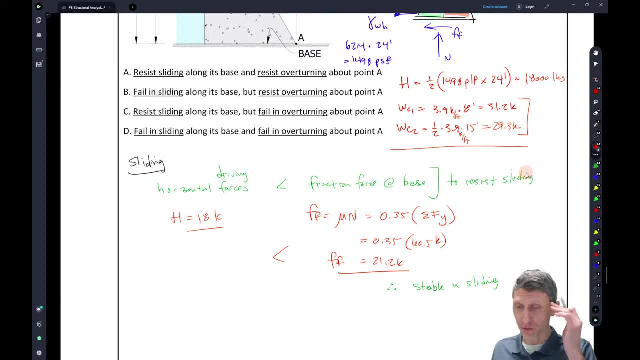 The only problem you get is when the water pushes it down right. So the only problem you get is when this horizontal force is bigger. Okay, so it is stable in sliding. So that means we can just go and cross out the fail in sliding. fail in sliding. 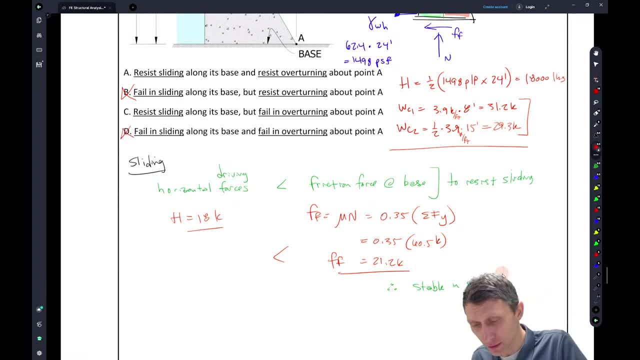 Okay, so we know it's going to resist sliding. And then let's take a look at overturning. So what's overturning here? So overturning You guys doing okay, I mean, you guys probably are sitting there with, like dinner. 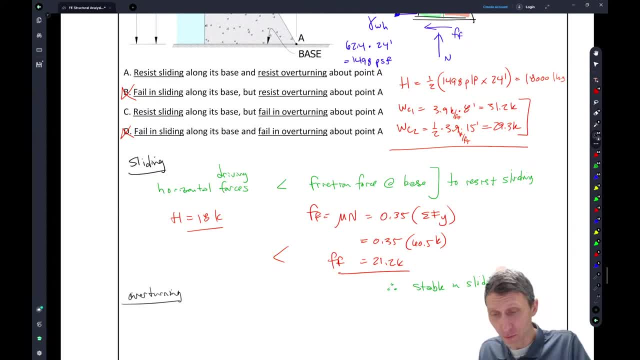 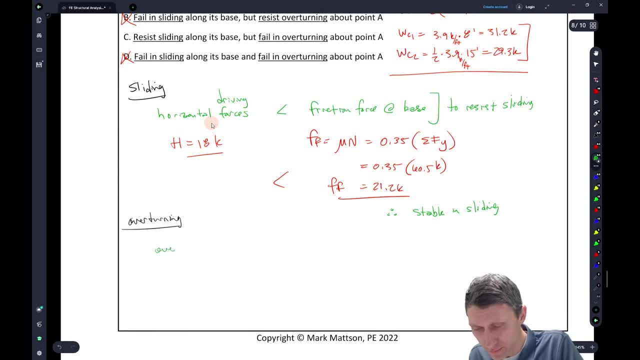 But who knows, Maybe not. But so what do we have? We have overturning. What do we want for overturning? So let's take a look at this And basically, what we want here is we want the overturning moments, We want, you know, to be stable. 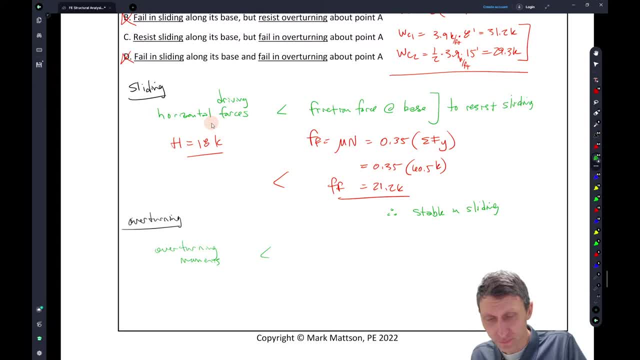 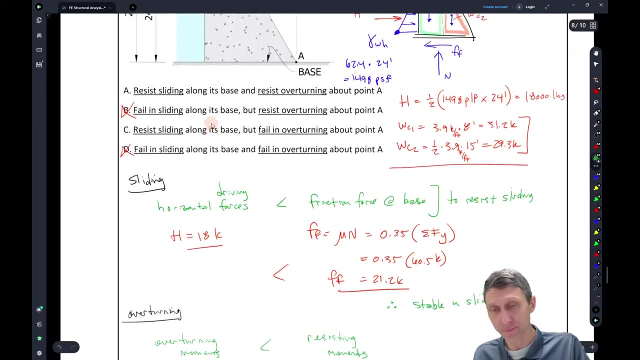 We want this to be less than the resisting moments. So, in other words, we want more holding it down, More holding it down than trying to turn it over. Okay, So what do we get? Well, what overturning moment do we have here? 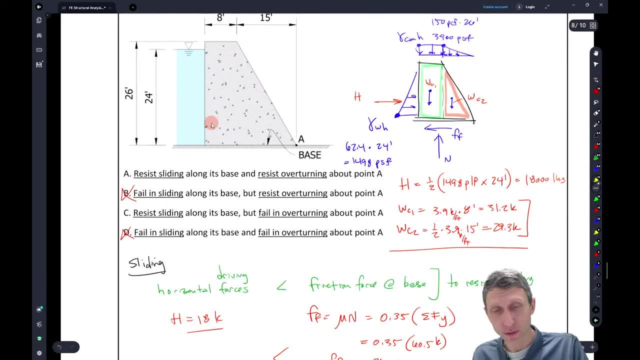 Well, the only thing that's trying to turn this over right is this horizontal force. The horizontal force is trying to totally push it over. Okay, what's trying to hold it down? The weight of the concrete is trying to hold it down. 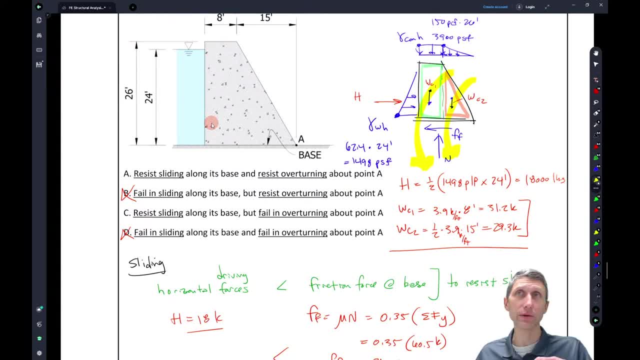 Does that make sense? So, basically, we get two moments from the weight of the concrete And somebody's probably out there saying: well, what about the normal force? Well, technically the normal force doesn't really work if the water's too big. 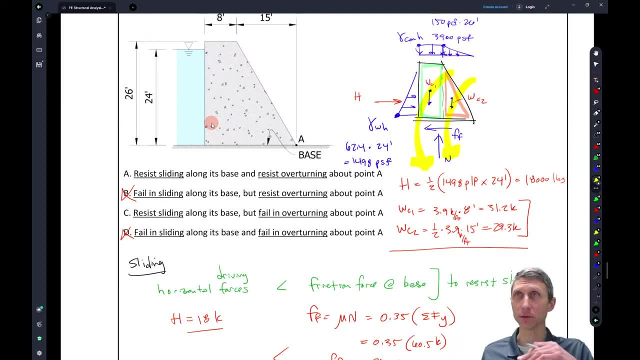 So if the water starts to overturn it too much, your normal force sort of goes away. But we'll go from there. So let's just look at those two sets of moments and see which one's bigger, And then we know if it's going to be stable. 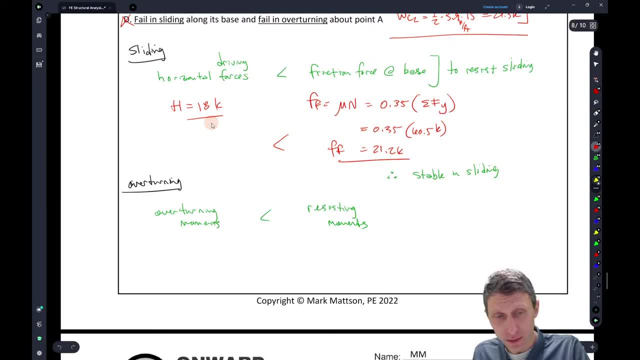 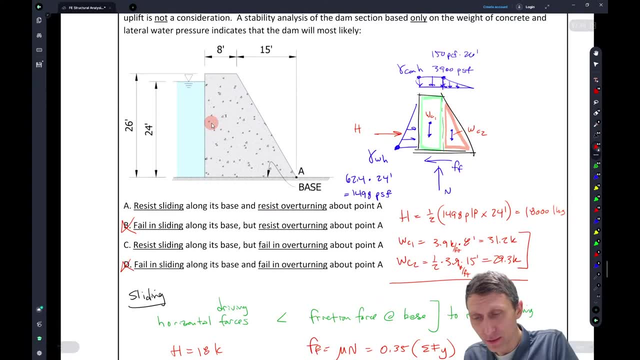 So let's look at the overturning moment. So what's that? It's going to be the horizontal force times its moment arm. So what's its moment arm? It's just going to be, you know, one-third of this distance, or 24 feet. 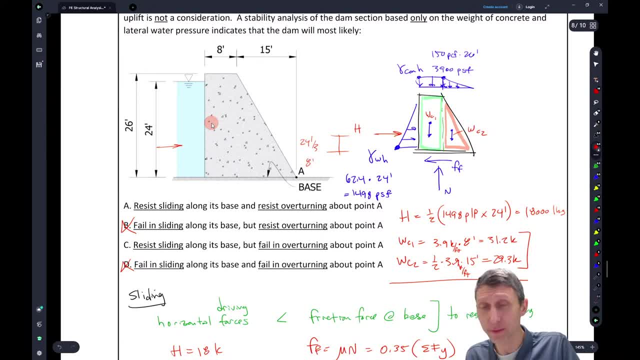 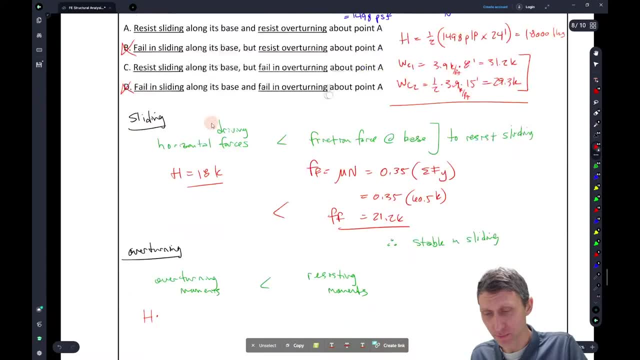 What's this? 24 feet over 3, which is going to equal what? 8 feet? Okay, And this is where uplift really comes in, But we're just ignoring uplift on this one, because that's what the problem says. So, 18 times this 8 feet. 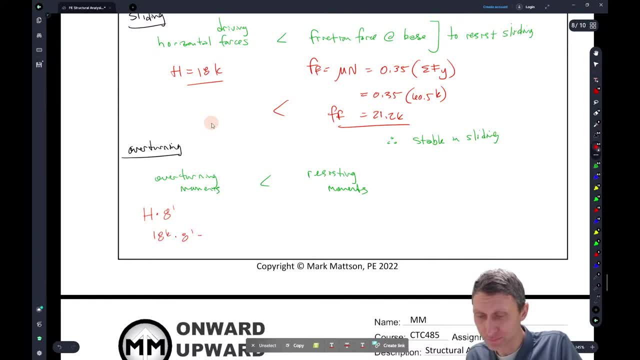 So this is 18 kips times 8 feet. So if I plug that in, what do I get? 18 times 8 is 144.. Did I do that right? I think so. I don't know. Let me check my answers here. 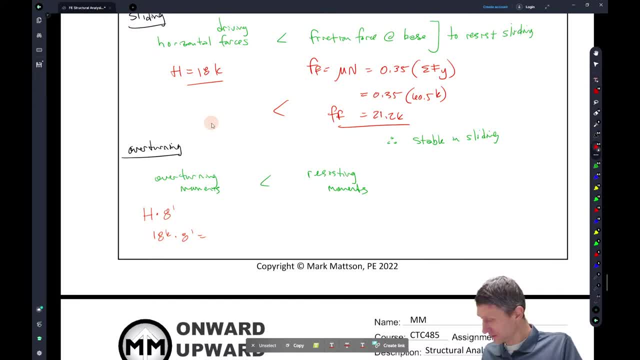 But hopefully it makes a little bit of sense. Yeah, that's the number I got. It's just I had remembered a different number. but who knows, 144 kip feet, So that looks good. The resisting moment is what It's going to be: WC1 times its moment arm. 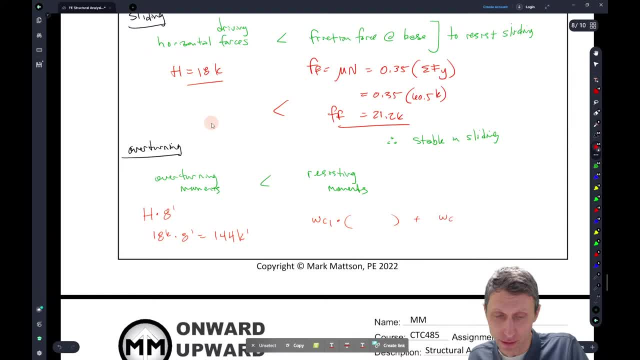 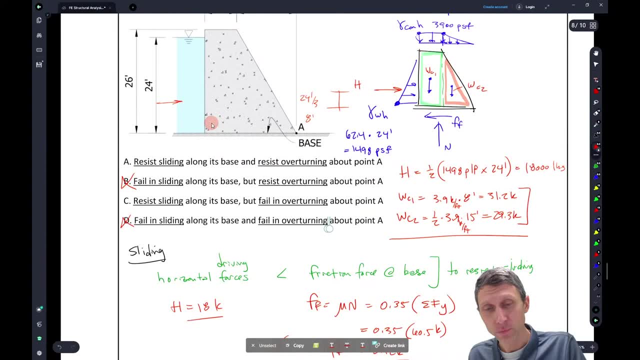 And you know, and we're going to add in WC1.. Okay, WC2 times its moment arm And let's go find those moment arms and then we'll figure out whether this thing's stable or not. So the moment arm for WC1, we're going all the way here to point A right. 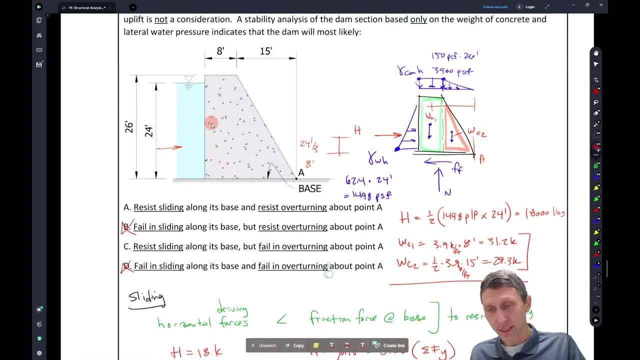 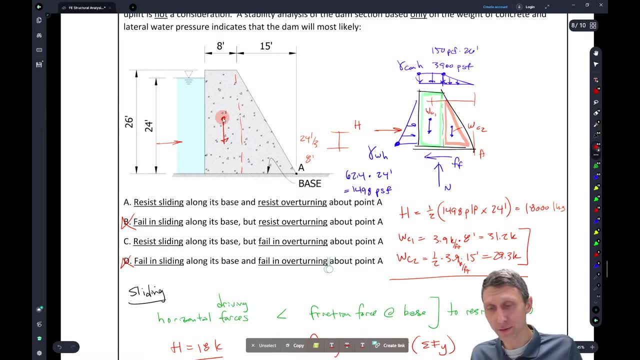 This is point A. What's that distance? Well, to get to, you know, if I come to my big diagram here, this thing's going to be right at the middle of that 8 feet. So to get to there, I need to come all the way to here. 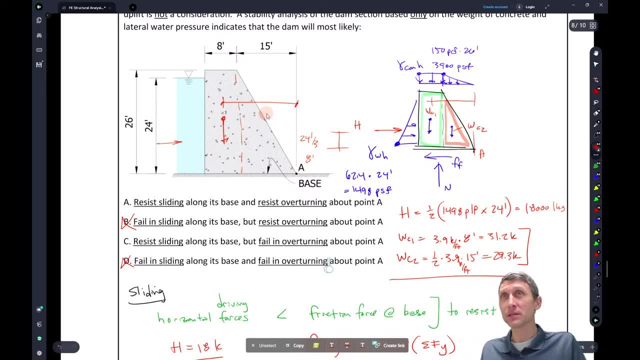 So it's at 15 plus 8 over 2.. Do you see it? It's this whole 15 plus half the 8.. So 15 plus half the 8, that's going to be 19 feet. And then, similarly, we're going to have this weight of the concrete here, which is just going to be two thirds of that 15.. 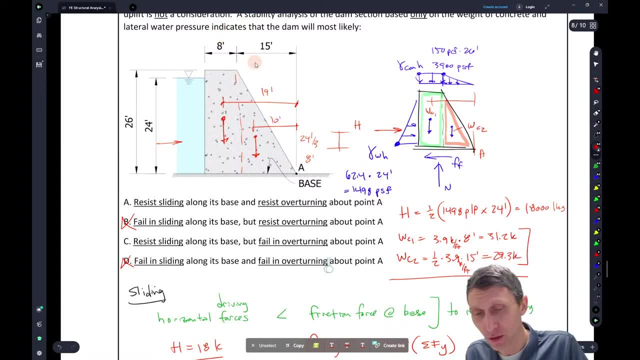 So two thirds of that, 15, this is going to be 10 feet. So we have that 19 feet. We've got 10 feet. So this is going to be 19 feet. This is going to be 10 feet. 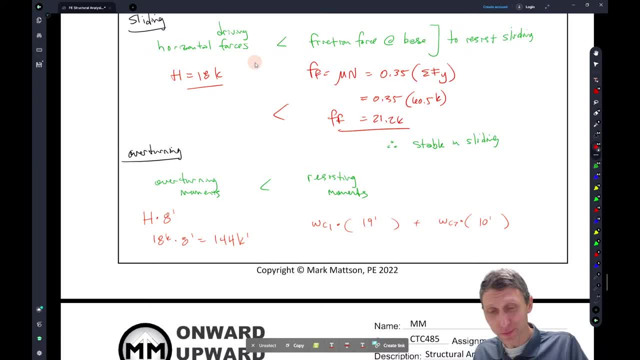 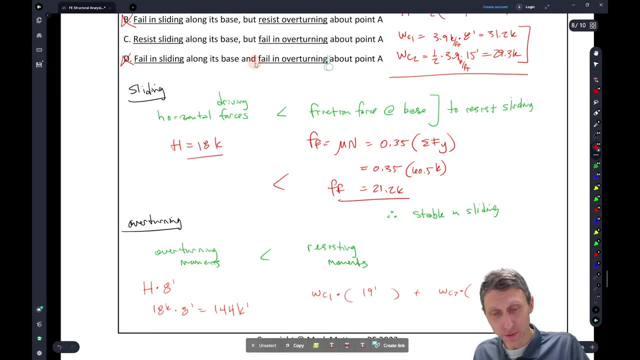 We can plug and chug this one out. And if I put the WC1 in, I think this was like what 29? I don't remember, I got to go look back. No, we got 31.2 times 19 feet, plus what 29.3 kips times 10 feet. 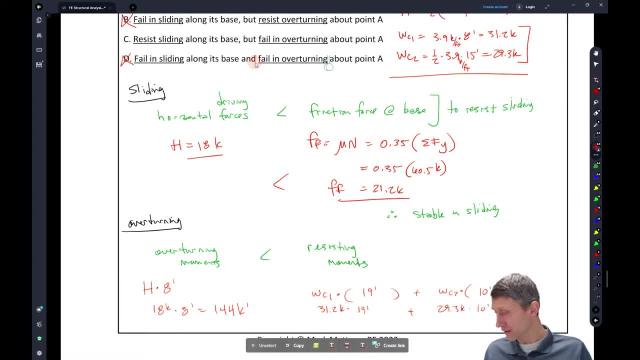 And hopefully you can see that this is just going to be a lot bigger. But the value I got was like 885 or something like that- 885 kip feet, And this is a lot bigger than our overturning moments. So that means that this is going to be. therefore, I'm going to say I'm stable in overturning. 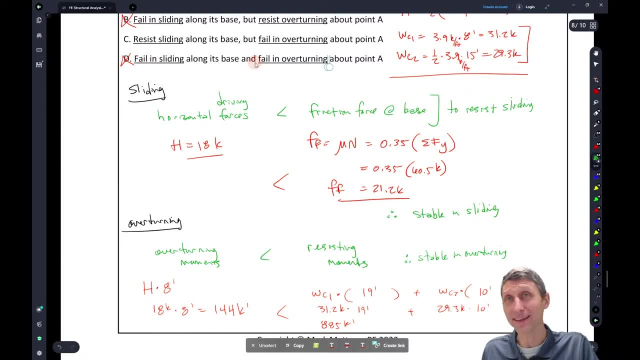 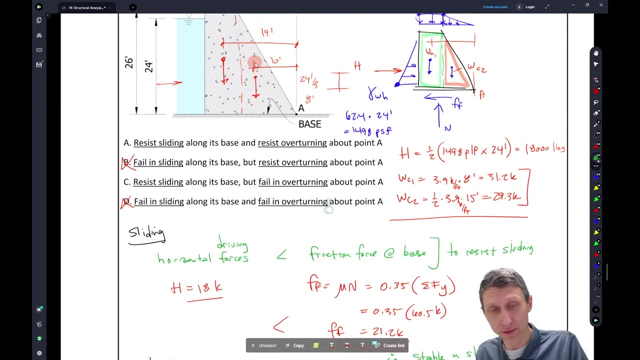 And, yeah, stability analysis get more complicated, especially when you start looking at uplift assumptions. I mean, the FERC guidelines for uplift have changed at various points over the course of the past 50 years. But what we have here is an answer that we're going to resist sliding and resist overturning. 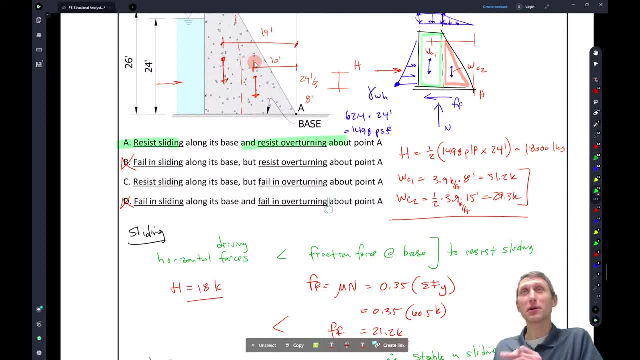 And we're stable. OK, Are we going to get a question that that's this crazy? Probably not. But you know, It just brings me back to the fun of consulting. So let's, let's go from there. So let's keep going. 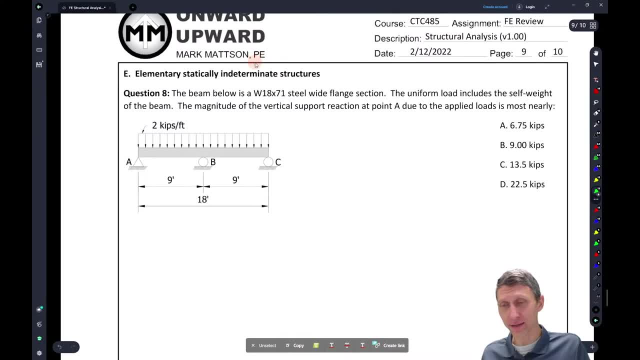 We got two more questions. These two are kind of on the sort of quicker side, But elementary, statistically, I'm sorry, statically indeterminate structures. So elementary is good, We like elementary, We like things not to be too crazy. But what we see here is if we start looking at- remember determinacy, we start looking at this: 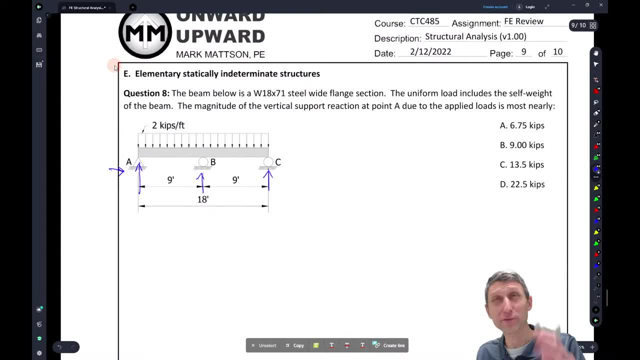 We got one, two, three, four. We got four reactions but only one beam. That means it's statically indeterminate. We have too many reactions for what we are trying to do, So this is statically indeterminate. OK, So we need to go ahead and solve this one. 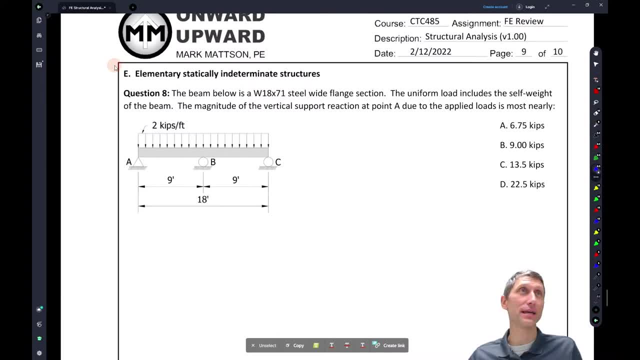 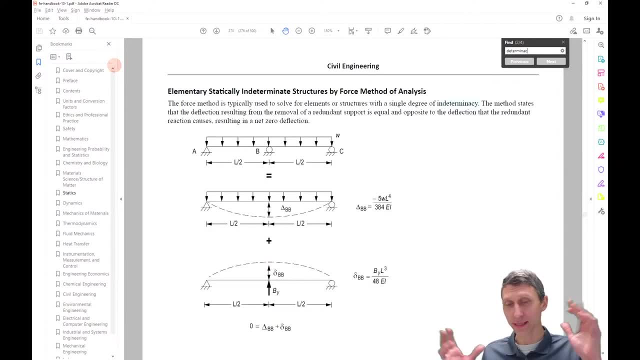 So let's go back to a reference handbook, And this is where, in the reference handbook, we actually have some things that are going to help us here. I threw this one in just because I think it's it's super, super useful. But here we have elementary, statically indeterminate structures. 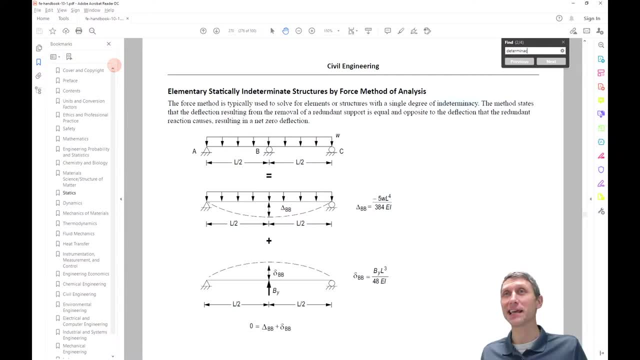 My force method of analysis Right. So here, what this is saying is it's saying like, let's take this, this, this, this roller out at first And we have some basic beam formulas for what this looks like. So 5WL to the fourth over 3D4EI. 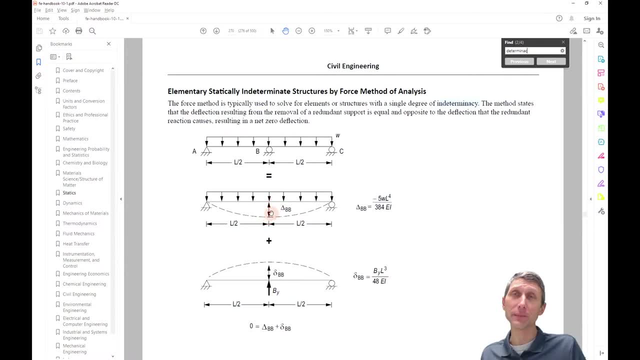 This is some basic beam formulas for the deflection at the middle of this beam without that roller support. And then the question is: what force do we need to push back up on that thing to get these two deflections to equal each other? So essentially, all that we're doing is we're going to set this deflection uniform load without that that roller equal to this deflection. 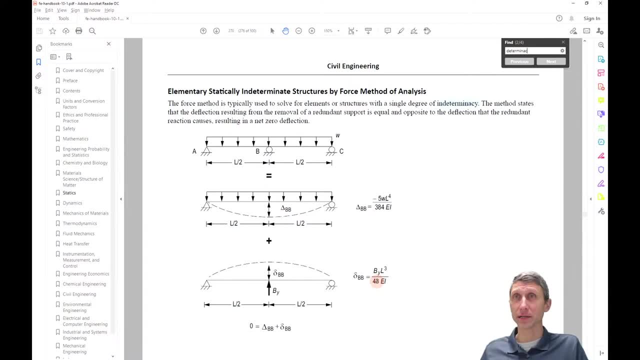 You know, this is the point load- to push it back to zero. OK, so if we know those two are going to work, basically all we're doing here is we're going to equate those two and push them back together. OK, so that's, that's what we're going to do. 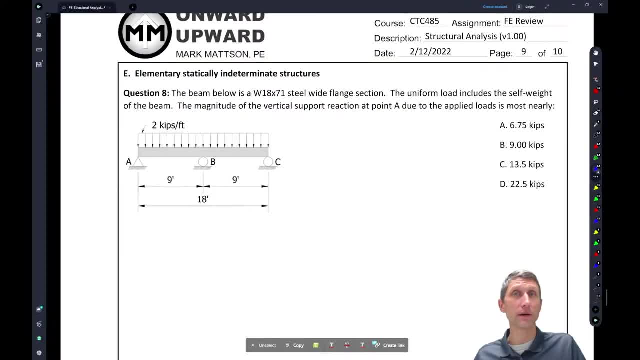 So let's write that equation down and solve it. So if we come back here We're going to say five- Let me get the right color here- But we'll say 5WL to the fourth over 384EI equals PL cubed over 48EI. 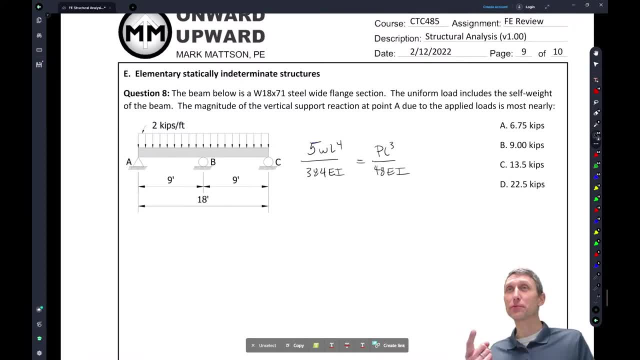 And this is so cool because somebody- I know somebody, probably because we have it- we're given a steel beam here. Somebody probably went and looked that up in the manual, So I'm going to go find I. But the good news is, look at this. 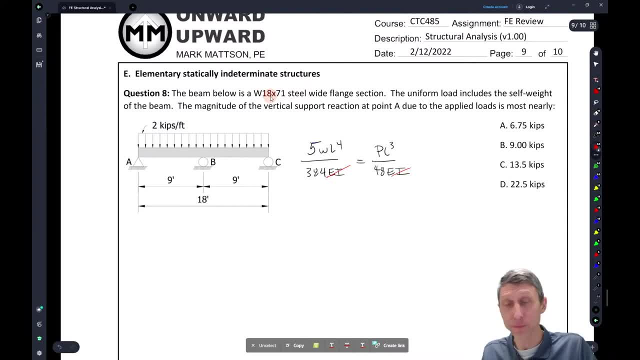 Look at this: E and I both cancel out. In fact, not only E and I cancel out, but we have three of the L's that cancel out. So when we look at this, what we're left with is just 5WL over 384 equals P over 48.. 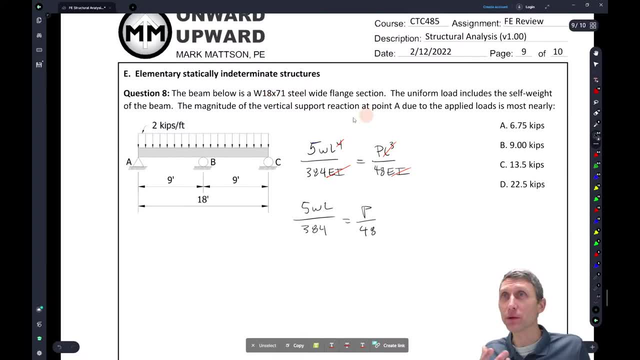 You see it? So? so this gives us something. But what are we asking for? The magnitude of the vertical support reaction: A. So so we need A, But this is going to give us B. OK, this is going to give us B. 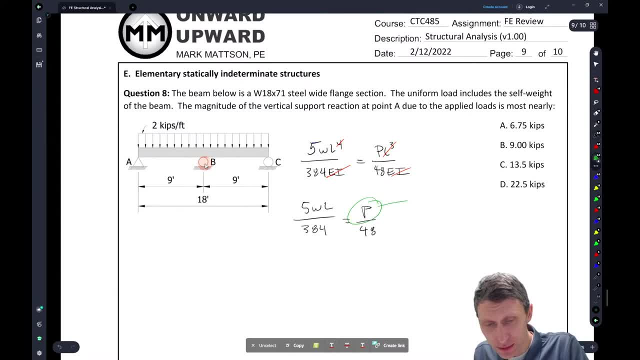 So P, in this case, equals. This is the reaction At B. OK, that's going to be helpful to us because we need to get there first, And this is how we're going to go through this process. So we're going to start with this and we're going to plug in. 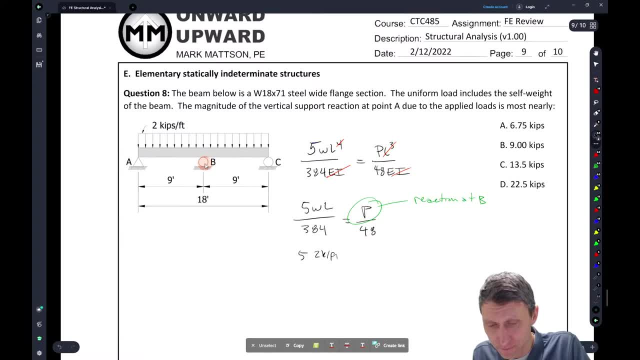 So five times W, which is two kips per foot, Times the length, The length is going to be: the total length of 18 feet divided by 384 equals P, Or I'm just going to call this BY Right. This is, this is really that reaction BY. 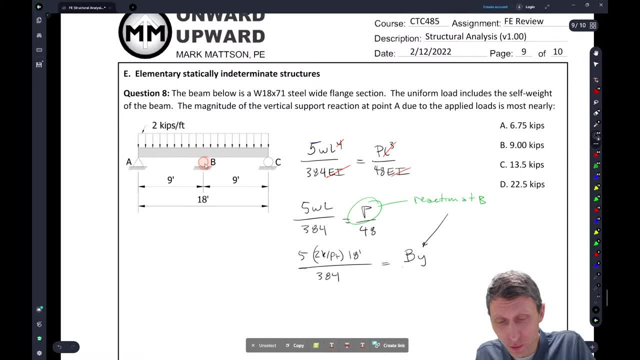 OK, so BY over 48. And rather than doing over 40, I'm going to cross, multiply by 48 and just put the 48 on this side. So now I can directly solve for BY. So BY is going to equal. 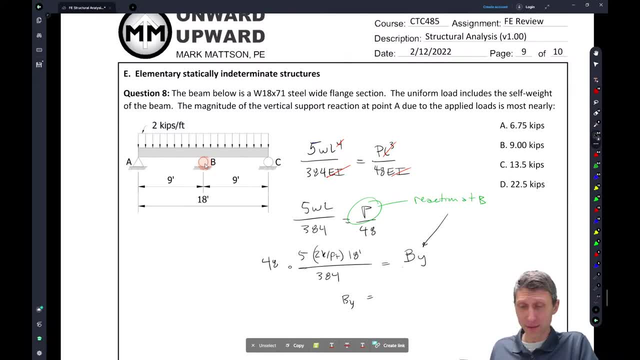 I did this right. Let's look: 48 times five times two times 18, divided by 384.. I got twenty two point five. Anybody else get twenty two point five, Twenty two point five kips. So that means this, this: you know, this force in the middle is twenty two point five kips. 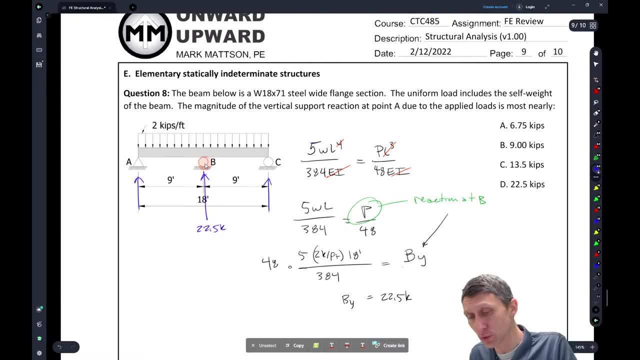 And then we've got two forces here, And this is symmetric too. So so what you see here is this: AY and CY- due to symmetry, They're going to be the same- And how much total force we have acting down. Well, two kips per foot times 18 feet equals what? 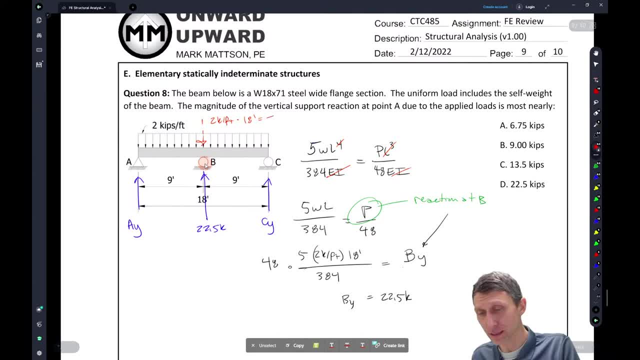 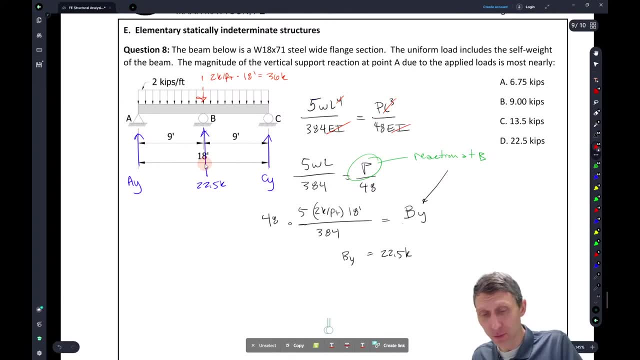 So two times 18 gives us a total of 36 kips. So now we have one thing left to do. All that we really have left to do is we. we just have to say, OK, let's, let's go here and let's just some forces in the Y direction. 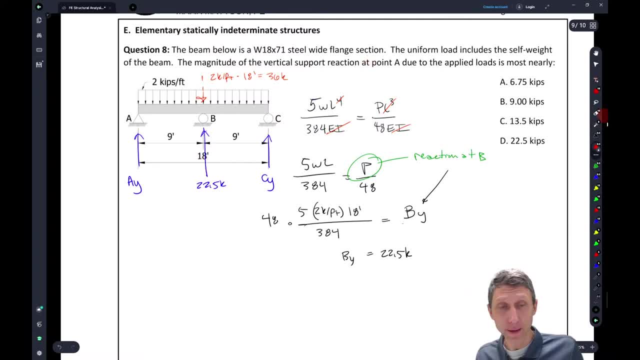 Come on, Not wanting to click, for me We can. some forces in the Y direction, Some forces in the Y direction equals zero. And what do we get Right? So we get AY, essentially AY. I'm just going to say two AY, because AY, you know, by symmetry, AY equals CY. 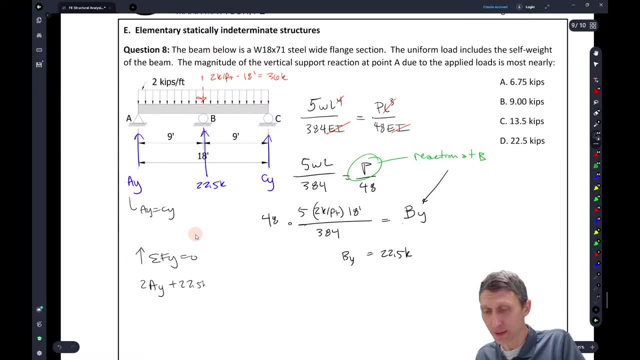 Two AY plus twenty two point five kips minus this thirty six kips equals zero. So we get AY equal to what Thirty six minus twenty two point five divided by two, And I get AY equal to six point seven five kips. 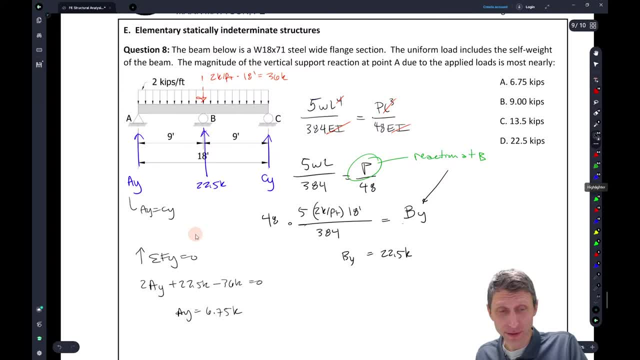 Which, fortunately for us, It's a good idea, But it's also an answer here, OK, So I will highlight that and be happy with it. So, again, what we got to do here is we have to, we have to know kind of like where to how to deal with these elementary statically indeterminate structures. 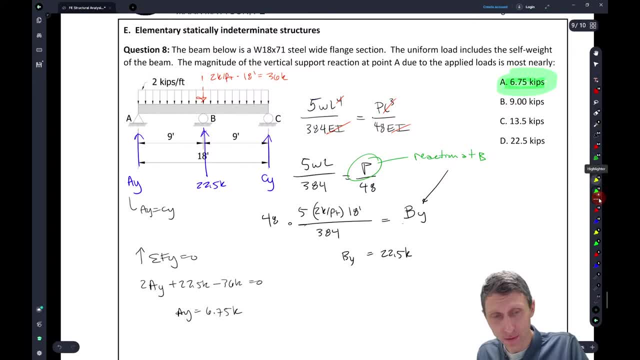 We have to recognize we can't just take like a tributary area here. OK, just take like a tributary area. uh, and, and solve this. sorry, my mouse stopped clicking, this is just annoying me. but um, like, we can't just take like, oh well, we're gonna take four and a half times two. 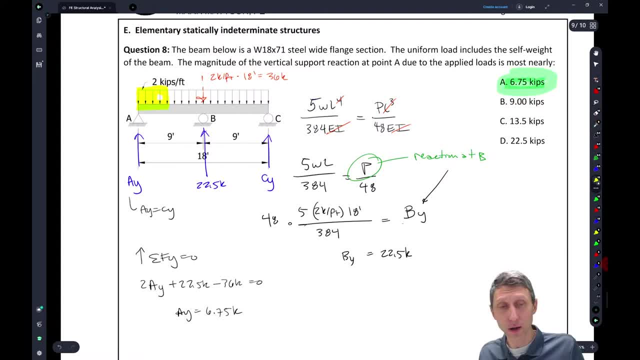 and that would give us nine kips, which would be uh, which would be wrong, right. so if we do, uh, the nine kips, that's wrong, right. four and a half times two, that's an easy answer to get, but it's the wrong answer. so don't, so don't, go down that path. it's not just a tributary with you know half the 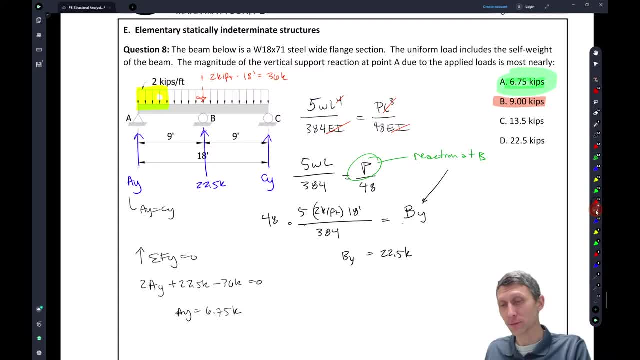 distance 4.5, and and that's because the, the force of this middle support does, uh does get a little bit bigger based on the, the, the way that this beam um acts continuously. okay, so let's keep going. we got one question and then we will uh be done, if let's see if my computer wants to respond here. 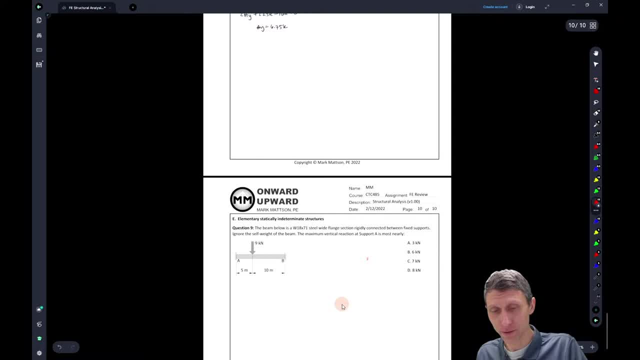 maybe we'll, uh you, if not, we'll, we'll come back and do this one another day, um, or i'll i'll shut it down and restart it, i don't know. but, um, let's look and see if i can make this happen. we got one left. 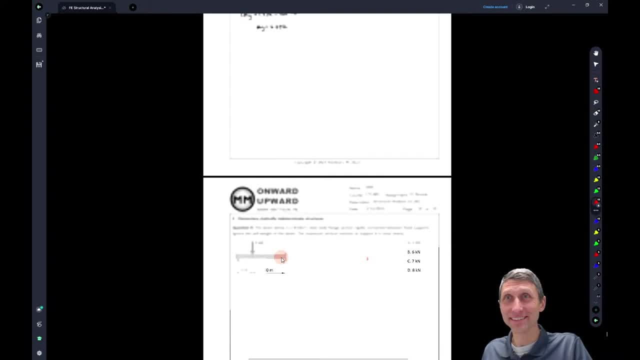 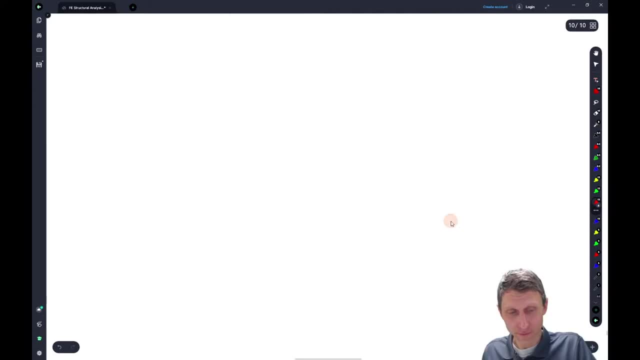 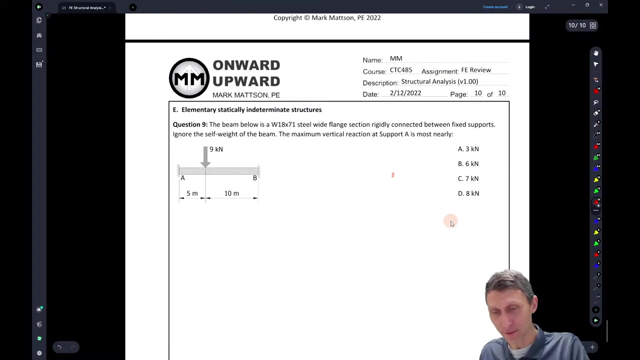 and, uh, it's not liking me here, okay, um, maybe, okay, i think we're, i think we're making it work, okay, uh, there we go. sorry about that, let's see if we can make this work here. okay, so, statically indeterminate structure. so again we have. 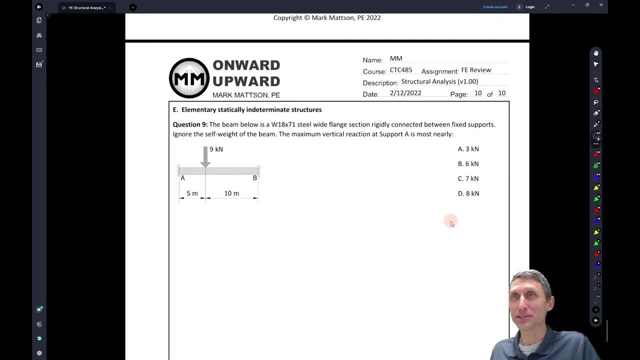 a beam. we've got a statically indeterminate structure here. we've got too many reactions. we got three fixed reactions on one side, three on the other side. we only got one beam and we gotta. we have to figure out how to solve this. so again, when we come to our, our um, our problem here, 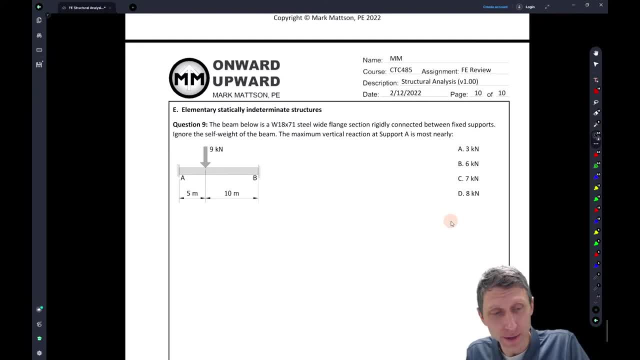 what we're gonna do is, well, let's just first draw a free, dissociative body diagram and see what this free body diagram looks like. so if we take this thing, um, i'm gonna draw my free body diagram i got. So if you take this thing, i'm going to draw my free body diagram. I got what a, y and x and y. 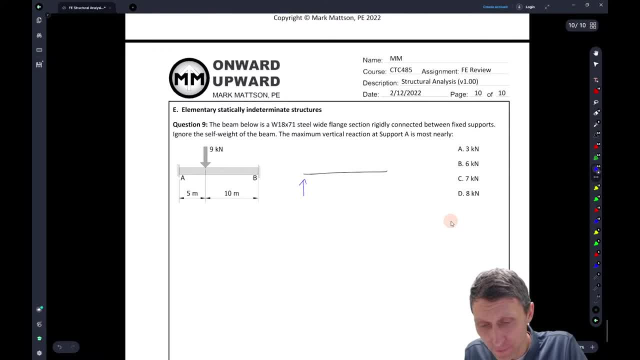 E consecutive ever day, είναιn kalminijthing. the only word we're going to need to do is probability elegant, and let's see what we can to do so before. everything should change as well, because in from we're my free body diagram. I got what a, y, b, y, a, x, b, x, and some of you are just tempted to stop right. 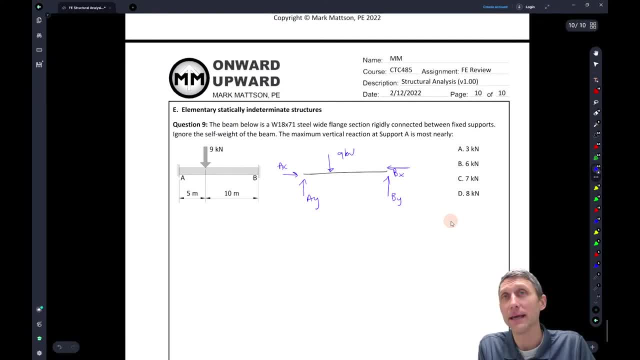 there because it looks easy, but don't do it because it's going to cause problems. okay, don't do that, it's not going to work. but what we can do here is we have to remember: don't forget your mother, didn't? I say that already? but what we have is some moments here. sometimes you'll see this m a. 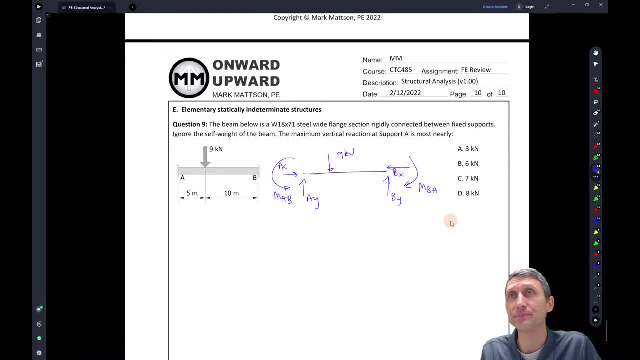 b and m b a, depending on your sign naming convention. but you have to deal with those moments so you can't just take like some moments about point a and solve because we have these two fixed end moments that we don't know. so that should ring a bell right when I say fixed end. 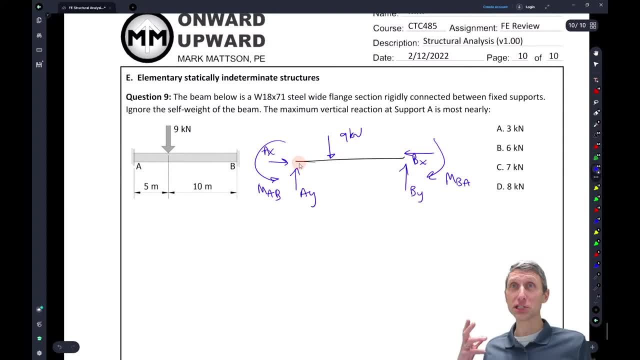 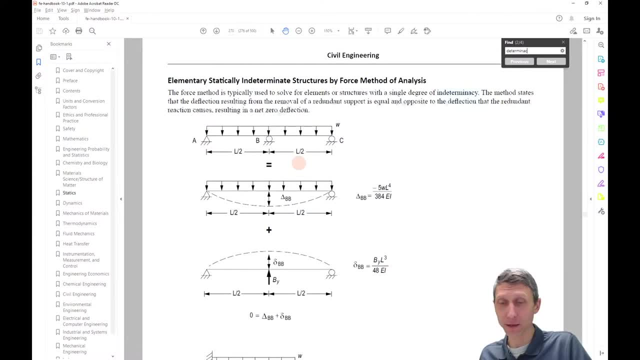 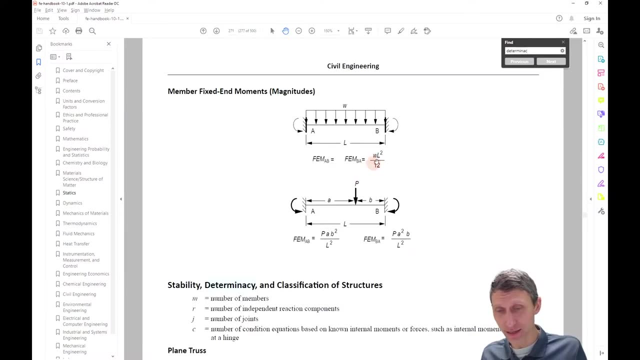 moments. that should ring a bell that there are fixed end moment sheets. do you remember those? so if we come back- and again we're back into this, this, the reference handbook- if we come back into here, we have some fixed end moment sheets and I can hopefully find this, can I? there it is, we get. the cool thing is like maybe the book we use is has like a whole 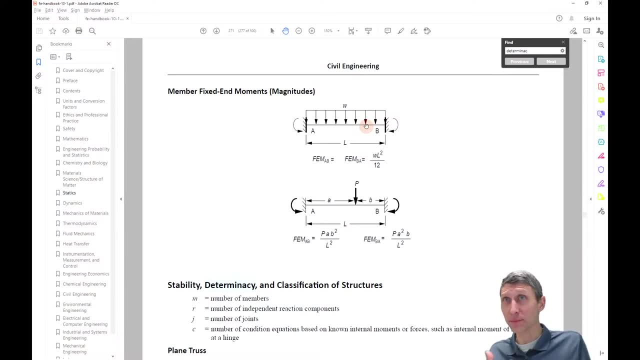 table of them, right? the reference handbook only has like two fixed end moment sheets. so if you're looking for a big long table, they're not going to be there. this only has two. so we got WL squared over 12 for uniform load with between fixed supports, and we got PAB squared over L squared. 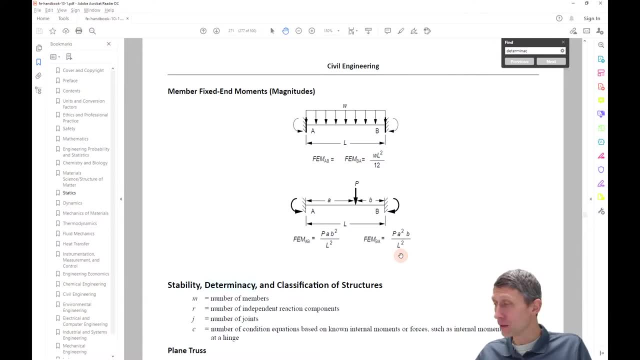 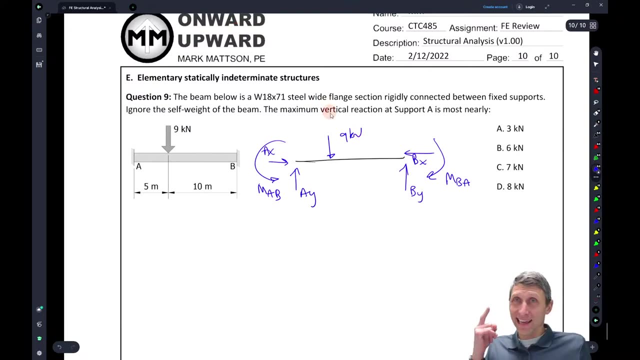 and PA squared. B over L squared. that's it. and you might have noticed that we have a little bit of a shift in the reference handbook and you might be thinking like that's great mark, but this asked for vertical reaction. didn't ask for a moment. in order to get the vertical reaction, you have to find the 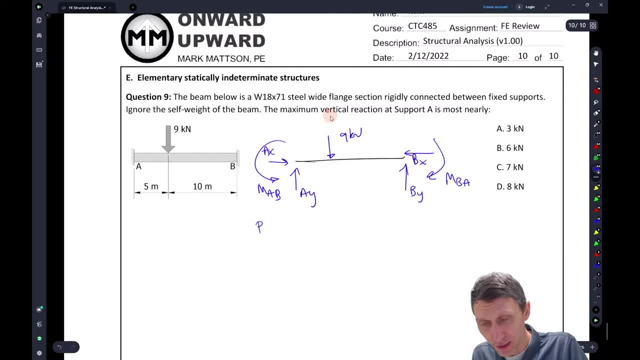 moments first. so if we take a look at these, we're gonna have formulas P- I think this was P- P a- B squared over L squared and P a- B a squared over L squared. so those are those moments and this shouldn't be so. those are those moments and this shouldn't be. 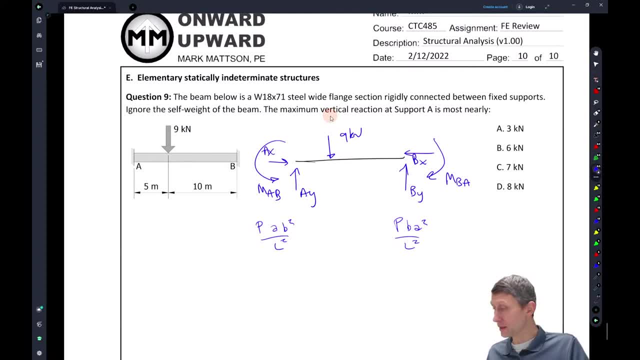 super, super tricky to plug in. we should be able to plug those in right away and solve. so let's, let's. this is going to give us our moments, which we'll then use to go get our vertical force. so let's, let's just plug in here, and what do we get? we get nine times nine kilonewtons, times a, which one's a. 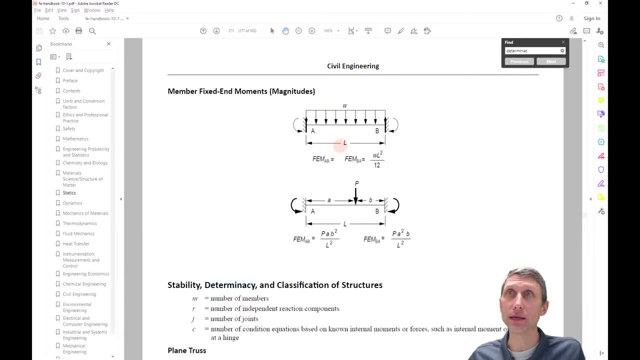 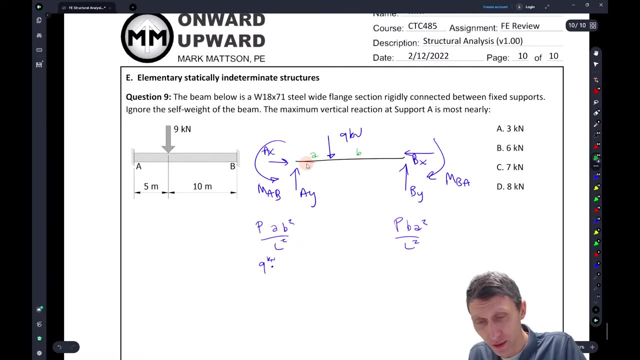 okay. so if we come back to our diagram here, a is on the left, b is on the right, so a is going to be on the left, this is going to be a, this is going to be b. uh, so what do we have? we have the five. 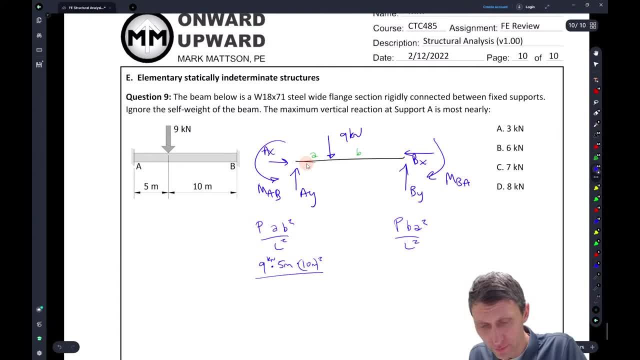 meters times 10 meters squared, divided by 15 meters the total length squared, and we can just keep coming down here and install what's nine uh times five times 10 times 10 divided by 15 squared, so i got like 20 kilonewton meters here. so that's at the moment of ab. 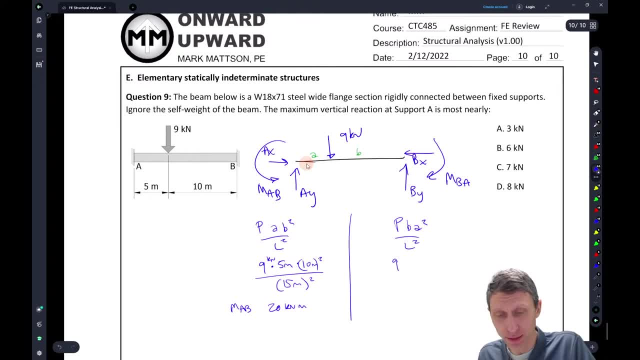 okay. and then on the other side, uh, let's see the other side here. so p nine kilonewtons times 10 meters, times five meters, uh, squared all over 15 meters, uh, and we'll square that. so if i plug that in nine times ten times five, squared, uh, divided by 15 squared, i get 10. the moment of ba is 10. 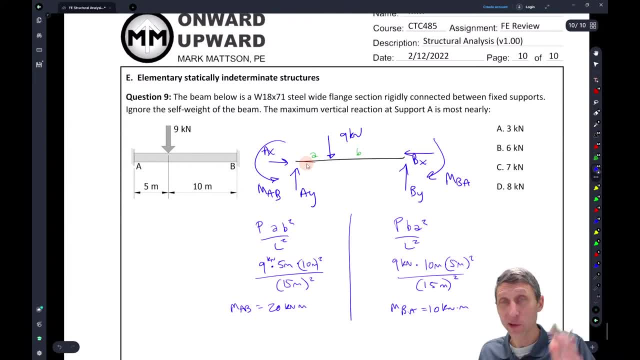 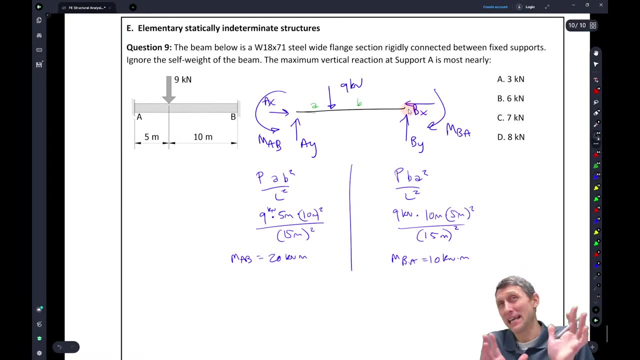 kilonewton meters. once you have that, what are we finding? we're finding this um, the reaction at support a. okay, so the good news is, if we have the reaction at support a, we can some moments at point b, normally like some moments today, if you like to some moments today. go ahead, some moments today and then some forces. but here i'm. 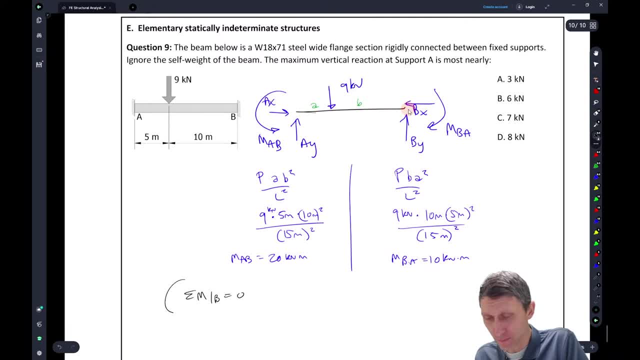 just going to some moments. at point b, this is going to equal zero. anything that's that's you know, in this direction is going to be positive. so i'm going to start with m a, b. that's positive. okay, this one's positive. then i'm going to have minus a y. 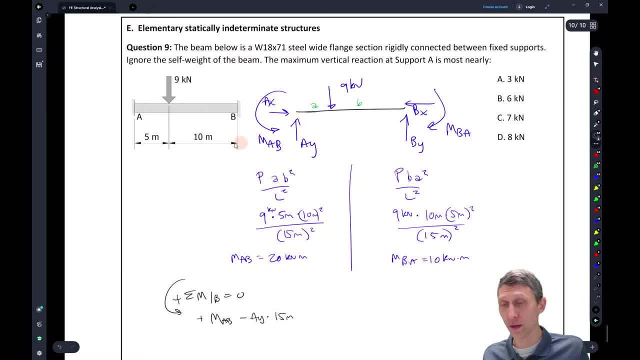 times 15 meters, the whole the whole distance here. and then i've got this nine kilonewtons. so i'm going to add in nine kilonewtons times 10 meters. i'm going kind of fast with those signs there. but again, rotation it's causing counterclockwise rotation, which is positive. and then what else? 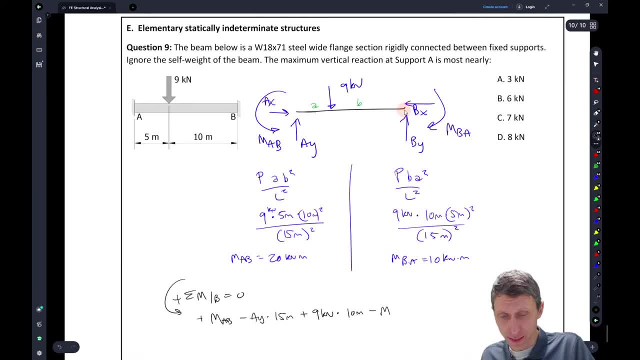 the only other thing that causes a moment here is mba, and i'm going to say minus mba, because that's causing clockwise rotation has to equal zero. we got one unknown and we're done okay. so we got one unknown, let's go solve it, send it, crush it and, uh, i don't know. 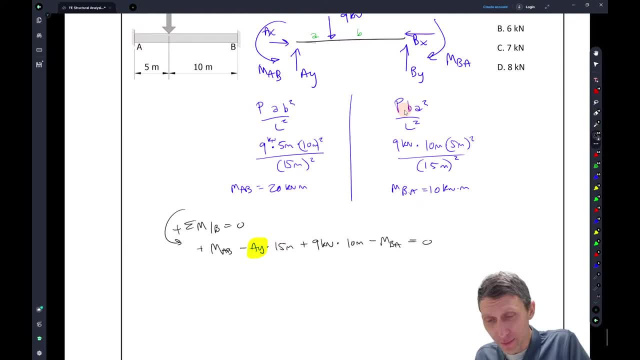 go win the gold. um, so what do we got? we got mab, which is 20 kilonewton meters. i'm going to put this whole term kind of on the other side of the zero. um, just to make it easier- times nine- actually, i'm just gonna say nine times 10, is what? 90 kilonewton meters, and then minus this, 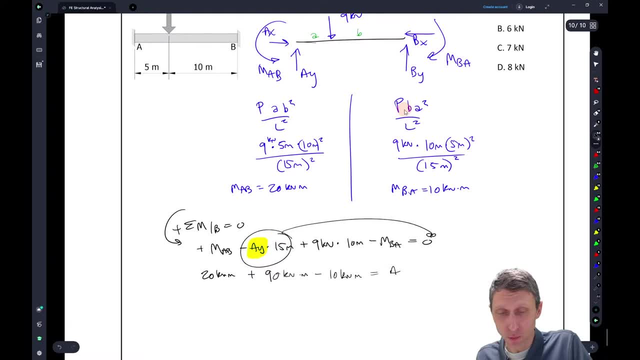 10 kilonewton meters. uh, equals what a y times 15 meters. so we're gonna get a y equal to what's this? we got 20. it actually works out kind of nicely, doesn't? 20 plus 90 minus 10, that's 100 divided by 15, is going to be what 6.7 kilonewtons. 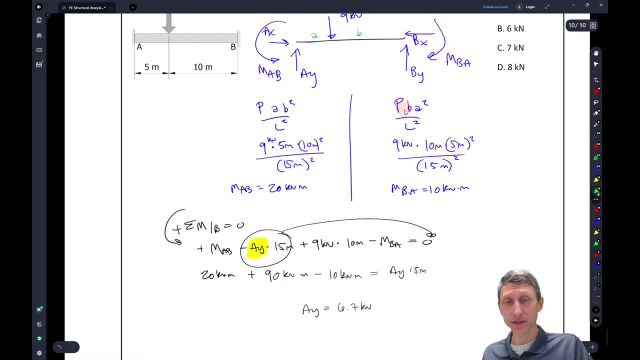 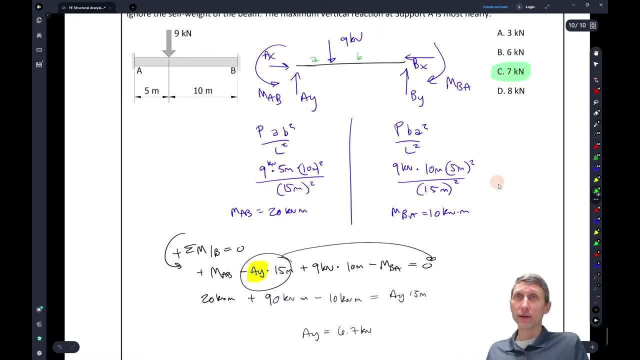 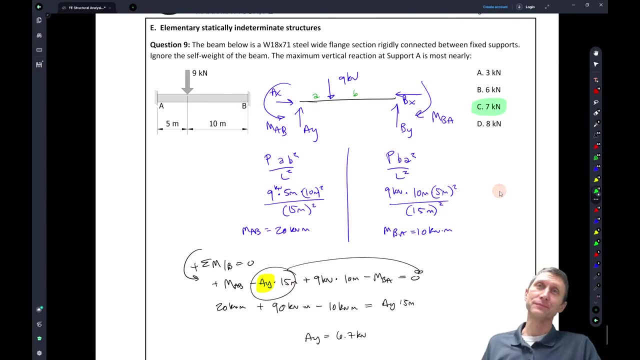 so, and most nearly, most nearly, we're in between the the six and the seven, but most nearly is going to get us to seven, okay. so, oh man, elementary statically determinant structures. did we have to do like moment distribution or, like you know, some other crazy, crazy method? no, we didn't here, but we did have to understand. 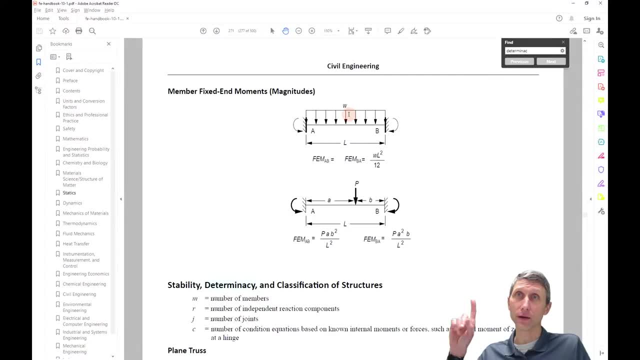 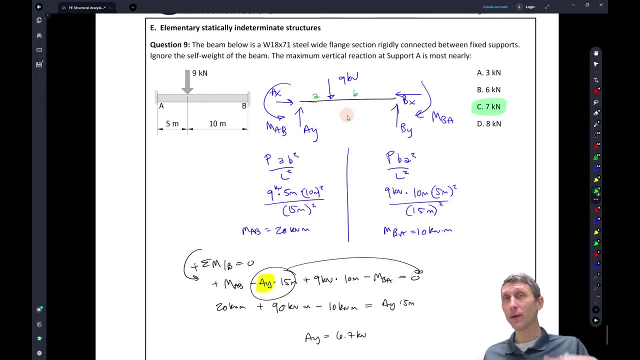 that, that moment, or the fixed end moment diagram up here, right up there. we had to understand that diagram. we understand how to put it in, how to solve it, but also what to do with it once we did so. man, there's so much in in structural analysis. i wish i could teach a whole course on it actually. 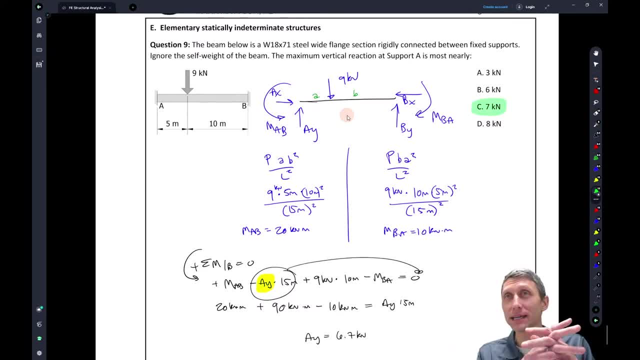 um, i do, but that's. you know, it is what it is. it's. it's: in structural analysis, you're probably going to end up using more reference handbook resources to a certain degree than in statics. right, you're going to have to go look up some moments of inertia. you're going to have to maybe do some more unit. 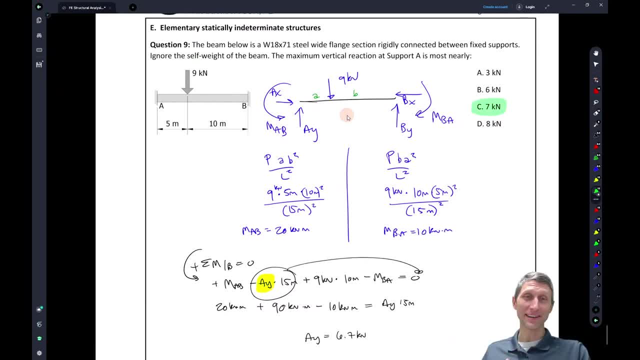 conversions and that sort of thing. but that reminds me of a story. okay, this is all done. actually, this reminds me of a story. my grandpa, he's like a hundred now, like literally, like legitimately a hundred. he sends jokes every once in a while and um, and he, he sent this joke. so matt. to answer your question, yes, this is totally. i could totally see. 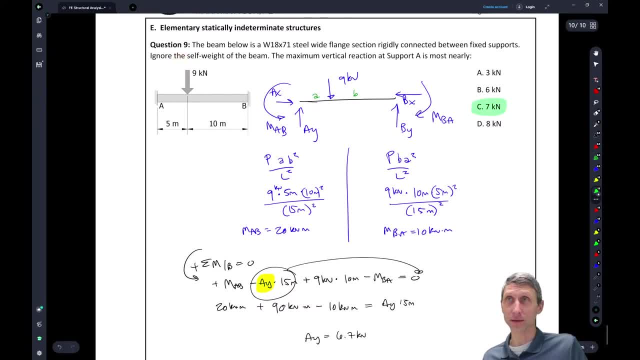 this question on the fe 100, like this type of thing. this is a elementary statically indeterminate structure. i could totally see something like this on there. i don't know they give you these these rough, these formulas. i could totally see something like that. it's not super crazy. 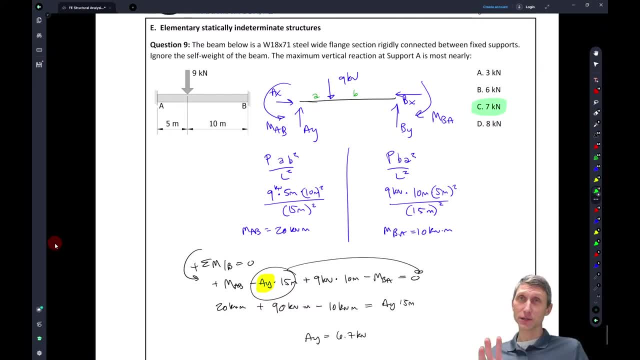 um, but in case you don't have resources, you might think of this gentleman. um, this is from my grandpa. there's a gentleman who's a professor at the university of america and he's a professor at the british department. um, can't uh graduate here, um, but um. but he a woman who, um, who was sent to jail. 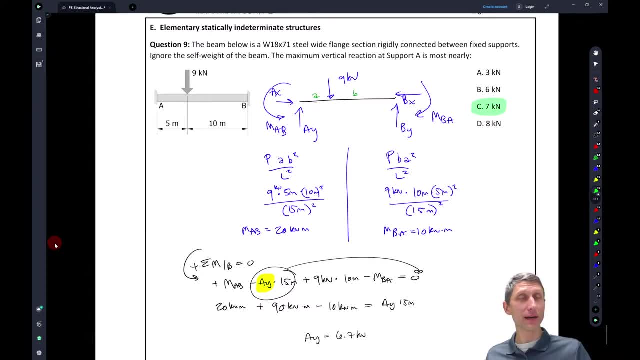 and he was really sad because his dad, uh, he'd always planted a garden. his dad was getting older and he normally dug the garden up for him. uh, but he couldn't because he was in jail. but he still was able to use his resources because he, um, he sent his dad. he said, well, his dad sent him a letter. 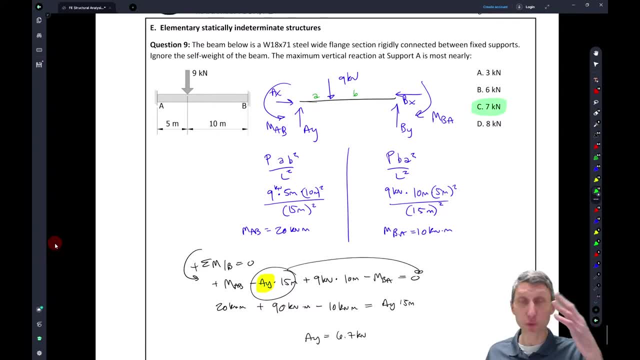 and said: hey, i'm feeling pretty bad because i can't dig up my garden. i'm getting too old and if you were here, not in jail, you could do it. so his son sent him a letter. he said: dad, dad, don't dig up the garden. that's where i buried the barn. 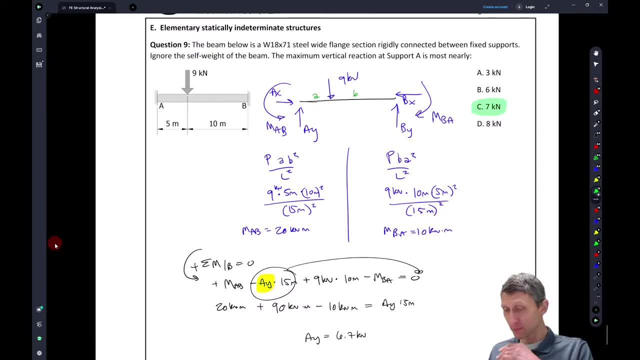 bodies. love your son. um well, at 4 am the next morning, fbi agents and local police arrived and dug up the entire garden without finding any bodies. um, they apologized and the old man left um. the same day, the old man received another letter from his son. it read: dear dad, go ahead. 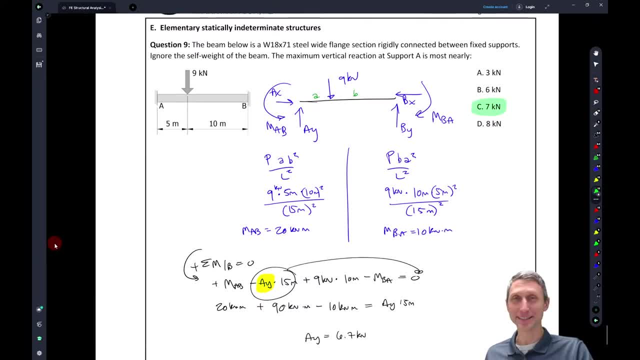 and plant tomorrow. um, the garden should be dug up now. it's the best i can do under the circumstances. i gotta love my grandpa. you know what that guy was resourceful. even though he's in prison, he, uh, he made use of it. um, honestly, you guys are resourceful. i know you can do this, this, this. 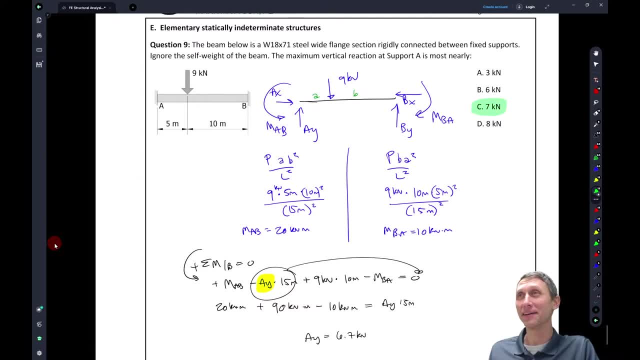 type of question isn't too crazy. it's something you can make work. but, oh man, i appreciate you tuning in here and going through some of these problems with me and, uh, hopefully, if nothing else, the joke is worth it. you know, i'll try to come up with a good joke. maybe it's not good, but 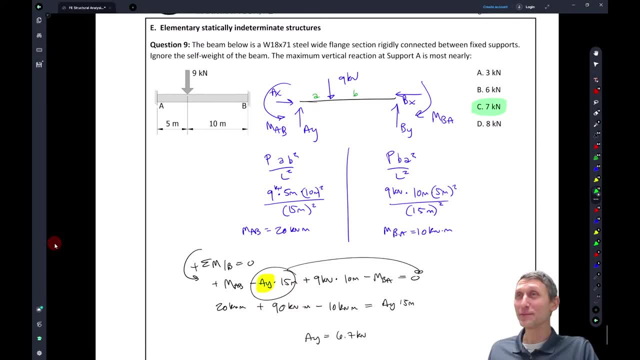 it's, uh, it should be fun. so, hey, um, if you guys have questions or you're in my actual class here, feel free to stop by tomorrow. i've got some time middle of the day so i'd be happy to to chat with you. but, um, you know, we can, uh, we can- go from.